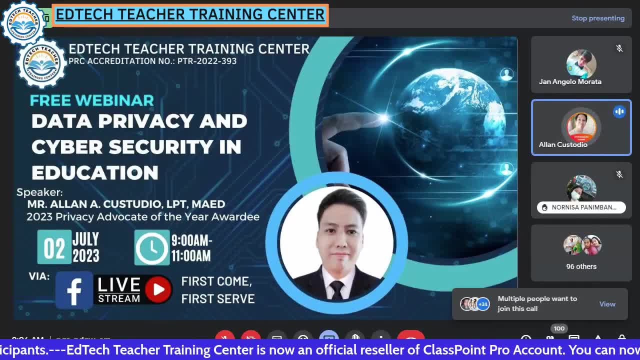 agad at usually hindi nila alam kung ano ang mga batas na nakapalawag. So for this moment, let me share po yung screen para makapag mag-engage pa tayo sa ating mga matatakel ngayong. 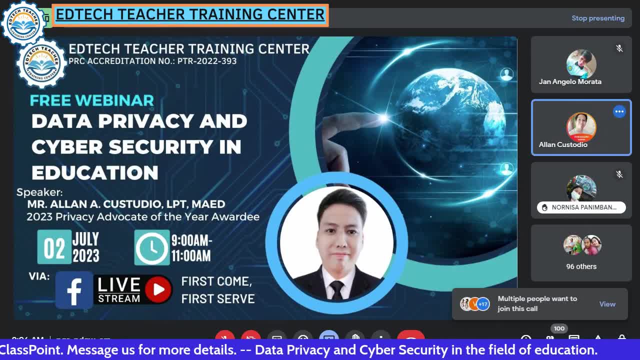 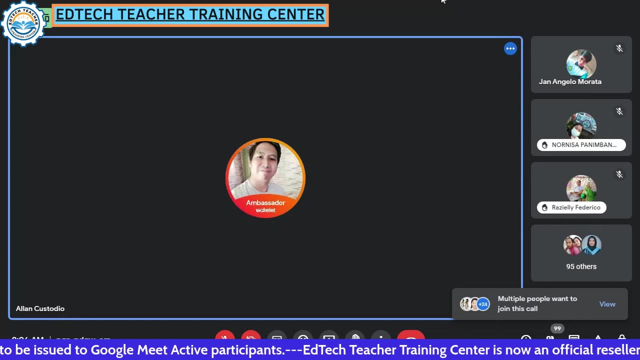 araw na ito. Okay po, Let me share po ang aking screen. Wait lang po. ah, Okay, so ayan, Share ko lang po ang ating screen para makapagkulang Collaborate tayo. So alam nyo naman po no sa ating mga talk. ang sineshare natin lagi ay ang: 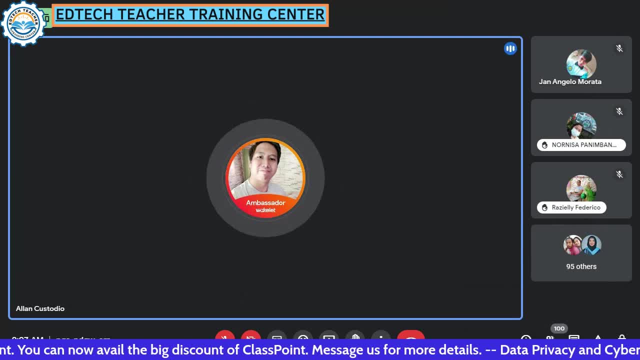 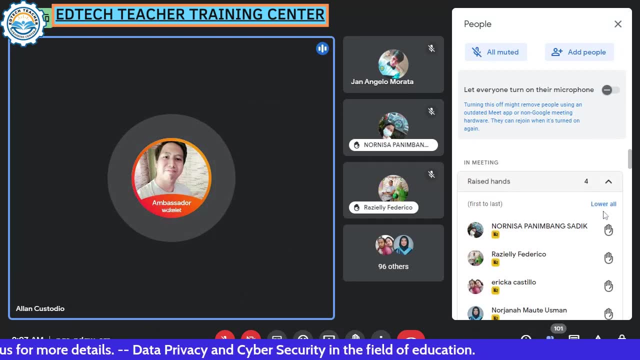 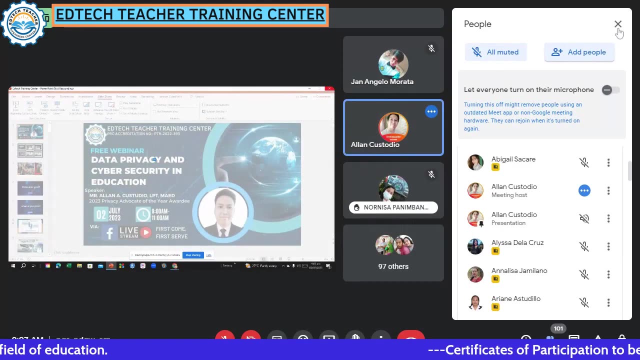 class point: Okay, So yung class point po ang gagamitin natin ngayon. Wait lang po ng konti At naulit ka po na Good morning. good morning sa ating mga naka-attend dito Ibat-ibang lugar. 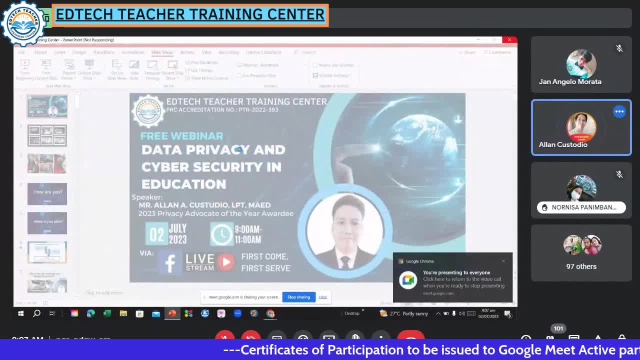 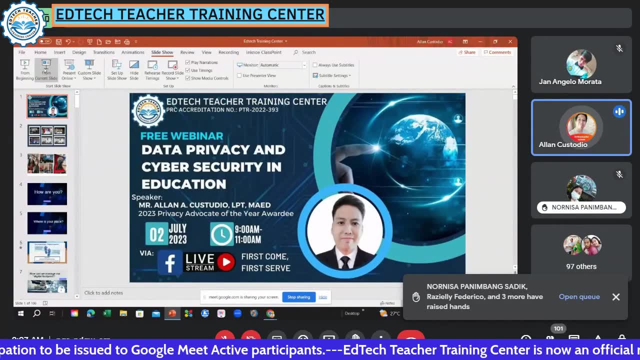 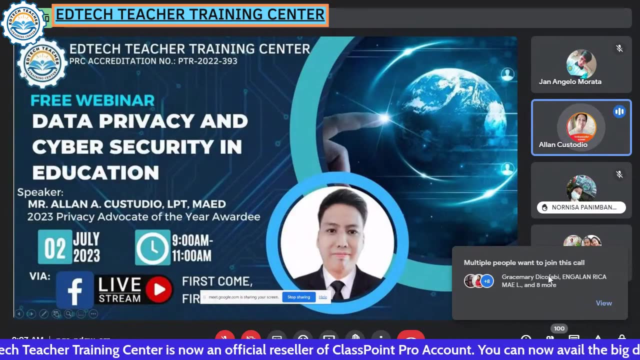 So hinihintay ko lang po mag-open yung ating class point Ayan, So from current slide Ayan. So magtuloy na po tayo, at sana po ay maging okay naman ng lahat, pati ang ating code Ayan gumagana. 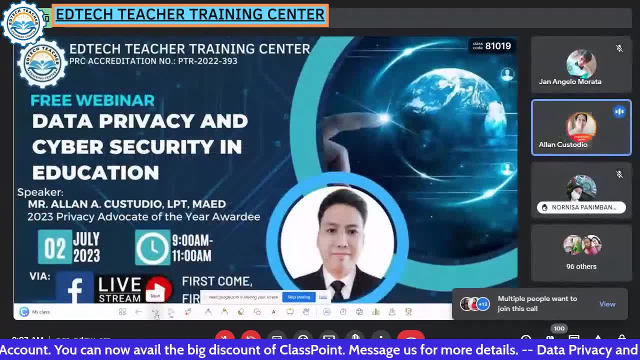 So, sa pagpapatuloy po natin, ini-invite ko po kayo na mag-join sa ating code na 81019.. Ayan, So, Iki-click po po ito Sige, I-click po natin yung code Para po makasali tayo, makita natin mga sasali. 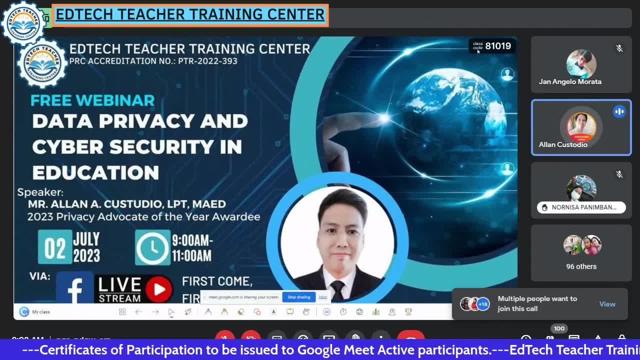 At medyo Sunday po. no, Alam ko ay yung iba'y galing pa ng mga simbahan, At mukhang may isa na po naka-join. Ayan, no Shout out po sa FB viewers natin. Mukhang ah, kiniklik ko, Mukhang ayaw. 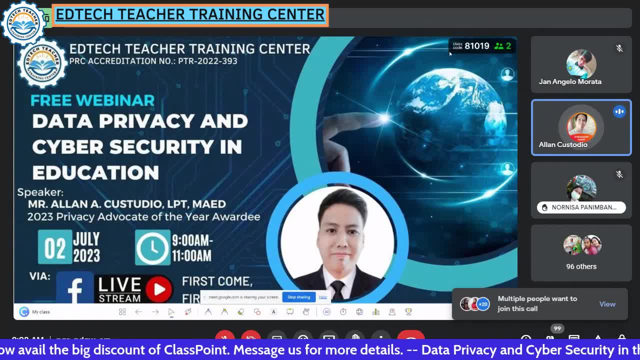 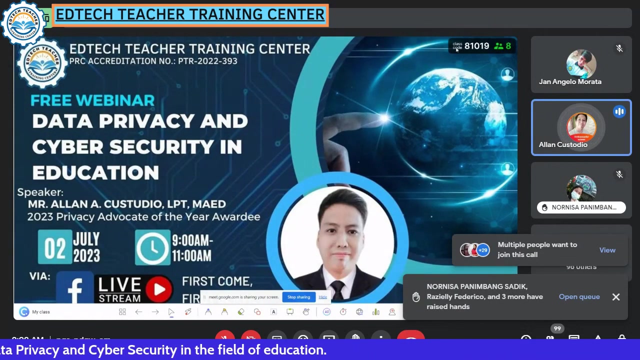 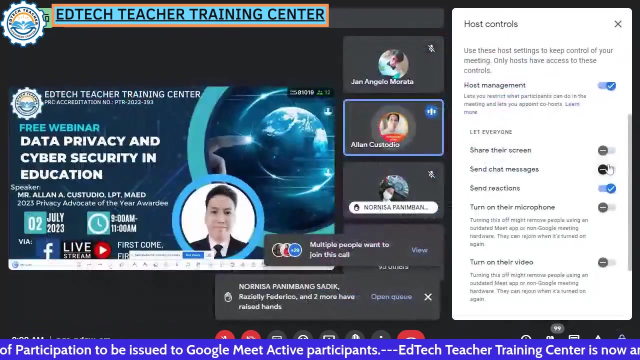 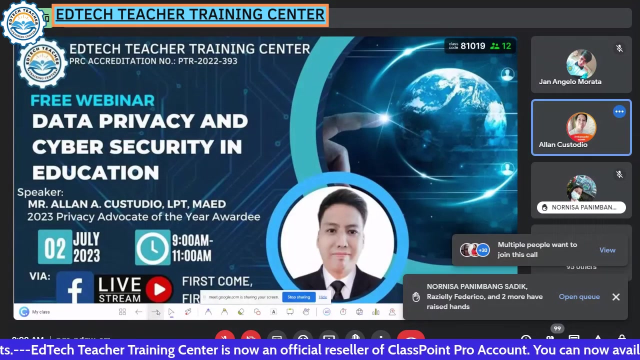 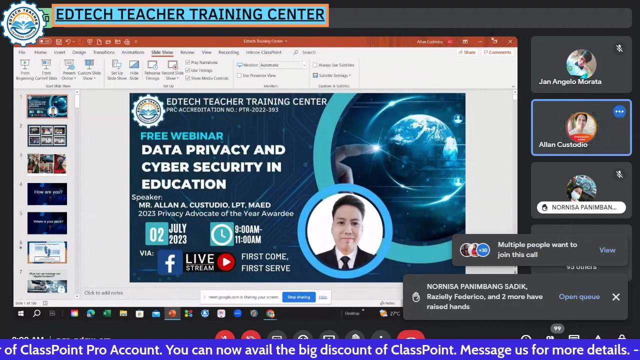 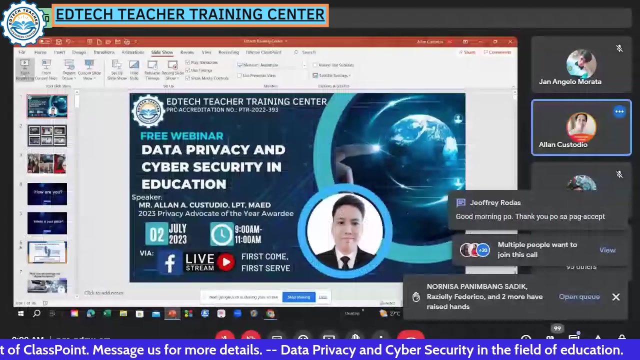 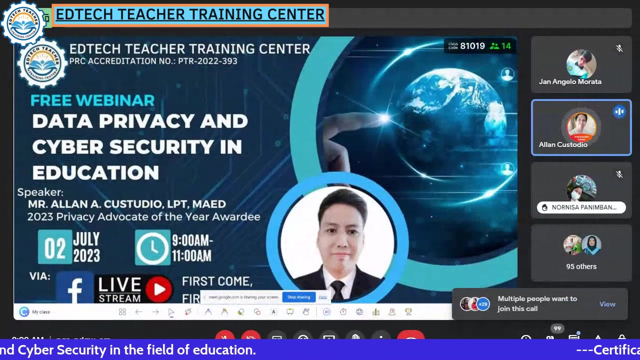 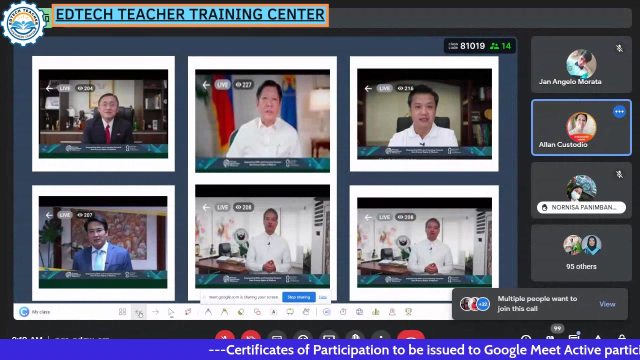 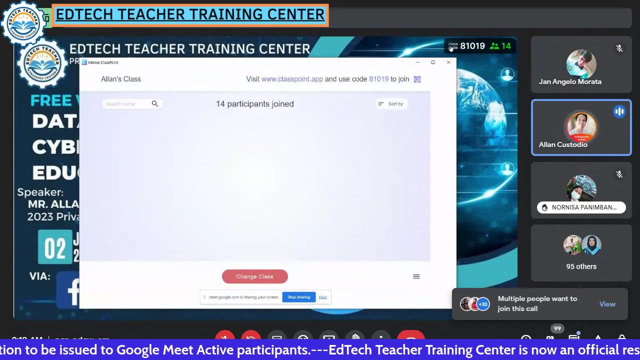 po mag-join. foreign ayan, foreign ayan, uh, um, foreign. okay, this is a day for all of us. we have 14 participants and hopefully it will go straight. I will just go back. we have code 81019, we have 14 participants and I know. 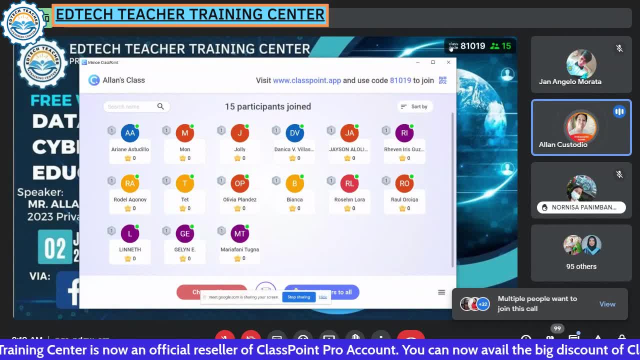 others can join wwwclasspointapp 81019. if you want this kind of presentation, just visit classpoint community. we are the same classpoint certified trainer. we can reach out to you. if you want this kind of presentation, avail use COT. we have promo now. 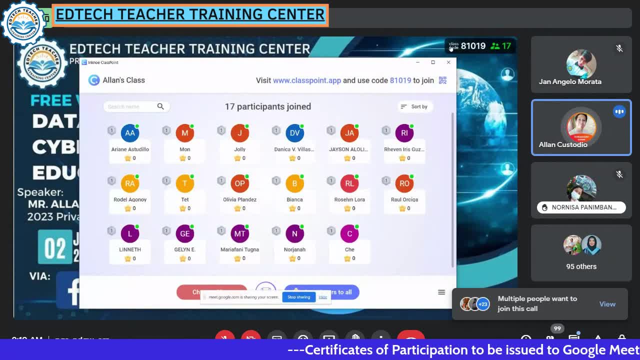 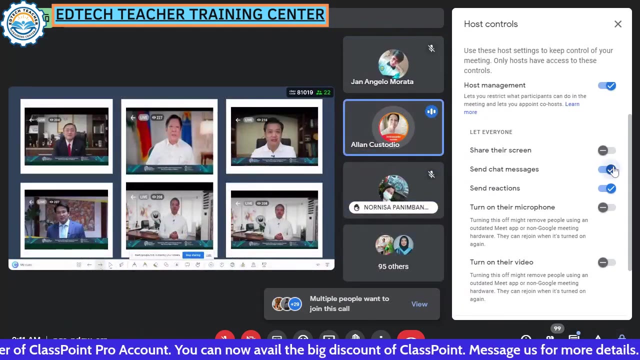 you know, we always use classpoint teachers and government employees who will go to the new 81019. we have 11 and don't move. we will give you information and let me cross this one to continue. so, in regards to data privacy, this is attended by 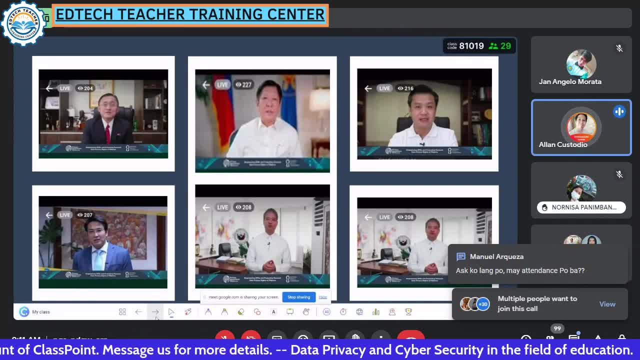 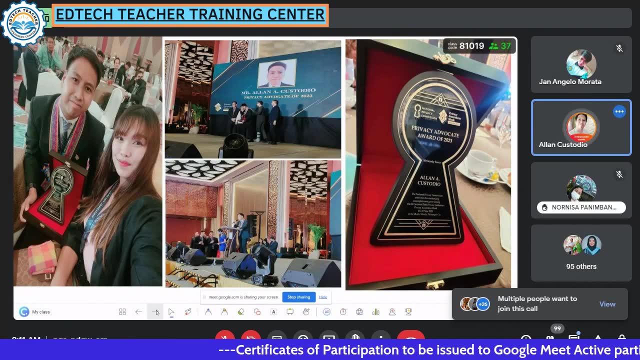 our honorable excellency, sir Bongbong Marcos, and other cabinet where they gave speech and we as teachers, we were chosen. actually we have a lot of enemies, but I said all of them are deserving, but there we were given by the Department of Education. okay, so before we, 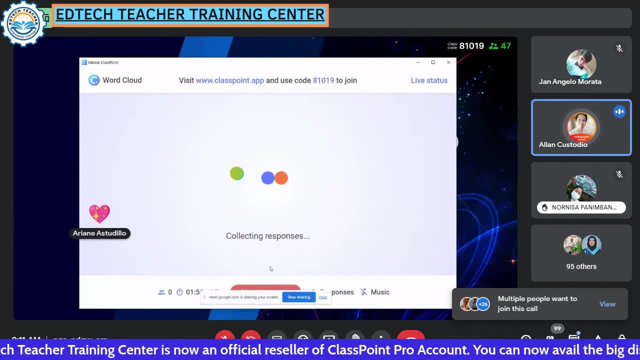 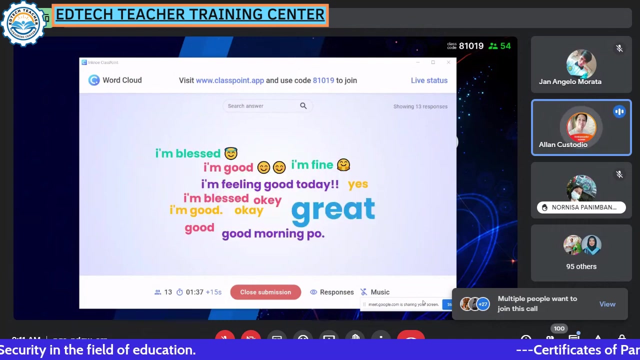 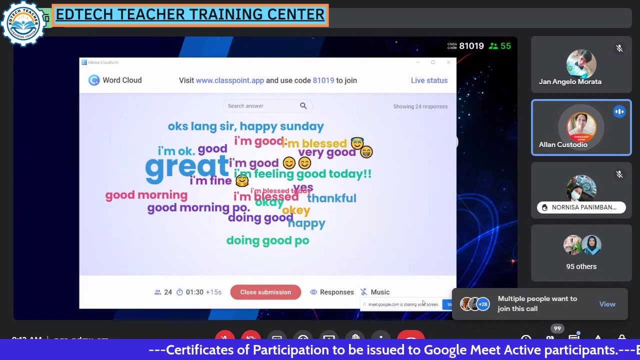 really start and now my presentation is okay, then how are you all? how are you all? if you can't enter below 81019 there, great, I'm okay there. how can you enter classpoint? go to google wwwclasspointapp and use 81019. the other teachers. 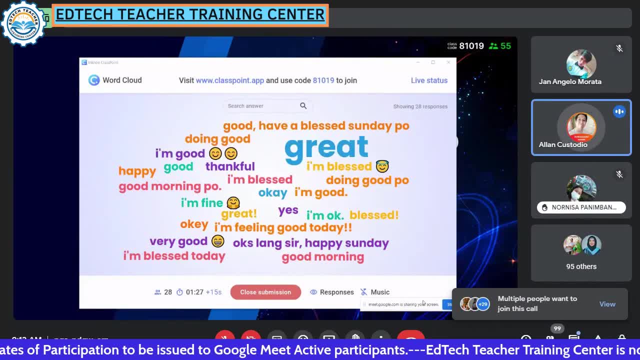 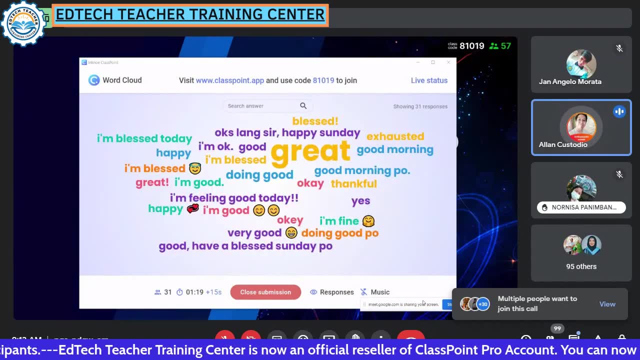 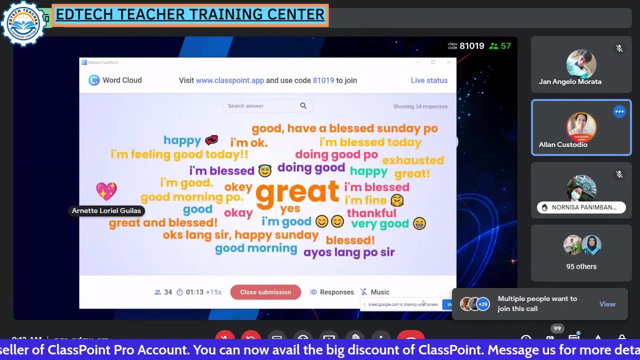 they are really scared and some of them tried. but I repeat, if you leave your comfort zone, you will get better. do you believe that you will get better, especially if nothing will happen to you? what will happen to you is counting time effort. of course you really need to sacrifice. 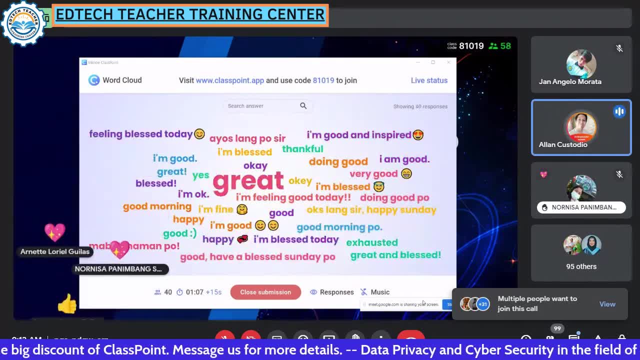 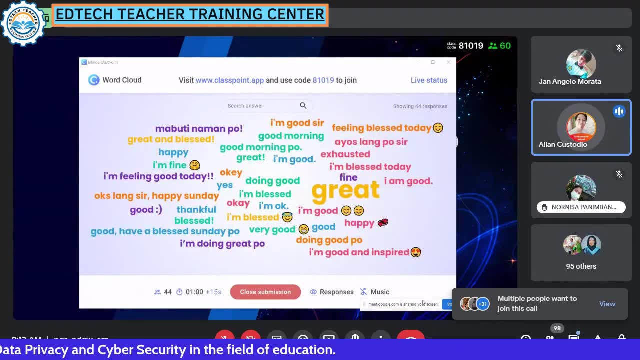 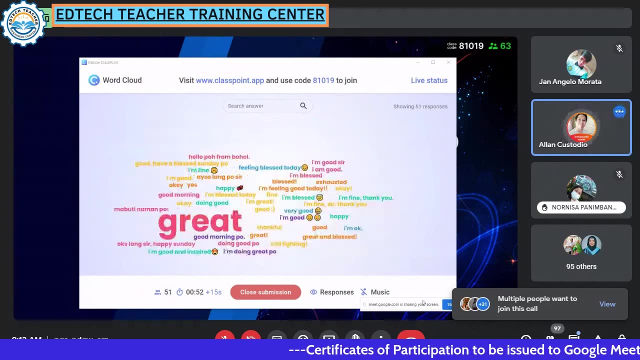 to discover new things. is that right? okay, so, for those who will enter wwwclasspointapp 81019 there: great, so our webinar is starting properly because of our way of and all of you are okay, okay. so it's really good to see that and I will close it. 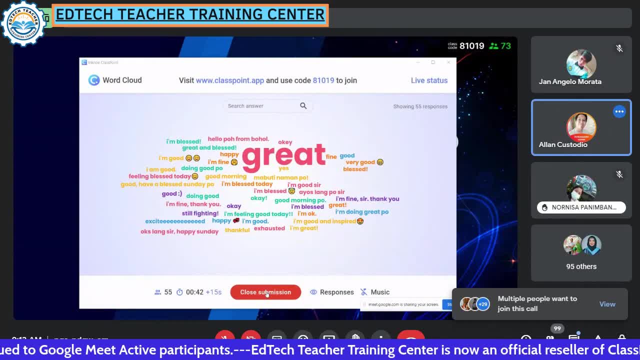 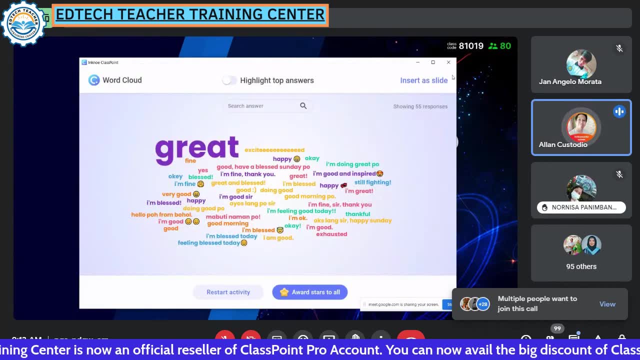 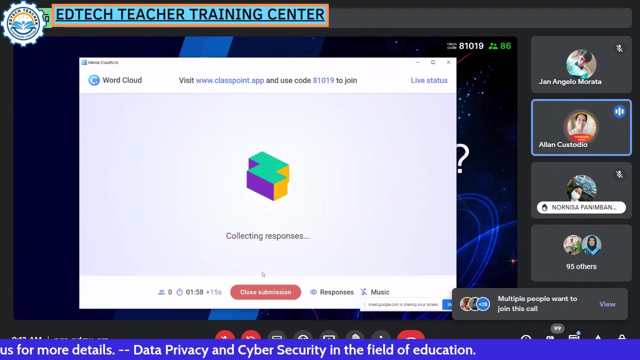 there. okay, there, and I will try to award. if it's okay, and let me cross this, there are a lot in our classpoint, I will close it. and in our continuation, what are our places for us to see? where are the people here? Iloilo, I am okay. 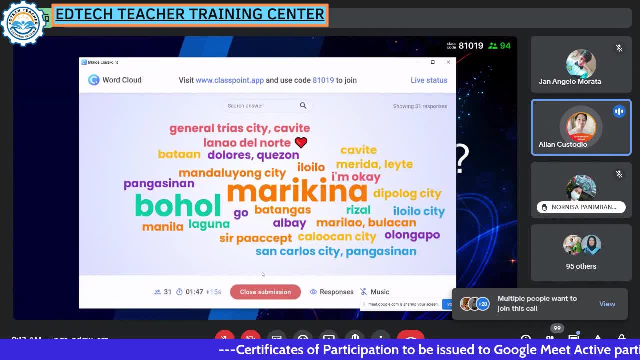 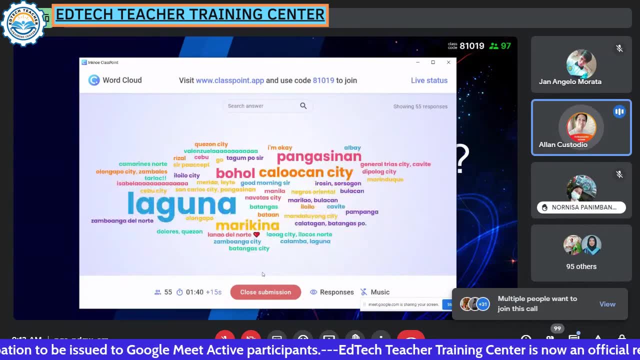 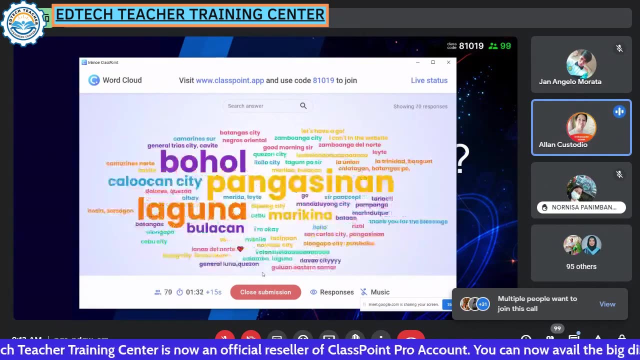 where are we from? that's the question. okay, Iloilo Marikina, I think there are a lot in NCR Kaloocan. maybe they are doing other forms while listening. it's good to listen because we will have orientation. is that right psychosocial. 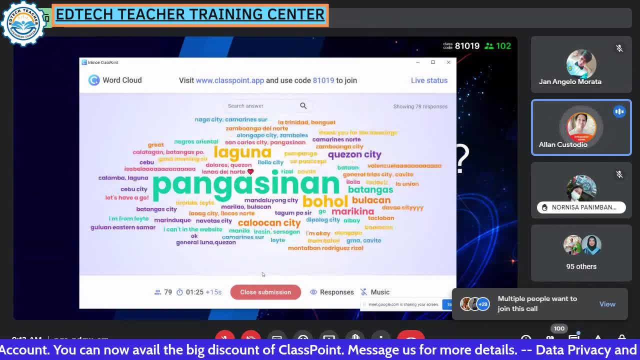 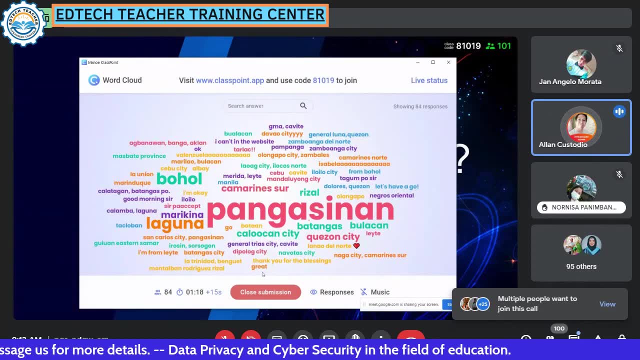 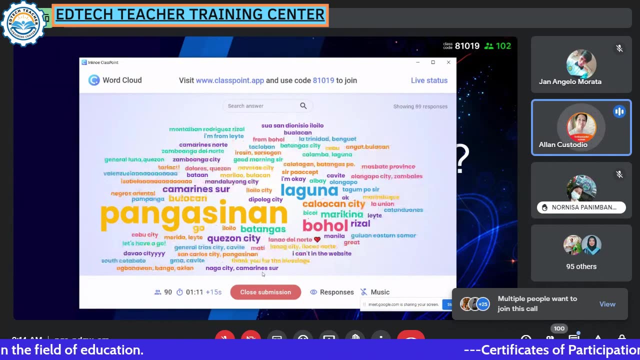 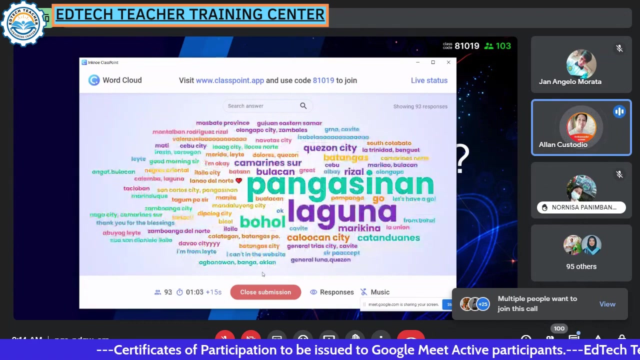 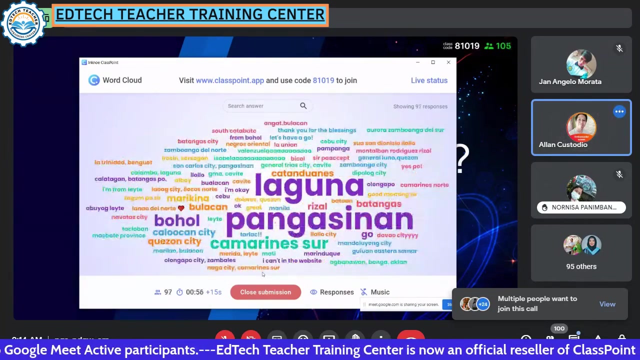 or psycho. what is it and what is it? is it is it so? because, see, this is it's good to listen, because you know I am a student, student bullock on a ya know, Napa Kodama Puno para pum pumasok double, a, double, a dot. 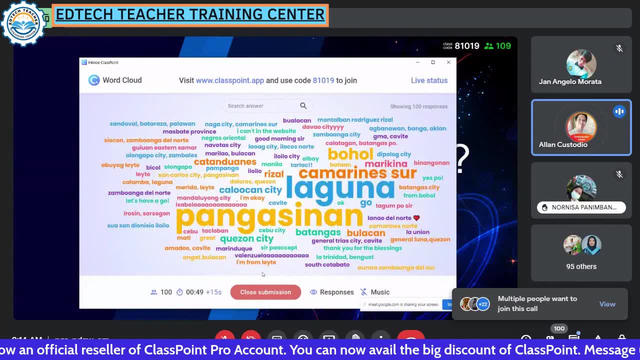 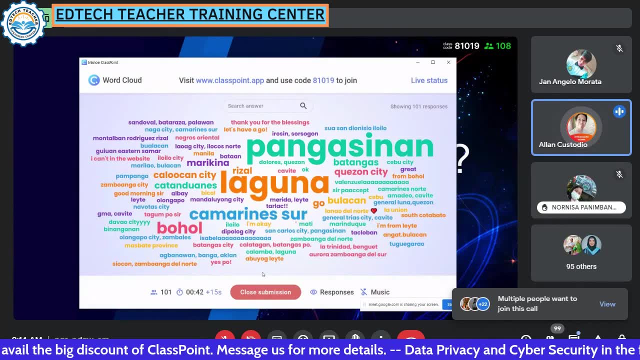 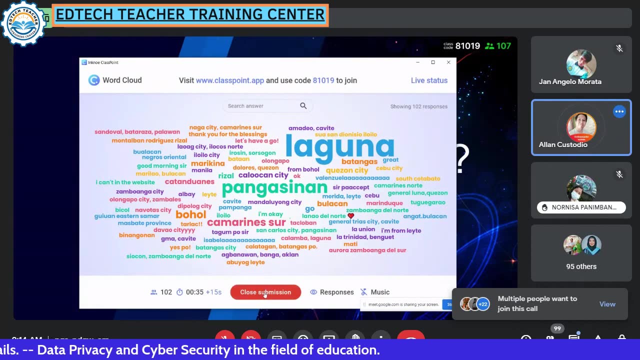 class point that up eight ten one nine I am so car on marine and surf on Garinan. so maraming salamat Puno, Samara, Samara got in laguna, napoleon domino laguna, so cross gonna pull a, I am, I am, thank you. 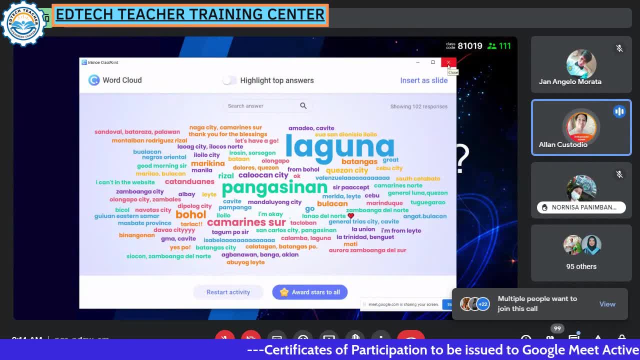 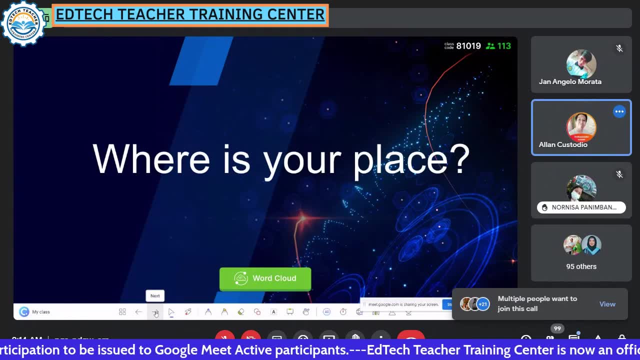 Puno Samana gc's. a got a pocket a me Pune at in a young umaga. I am so Papa Patoly, Pune at an an extra long for it. oh wait, don't go, I'm gonna come on a king, I want an internet. Oh, so totally put a us at in the slide. like you, my internet on a lamp or time on. 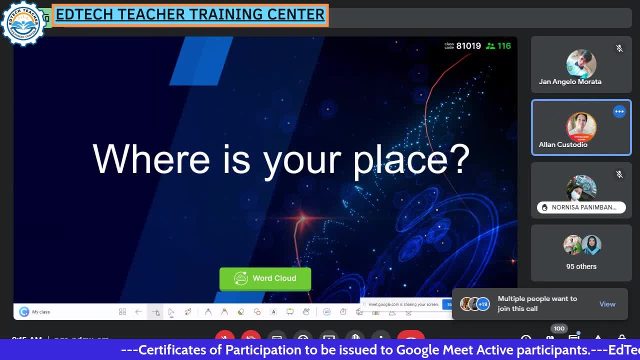 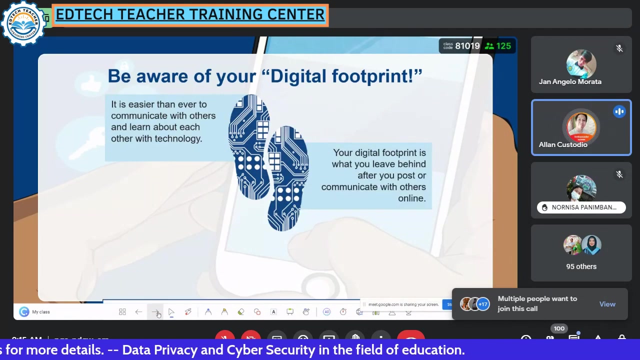 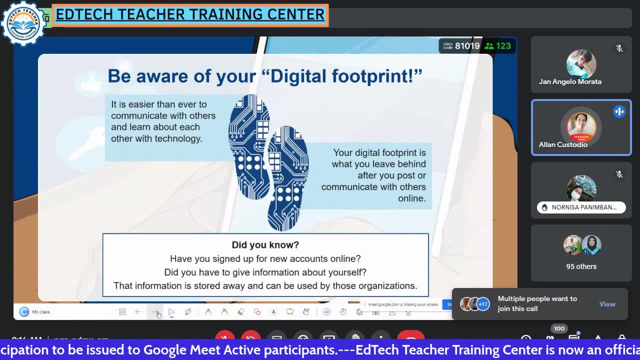 I'm donít know how are the websites that we opened yesterday or even a while ago now, if the websites that we opened are okay and the ones that are not okay, it will reflect on us especially, especially if the ones that we opened are not secured sites. 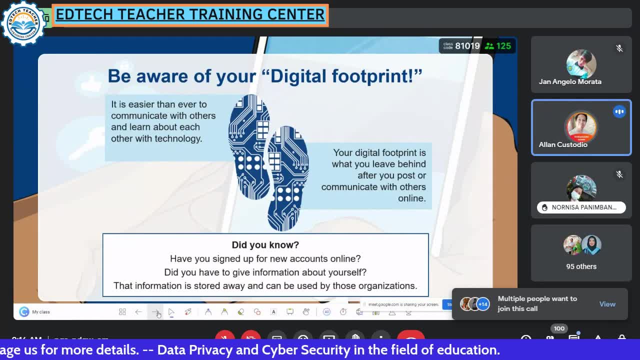 those are the ones that are not starting from wwwhttps. those are the ones that are unsecured, okay, so let's be mindful there. usually, our search browser is google, facebook, twitter, instagram. all of them are protected, but the ones that you don't know. 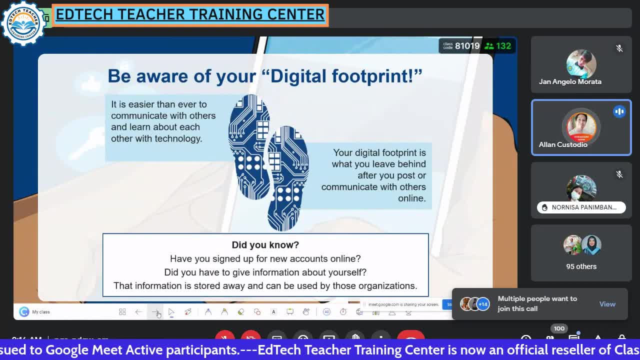 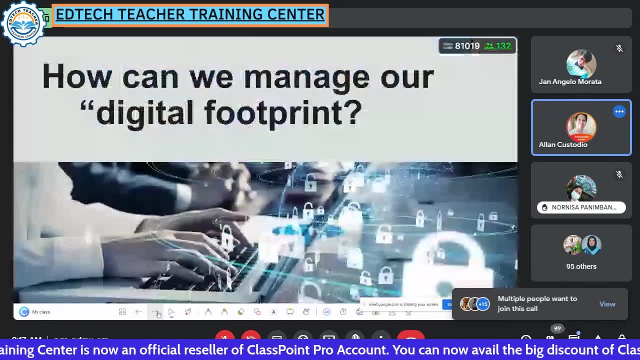 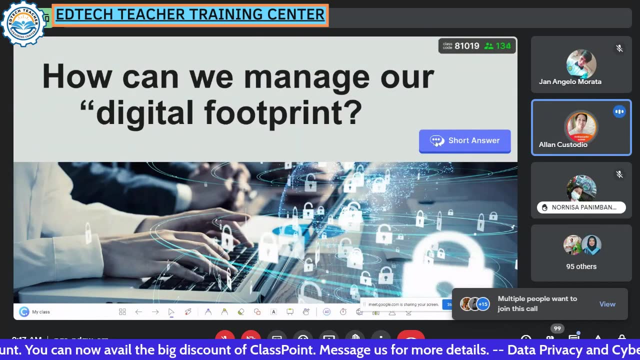 maybe you need to not click on it because you might get some information later, especially if you are using third-part parties and cookies. okay, so how do we manage our past? okay, not the past that you love, the past that happened to us online. how will it be better? 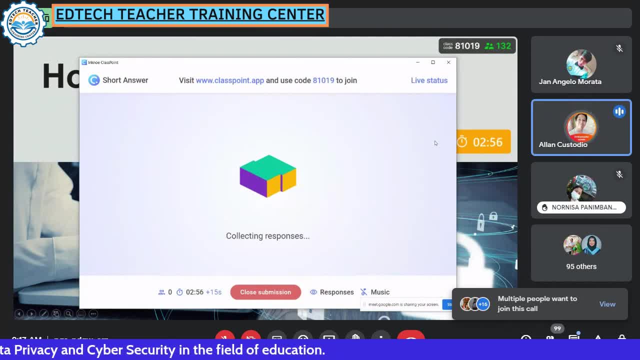 okay, how will our past be better, our past in online history? let's see what our participants will answer. the digital footprint: these are our pasts, okay, this one apply the think before you click: think before you click- okay, this is good, but I also see. 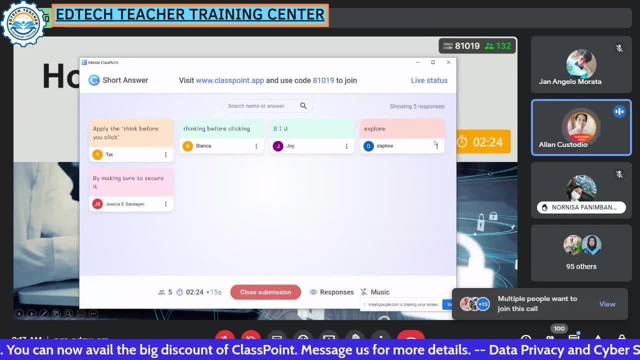 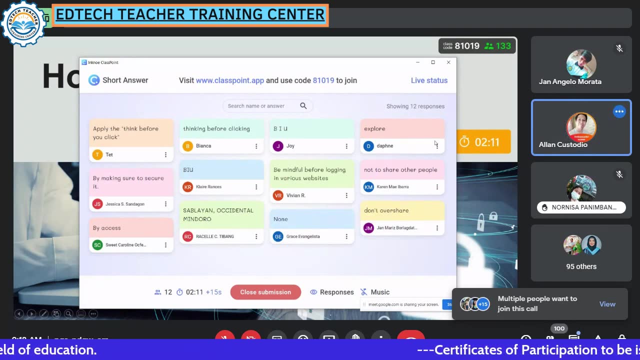 think before you click. you are thinking, but it is also good. maybe, for example, our post is good, but sometimes what happens is they don't like it. they don't like it. so if you clicked, you are also ready for what will happen to you, because sometimes 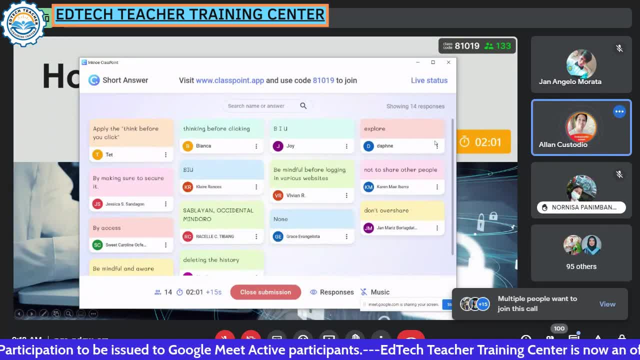 my post is good. why don't they like it? so it means it is also good to prepare our emotion aside, you know that your post is good, but are you ready that the one who will like your example is your mother, your cousin, your best friend? 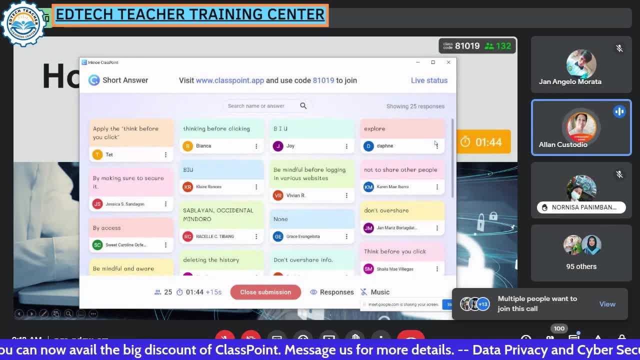 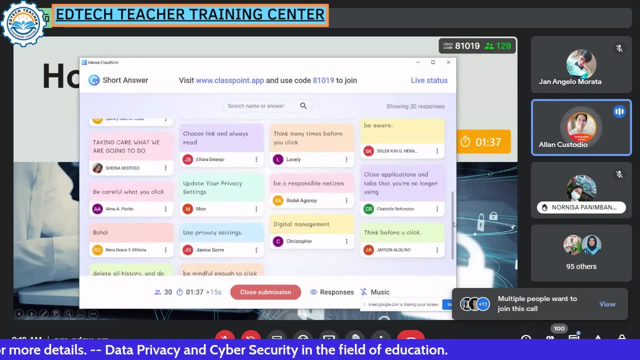 nothing right. so we will look carefully also our emotion, so that you are ready, as they say, when you post on the internet. other people are not your company. no matter how good your post is, you are still bad in their story. so we are always ready. 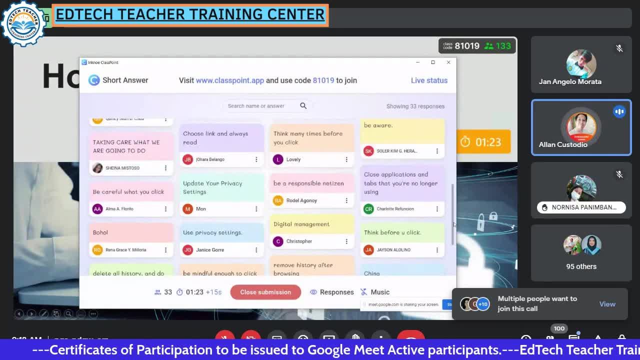 and don't pay too much attention, because your main goal is to share your good things, to share the happiness with your family or what whatever we want to share on the internet, right? so, all of you, Ma'am Alma, Ma'am Sermon, Ma'am Rodel. 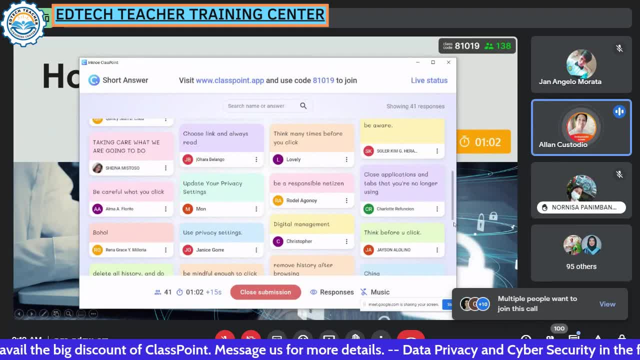 Ma'am Charlotte, Ma'am Soler, all of you are right, taking care of what we are going to do. China, yes, being accountable, because we really need to be responsible for what we are doing, because there is evidence we can see our posts right, okay, so let me cross that. 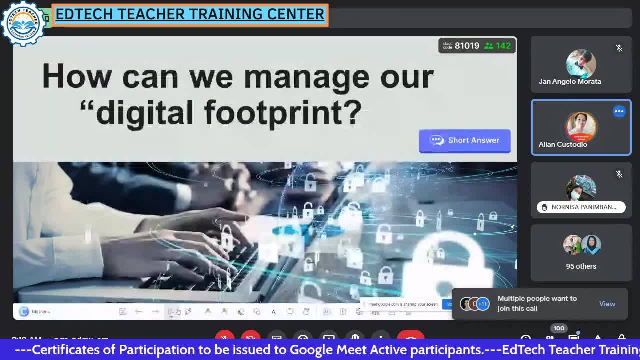 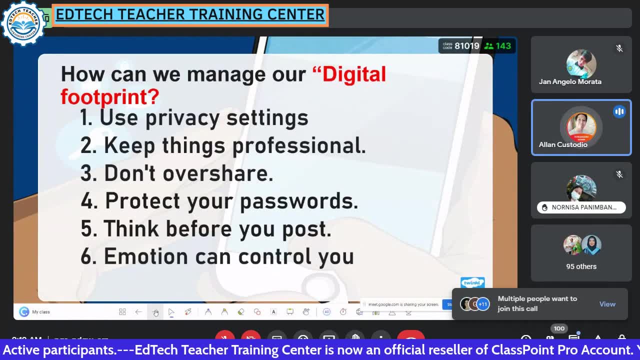 and let's exit now. now let's continue. so these are my tips almost always, and these are: number one: let's do privacy setting. okay, in privacy setting, only me the number address there and then keep things professional. basically, other people are thinking that because you are not studying, 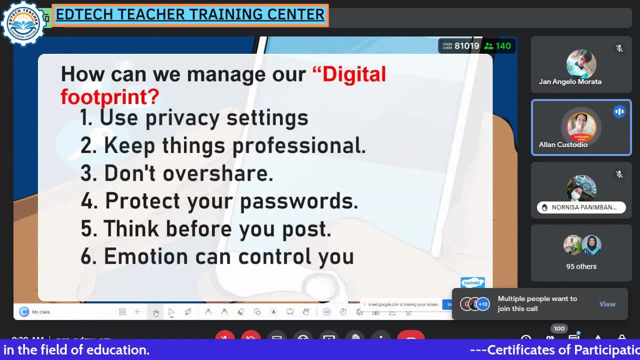 or something like that. they are just wasting their posting. what I am pinpointing here you will use in the next situation your social media. now, if you use that, and the latest in the job, they put social media Twitter account, Facebook, because it is included in the criteria. 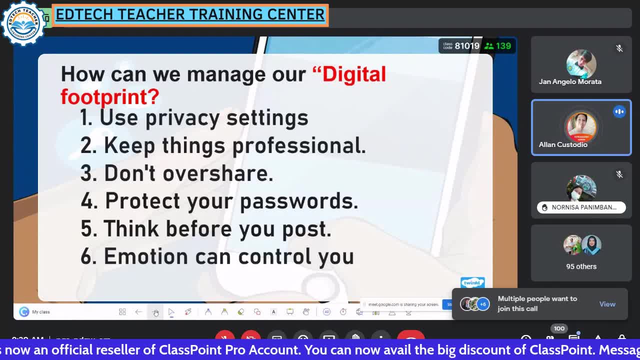 that is social media and you can use that and it is also a part of HR. okay, that will hire you that you should. your social media should be in good condition. do you believe that our social media should be in good condition? please chat to us on our 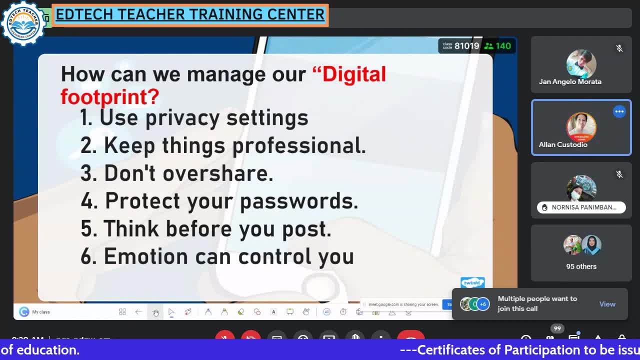 live or to our live. number two. number two to our live, if our social media should be in good condition. number two, there on the live Facebook, if it should be in good condition. ma'am marie, ma'am marinelle, sir raymond, sir, sir mark, ma'am glenda, correct, 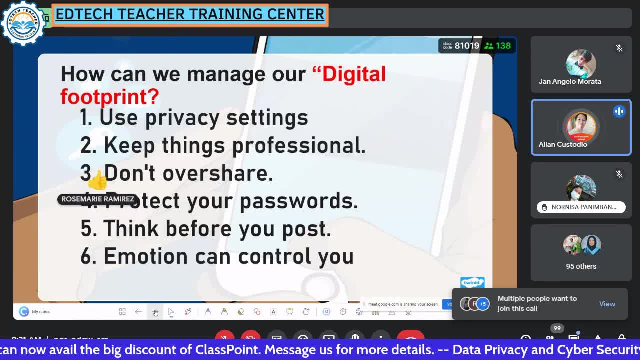 kasi pag hindi maganda yung social media natin nagre-replic sa atin number three, yung do not overshare syempre. ah, napakadami mong sineshare, nagbakasyon ka, tapos sabi mo: ay bukas bahay mo. 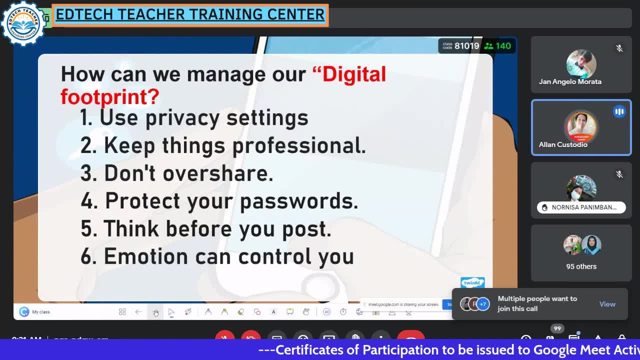 siyempre malayan ay magsanakaw, nanakawan ka na now. shout out po sa lahat ng samagot ng number two. ah, napaka active naman pala ng mga andito. okay, so wag ka mag overshare ng masyadong madami. 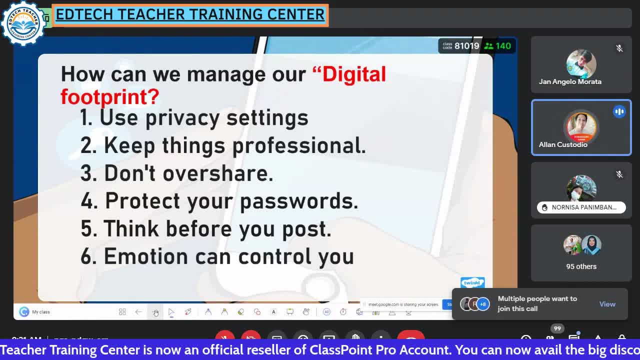 may tinatawag na rules nung naka-attend po ko sa ibang banta, pagtapos na yung isang event, saka sila nagpo-post. ayan, pagtapos na isang event, saka sila nagpo-post, kasi kapag ongoing ka nagpo-post. 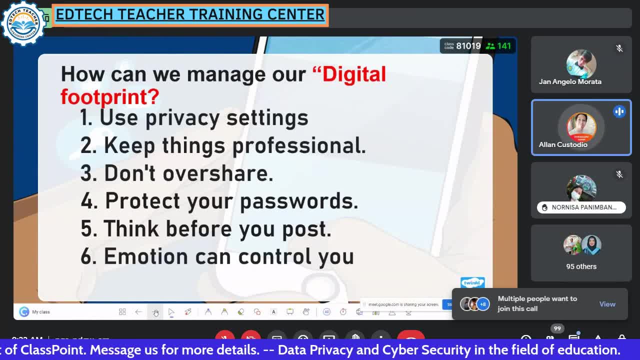 sometimes, kapag may mga kawatan, lalo na may daladala kayong pera or something, ay pwede kayong targetin, pero kapag nakalipas na yun o kahit puntahan kanya, hindi kanya madi-detect, kasi wala ka na dun, tapos na. eh may tinatawag silang. 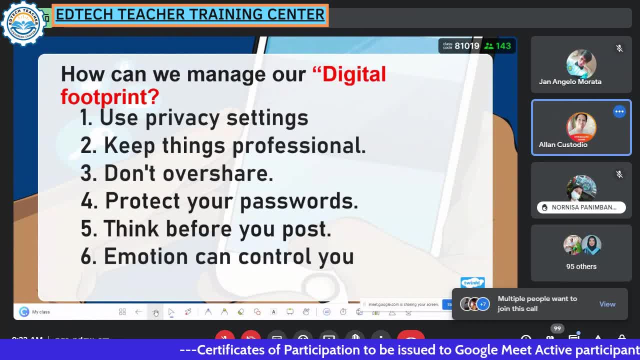 rule na ganun: pagkatapos ng isang event saka nagpo-post, pero nasa discretion mo yun, kung gusto mo lang, happy ka lang at the moment, pero yun nga accountable tayo at responsible sa pagpo-post na yun. kasi talagang lahat ng consequence makukuha natin kung sakaling. 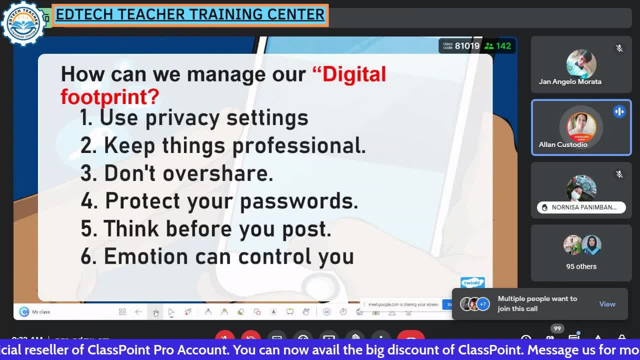 talagang. ah, yun ay paninindigan natin, mabuti man o masama, kaya lagi natin tatandaan na para sakin magandang gawin yung technique na pagtapos yung event. pero nasa inyo din po next natin is think: 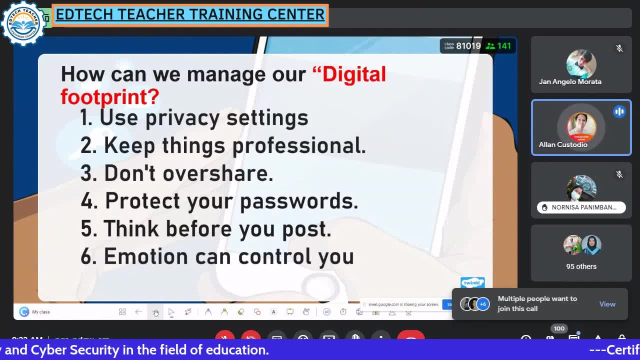 before you pause: talamak na talaga ito, kasi kailangan mong mag-iisip. pag hindi ka nag-iisip, nagpo-post ay mapapahamak ka. mapapahamak ka talaga, kasi ang rules natin sa social media ay hindi siya. 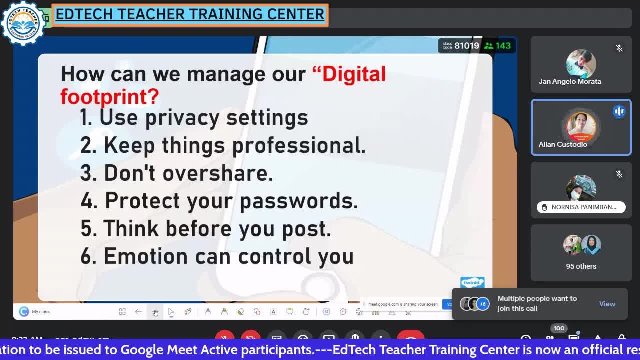 nang wala hanggan. hindi dini delete ng may ari unless nireport ka. pag nireport ka pangit ka si post mo may pwedeng i-delete ni post bok ma warning ka niya. you have been banned for 24 hours for. 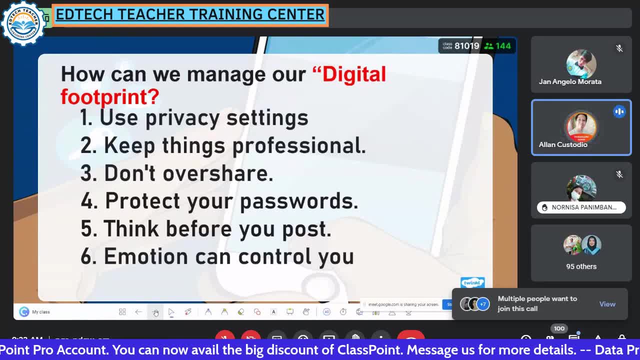 posting irrelevant or harassing issue. papadala ka lang message sa facebook number six. emotion can control you pag galit ka sobrang. uh, uh, celos, or watch something. wag ka muna mag-socialize. yah, it was the first time kasi na sinubukan ka lahat ng mga quote. huwag ka muna mag socialize. 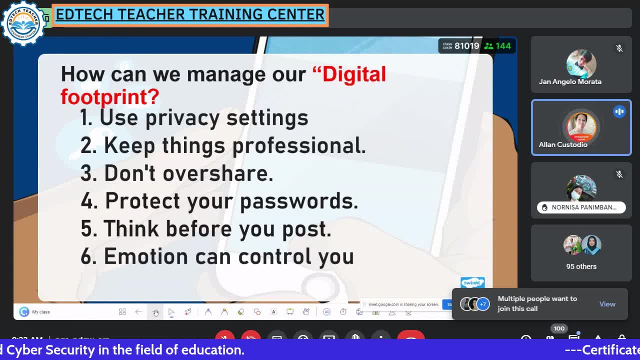 ang socializing sa facebook number six. emotion can control you. pag galis ka sobrang ah, ah celos, or to say something or what something, wag ka muna mag social media makakokontrol ka, pero sino ba dapat kumontrol sa emosyon. 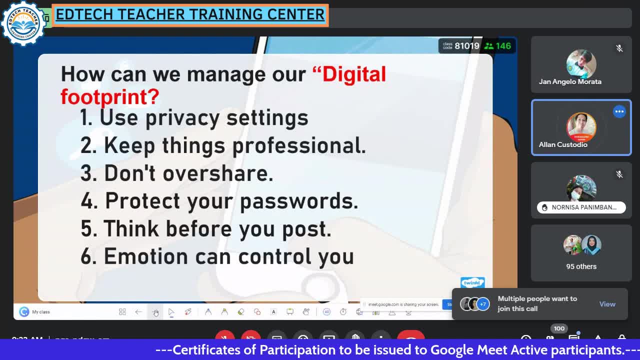 diba, tayo po yon, part mo kasi yon. so ibig sabihin, ang emosyon, ang their happiness, lahat ay ikaw ang kukontrol, sa huli, ikaw pa rin ang magpopost kung anong gusto mo. 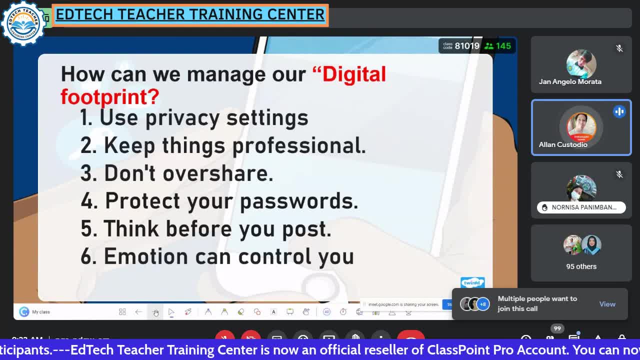 sana ipiliin mo yung mabuting ipost kesa sa masama, kasi kahit na hindi ka masyadong napapansin sa mabuti, ang balik na lang nun sa iyo ay neutral ibig sabihin. 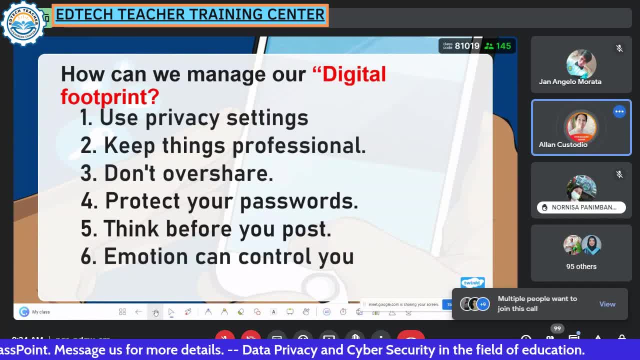 wala kang inapakang tao, pero kasi kapag nag negative ka may pinatamaan ka nag matretest ka ay tignan mo yan ha pagkataas ng 2 days marami dun magkocomment. 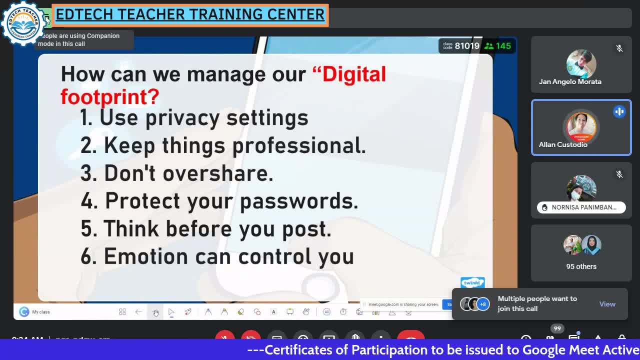 sino ba yan, sino ba yan? tapos yung iba, marami na dun nagpipid, nagpipid, or reveal na yan, at reveal na yan, at tatadta rin na natin ng comment. you see that, nakita nyo, nakita nyo, kung. 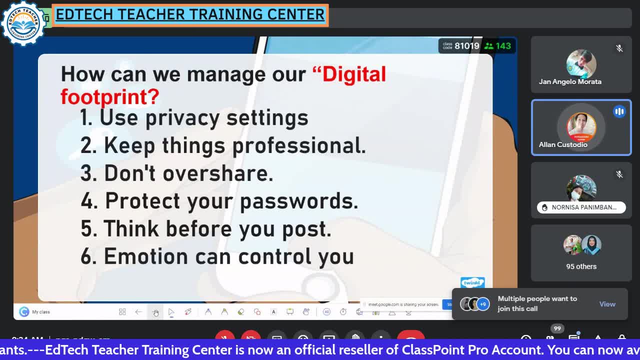 gano katin, hindi, kapag nag negative ka maraming makikisampat siya, pero merong minsan sasausaw na wala naman talaga sa issue at dudugtungan gagatungan ka. so titignan yung. 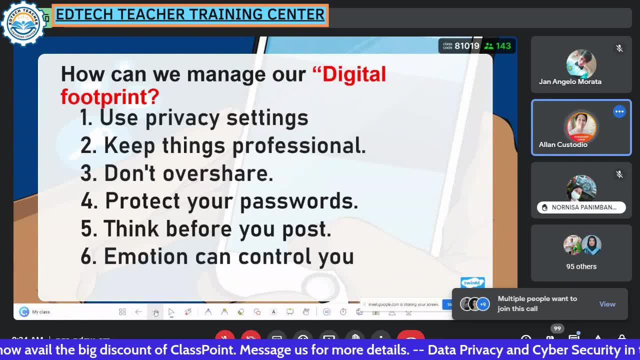 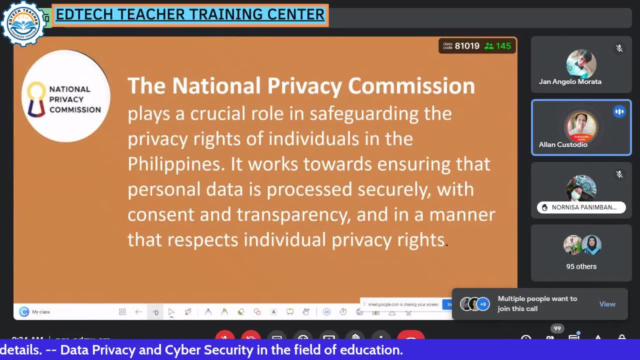 mabuti mga mam. yun ha, sir ha, yung mga ganong gatong gatong hindi dapat tayo nagaganon, especially government employee, kasi tayo may pinakamataas na tolerance sa sinumpaan natin sa ethical code. 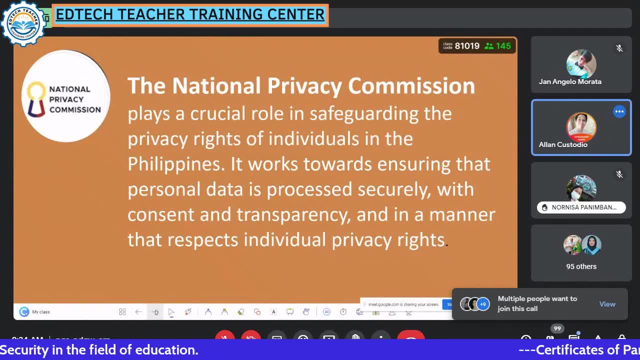 tama po ba. okay. so meron po tayong mga pangalan nito pinapalo ng mga pangalan page. example, edtech training center, na nagbibigay ng mga free webinar at napakadami talagang free at nagagamit natin. 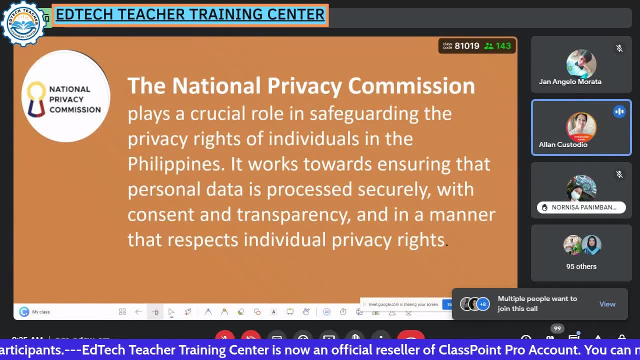 kita nyo po napakadaming natutulungan at nagagamit talaga sa ating professional development, pati sa ranking ngayon. pwede rin nyo rin po ipallow yung DICT, National Privacy Commission, na nagbibigay? 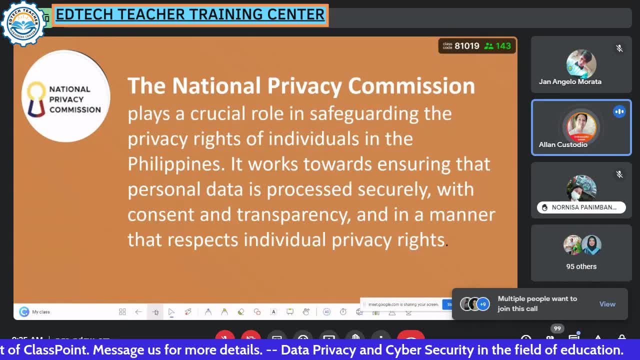 ayon siya ng gobyerno nagbibigay ng kalaman batas, nagpapakulong sa mga kriminal. ka basta po nasasakupan ng jurisdiction. when we say jurisdiction, eto yung nasasakupan na kung ano. 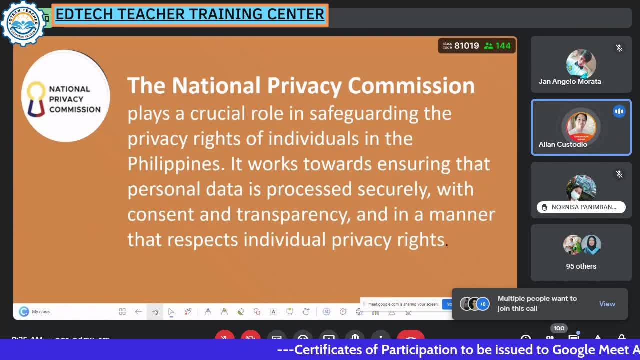 ang saklaw, ang saklaw po ng mga agency na national ay buong Pilipinas. ang ibig sabihin po ng national: buong Pilipinas, at walang sinisino ka, basta't nasa jurisdiction ka, kahit foreigner ka. 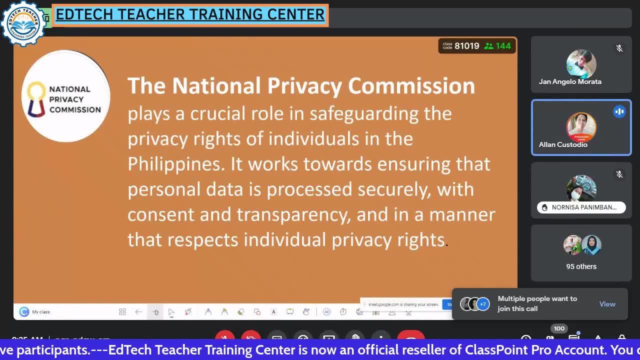 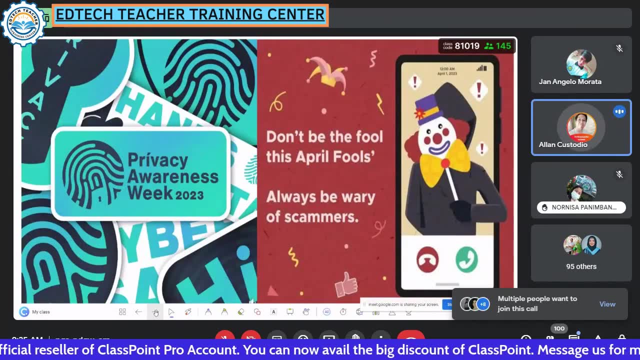 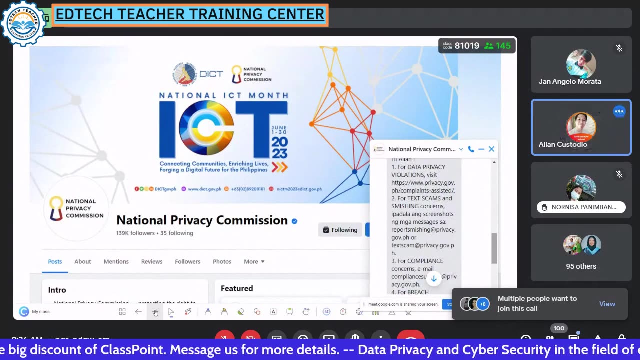 basta't lumabag ka at nasa jurisdiction ka ng Pilipinas, ay makakasuhan ka. okay. so sa pagpapatuloy natin, may mga privacy awareness week yan pwede niyong ipalaw. eto etong official page. 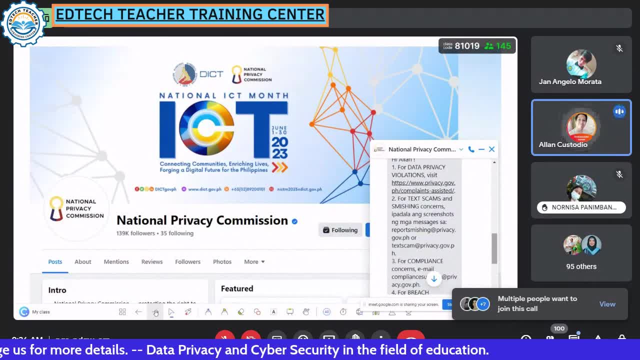 na to 139 k-follower. yan pwede niyong ipalaw din yan, kasabay po ang ating edtech trainer center na kunsaan may mga ganito. tayong in partnership and pag nag gusto niyo magreklamo. 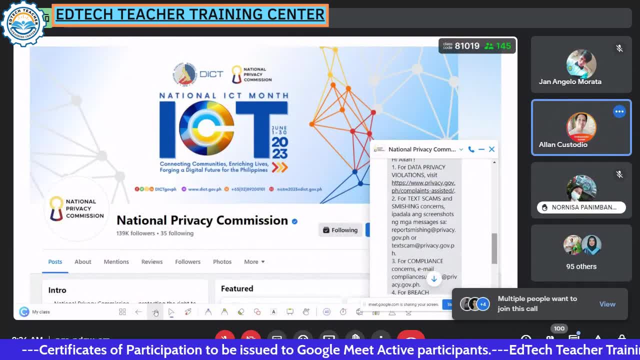 i-message niyo lang, yan may lalabas diyan. nakikita niyo po na form. kung may phishing, i-screenshot niyo muna, find the evidence and then isend niyo diyan para sila ang mag-imbestiga. 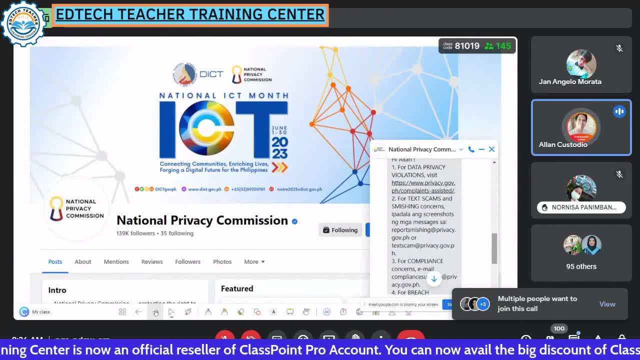 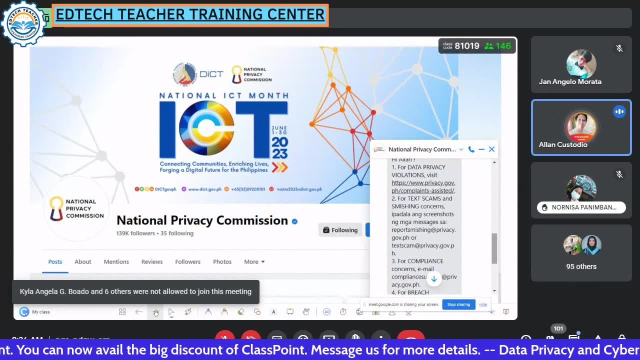 okay, ngayon tandaan niyo po ito. kapag nag-agree po tayo sa lahat ng social media, may pinipil-upan ka doon. eh, agree, di ba po ngayon nakalagay doon sa standard ng community. 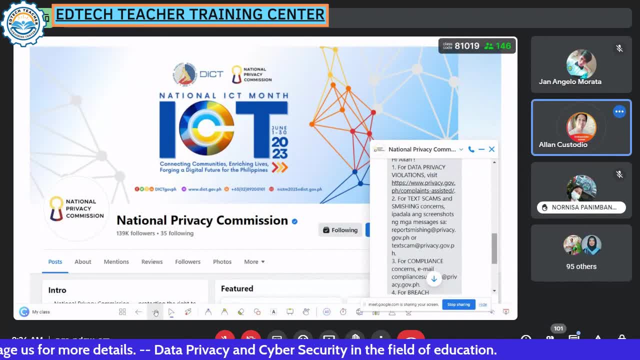 na we can report and we can help the community to continue the harmony and humanity. parang ganon po yun. eh so may karapatan ka mag-report hindi ka tinanggalan na karapatan na isumbong at i-report kaya nga po. 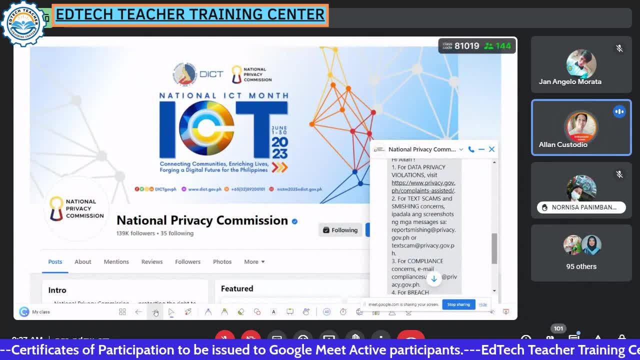 may nababan ng mga page. eh kasi ni-report, kasi hindi appropriate na makita. okay, kung sang ayon po kayo sa pinagsasabi ko, number 4 nga po sa chat sa live at saka sa ano, number 4 nga po. 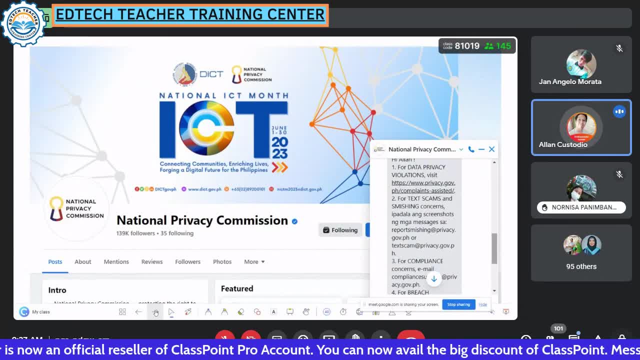 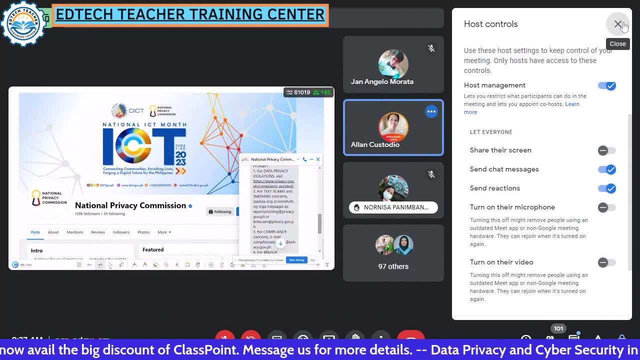 sa live, ay sa live. sige, nga po number 4, nga po tayo chat, nga po tayo number 4. ayan, o ma'am Ruth, shout out sa'yo, ma'am, ah. ayan, o meron tayo sa mga google meet natin din. 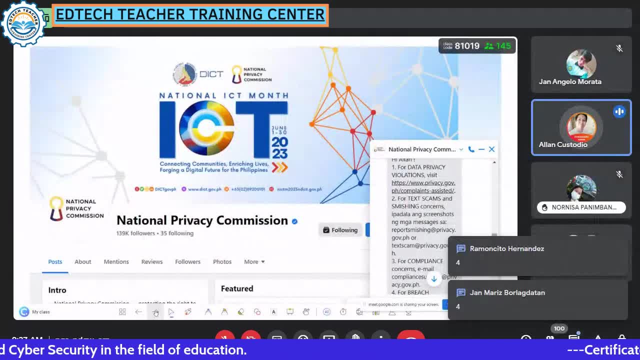 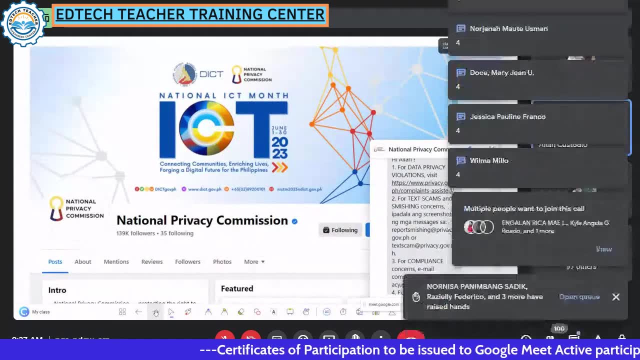 ang mga sagot. so Florey, ma'am, Anne, Sir Jan, so lahat din na nasa google meet ay nagpopor. so ibig sabihin talaga nakikinig sila at mamaya sasabihin ko yung mga batas. 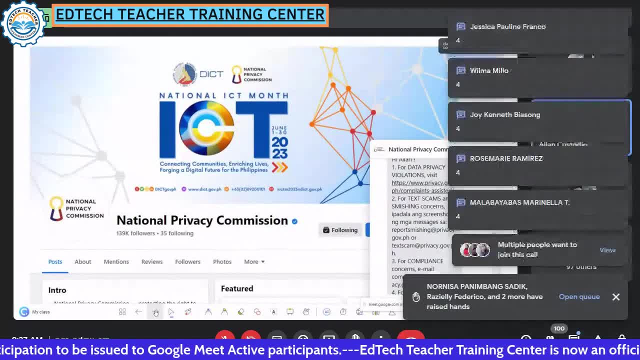 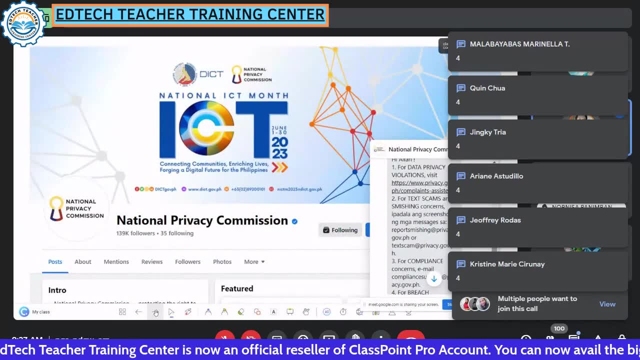 na nakapalaw sa jurisdiction naman ng school in terms of cyber bullying, pero nakapalaw pa rin po yun sa cyber crime act, which is 101 act of 2012 ng NPJ. so maraming jurisdiction, pero titignan natin. 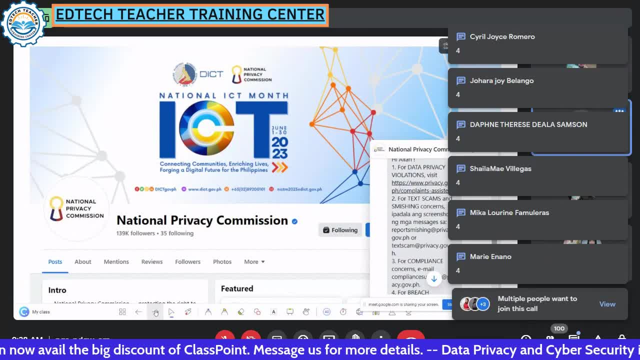 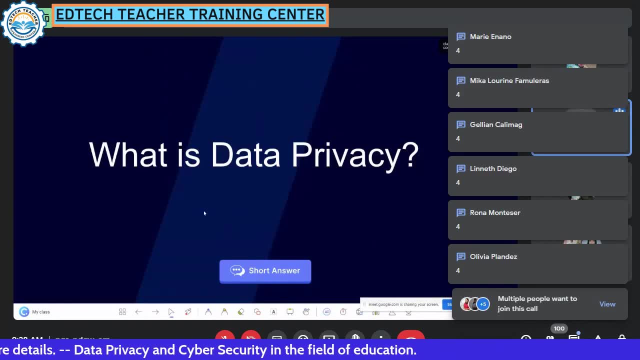 yung mga ipapataw sa mga under 18 years old and then above 18 years old dahil na ddsw diyo under 18. tama po ba ngayon? ano ba yung data privacy? magpaka lalalim na tayo. 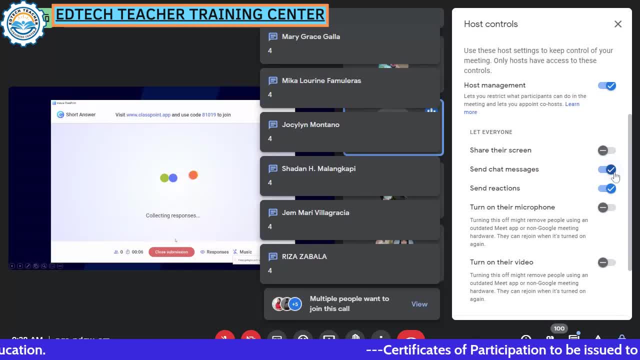 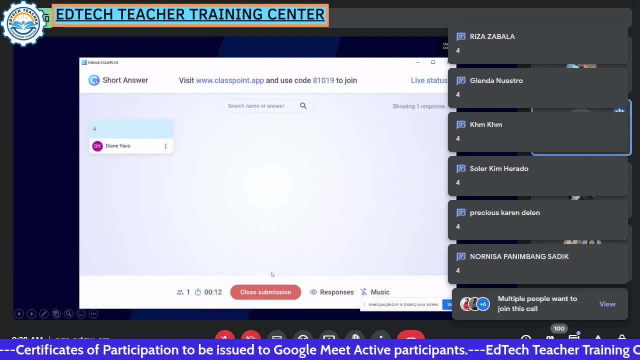 ngayon. pero eto ang simula. okay, magdadive in na po tayo sa ating mismong definition at gusto po namin na makita ang inyong response. ano ba ang data privacy? okay, dito po nag nag force ni ma'am. 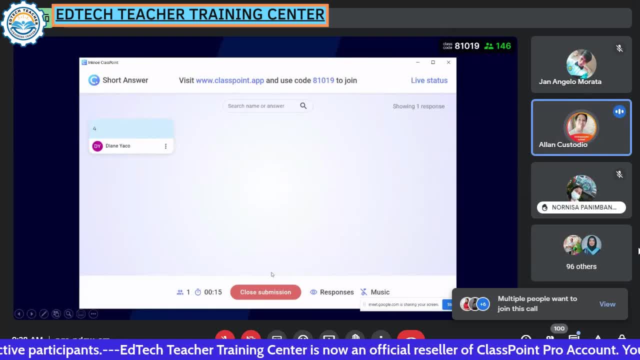 Diane, ano na po ito, tanong na po ito: what is our data privacy? and the question is tama. hindi po nakakapasok no, sa ating meet or dito. pwede po tayo sa class point, wwwclasspointapp 81019. 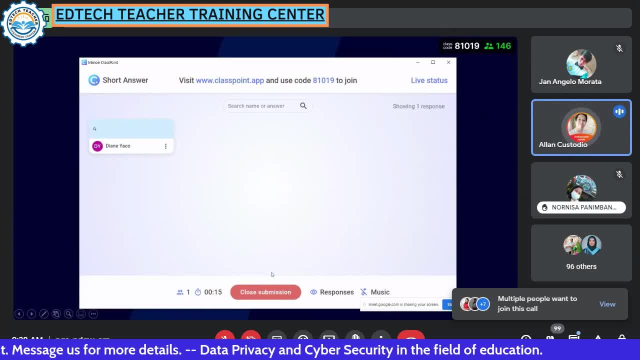 yung code tama, hindi po nakaka-experience ng class point. experience nyo po kasi pwede ito sa classroom nyo. okay, karapatan na itagwang personal na information o tagalog. si mo, ma'am, nalalapit na din. 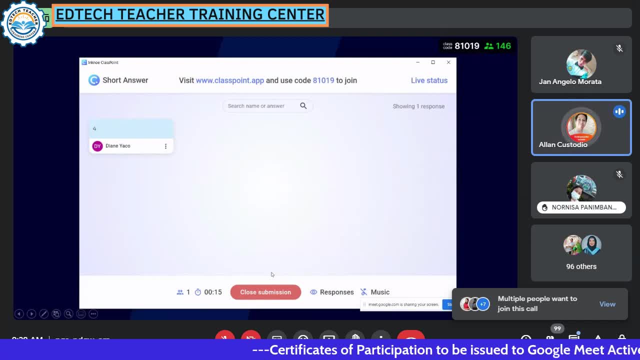 kasi yung tinatawag nating buwan ng wika eh diba buwan ng wika. lahat tayo may karapatan. correct po the right: securing the data. knowing the importance of data security, correct number four. may natututunan po sila. 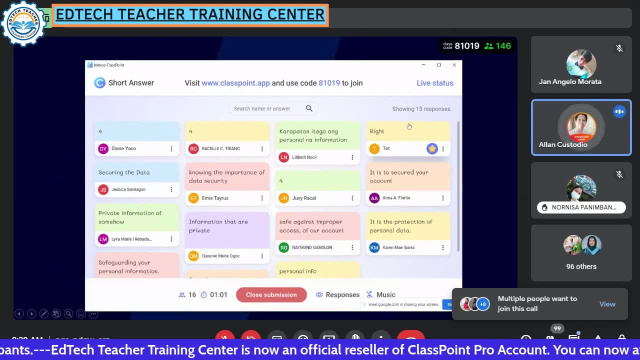 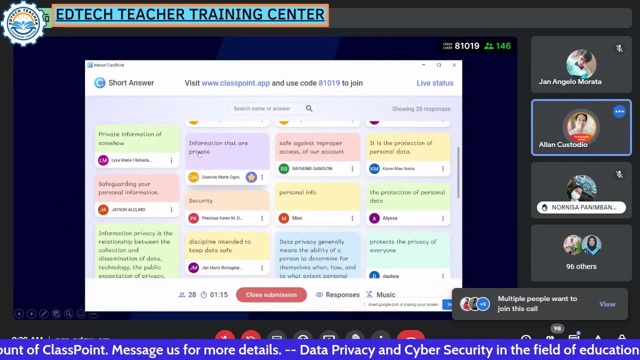 ma'am UB. ma'am Diane, it is to secure your account. ma'am Alma, it is to protection your personal data. ma'am Karen. sir Raymond, safe against improper access, correct, siya, sir? sir Raymond, ma'am Queenie: information that are private, correct? ma'am Queenie. ma'am Laika. 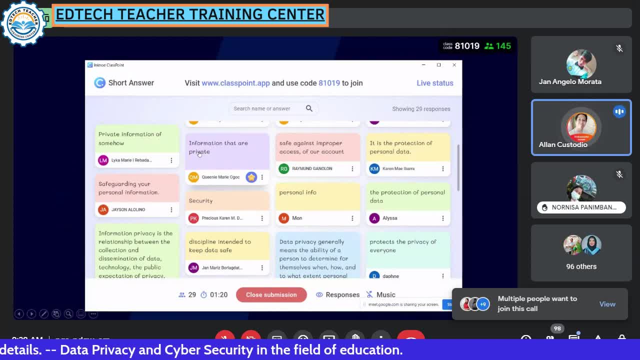 private information somehow, and marami pa pong ibang sumasagot sa baba. no, basa pa po tayo, sir Jason. ah, ma'am da, ma'am da, da po ba yung pagkakasabi dito. da pin, sir Jeline. 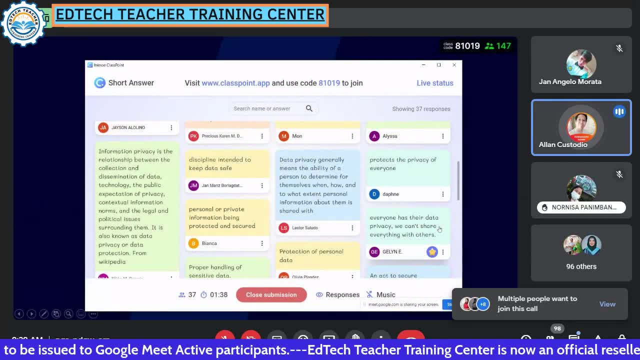 ma'am Jeline, ma'am Leonor, sir ma'am Bianca, sir Jan Maris or Jan Maris, parang lalaki baba discipline to intended keep data. may mga baba pong sagot dito. ayan no sina shout out po na po kayo. 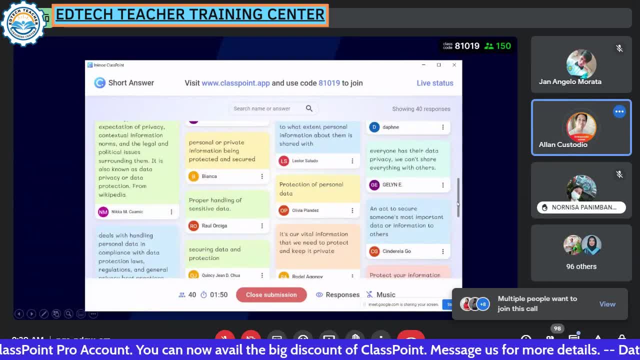 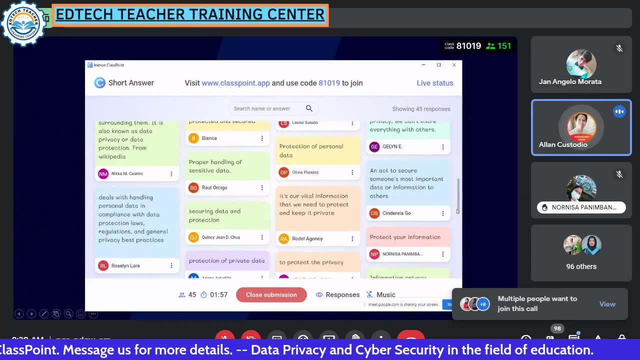 na nakikita naman sa screen po yung sagot nyo. eh, ma'am Nika, sir Raul, sir Rodel, sir Olivia, sir Queen, ma'am Quincy, ma'am Roslyn, ma'am Nornisa, sa mga gusto pong sumali sa class point. 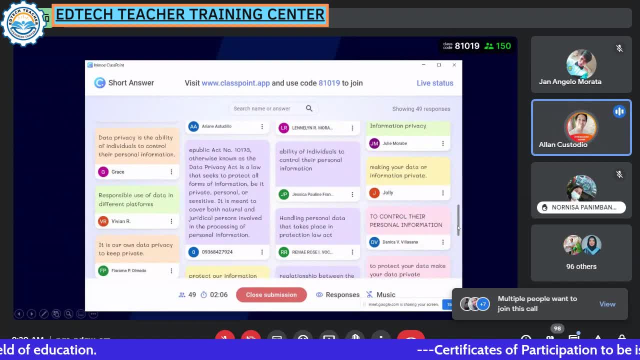 makikita pangalan nyo sa screen. live po ito. no, as of now, wwwclasspoint. punta sa google code 81019. sabihin ang inyong name. okay, malapit na po tayong mapunong sa class point. 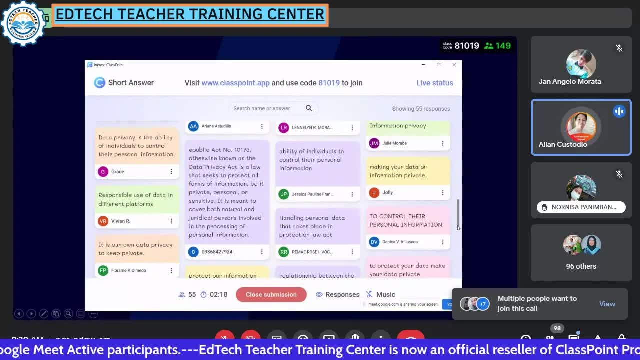 we have 50 slot na lang din po okay making your data information, sir Jeline. so lahat po yan tama act of one 173, otherwise the republic data privacy act. tama po yung sinasabi ni 0936 number ba po talaga no. 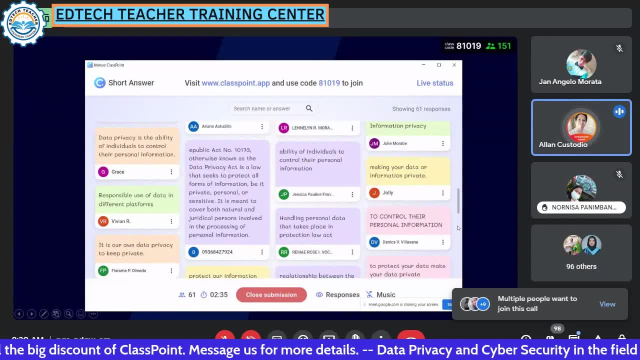 and dagdagan ko lang po no DPA 2012 and na-enact po ito nung 2000 mamaya. makikita natin at effective to September 2012, 2016, yung data privacy, natin, yung mga batas. 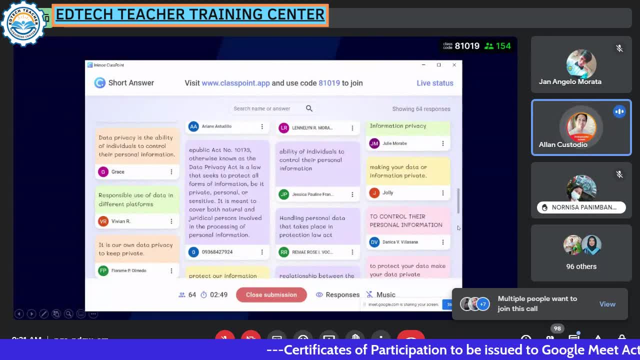 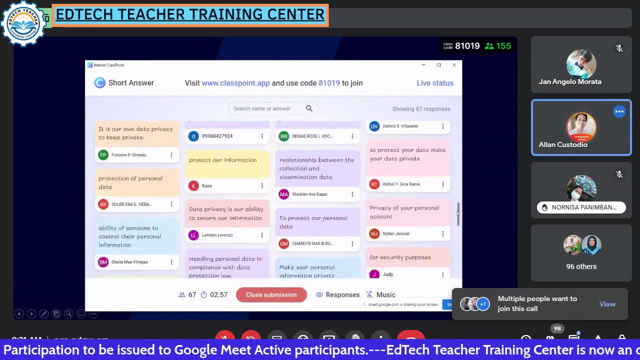 okay, so responsible to use of data and the different platform, mambibian and lahat po yan tama, sige po, magpakalalim po ako para makita lang din makita sa buong live ang inyong mga sagot. syempre effort yan, eh. 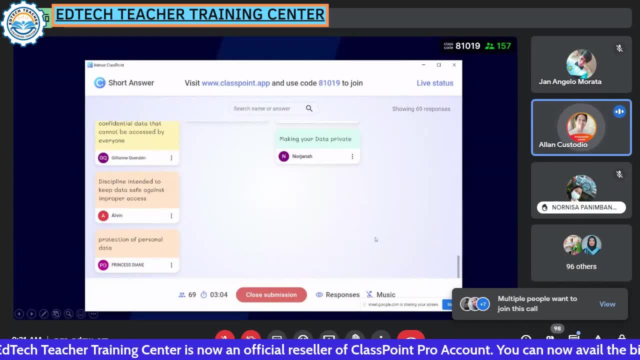 okay, ayan, no, hindi ko man po matabi, natadulo na po lahat okay, maraming, maraming salamat po, sir Alvin, from Princess Nordiana. thank you, thank you, okay. so sa pagpapatuloy natin, alam ko talagang. 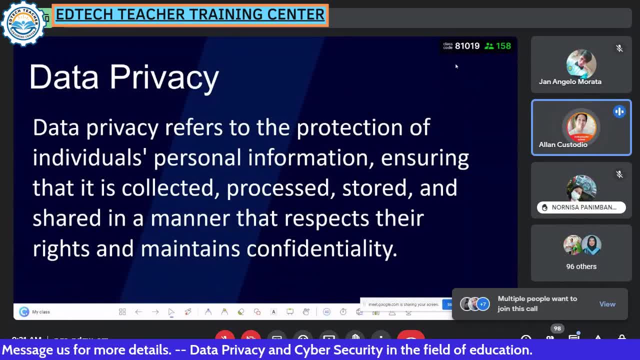 kayo ay na-excite, no, na-excite din ako sa mga sinishare natin. so yung data privacy, tama po yung mga sinabi nyo- protection ng individual personal information- and collected po ito ng, na-process, na-stored at mga manner. 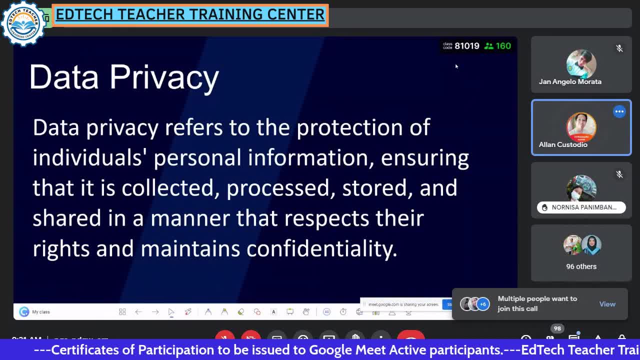 that respect their rights and maintain confidentiality. kapag walang confidentiality, ang lahat ng tao ay magkakaroon ng disrespected. ibig sabihin ay wala ng privacy. ibig sabihin hindi na magkakaroon kahit sino. 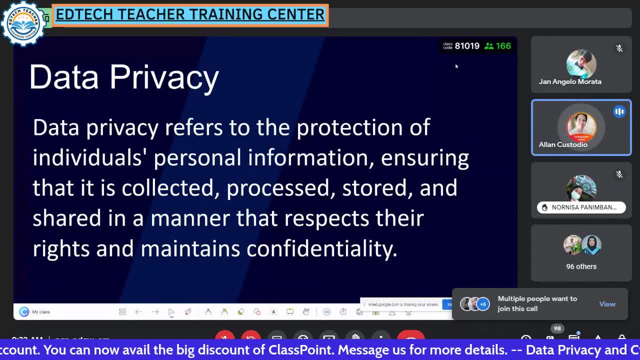 pwedeng matulog sa bahay mo, pero mamaya kong magpapakalalim muna in terms of normal literal na mga privacy. pero dito kasi data yung sinasabi natin: tama po ba at bakit ba? 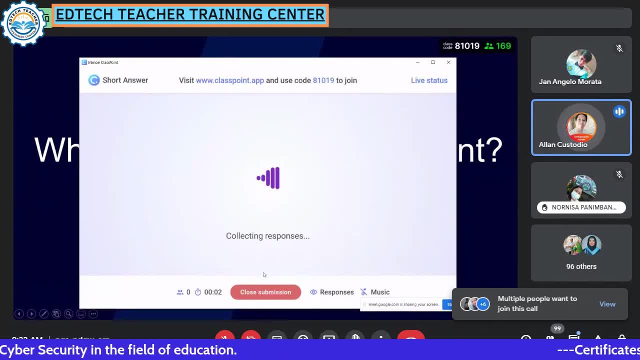 importante yun yung magkaroon ka ng confidentiality o privacy sa data mo. sige, tingnan natin ang mga isasagot. okay, search class point google at code 81019. okay, to secure the information. mam analisa, mam queen, queenie, mam rochelle. 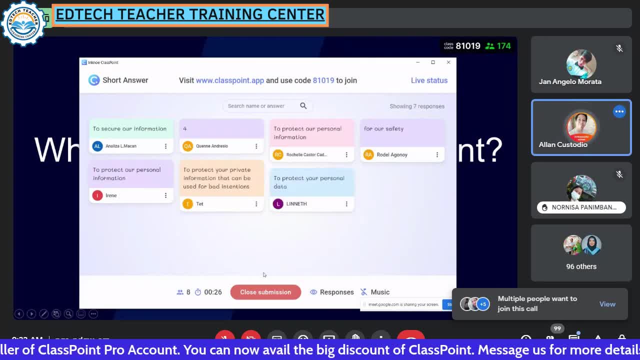 to protect personal information for our safety. correct ibig sabihin po, habang sumasagot kayo dyan, explain ko lang lang ng konti din: mamaya, i jajat down natin yung mga sagot nyo. no, paano natin yan. 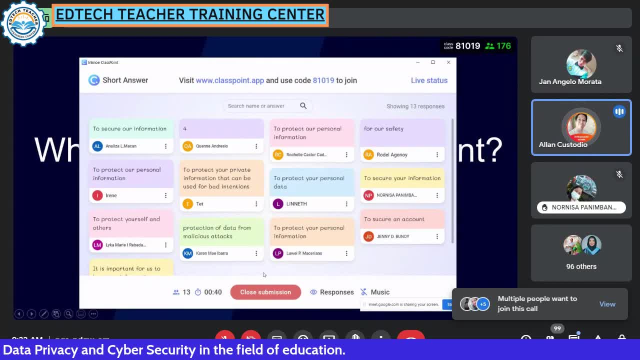 hanggang baba. so kapag walang privacy ang isang bansa, isipin nyo po ito. ah, so ibig sabihin, lahat ng tao alam yung number mo, lahat ng tao alam yung password mo. 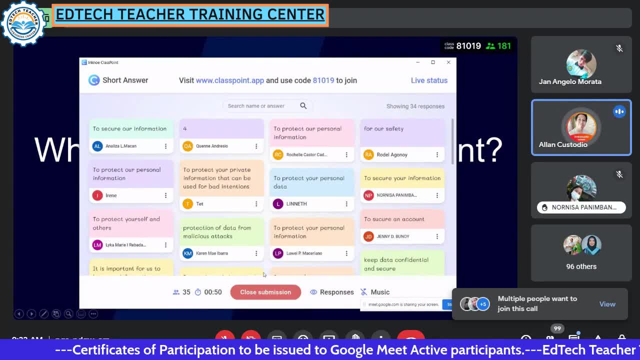 lahat ng tao alam, pa pwede niyang malaman lahat ng tinatago mo, video mo, picture mo, kasi walang privacy, walang batas, so ibig sabihin yung limitation ay: ay, ay halos wala, at yung respeto. 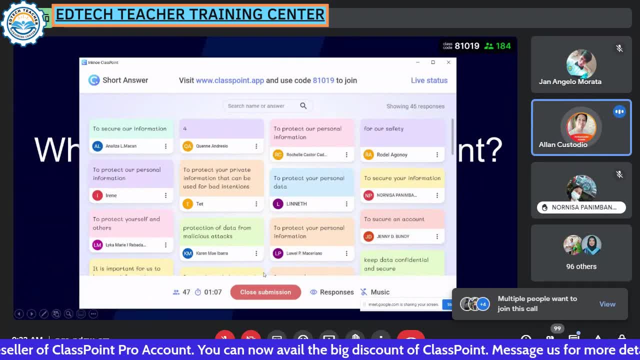 sa bawat isa ay nawawala. so the balance of the nation and the count in terms, lahat mga bagay ay mawawala, kasi magkakaroon ng kuhanan ng mga data, kuhanan ng mga account, ibig sabihin ba. 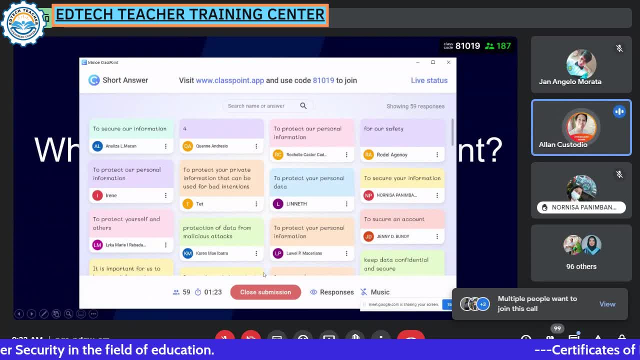 yung ATM mo. alam ko yung password ng ATM mo. pwede ko rin i-withdraw yan. pwede ko yung gamitin. so walang confidentiality, walang balance, walang harmony, walang magpo-protect, because walang batas, isipin nyo. 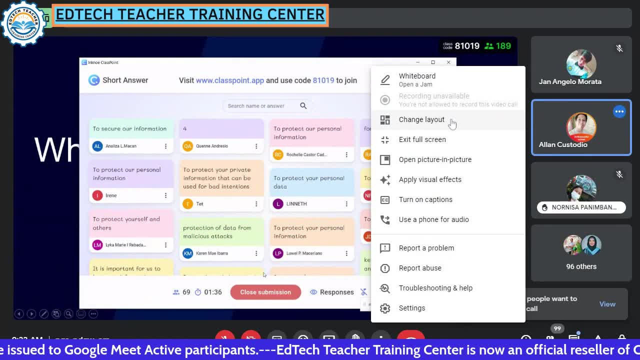 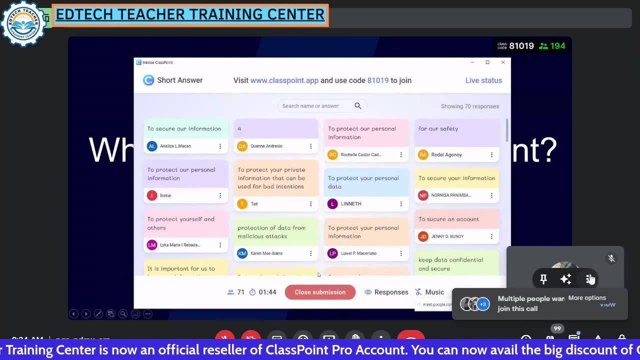 kung gaano kahirap ang magiging bansa kung walang privacy. sa data pa lang yun. pero kung ilalagay natin sa karapatan na kung mga sa ari-ari yan at ilalagay mo pa, 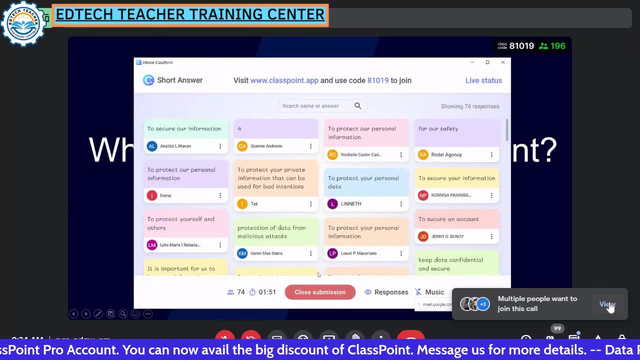 kasi privacy din at confidentiality, yung mga titolo, pati perma mo pwedeng gamitin ng iba. ano na ang mangyayari sa mundo? ganon kahalaga ang pagkakaroon ng privacy sa malalim. 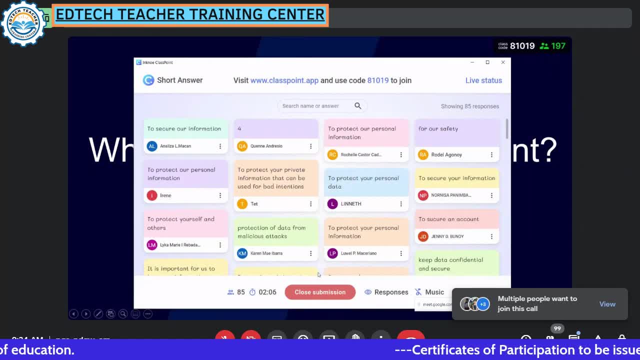 na paliwanag. okay, ganon siya katindi at magkakagulo ang buong bansa. imaginein mo, pwede kang pumasok sa system ng google kasi alam mo may password, tapos ikaw na magpatakbo. 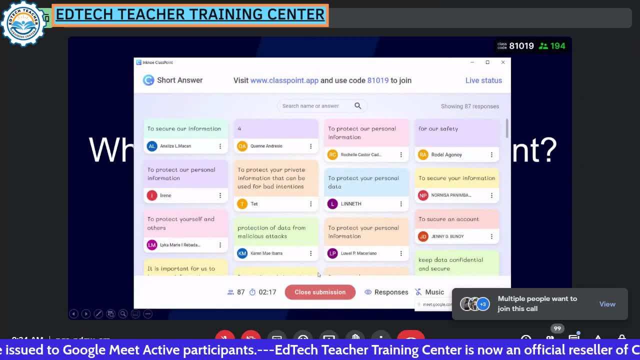 ng kompanya bukas, ibang sa'o naman dahil alam mo yung password. imagine, in that diba maraming mga naghirap, maraming mga gumawa ng mga bagay-bagay, pero sa mga pagkakataong 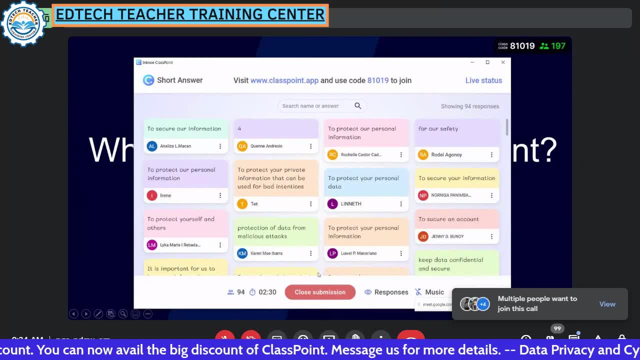 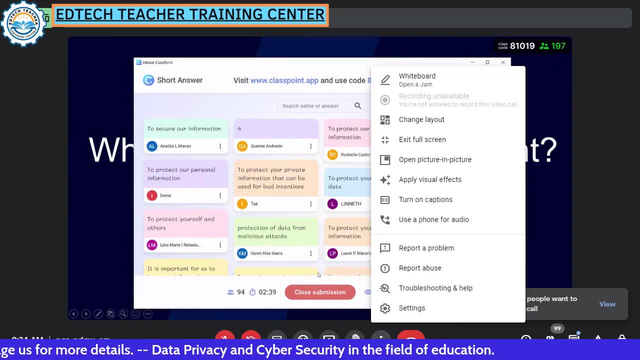 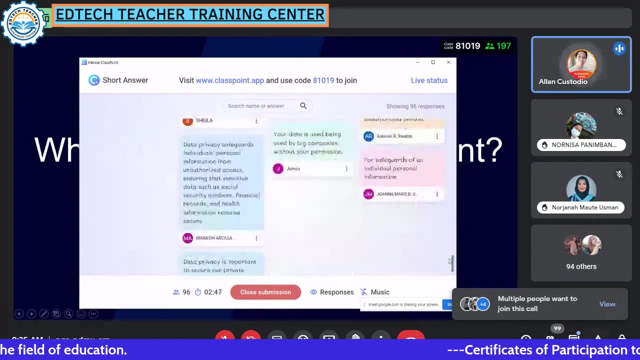 walang privacy, eh, masisira lahat ng mga effort natin, lalo na ikapayapaan and peace and order sa ating country, pag walang privacy, okay. okay, kung kayo po ayan, no, kung kayo po ay nasisiyahan. 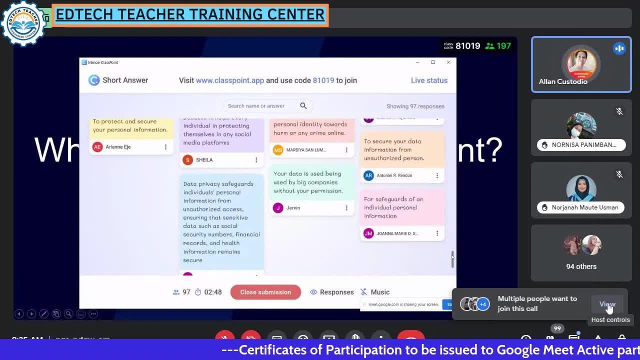 ayan, nasisiyahan din po ako, din ang dami po ating sumasagot. so 198 konti na lang, dalawa na lang po sa slot ng class point at lahat po kayo ay makikita yung sagot. 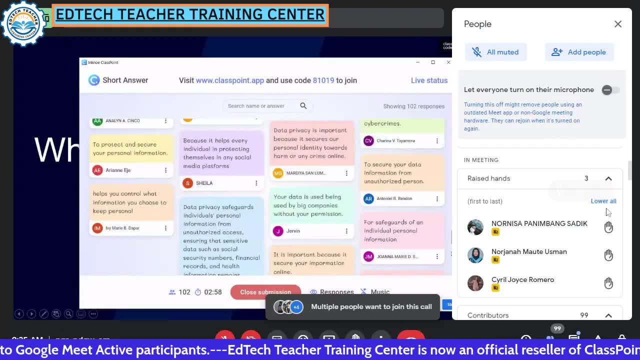 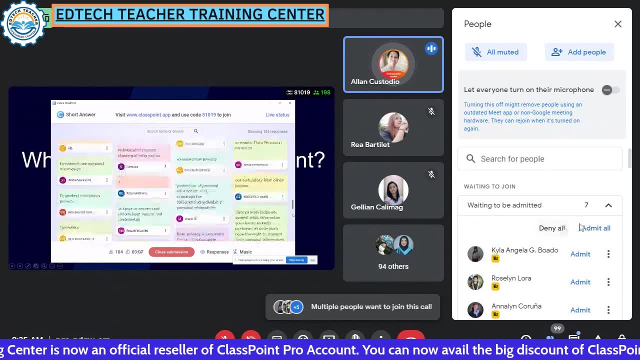 ibababa natin. ayan, makikita nyo. no, ma'am Arlian, ma'am Sheila, ma'am Mardia, sir Antoniel, ma'am Sharina, sir Jen, ma'am Rose, ma'am Annalyn, ma'am Rina, ma'am Marie. okay, so lahat po. 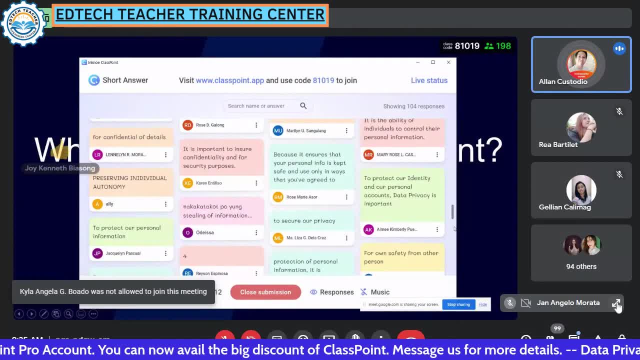 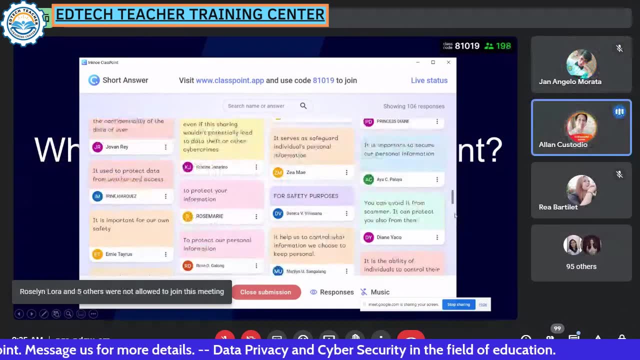 ito tama? no, ma'am Marie, ma'am Karen, ma'am Alay, ano pa ba dito. ma'am Danica, ma'am Rosemary, sir Jovan, ma'am Princess, sir Raul, ma'am Pweenie, ayan ang dami sir Jason. so lahat po. 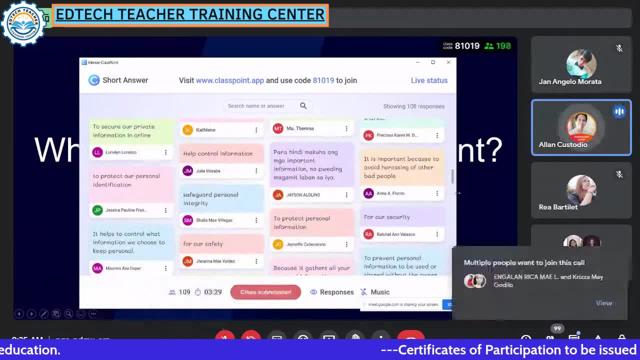 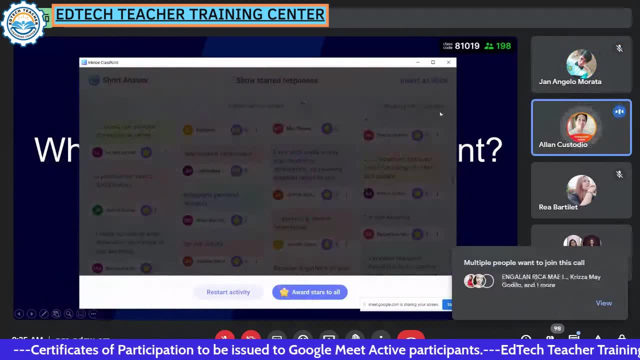 ng sinasabi nyo ay tama, at napakaganda ng sharing natin. and let me close po natin ayan and award all stars. okay, so sa pagpapatuloy natin. ah, okay, the importance, eto pinaliwanag ko rin. 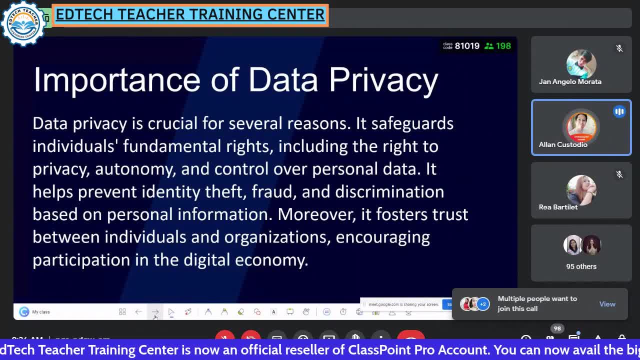 kanina at mababasa nyo dito sa ating ah, meaning na fundamental talaga na magkaroon tayo ng right ibig sabihin, maintindihan natin mas malalim yung mga bagay. kung irerespeto. 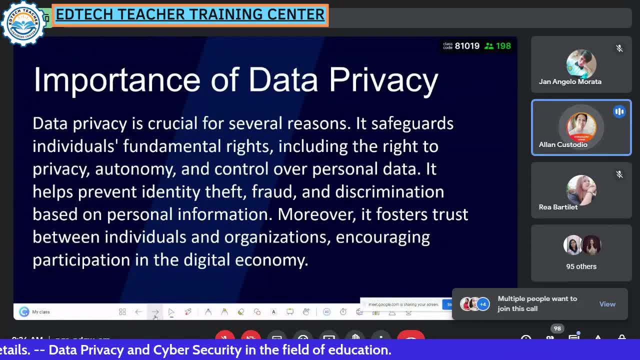 yung ating ah individual na data sa pagkataon natin. kasi kapag nawala ito, ang mga nangyayari sa atin makakakontrol yung ibang tao ng personal na buhay natin. 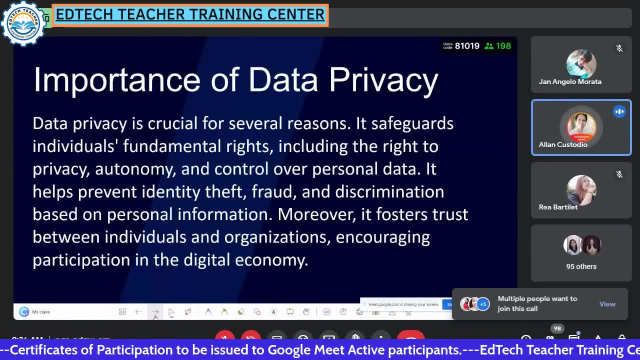 kasi alam niya lahat, eh. so dadami magbablackmail. so, moreover, posture between individual and organization encourage participation in the digital economy. so lahat tayo ina-encourage na magkaroon ng trust. tiwala sa mamamagitan din. 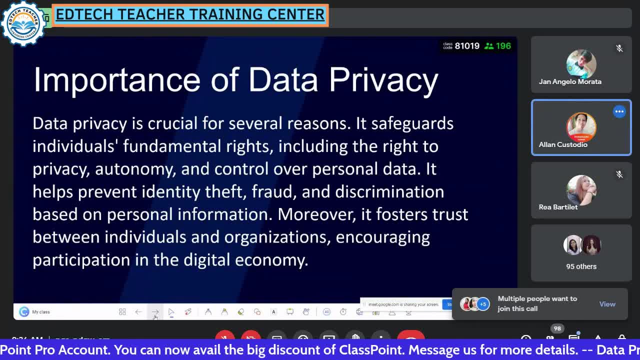 ng mga limitasyon na hindi na dapat natin gawin para nang sa ganun yung yung ekonomiya natin. ano na po ba ekonomiya ngayon, physical o digital? kung titignan niyo kasi ano eh. 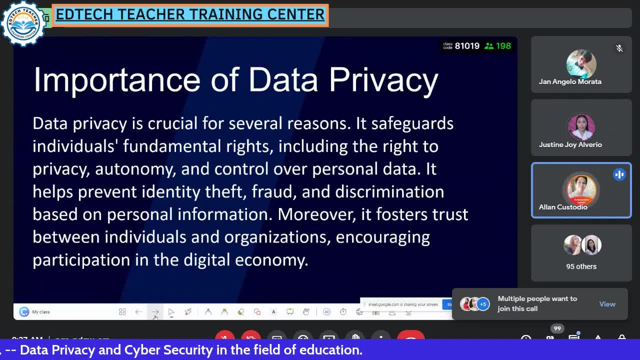 nahati na siya at papalaki po ng papalaki digital digital economy saan umiikot ang pera. makikita niyo diba mga charts, saan niyo makikita yung mga logistic statistics, analytics, lahat po yun. 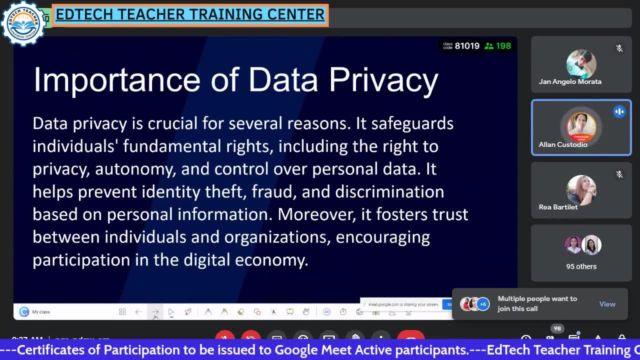 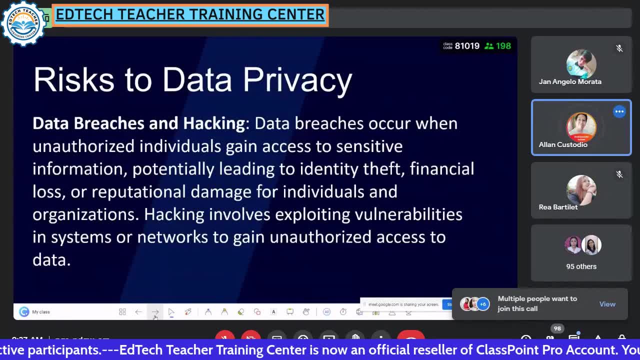 digital. eh di po masusulat ng tao yun. eh oo, mapiprint mo, pero lahat ng presentation na yun ay digital, at lahat yun ay may privacy. okay, so eto yung mga pag-uusapan pa natin. no. 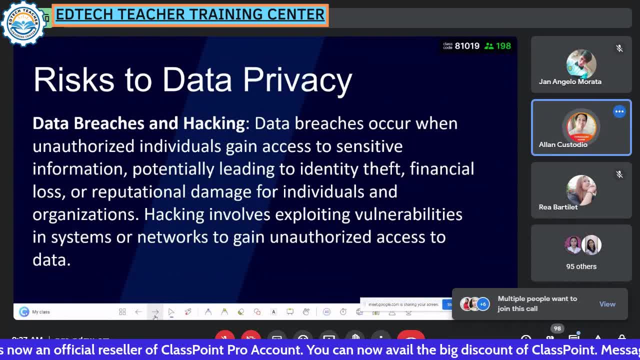 breaching and hacking. ano ang breaching, ano ang unauthorized disclosure? papaliwanag natin, mamaya yan. so eto yung mga risk na data privacy. mamaya, papakalalim po ako dyan ngayon, may pangalawa tayo. 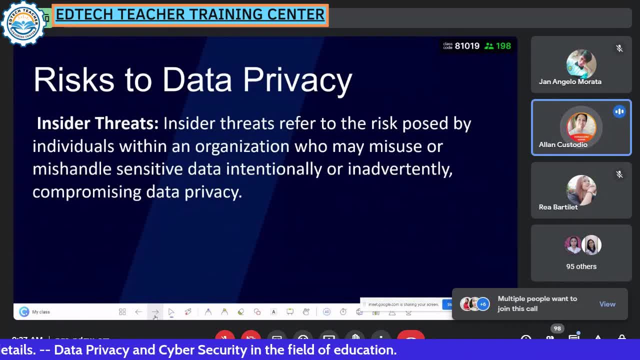 insider threats, mga taong hindi naman authorized. pero mabubuksan yung facebook mo, ayan mamaya nangihiram na bata. tas binuksan yung facebook mo, mamaya papakalalim po tayo. third party data sharing. 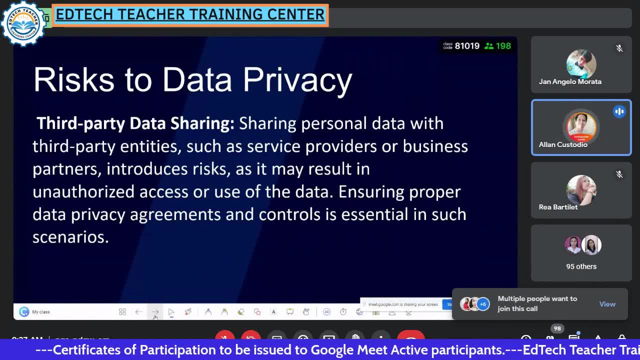 nag accept ka ng cookies. bago mo i-accept, tingnan mo yung mga terms doon nakalagay doon. after you are clicking this cookie, you are agreed to share your location. bla, bla, bla. tingnan yung mabuti yun. 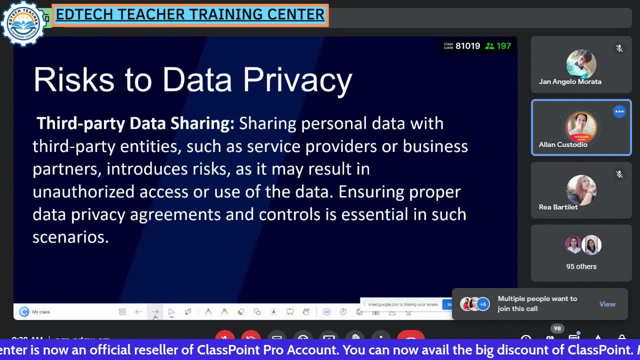 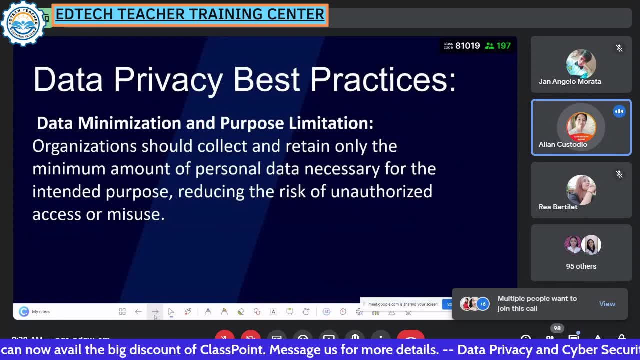 tas nakalagay pa pala internal storage. patay tayo dyan makikita talaga lahat ng baka. mayroon ka pang number ng bank account. data minimination purpose and limitation. sino ba dapat ang magpaprotecta sa school? 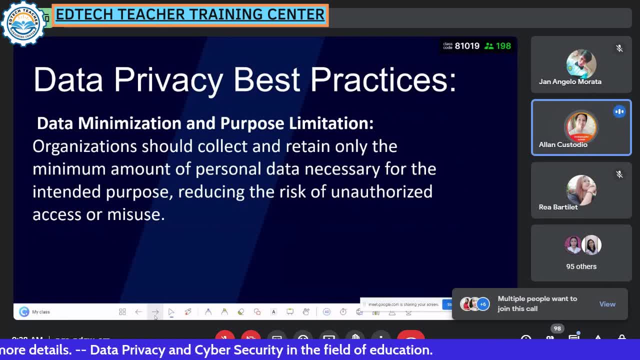 sa school page. sino ba ang mga tinatawag nating data protection officer, DPO? sino ba ang mga dapat makalaman ng iyong password sa facebook or kahit saang mga bagay? sino ba dapat ang mga nakakaalam ng mga tao? 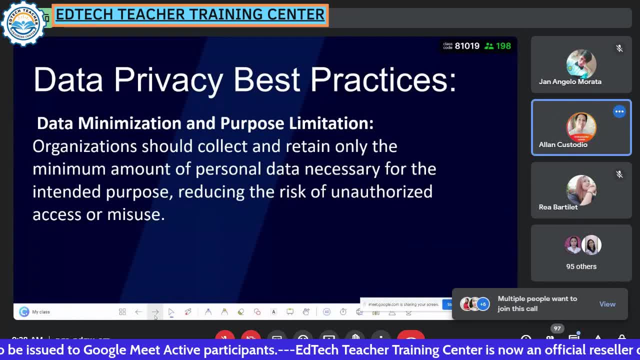 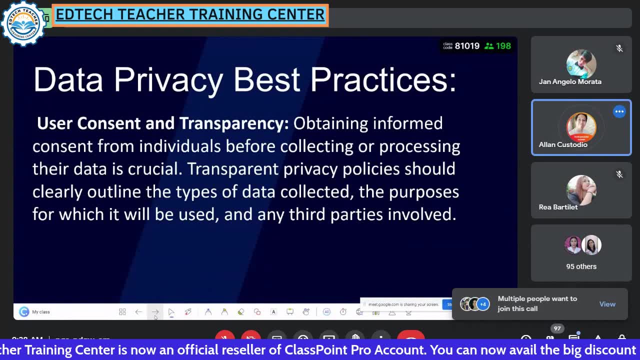 or ma-minimize yung mga pangyayari na yun. mamaya iditingnan nating mabuti. yan yung consent and transparency. eto yung mga best practices, pag may ganito ka. eto yung tinatawag na kuwan e. 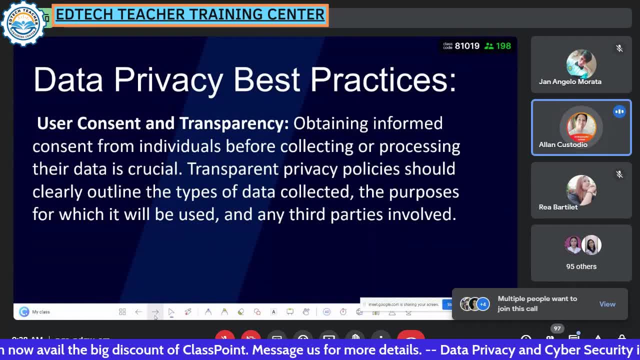 example, simple example: humiram ka ng walis tambo sa kabilang room ngayon. paggamitin mo yung consent. anak, hiram ka nga kayo mam nang ganito, kasi wag ka mo nang kumuha mag good morning ka. 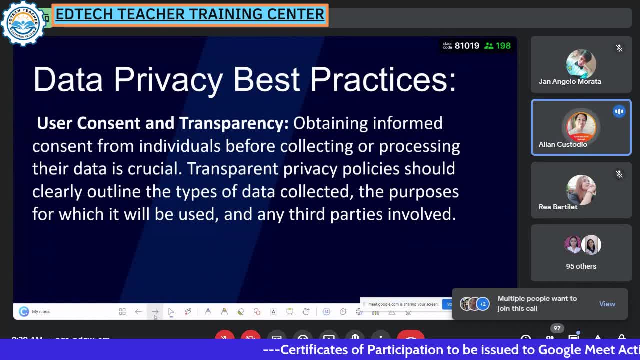 humiram ka kasi. eh, hindi natin mahanap yung walis tingteng may bisita right consent po no. and then sa transparency o ibalik natin pagkatapos, kasi talagang gagamitin din nila. mam. 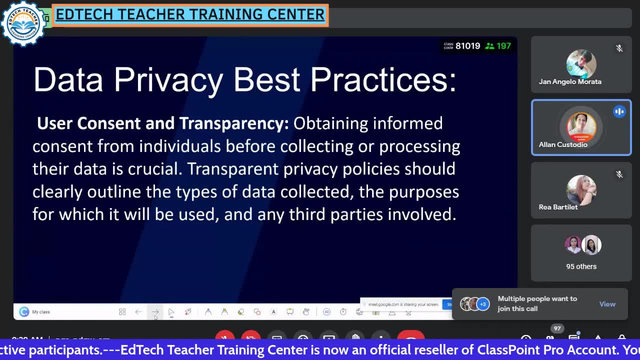 hiram lang tayo ng isa. so yung consent and transparency kailangan yan meron. nakikita, yung may ebidensya, nakikita na maayos na nakikipag ugnayan ng bawat isa. usually ang consent pwede rin yan a piece of paper. 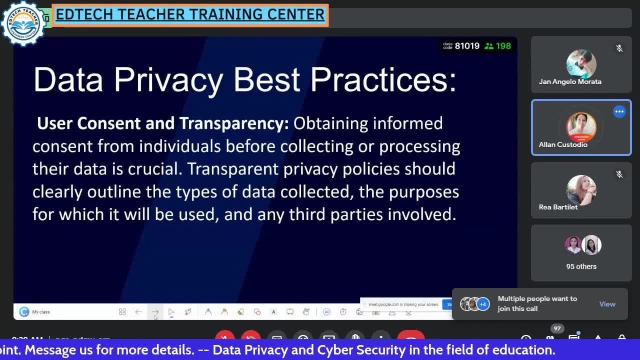 when we say a piece of paper, eto yung agreement. pwede sa guidance office, pwedeng consent na papayagay niyong anak mag tour, at marami pang iba. kapag nabaliwala, yan ay magkakaroon ng. 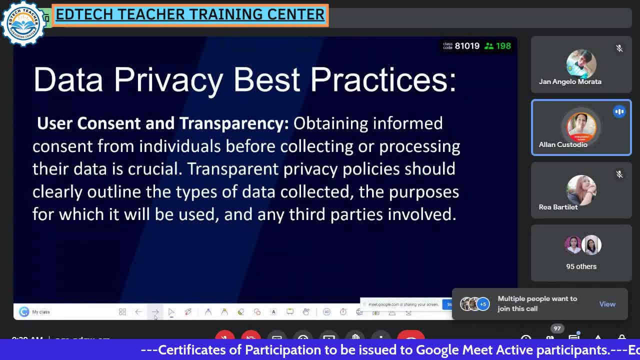 hindi balancing usapan at hindi maganda yung kalalabasan ng kahit anong usapan, lalo na kung natatamaan ang privacy natin, ibig sabihin yung pag oo at hindi at pagproseso ng ating mga informasyon. 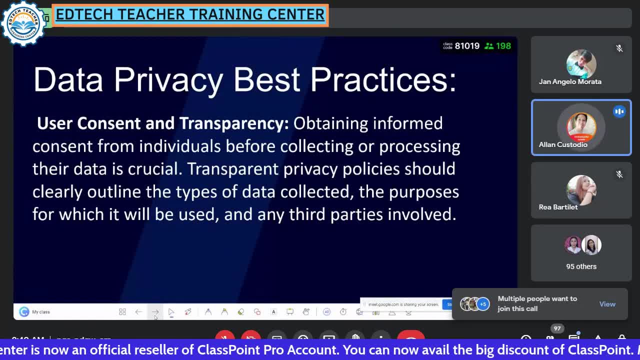 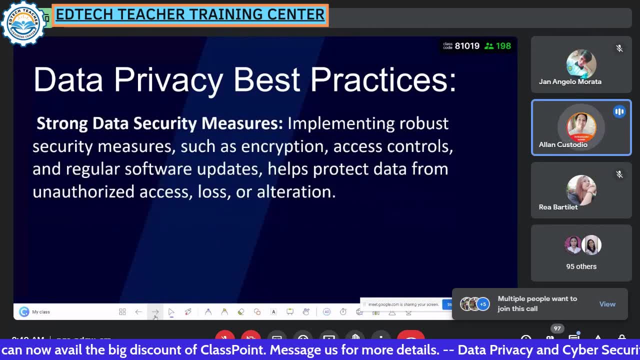 okay, kung kayo ay natutuwa sa usapan natin, magchat kayo number 6 ayan. magchat nga po kay number 6 ayan sa pagpapatuloy natin. next natin we have the data best practices. 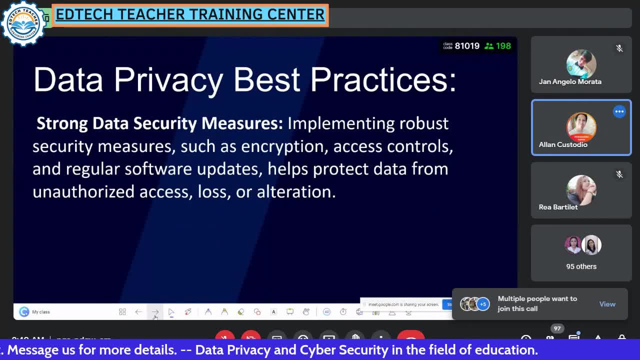 strong data measure ayan, so sa strong data measure ay kailangan malaman niyo. mamaya tuturuan ko kayong mag meta facebook na kung saan ano ang latest ni facebook sa data security? dapat alam to ng buong yung ano eh. 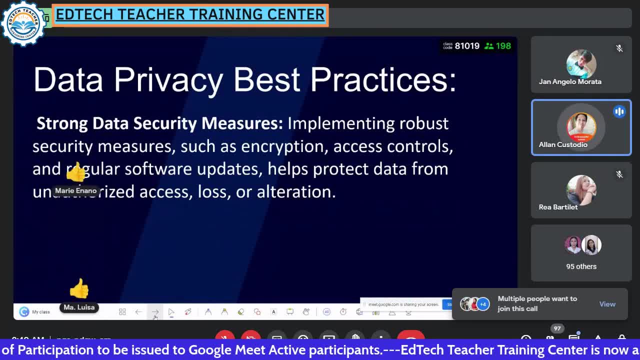 ng mga estudyante. eh, as of the latest survey, 2022, by hatsuit ayan, ginagamit po namin yan maski sa common sense ambasador, na ang Pilipino daw ay marami silang social media, pero may isang application na nangingibaba. 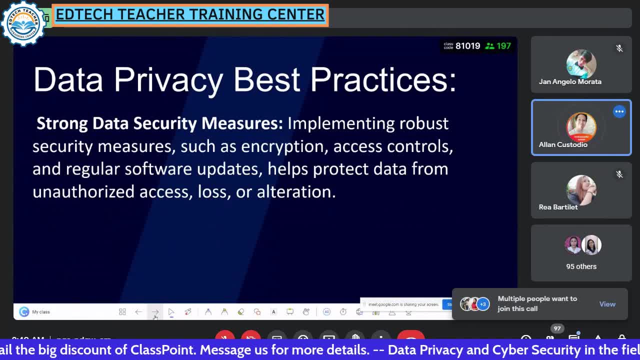 which is the facebook, and 99% out of the survey ay nagsasabing alam nila ang facebook o may meron sila nito, o ibig sabihin ang mga hacker ay halos andoon at sinatarget nila yung matatanda. 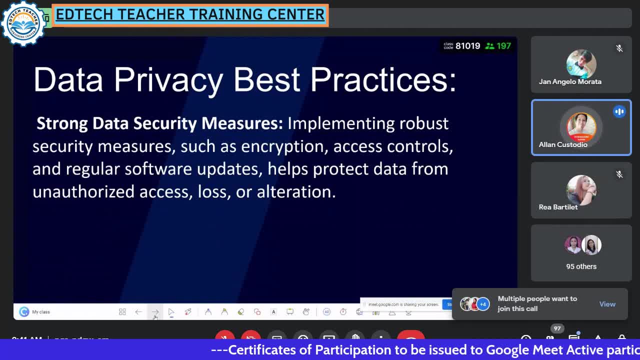 sinatarget yung mga nanay natin, pwede rin targetin yung kabataan sa pamamagitan ng catfishing. when we say catfishing ay poser, poser, pala siya. patay tayo sa mga poser na yan. 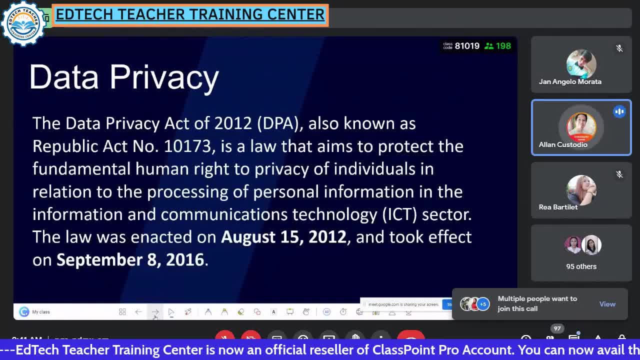 ngayon. kailangan nilang malaman yun, mamaya ah. so sa data privacy, eto na papasok tayo sa republic act 2012, dpa, also known as 173. yung sinabi ni sir kanina, nakita ko no. 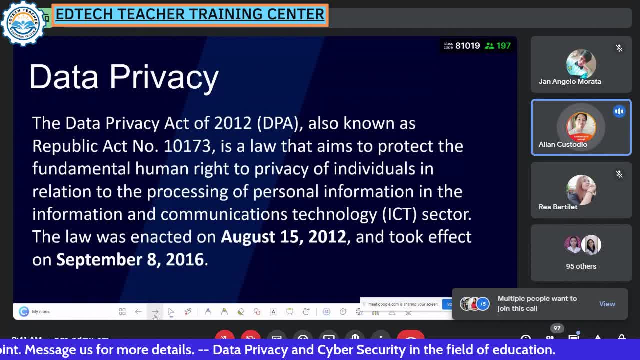 ah pinirma nito ni late presidency ah minoy aquino na august 15 2012 at effective nung september 18 2016. so ibig sabihin, may pangil na po ito no 2016, at talagang eto ay pinag-aralan. 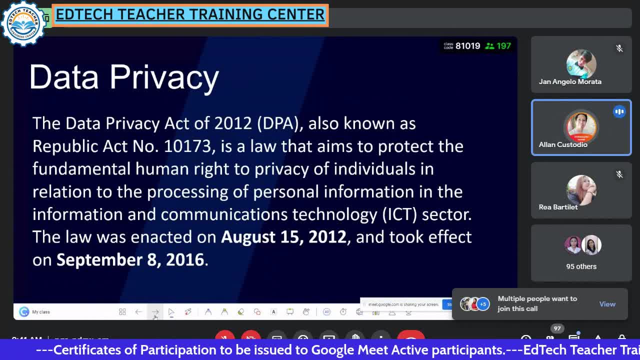 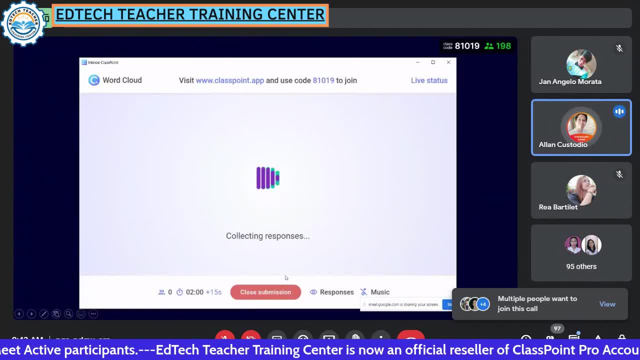 ng iba't ibang sektor, especially the ICT sector, at tung ano mga ipapataw na batas. so pero, bago yun, ano ba'y tinatawag nating precious detail, okay, ano ba'y mga dapat nyong pangalagaan. 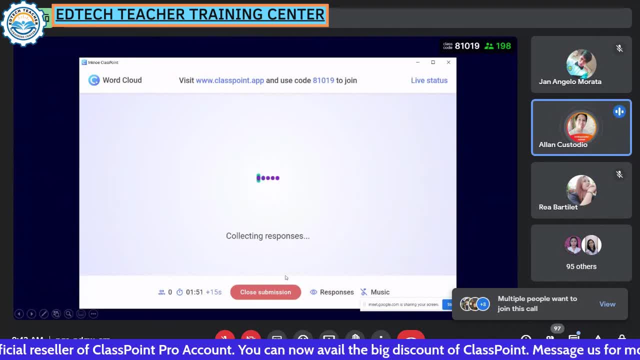 so sa class point we have 198 halos. ah, ano na puno, punong, puno na. so password correct. ano ang dapat nating pangalagaan? baba ko lang po, ah para makita nyo ito nung sa live yan. 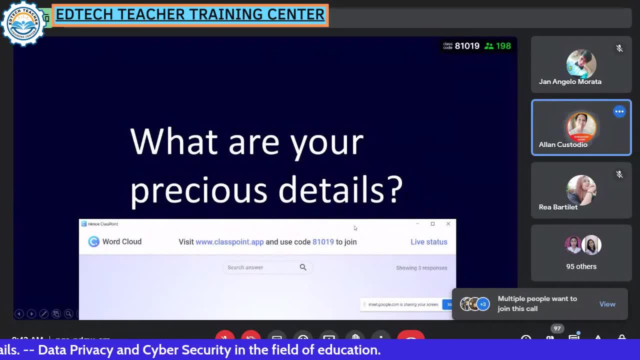 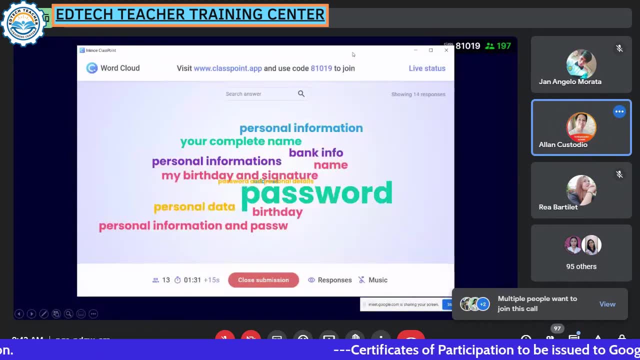 what are your precious detail yan? ano ba yung mga precious detail natin hm makikita natin hm. so we have the password, we have the personal signature, we have the address, we have the bank info. so lahat po ito no tama. 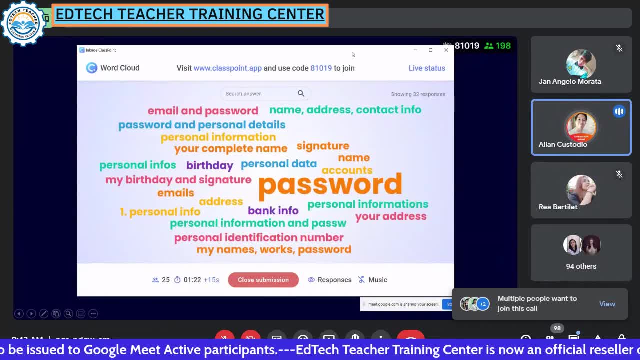 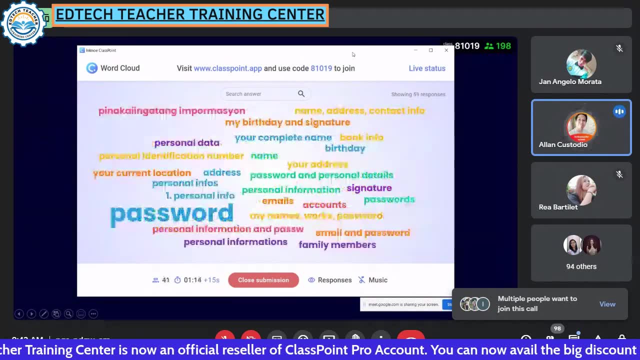 at talagang makikita nyo yung mga sagot nyo. full na po ang class point. thank you po. no, full na nga po eh, pero nasa, nagbabasa po ako sa live, nagbabasa po ako sa live sa facebook, ayan. 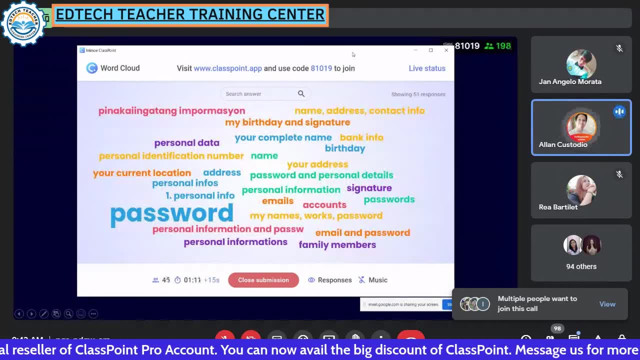 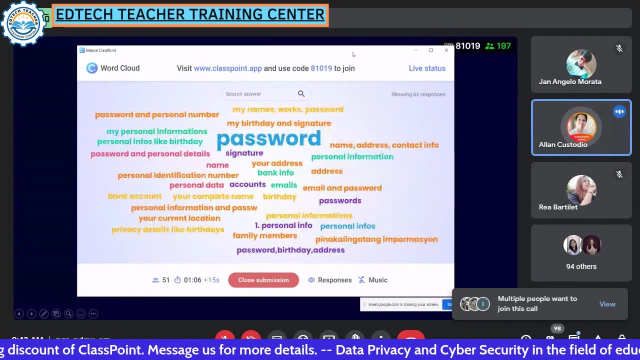 hindi po kayo mali-left behind, okay, no ah, nakikita po namin dito. maria luisa nagsabi po ng full mam may ann, ah, mam angeli, mam jezabel ayan, so ah, nakikita nyo dito. 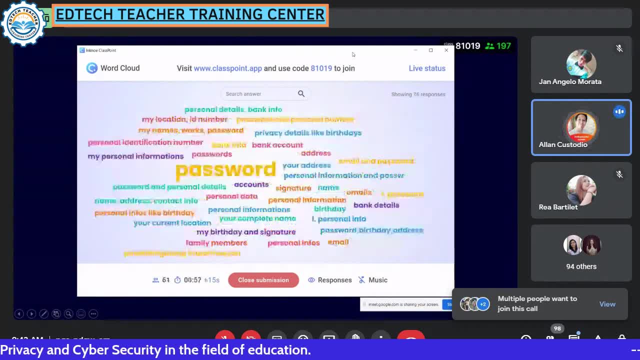 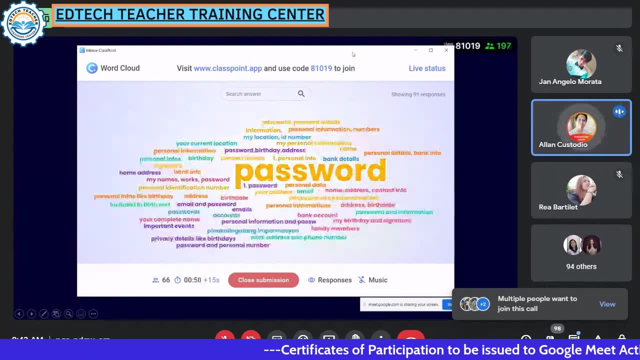 signature. nakita ko yung signature. pag ginaya yung signature mo nilapat sa iba ay nagkaka problema, kasi talagang magagamit yung rights mo sa mag pagpapawave or pag didisclose ng isang agreement. 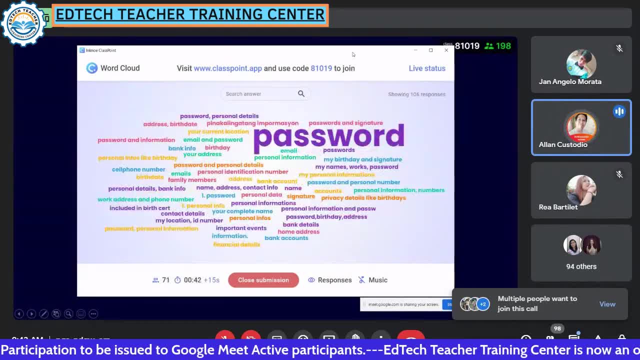 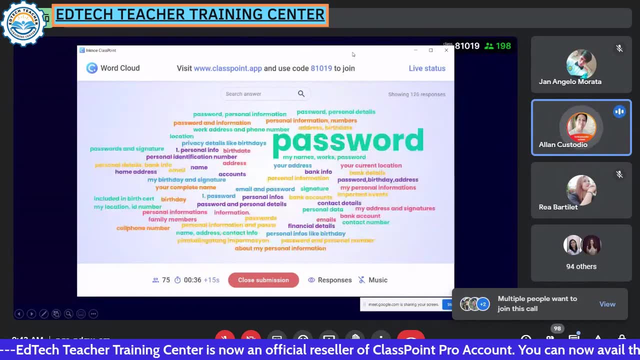 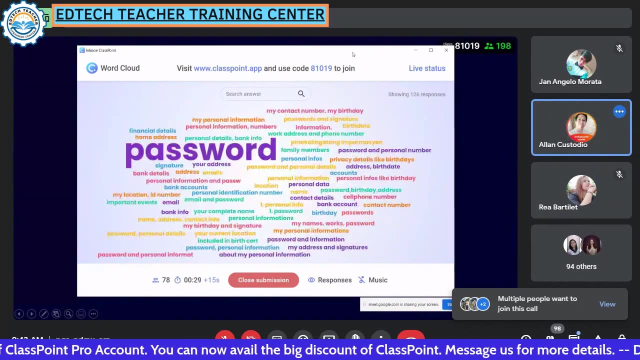 so dito, nakikita ko talaga na cellphone number talagang password ang pinakamatinde, kasi syempre alam natin ang daming secret na number, secret na password ng bank account, secret na password ng facebook mo, instagram, mo, twitter mo. 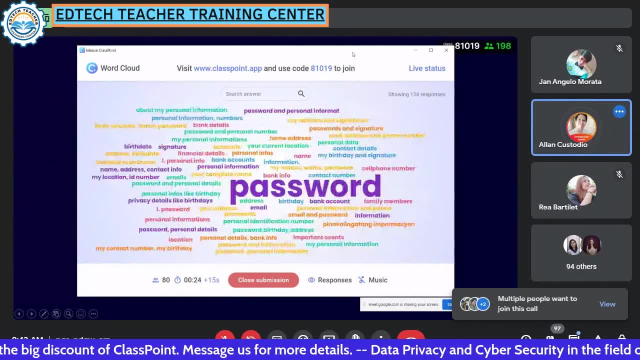 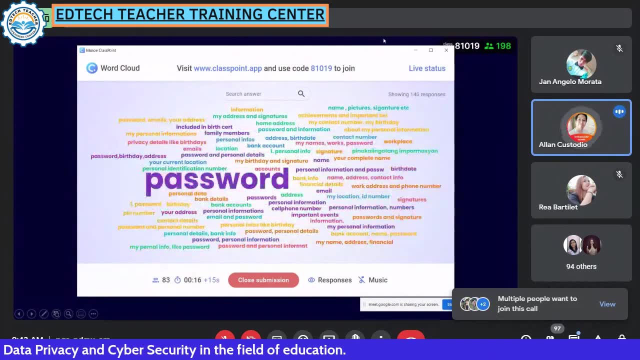 at lahat pang iba. okay, so napakadaming nagkakolaborate and napakagandang tingnan. okay na tayo ay nagkakolaborate. okay so cross ko na po. ah, lahat po yan tama and bigyan ko po kayo lahat. 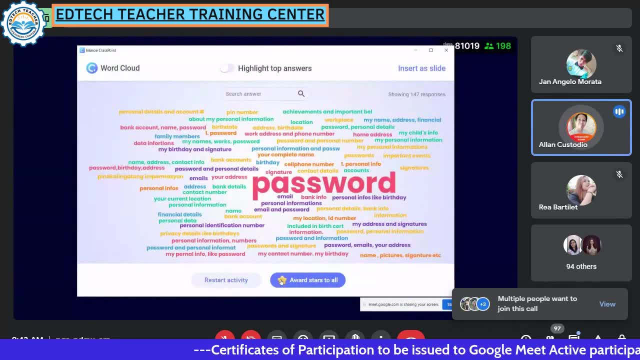 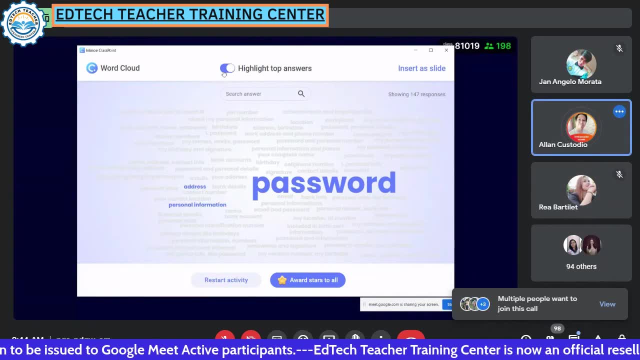 ng star. okay, so pinakamatindi pong sagot is password. so yan mamaya meron po akong sa slide dyan na hinanda password, address and personal information. okay, pero alam nyo po ba na may sensitive information, alam kong, alam nyo yun. 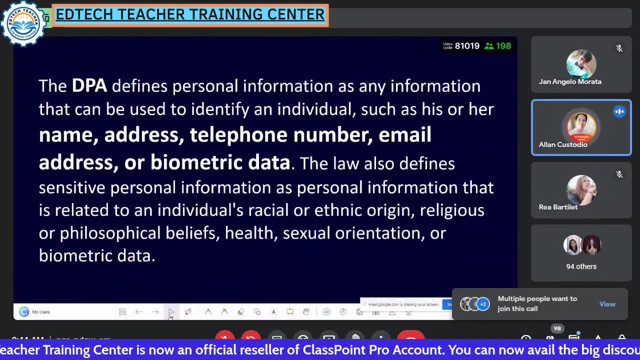 pero tuli po natin. the personal information refers to the name, address, telephone number and biometric data. biometric data po yung mga pinapunch natin ng ating footprint ay print ng ating footprint, ng ating ah finger natin. no ngayon. 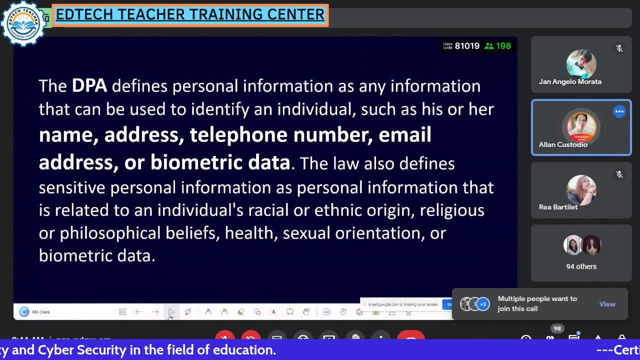 may tinatawag tayong sensitive information under yun kay personal information, which is ah racial, ethnic origin, religious belief, health, sexual orientation or biometric. sino po dito ang, kapag nakakakuha ng medical record ay nauna pa yung kasama. 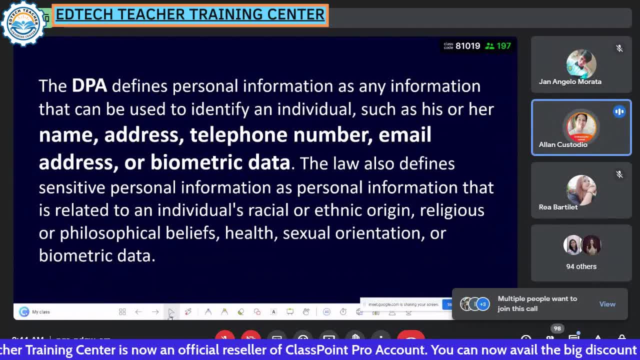 niyang makita. set nga po kay number seven. meron na po bang ah instances na yung medical record mo nauna pa yung kasama mong makakita that is confidential. set nga po tayo sa box natin number seven. bakit kaya? 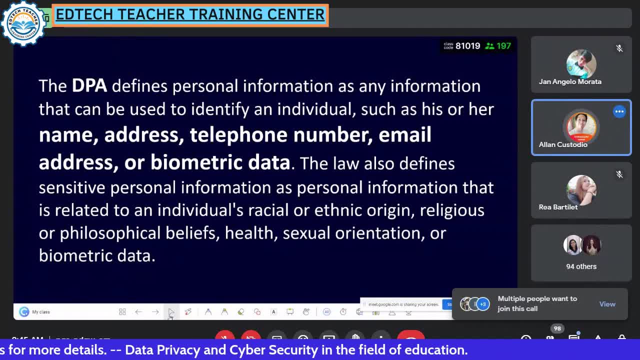 niya pinakailaman yun, yun ay confidential. nakapasok pa po yun sa mismong ah ah envelopes na brown ayan o ng mga experience. so ngayon alam nyo na po: no, ang tangi makakita lang nun. 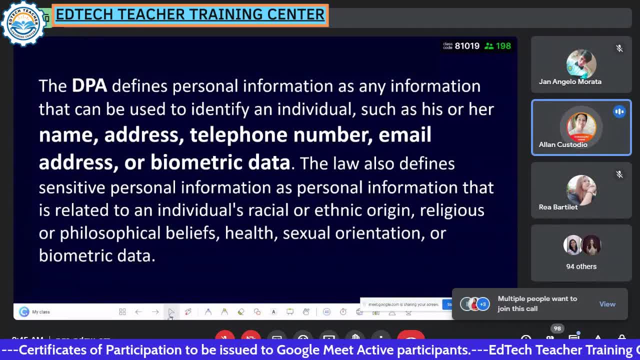 ay yung siyempre, yung nurse kinagpadala at saka yung talagang nurse nyo sa school, kasi sya yung pwede magpayo pa, pero hanggat nga maaari, ay dapat. eh, ikaw lang talagang nakakaalam nun. 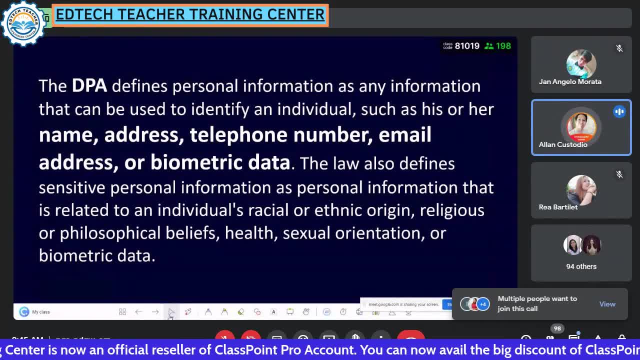 kasi yun ay high sensitive information under personal, yung health, sexual orientation at saka yung religion mo. pwede mong sabihin kung hindi kinakailangan mag reject, mag object kung ayaw mong sabihin yung religion mo sa isang tao. 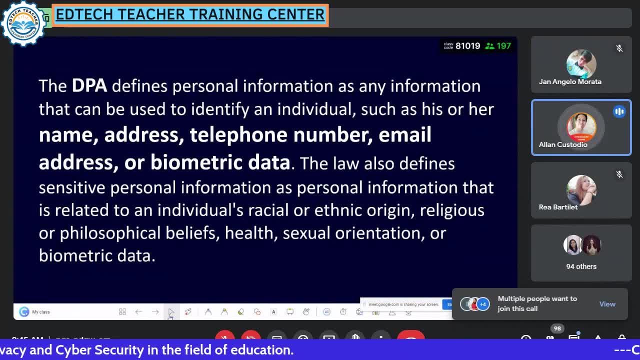 pwede mo rin namang. ah, may karapatan ka, kung ano ang iyong ah nation, filipino, amerika ka o europe, nang lahat ng yun ay maging confidential para sayo. okay, nasa sayo po yun, kasi yun ang. 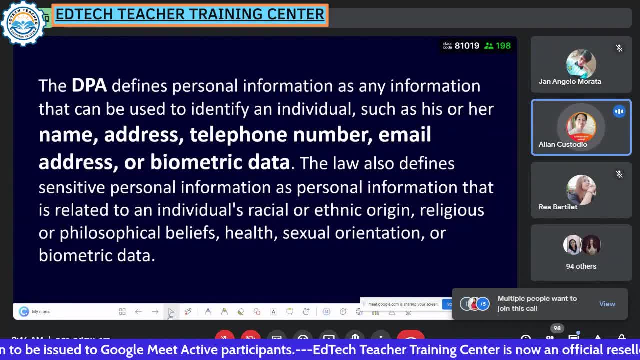 ah. sensitive na to. eh, ibig sabihin highly confidential na to. alam natin, na alamin natin yung ah ah, ah ah, cokie, ano, kung gusto mong sabihin yung pangalan mo o hindi, tama po ba? e pa pwano pa yung sensitive. 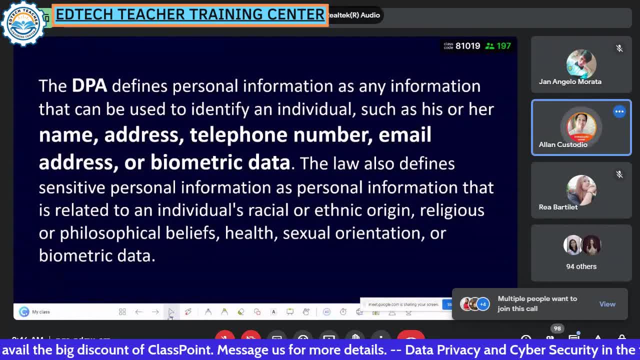 dapat. eto talaga kinakeare of. so ang dami po nagsgeben. kaya po sa susunod ay: protectahan niyo bawal makikita ng iba at huwag kayong papayag at binababy nyo na lang. 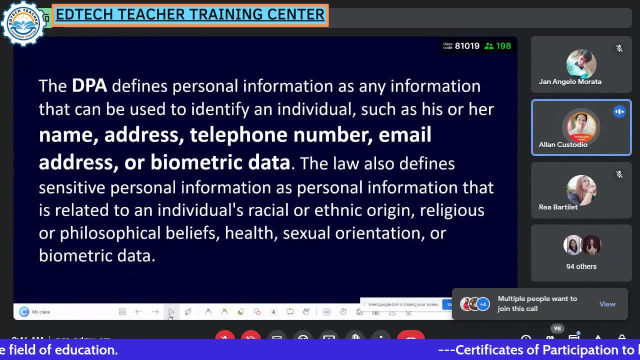 porkit na bestfriend mo, andito na yung medical mo, o pwede mo ko bang makita? oh yes, pwede any time. oh e pa pwano pala pag nakita may taneng ang buhay mo, Tapos minare-test ka. ayaw mo sanang ganun ang mangyari, kasi gusto mong i-treat ng confidential. 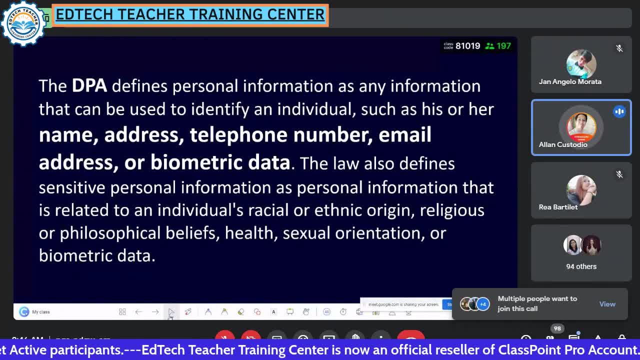 Paano yun Sige tanungin ko kayo Nakalagay doon? meron ko na palang stage 2 cancer Ngayon nakita niya na bigla siya and then she learned niya. 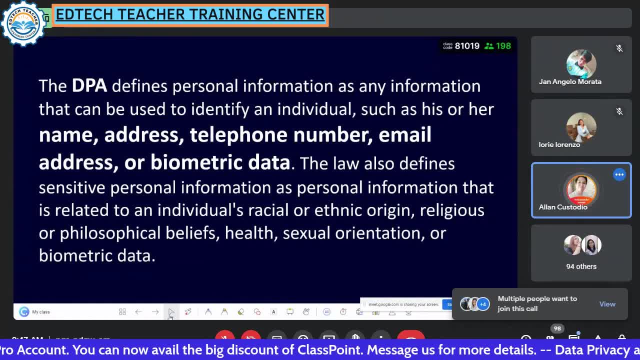 Bigla niyang na-share at hindi niya inaasam, binura niya kumamin sa'yo Kaso na-screenshot na ala na kumalat na Ngayon. lagi natin tandaan to. 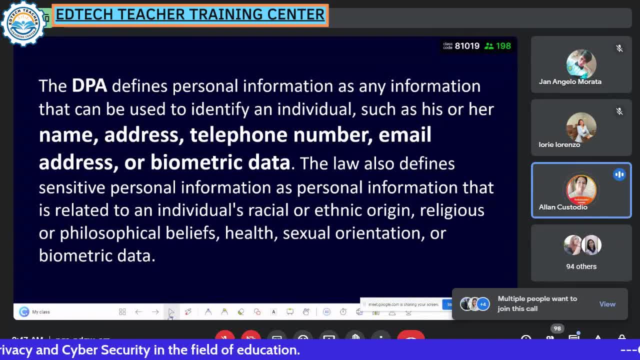 Hindi porkit na best friend mo, Hindi porkit na makalapit sa'yo yung mga bagay na sensitive ay ibibigay mo na Hindi ganun yun. Huwag niyong bibihin ang mga kaibigan nyo na nanghihingi ng hindi dapat at may limitasyon. 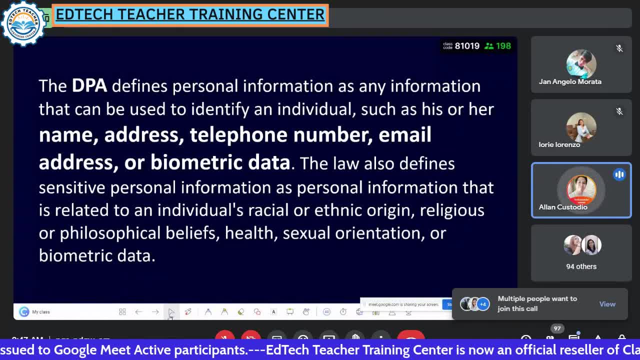 Kung nag-agree po kayo number 8.. Huwag niyong silang bibihin, kasi porkit ba na ano, Ganun na lang ba yun. Hindi po ganun. yun. Okay, number 8, nga, kung kayo ay naniniwala sa sinasabi ko. 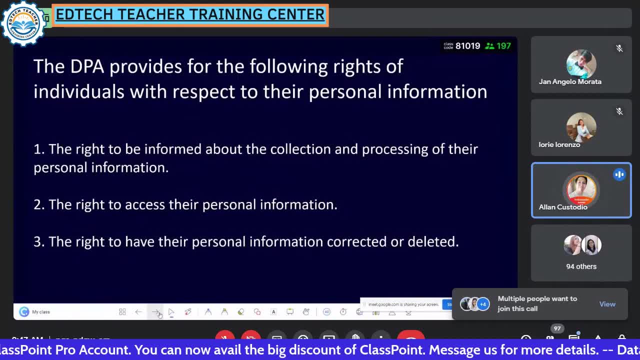 Ayan, maraming salamat po, Kasi kailangan talaga natin na pangalagaan ang lahat ng informasyon, Especially yung sensitive. talaga Okay, Grades ng bata nga sensitive, eh Diba. 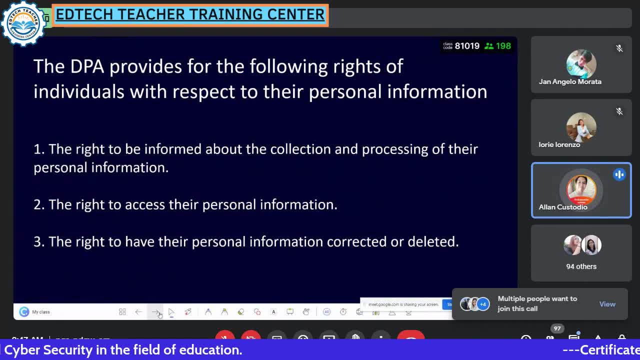 Anggat maari magulang lang at siya Bawal yun sabihin sa ibang bata na hindi naman niya grades. Am I right? At nabubuksan lang yung confidentiality ng record mo? 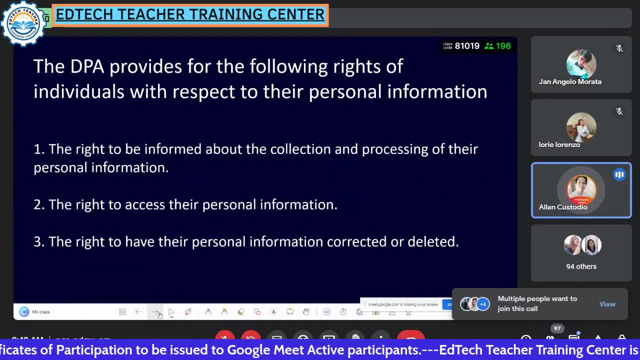 babag merong magulang na gustong makita. Pero yung bata na gusto niya at hindi naman sa kanya, yung pangalan ay hindi po pwede. Kahit anong gawin niya, hindi po pwede. 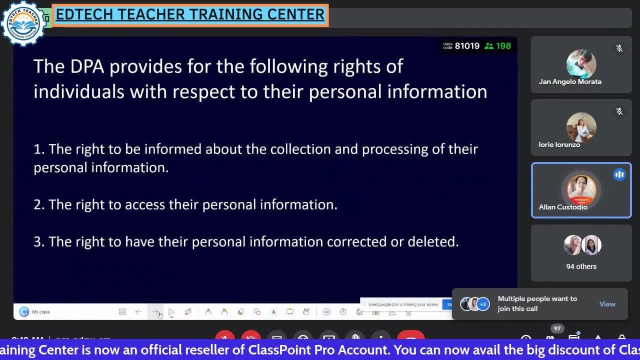 Kasi yun karapatan ng ibang bata, yung grades na yun Okay, Agrees sila O huwag natin binibaby ang mga alam nyo na Hindi naman sa pagiging best friend kasi. 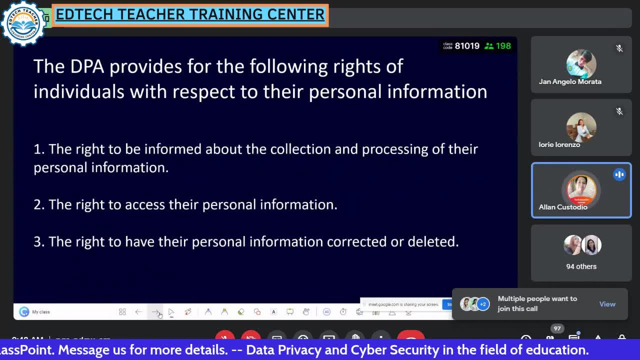 Imaginin Kung best friend mo siya maiintindihan ka niya na yun ay confidential At doon mo mapapatunayan na hindi ka niya imamaretest Kasi nag-agree siya eh. 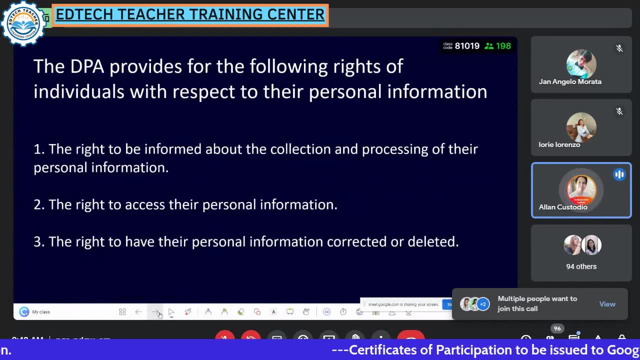 Na huwag nang malama yung mga bagay na yun At dapat naiintindihan niya yun. Okay, Kaysa magpapatuloy natin sa DPA daw may individual respect and their information tayo. 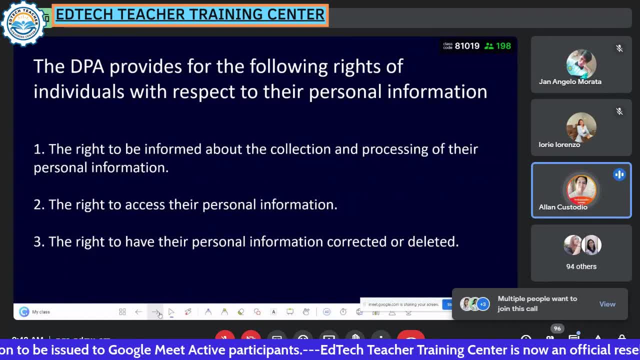 Ito yung tinatawag natin. Pag ikaw kinolectahan ka ng information na kung saan pinroseso ang iyong personal information, eh kailangan ma-inform ka Example. bigyan ko kayo example. 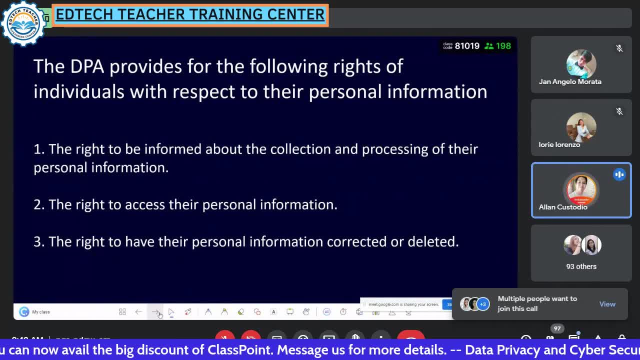 Gagawan ka ng ID, pero hindi sinasabi sa'yo Ganito gagawin. Sir, amin na po yung pangalan, address nyo, Amin na po lahat ng ganito ding social medium nyo po. 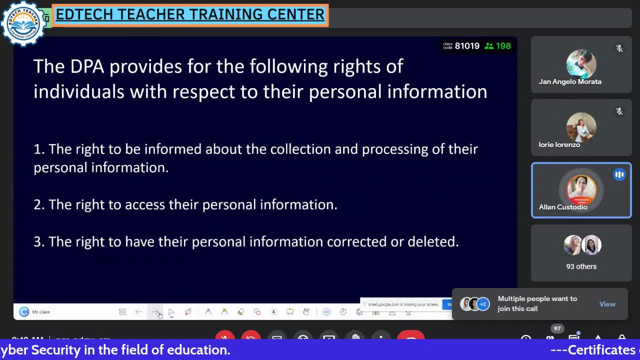 At saka yung pangalan nito: Pipirma po, sa likod ng ID ng ano nyo gagawin namin. Eh, para saan ba ginagawa na yan? Para saan ba yan? Tapos sumagot siya. 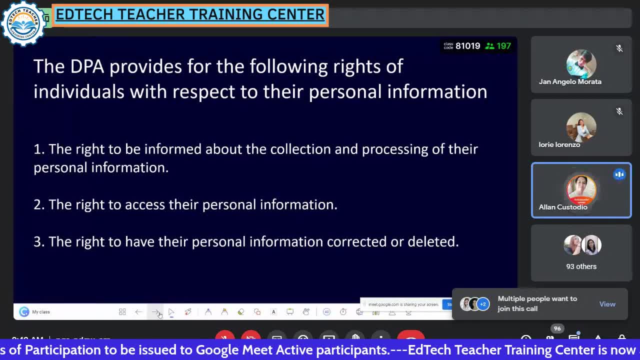 Ay, wala po, sir, Basta po ibigay nyo na lang. Kailangan po ng company. Hindi pwede yun. Hindi po pwede yun na hindi ka ma-inform kung saan gagamitin Walang ganon. 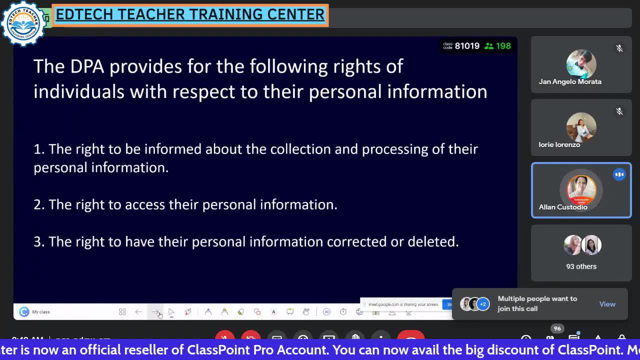 So lagi nyong tatandaan na may rights kang ma-inform Saan, gagamitin ang information nyo. Bakit Ano ka ba doon? Diba empleyado ka doon. So may mga rights doon kapag pumirma ka ng kontrata na i-re-respect ka. 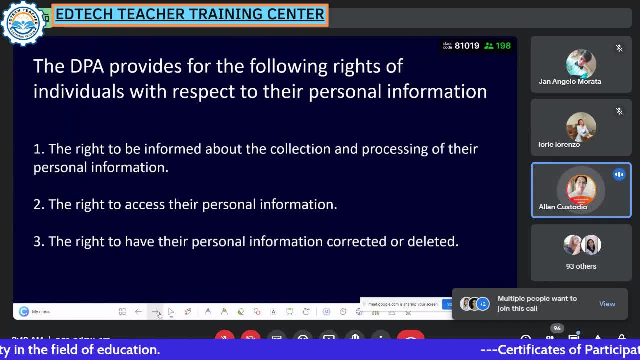 Pero nakalagay din naman doon na huwag kang gagawa ng unethical, Kasi pwede yung maging ground ng pagkatanggal mo, Diba Tama. So pero under ng DFA i-inform ka kung ano dapat ang ipoproseso sa'yo. 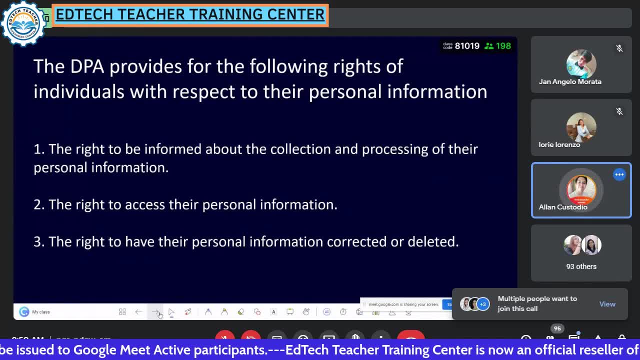 Number two Right to access Kapag ikaw ay kumukuha ng mga information at di ka nagpapaalam bawal yun. May nakita ka ganito, Yung iba naman po kasi ganito eh. 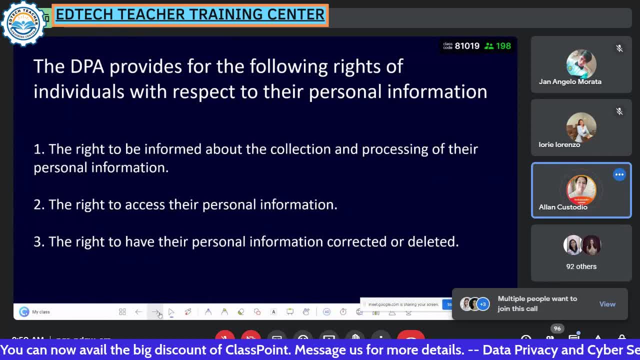 O Eto, Huwag niyo butong gagawin. Kapayo ko lang Maraming mga government employee na nakalagay yung pin number sa table Number ng pill health, sa table Number ng lahat doon sa ibabaw. 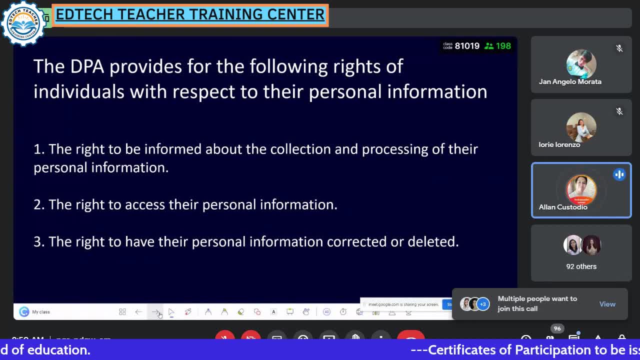 What is the point? The point is: hindi dapat nila makalimutan. Am I correct? Tama, Pero mas magandang itago doon sa may cabinet o sa merong hugutan sa ilalim at mag padlock. 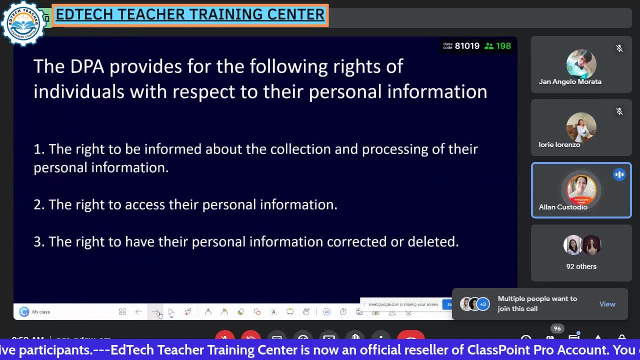 Because kasi yun ay sensitive information, Yung mga number na yan, Hindi yan po pwedeng ilantad sana. Pero marami kasing ang ginagawa ay taking for granted Sa sarili nila: Nare-realt ako po kayo ah. 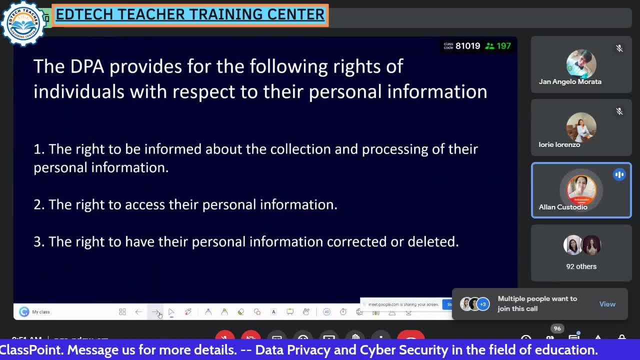 Inilalagay sa ibabaw, So yung iba nagtataka sila bakit nakukuha Eh nasa ibabaw ng table mo, Pati yung bata pinikturan na Eh may kaibigan siyang hacker. Hinak ngayon, yung nakalagay mo doon pin number at huwag ibinigay, Huwag niyong inilalagay sa ibabaw ng table niyo yung mga sensitive number, Tapos biglang magtataka kayo na hack na kayo. 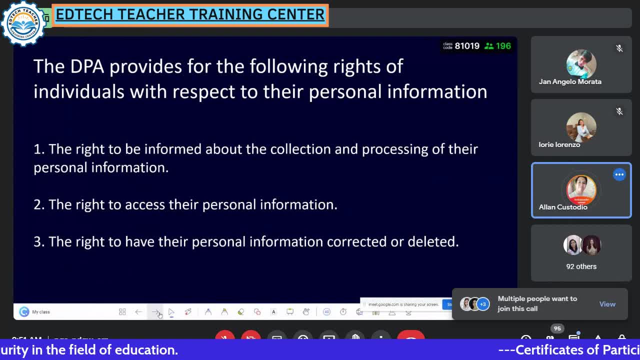 Okay, Marami, kasi talaga. eh Realt ako po kayo. ah Inilalagay sa ibabaw So yung iba nagtataka sila bakit nakukuha Eh nasa ibabaw ng table mo. 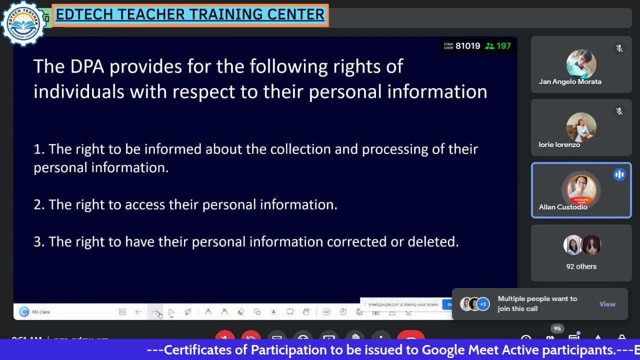 Ah, Hinak, ngayon yung nakalagay mo doon pin number at huwag ibinigay, Huwag niyong inilalagay sa ibabaw ng table niyo yung mga sensitive number. 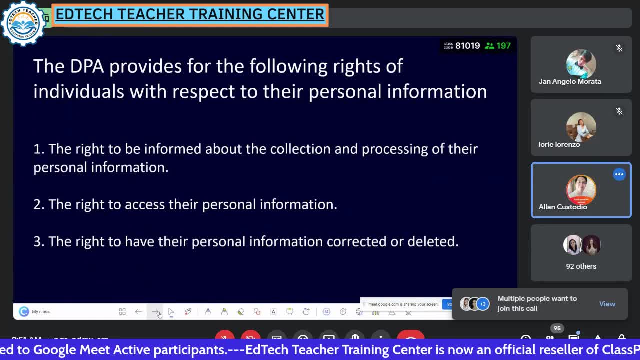 Tapos biglang magtataka: kayo na hack na kayo. Okay, Marami, kasi talaga, eh Realt, ako ko po kayo, kyon, Inilagay na niyo nalang doon sa may hugotan drawer at hi-padlock nyo. 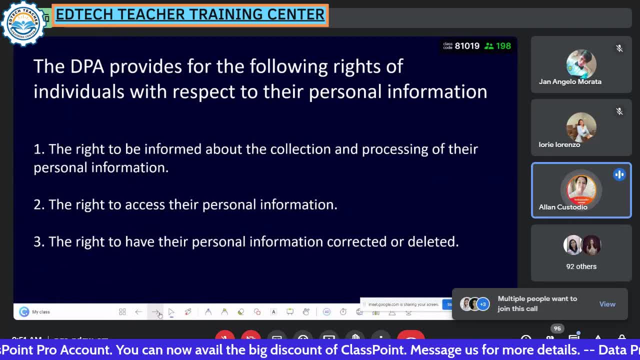 Pag may kumuha doon, Obligado pa siyang magpaalam sayo At hindi na niya basta titignan sa ibabaw mo. Magkakaroon ka ng rights at may save secured ka Yan. 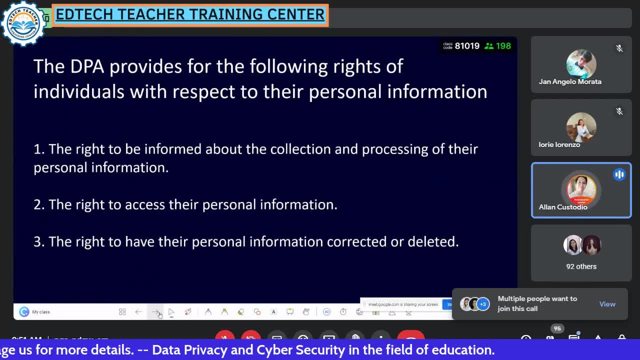 Sa inilalagay nang dapat gawin. okay, ayan no, pwede po bang gumawa ng mga fake ID. sempre po mali yun right to object ka rin doon. pag gumawa ka ng ID lead to falsification of document, it depends upon the severity. bibigyan ko mamaya kayo, kung ano po pwede, ikaso dyan. 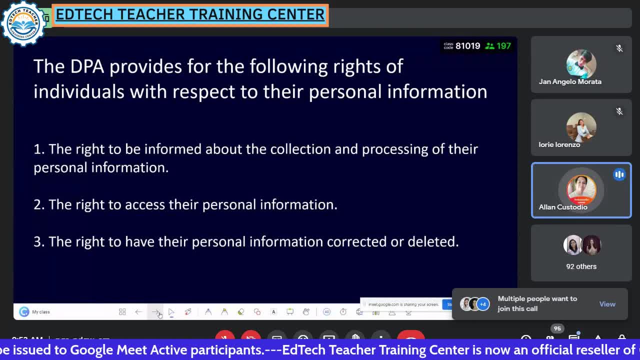 yung rights ng personal example: mali yung ID mo, gusto mo i-correct? wala ka bang karapatan sa kumpanya at saka sa kahit saan. abay malaki ang karapatan mo, pwede ka magpatama dyan. ipatama mo yung mga bagay na mali sa'yo ngayon. pag hindi ginawa yun, punta ka ng NPC at ayong ipatama. 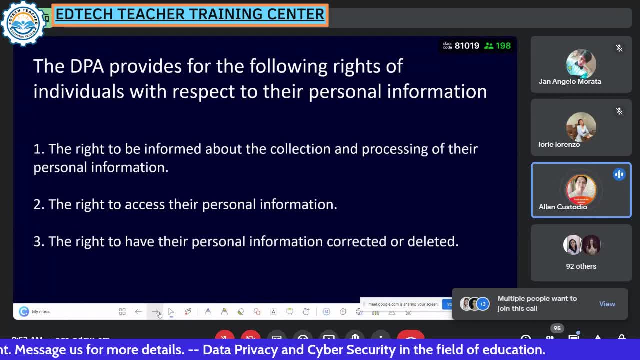 pwede ka siguro magreklamo, pero wala namang ayan siyang ganoon, kasi paano mong gagamitin yung maling ID mo kung hindi mo i-correct at kumuha ka ng pera? mali pangalan mo, hindi ka mababalidate, kahit saan gamitin mo yun, hindi ka validate. e mali yung pangalan mong, Jane, walang letter E. 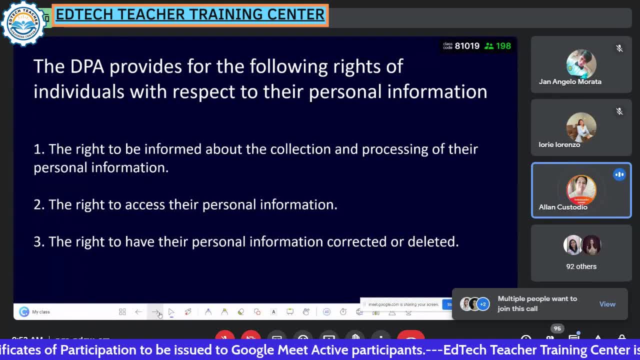 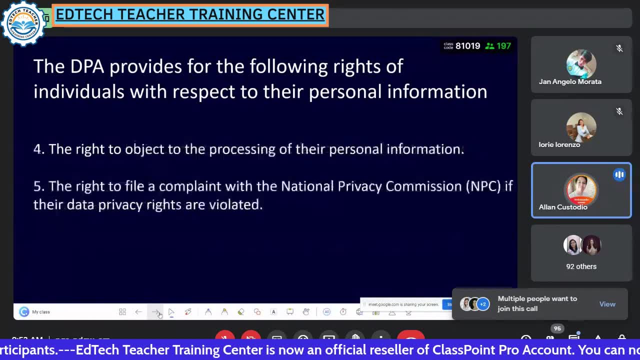 ang nakalagay ay triple E, isang letter E lang, sana yun. so hindi ka mababadalan example lang po. no ng mababang example, tuloy tayo. kailangan mong mag-object. eto yung ginagawa ng mga ID-ID. 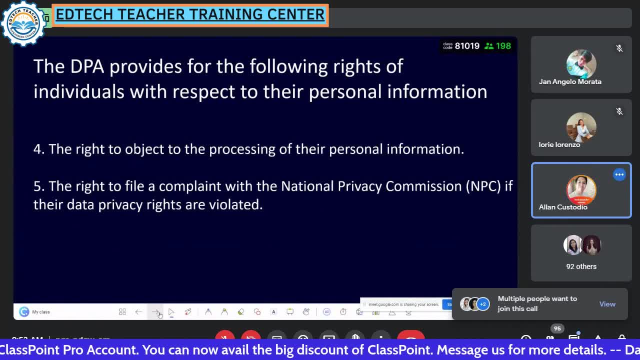 or kaya diploma, para lang makapag-abroad agad. eto po, ah, mahirap na po yung buhay. lahat naman hindi pantay-pantay estado, pero ginagawa pa illegal. kasi nga sabi siya: sir, walang makapita na matalim eh. 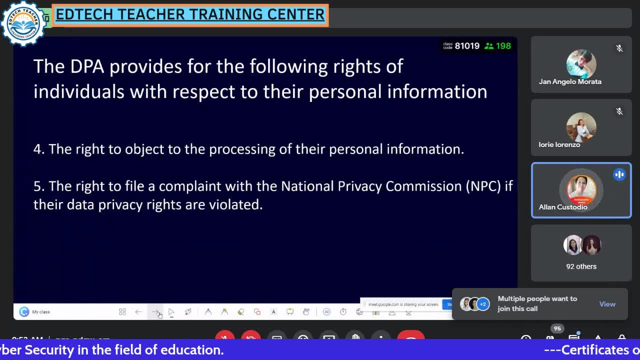 pero may papayo po ako sa inyo: ang isang mali ay hindi matatama ng isang mali. kaya kapag gumamit ka ng mga ganyang bagay, mahirap na ang buhay, lalong hihirap yan. 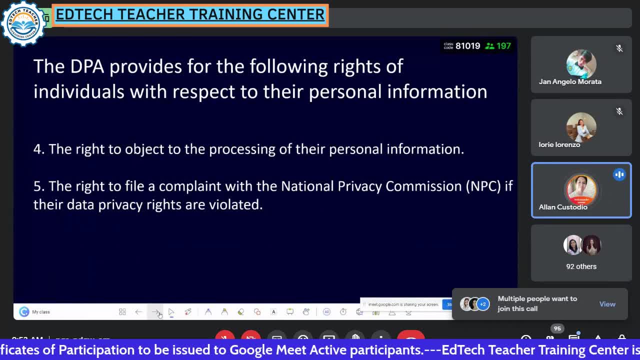 pag na huli ka at nahuli ka pa sa ibang bansa, nag TNT ka na dahil ala na eh alang choice. so lagi nating tatandaan na may tamang time para sa lahat ng bagay at huwag tayong susugal. 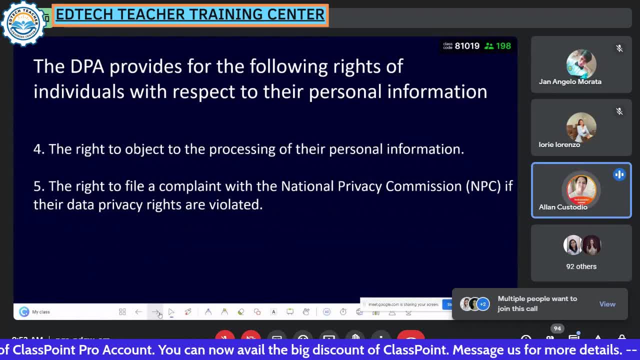 sa mga ganyang bagay na illegal, mahirap na yung buhay, lalo pa nating imamali. eh so sa tiyaga, at kung ano man ang gusto nating gawin, eh magkakablessing kung naniniwala po kayo. 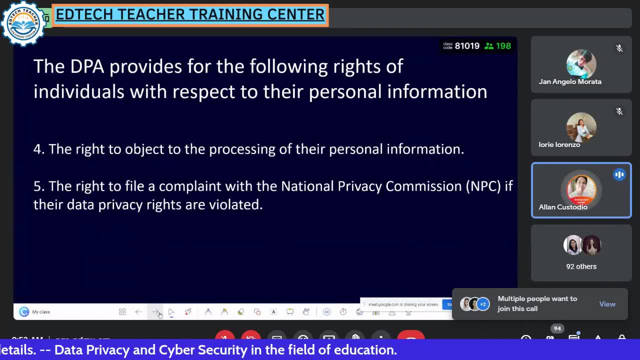 dyan. ako naniniwala hindi matatama ng mali ang isang mali, kailangan maitama yun ng tama. so huwag na tayong sumugal sa ganon. no falsification of document. ako lalo na. 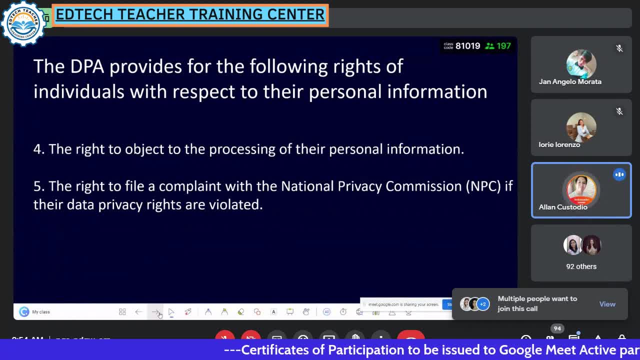 pag ikaw ay government employee para ma-promote, ay naku a big no may tamang time para ma-promote ka. tiyaga ka lang ngayon. tapos number 5: kailangan mong mag pwede kang magreklamo. yan yung sinasabi ko, kanina. 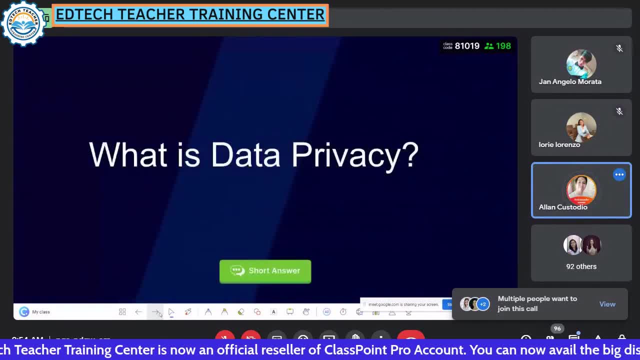 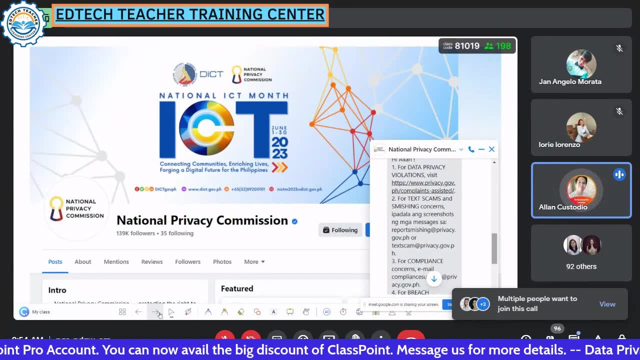 way back. so andito ba yun sa may ating ayan. punta ka sa facebook page ng national privacy commission under dyan yung mga iba't ibang klase may form ka. dyan pipilapan, hindi ka lang nasama sa presentation. 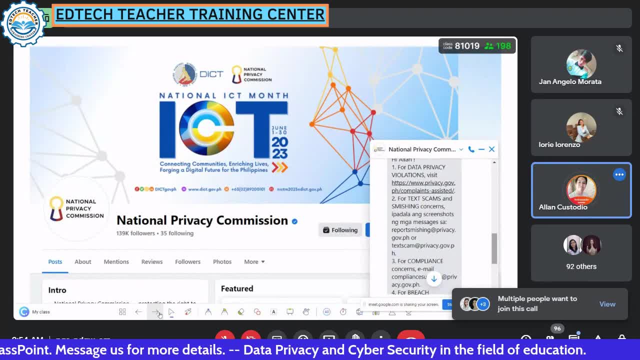 pero let me, let's check. yun na lang, po, at hanggang lahat ng klase na pwedeng reklamo. last time nagpakulong yung NPC nagbam joke sa kanila. pa talaga ng bam joke, so tinrace nakita sa ilo-ilo. 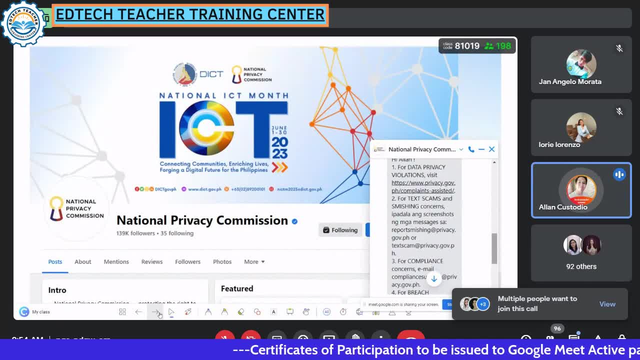 marami kasing dun kasi sa may NPC. marami pang masayang ngayon ng gobyerno nagtatrabaho may nagbabam joke dun so iba-iba ginamit ng mga FB na trace ayun binigyan sila ng. 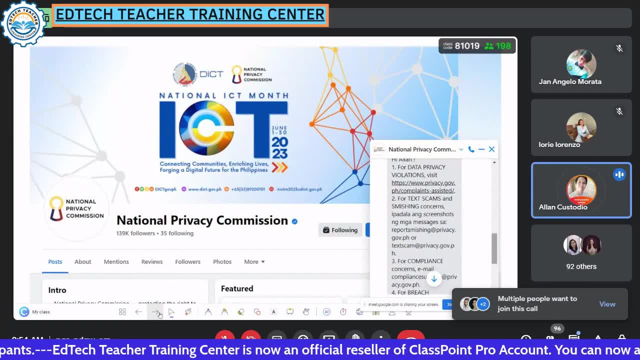 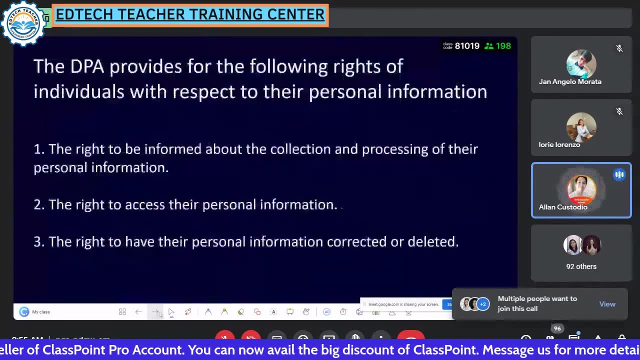 binigyan ng sanction yung taong nagtitrip. yan ang sinasabi nating mahirap. no, kasi hindi na alam ng ng ibang tao na ang joke ay ganun-ganun na lang. okay, so sa pagpapatuloy natin. 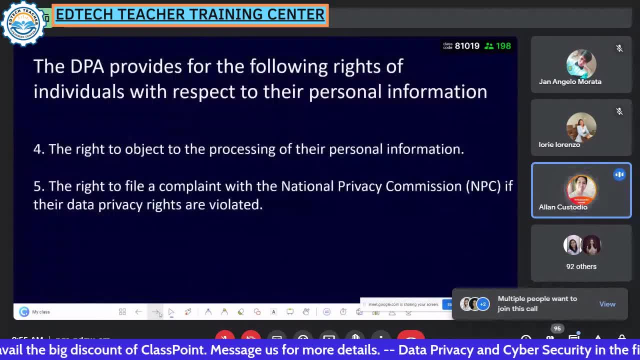 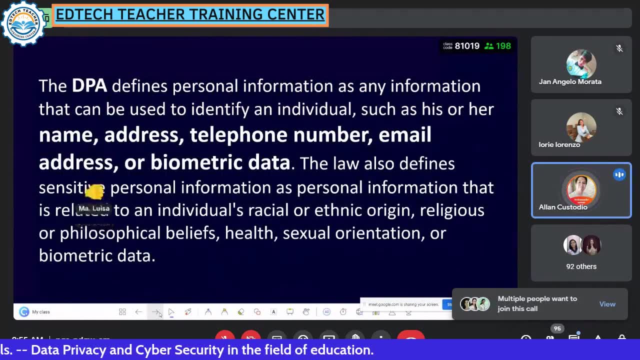 sana mo may natututunan. kaya, kung may natututunan nga po kayo number 9, may number 9 yan no number 9 nga po tayo. sana mo sa ating live number 9, ayun no full po tayo. 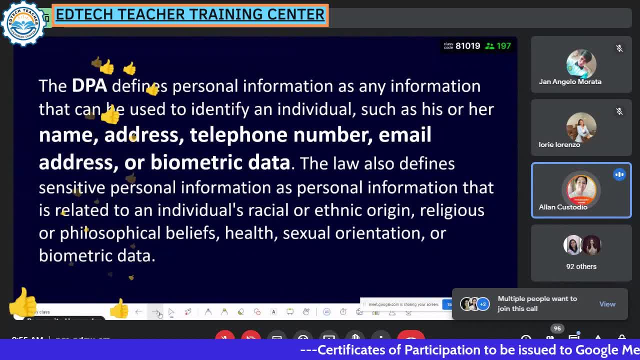 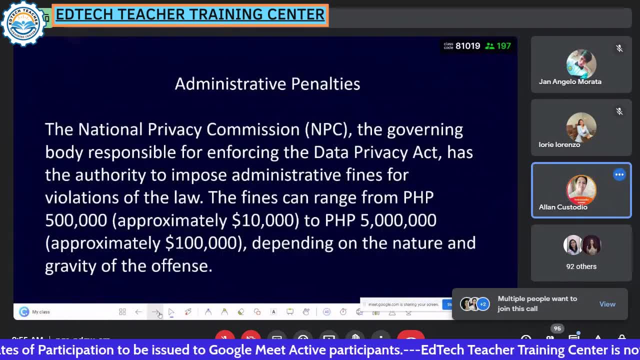 sa ating class point. no, napakadami ng nasa class point natin, o number 9. okay, so sa pagpapatuloy natin. ayan, nililipat ko. eto po administrative penalties. una kong paliwanag sa inyo. 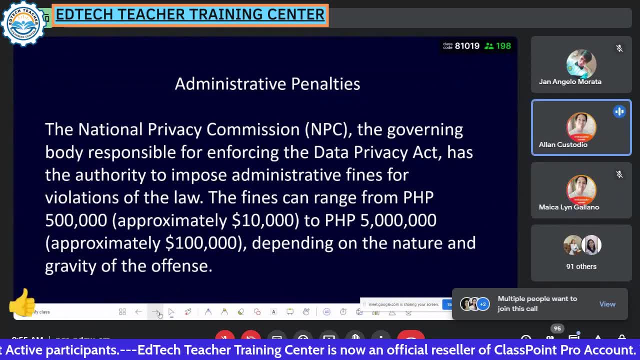 sa data privacy natin. na unahin ko itong mga empleyado kasi kasali to sa education. bakit ko sinama to kasi maraming mga taking for granted. eh, eto, unahin ko kapag ang NPC nakita ka. 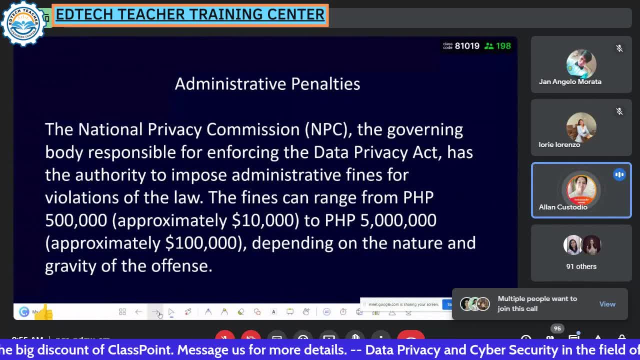 eto governing, eh meron tayong nasasakupan na jurisdiction sa school. tama po ba ground for grievance committee pag may ginawa kang unethical, kahit ano pa yon, pero nasasakupan pa rin yun ni NPC. 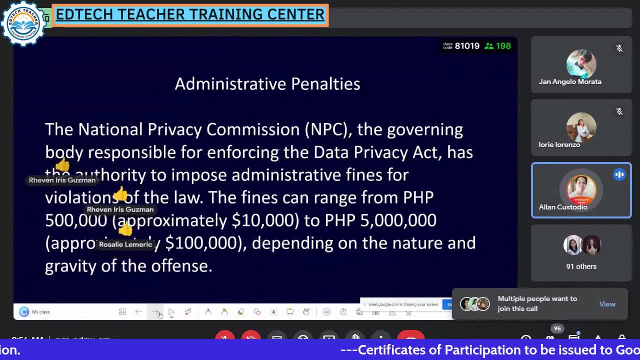 which is pwede ka magpailang administrative case doon, sa mismong website natin, kung may mga kanyayaring, disclosure or breaching or kahit manipulation ng data mo na hindi maganda. now ang fine ay kalahating million. 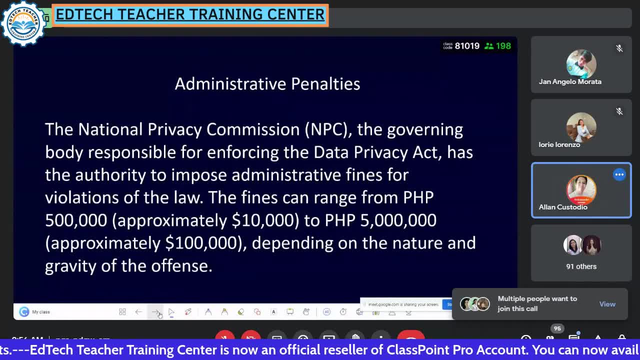 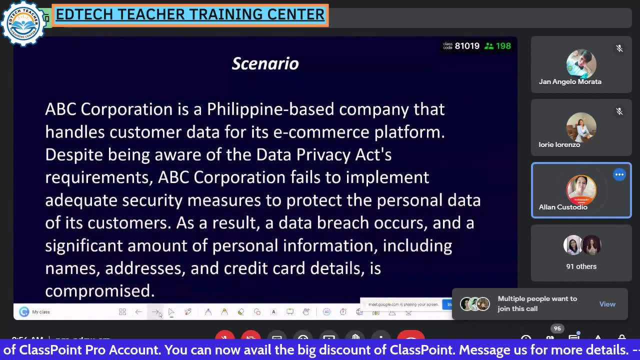 hanggang limang milyon, depende doon sa nature at gravity ng offense. this is the example. now yung ABC corporation daw example. eto example: may private institution na nagahawak ng data at aware naman sila sa data privacy. 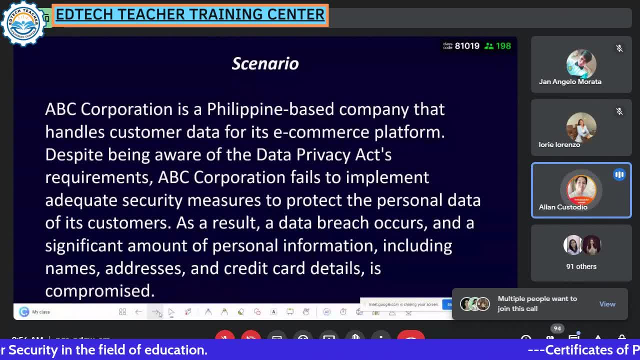 act ngayon yung private school na yun nagpail sila ng implement ng adequate security. etong example na to ay example ng data breaching. eto example nagbigay yung mga bata, kasi alam natin private school. 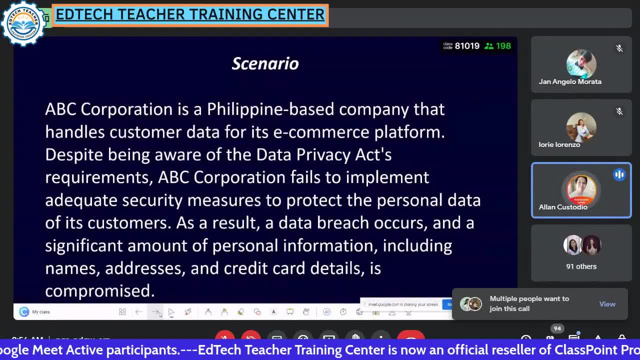 marami ding mga may mapaperang magulang or sabi natin nakaginawa at ang nangyari mahina. yung system nila madaling mapasok yung password. ang ginawang password ay kunwari. 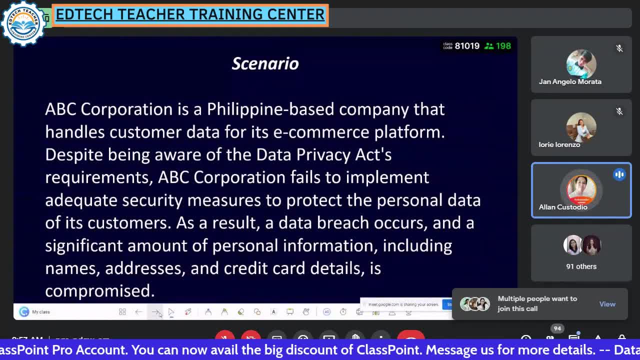 ay pangalan ng school, pangalan ng may-ari at saka favorite number na iba-ibang klase. pero nahulaan at napant out na lahat ng mga na perwisyo ay nakuhanan sa GCAS, nakuhanan lahat. 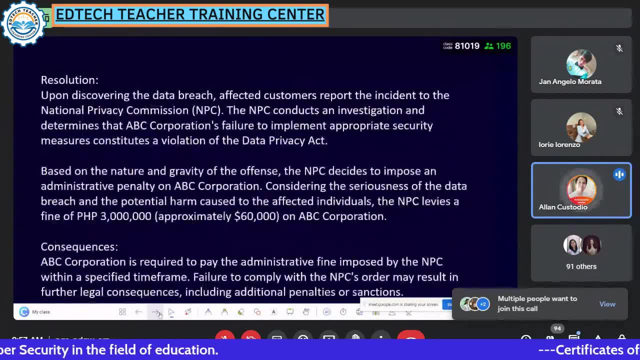 ng mga pensyon. so inimbestigahan, based on the resolution of NPC, na nag-amount siya ng $60,000 or 3 million pesos, dun sa gravity at perwisyo ng nangyari. now para po ito sa mga. 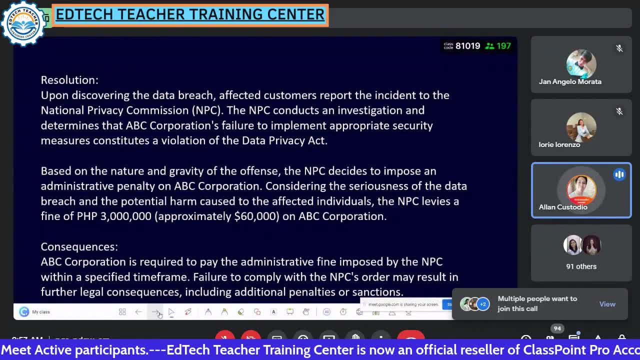 employee government. last time po nagtalk po ako Philippine National Police, kahapon lang po, kahapon lang po ako nagtalk sa Philippine National Police at na inariyan ko po sila dito ayan PNP po ng ating ah Pilipinas. 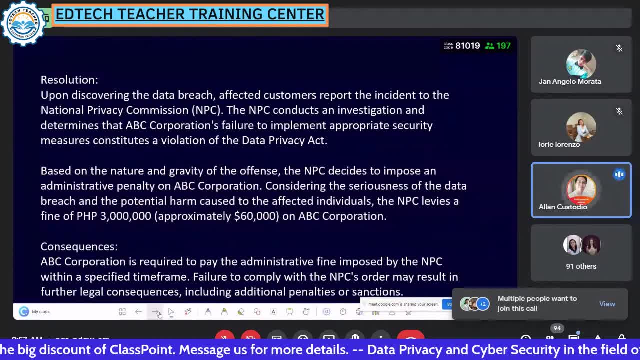 dun po ako nagtalk, yun po ang ating mga naging ah. at ngayon naman po ay kayo, mga teacher at government employee, kahapon lang po, katatapos lang po PNP, po ngayon nagpe-pay sila dun. 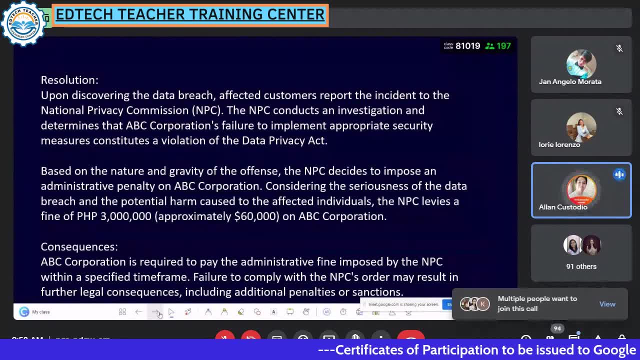 ng fine yung admin dun at depende yung sa tao na yun kung sino ang protection or may hawak ng page. kaya hindi po basta-basta humahawak ng page kung hindi natin masyadong kabisado. 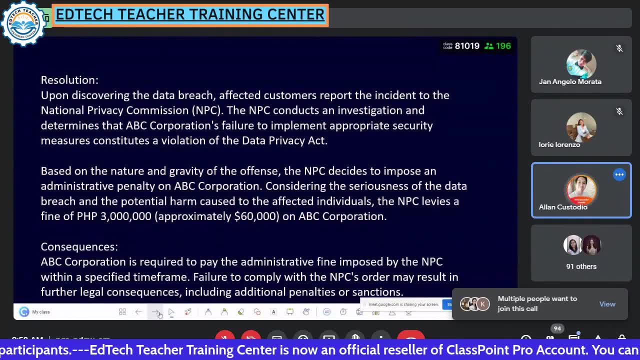 kaya, kung hindi tayo masyadong maalam, magtapat agad tayo, huwag tayo agad yung misan, kasi may nagmamagaling na alam mo naman, pero mas maganda kasi. 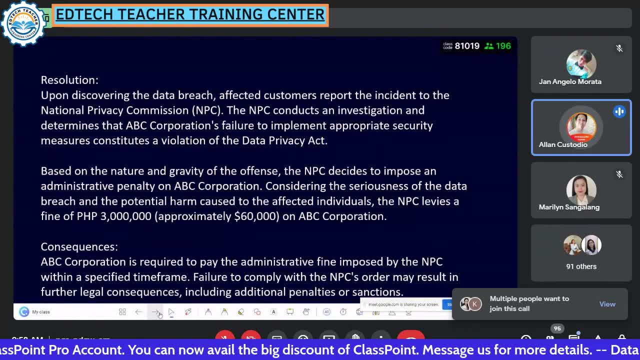 magsabi sa sarili mo na hindi ka pa tapat doon sa bagay na yun para matulungan ka ng management ng school or something institution. ay kailangan nila mag-fine, tapos ayusin nila sa time frame. 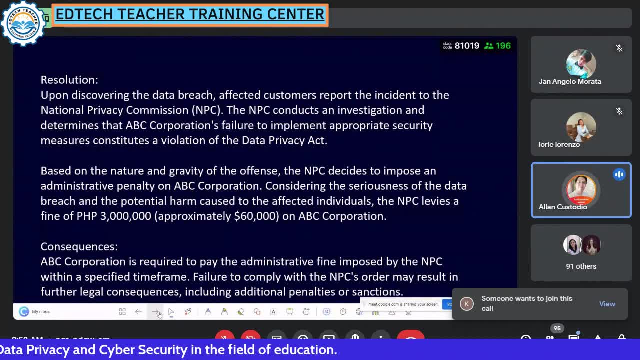 ganito yan magme-maintenance habang inaayos yung system para sa pagbabalik. wala nang ma-perwisyo, kasi, hanggat hindi kina-close ang system, patuloy ang data breach. ang hacker ay laging andon. 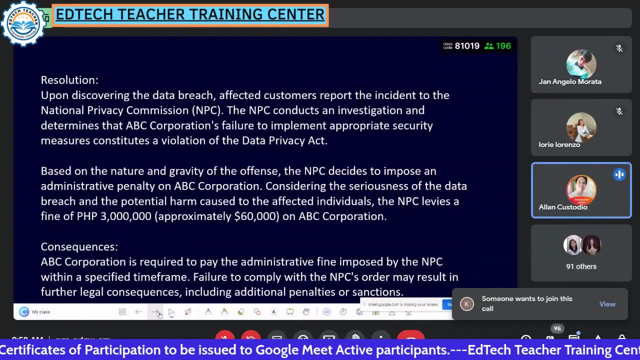 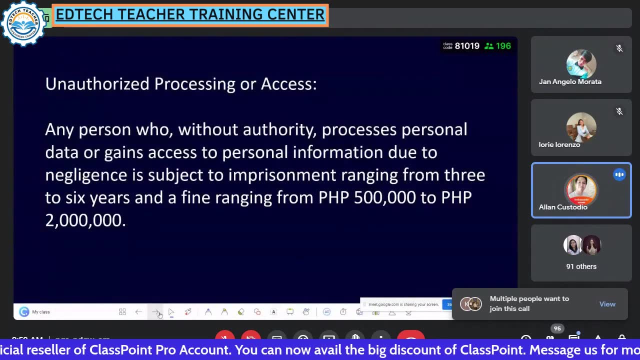 so i-down yung system or i-delete yung system. gagawa ng panibago, ng strong yan yung gagawin ng private institution, or yung dito example ay ABC Corporation. okay, now, eto, eto, marami eto. unauthorized process. 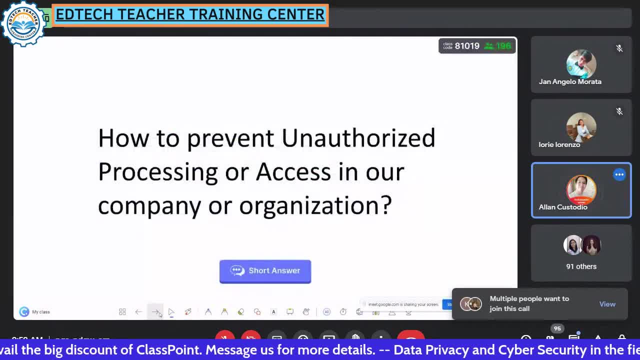 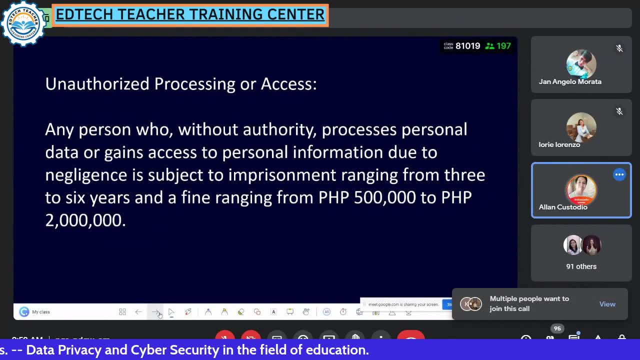 and access okay, pero bakit ba naman nauna yun etong unauthorized ay magli-lead ng kalahating milyon hanggang dalawang milyon at pwede kang makulong ng six years, depende sa perwisyo mo. 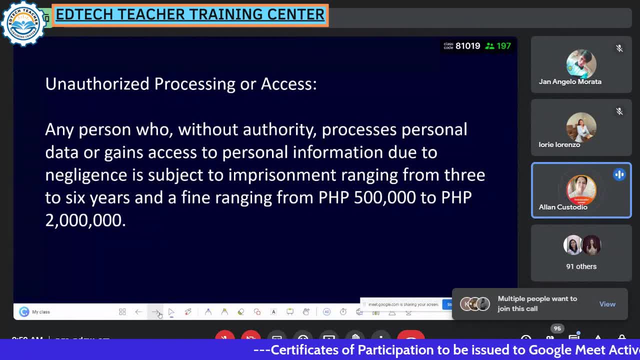 unauthorized process. ang unauthorized process: po pumasok ka sa isang room ng admin kunyari kinuha mo yung mga files doon. walang tao, kunyari isa kang teacher gusto mong kunin lang at meron kang data doon. 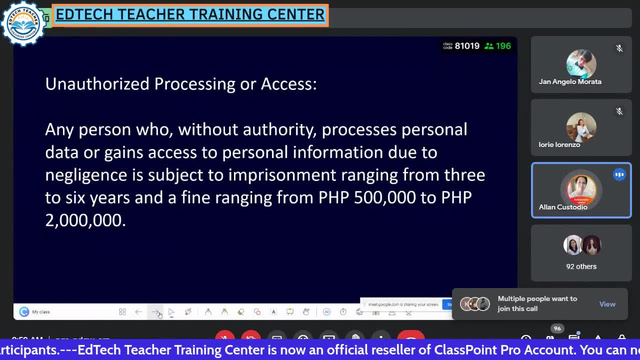 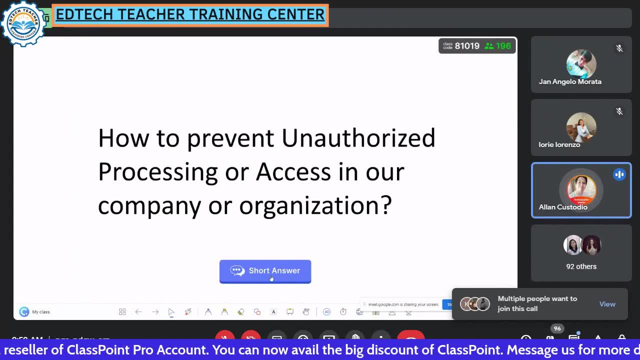 kasi may mayaman na estudyante may gusto kang gawin, may makaibigan kang hacker, or kaya meron kang gustong um mangyari. kunwari lang po paano natin malilimitahan yun. sige, sagot nga po tayo. 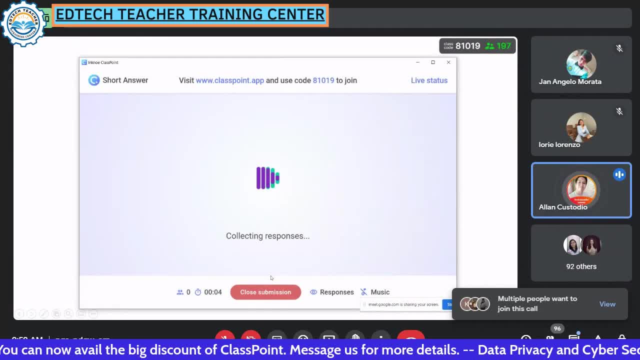 yung mga pagpasok na yan ng mga kakaibat, pupunta na lang bigla sa desk mo at may kukunin unauthorized po kasi yun. eh, ang tanging authorized lang doon, kapag nag-o-orient tayo, ay yung mga admin. 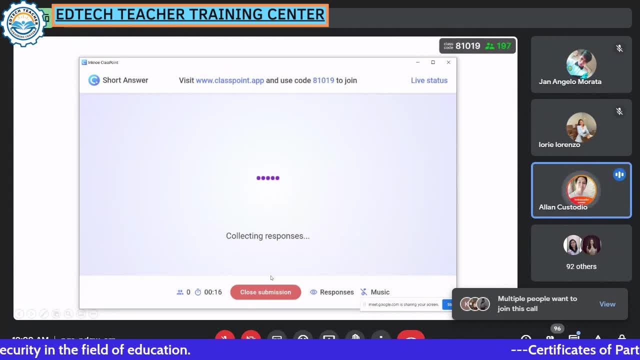 alam naman natin: AO1, AO2, admin officer 1, admin officer 2: sila yung may hawak ng mga files, and pwede rin yung DPO data protection officer. si si sila, mam nga halos hindi gumagalaw doon. 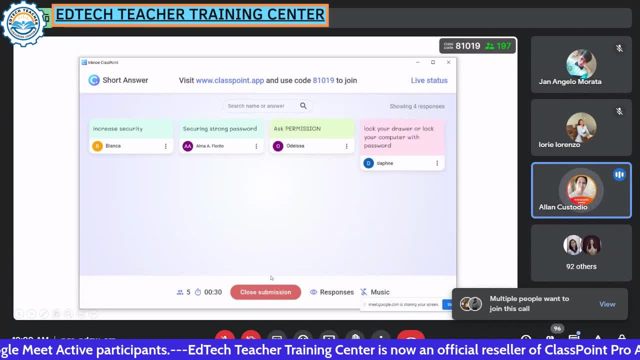 yung principal diba, kasi ang may hawak doon ay mga admin, o tinatawag nating AO, sa school. ngayon, paano natin malilimitahan yung pasok mang pasok, bigla na lang magkiklik sa computer? 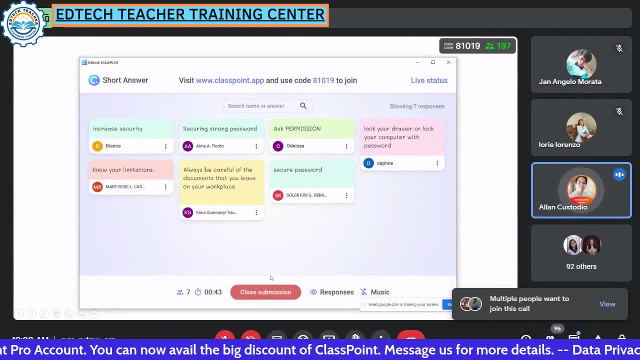 ni admin AO tapos biglang may kukunin na files nung bata. tama ba yun? tama po ba yung ganon? o sa ibang school na napagtrabahuhan ko po meron silang off limit? alam nyo po ba? 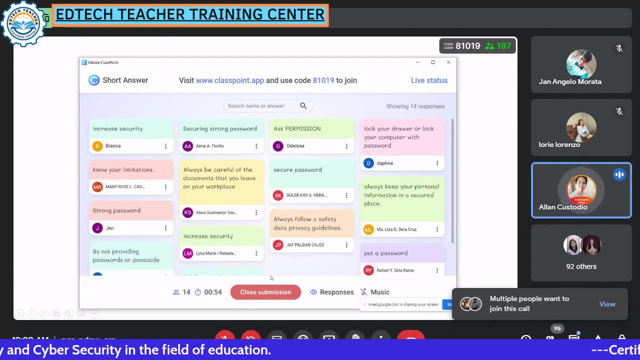 yung off limit, yung parang may kahoy din, tapos nagbebel yung mga admin sa gilid, parang maliit na bel na kulay silver, kasi off limit na sila, lumalag pa sila doon. 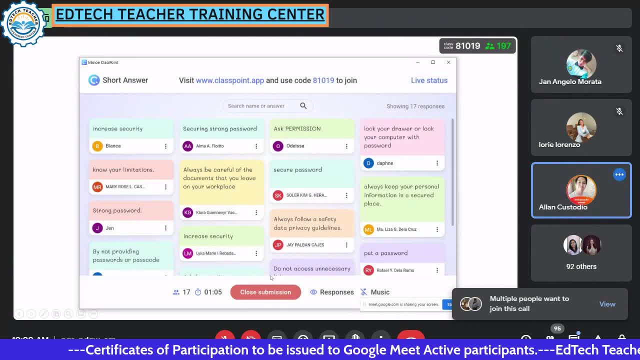 yung parang dudungaw na sila sa computer. bawal po yun, kaya minsan nagbebel sila na ganon ibig sabihin lumayo ng konti. ganyan yung tamang proseso ng mga admin. 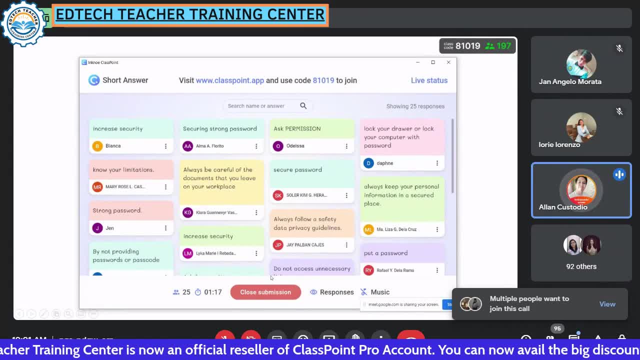 kaso kasi yung iba, dahil friend mo na baby mo. sige, tingin ka sa computer password natin ganito: ayayay, mali po yun. mali yun lalo na na bypass mo yung principal doon at saka. 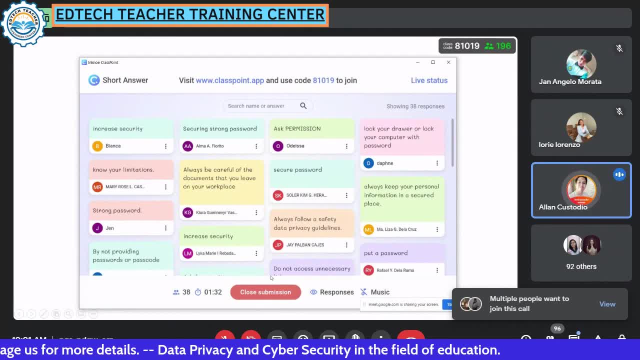 yung ibang mga bagay pa kasi yun ay pinagpapaalam. hindi mo naman kasi gagamitin yun. sabi natin: gagamitin mo sa personal mo, pero yung kukuhanan mo ba doon. 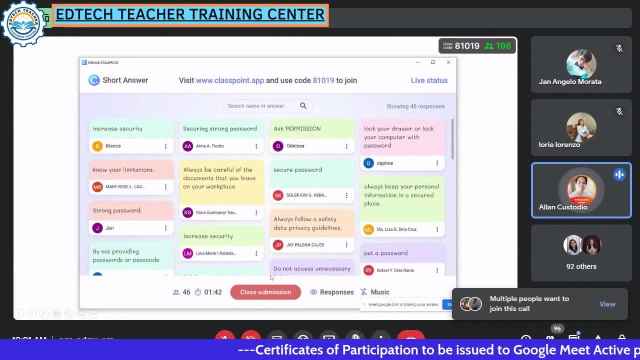 ay gusto ba niyang kunin yung information nya? syempre hindi, so wag tayong mag taking for granted na naman ngayon ang daming sa magot dito. let me read some sa sagot: secure password correct. pwede tayong? 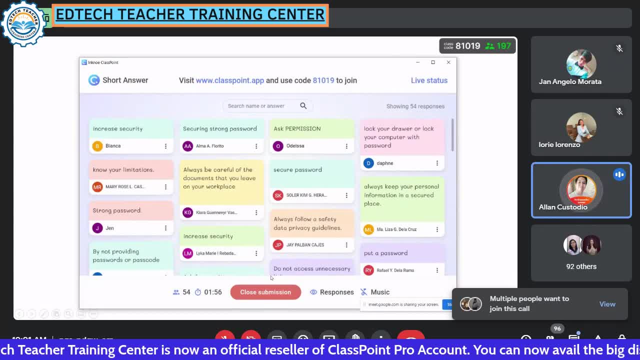 mag double password or mag encrypt, yung tinatawag na encrypt- lalagyan mo ng password, yung word lalagyan mo ng password, yung example nakalusot sya sa una password doon sa laptop e yung nilagyan mo. 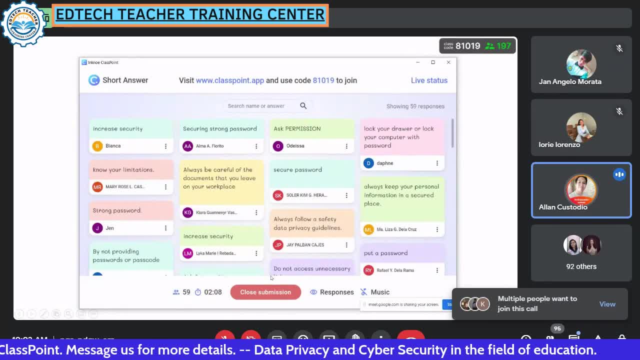 ng encryption, nilagyan mo ng password yung excel o diba hindi sya makakapasok, kasi naka encrypt ngayon. always keep your personal information secured in place. correct, pwede din yan? o lagyan natin ng encryption or password. 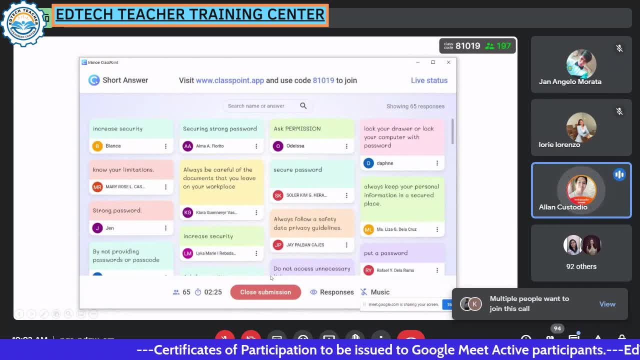 increase security sa increase ng security, yung iba kasi bumibili pa talaga ng system. e ibig sabihin, kapag may gumagalaw doon, mag nonotice kay boss, mag nonotice sayo kung sinong may hawak. 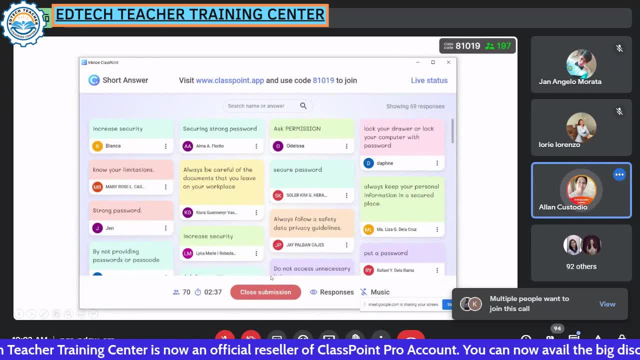 nung files na yon. ibig sabihin nag nonotice, someone is having control with your document, may mga ganun po e may nakita akong system na ganun, yung iba bumibili pa yung kompanya, para lang talaga. 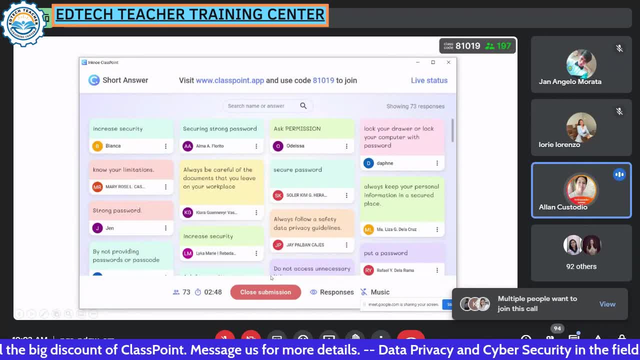 walang data breach, kasi tatamaan sila ng file na hanggang limang milyon. ano yun matindi yun ngayon babaat pa tayo. okay ngayon. detect response to the instruction quickly, Jessica, correct, ma'am no. 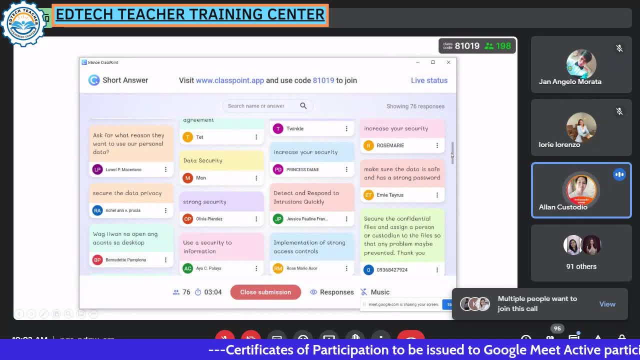 mas mabilis kapag may mga problema na ayusin na yung system that is correct and strong security. wag iwanang open ng account sa desktop. ma'am Bernadette, gusto kayo sagot na niyan, because wag ka mag taking for granted. 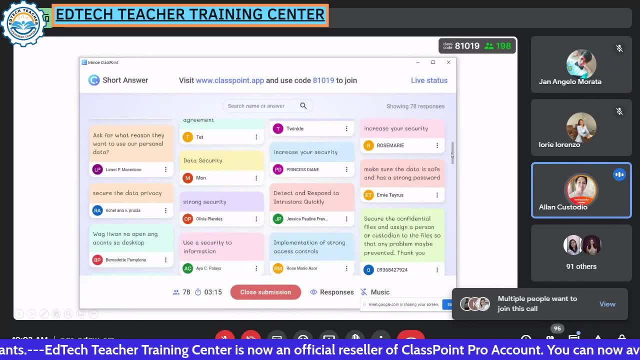 nag CR ka, nag kapi ka sa labas, saglit bukas yung files mo e meron doong isa na halos ka office mo o nakita, tapos sakto pala may yung hinahanap yung data, pinatimingan ka niya. 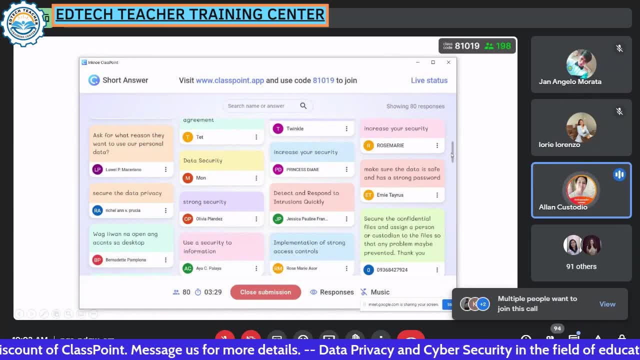 pinikturan niya and ayun pinahack niya. so nung nahack naghati sila, nung nagbabayad nung hack, alam nyo the possibilities or the the scenario yung tayo magpaka taking for granted. 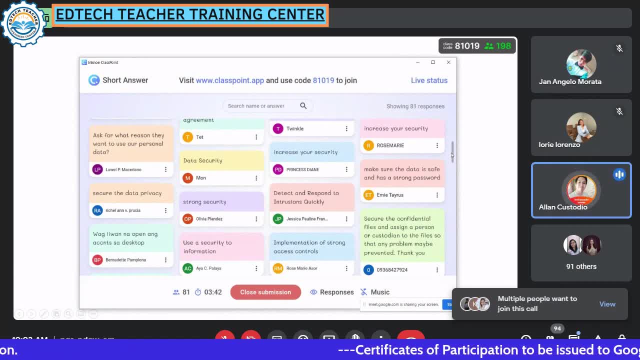 trabaho lang. so i-keep natin ng maayos at walang magiging problema. hindi masamang gawin ang dapat mong gawin, at hindi rin naman masama na pagbawalan mo ang mga bagay or mga close mong. 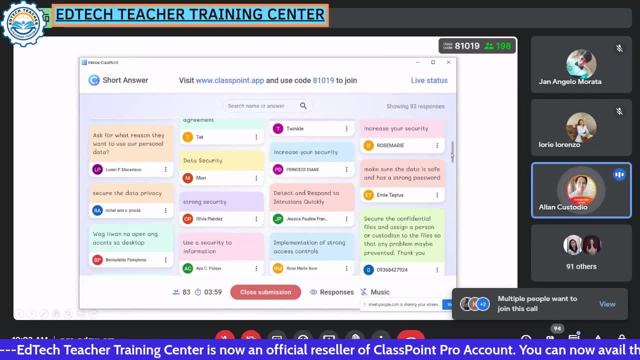 tao na hindi dapat nila gawin ang pagpapakita ng mataas na pagsunod sa yung ginampanan dyan masusubukan kung gaano ka ka-professional, kung paano mong tutupad din. 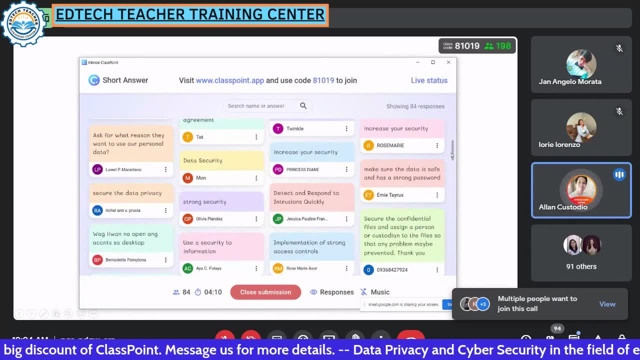 ng mabuti ang gawain mo. dyan mo mapapatunayan kung isa ka talagang professional at ang kaibigan ay magkaiba sa trabaho, kaya may kasabihang trabaho lang, walang personalan, okay. 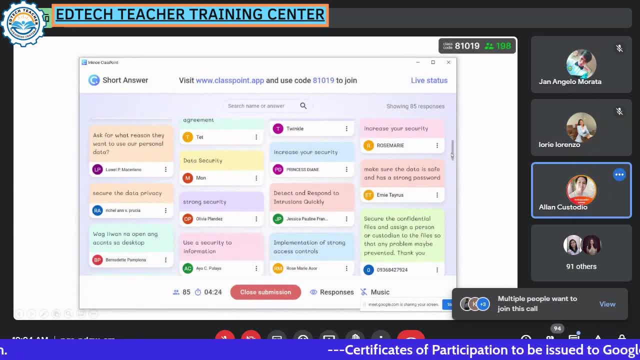 naniniwala, po ba kayo number 9, number 9, number 9, sige nga po number 9 ayan. o shout out: ma'am Dela Peña ayan trabaho lang, walang personalan, kasi need natin talaga. 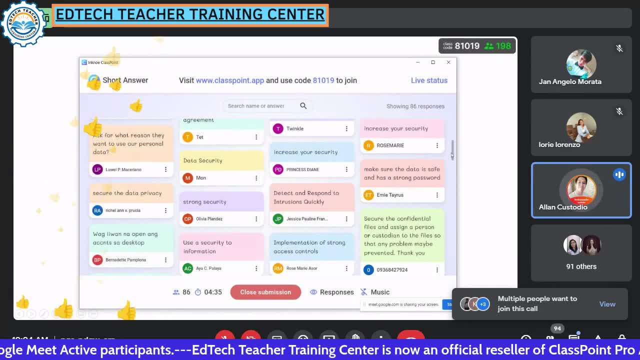 ng maayos na trabaho, especially sa government. ang client natin ay public people halos sa totoo lang po, ah real talk na din. usually yung yung mga cliente natin halos wala alam sa data privacy. eh, tapos tayong may alam. 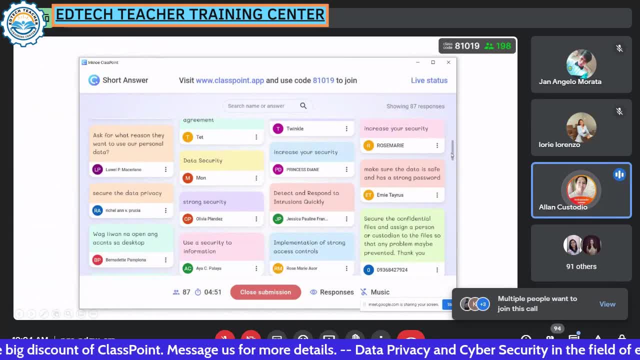 magkakaroon ng unauthorized disclosure, papamigay na lang natin abay, hindi naman nasasabang. kapat naman sa kanila. yun, tayo ang poprotecta sa kanila at hindi maghaharm, tama po ba? 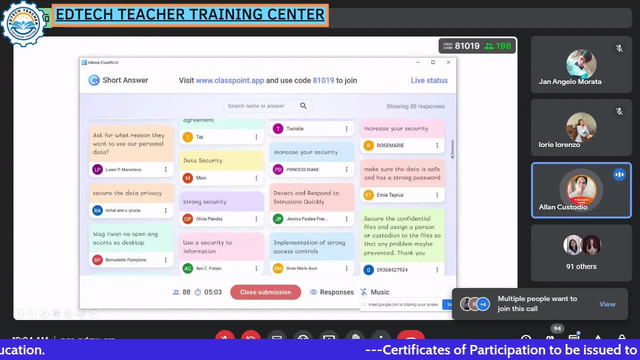 mga government employee, lalo na dito, kung may mga estudyante dito na magiging government employee din or private na employee. tayo kasi poprotect sa kanila, hindi tayo maghaharm. ayan, no, napakaganda ng usapan natin. 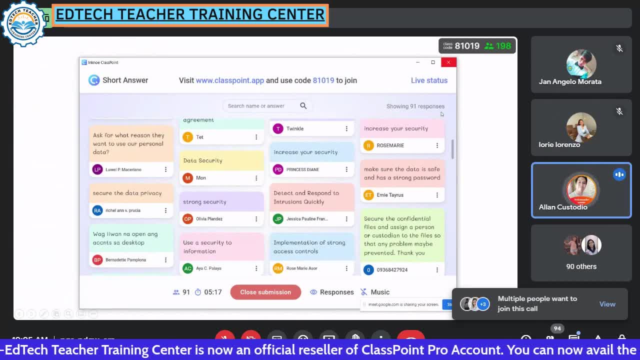 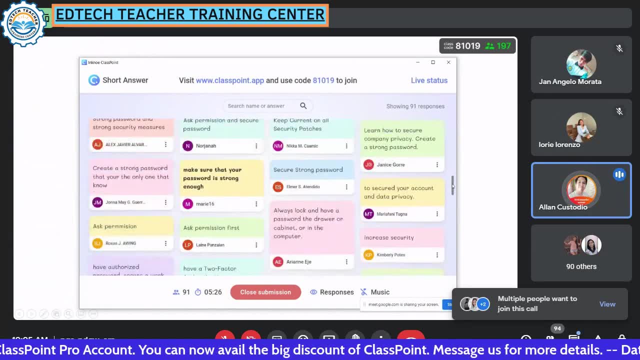 napakaganda ngayon. i-close ko po yan. ah, i-baba natin konti para makita nyo mga sagot nyo ayan, o makikita po sa live yan ayan yung mga sagot nyo. tama po lahat yan. 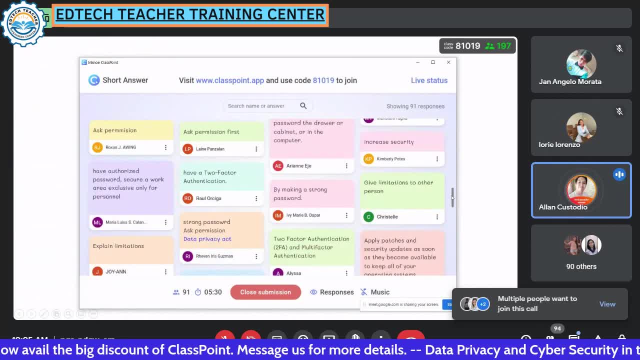 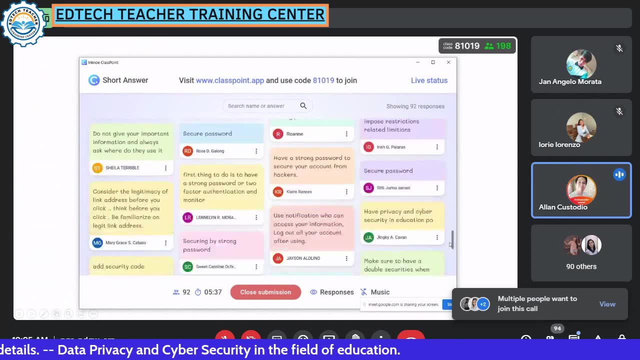 mam kimberley, mam lane, mam roxanne, mam ivy, mam christelle, mam queenie, ah mam jem ayan. ah, sir joban, okay, mam rose ayan, lahat po yan no nakikita natin hanggang baba po no, so close natin. 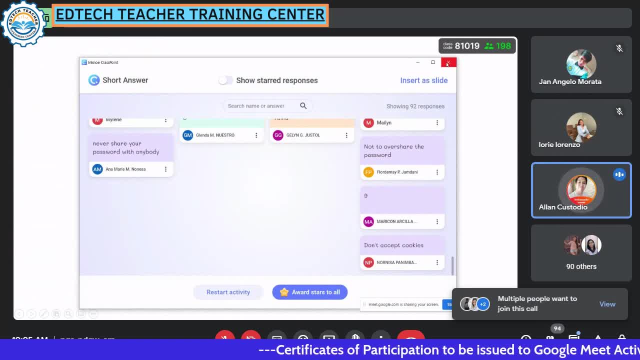 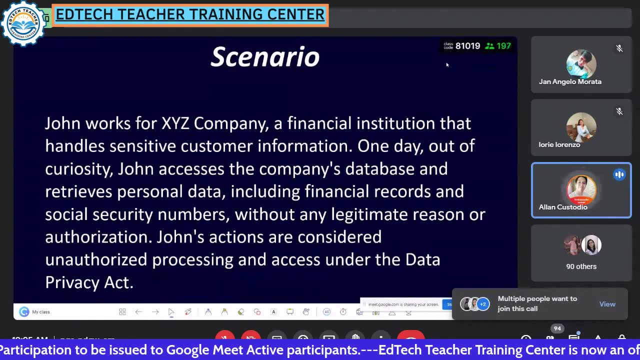 and ayan, ayan na. so nakikita nyo na po yung mga ilang batas. ten five, another example sa organization daw. example: sige, iyan na natin sa school muna, dahil edukasyon, si jan daw ay nagsatrabaho sa isang private school. 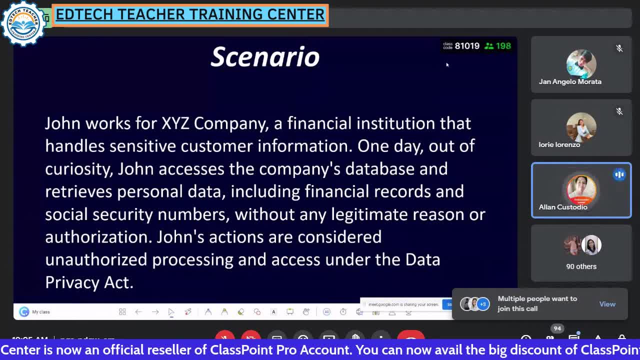 xyz company. one day na curious si jan at nag access siya ng database at ngayon na retrieve niya yung mga financial record example, nakita niya lahat nung mga hindi dapat buksan utang, nung mga mga ano niya. 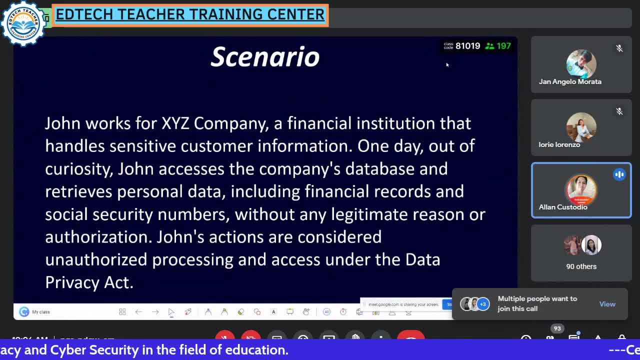 ah, kako teacher niya. nakita niya na may mga teacher na walang utang, so nakita din yan na parang yung na ngayon ay wala ding alam at parang madaling lang lokohin, kung sakaling magpapanggap siya. 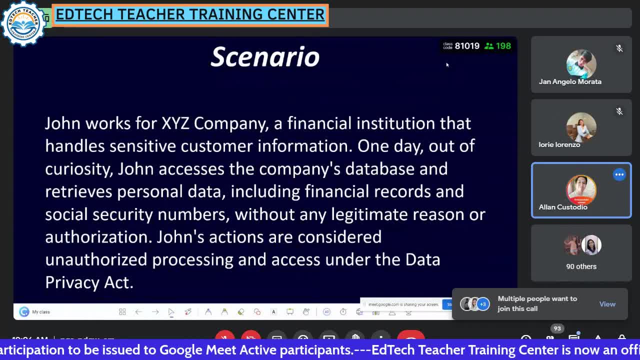 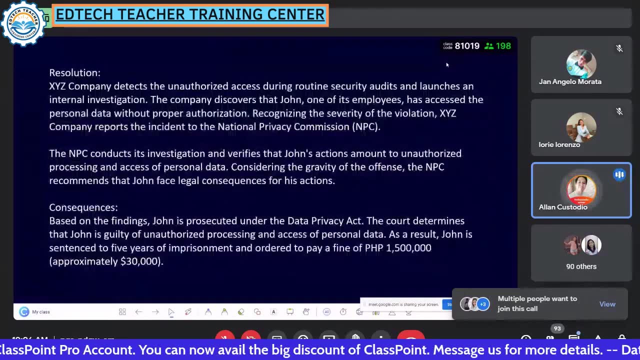 ngayon ang tawag doon unautorized disclosure, when we say unauthorized, walang autoridad na sa kanya ay kumuha ng ganun informasyon sa database, sa resolution ng NPC, ang nangyari na na verify, na nagpo-proseso si jan. 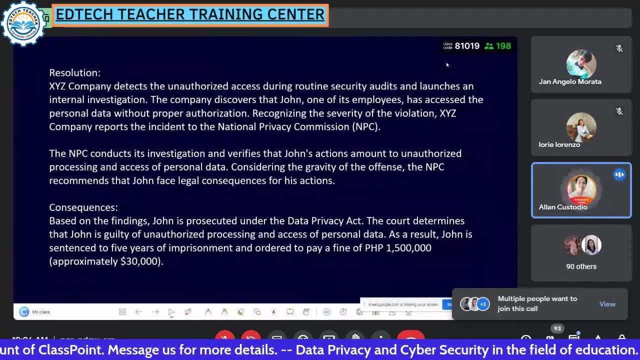 ng personal data at under ng personal data. personal data, I'm telling you, is the sensitive and others. Now he is guilty and he fined the severity of $1.5 million to $30,000 because he also got a lot of permission and he was sentenced for five years. 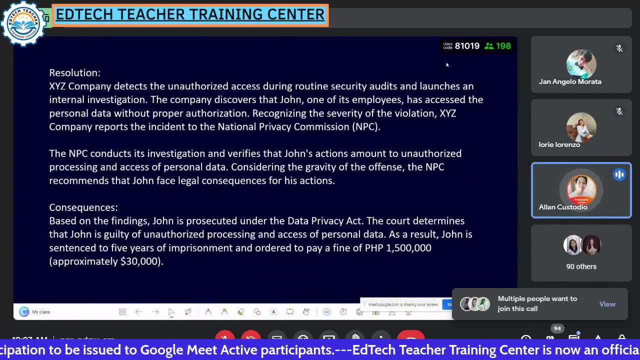 Because that is not allowed, especially if you don't have the power. Who here has experienced this? A teacher suddenly goes and prints something and suddenly says: Hey friend, I printed this because you know that we are friends and you know that there are data there. 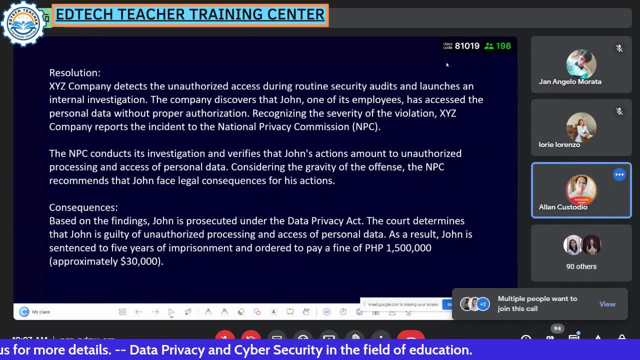 So always remember this: If we really have respect for each other, say goodbye, Friend, can I print this for you? Don't suddenly say goodbye, or even if you really need to, Okay, Because we need to have proper accounting and proper responsibility for things. 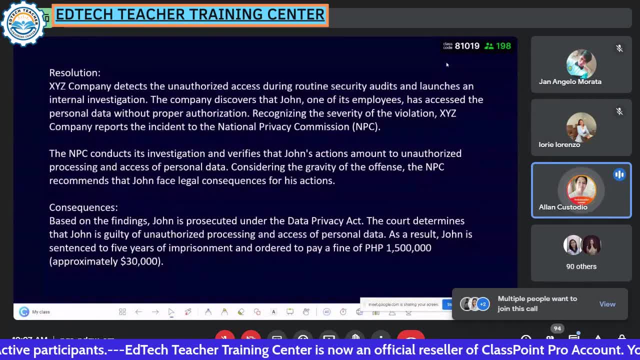 Like this. This is not allowed. This is not going to be allowed. Why is he going to get a financial record? Because it is not going to be allowed. That's why what happened was really intentional. Intentional is what happened to Jan. 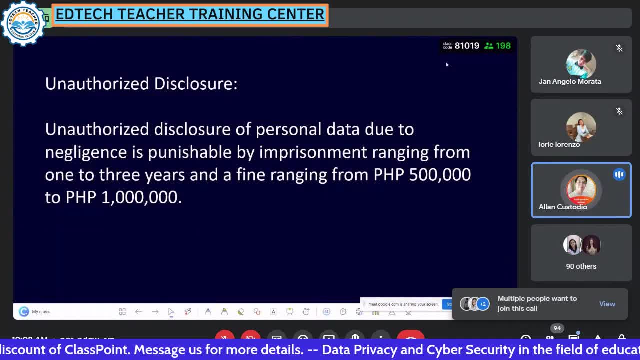 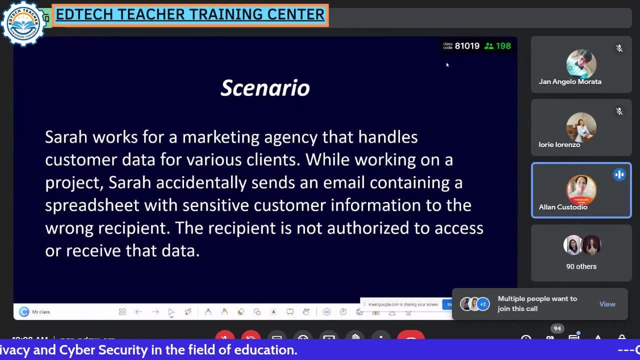 Now, in the unauthorized disclosure- this earlier too- $500,000 to $1 million. we have an example: Sara is working in an agency, a marketing agency. I know there are other agencies here, but let's just say it. 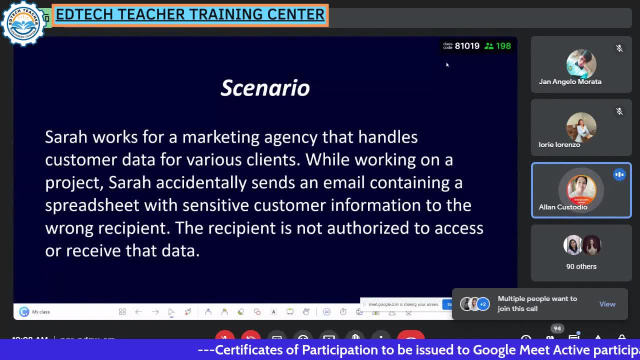 Marketing agency of education or private school. She handles customer data, various clients, Different of course. Now Sara accidentally emailed someone else, But she shouldn't have access to that Now because she doesn't want to be exposed, And unintentionally. she is also not malicious. 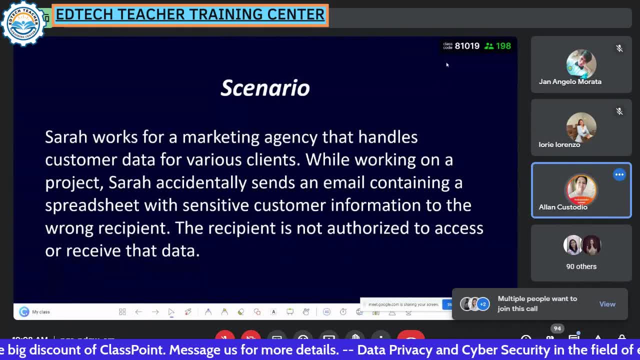 Maybe it happened that she shouldn't be there. But she just wants to send that information to the right person. But she shouldn't be there. She already has a case. She wants to do it. It's a karma. For example, she was sent to another person. 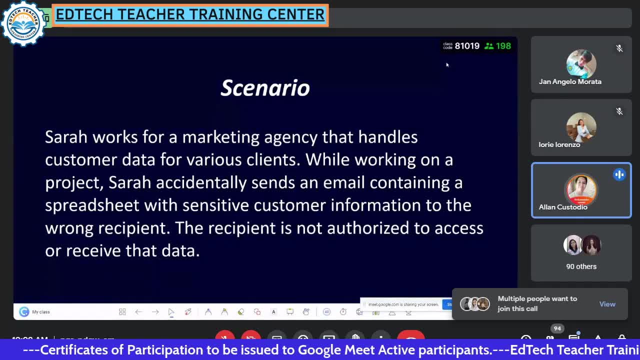 But she doesn't really want to be sent there. Maybe she just wants to be sent to her boss or to someone higher up Because there is an urgent report But she doesn't really want to open it, Or there are other people. She was forced to do it because the report is urgent. 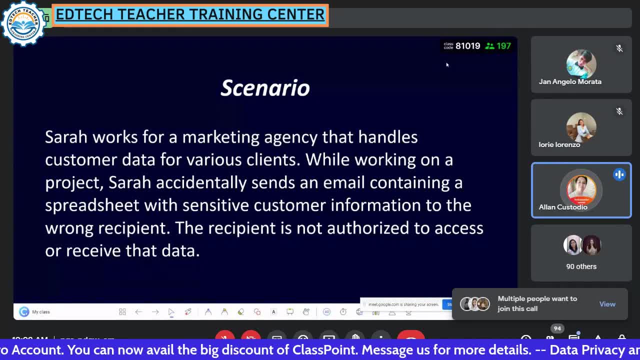 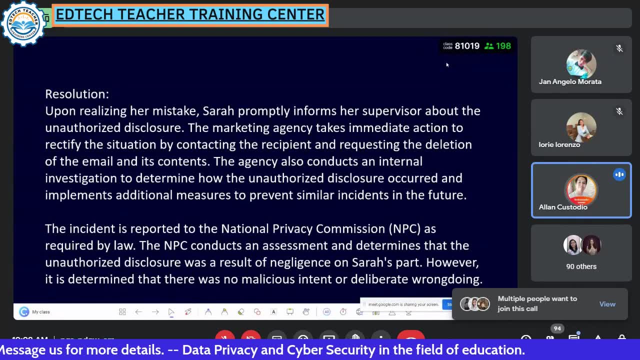 So she opened it. She accidentally gave it to another person. Now the one who complained was the one who got permission And Sara was the one who complained. Now the incident- Sara- was reported. She was also banned out. Many were hacked. 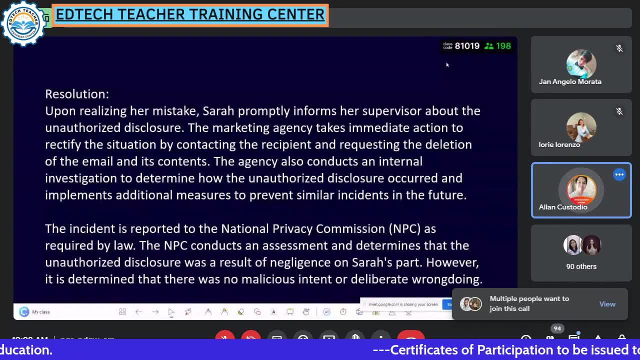 The pensions, The OTPs of GCAS, The ones that are no longer there. The parents were targeted. The one who was sent there was a hacker. Now in the assessment of the NPC, However, there is nothing malicious that Sara really gave. 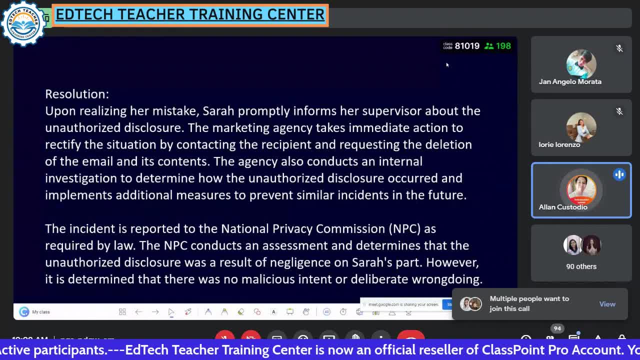 It happened that she was able to get permission from someone who sent it And when she received an email, the person's name was omitted from another letter that she sent. Now she will be fined P750,000.. It depends on her. 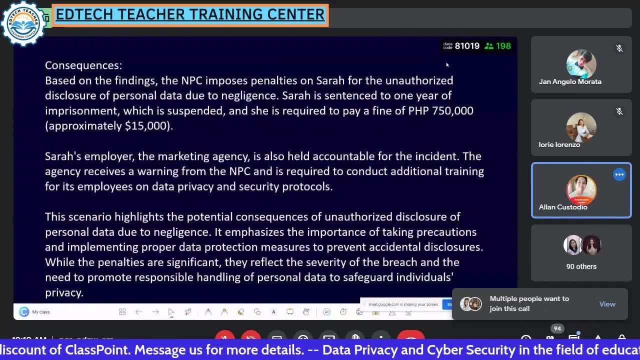 And she will be in jail for a year And it depends on her if she will be removed from the company because there is a jurisdiction, Because it is unethical. Now, this scenario highlights that it is unauthorized because it cannot be given to others. 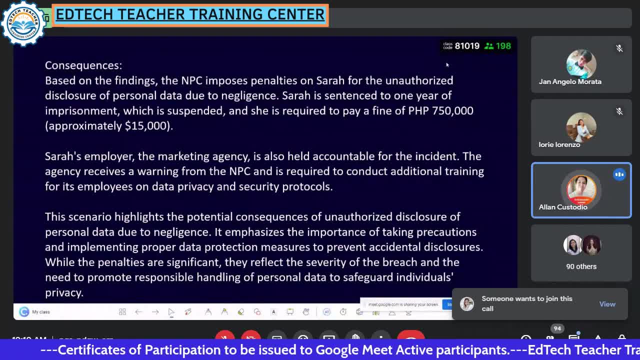 And there is also a negligence, The company, Because suddenly there are people who can get it and can access the information. Imagine this: There are many cases. So the school, They let it go, Or anyone can get the data. 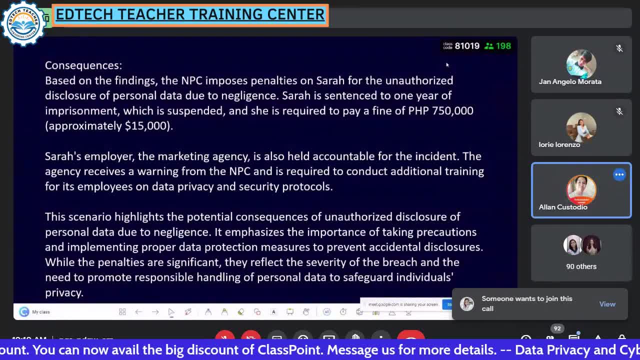 So there is also a negligence on the part of the admin. Now Sara also has negligence, Even though it is urgent. Why is she not saying goodbye? Or she doesn't have consent, Or she doesn't have authority. because of that, 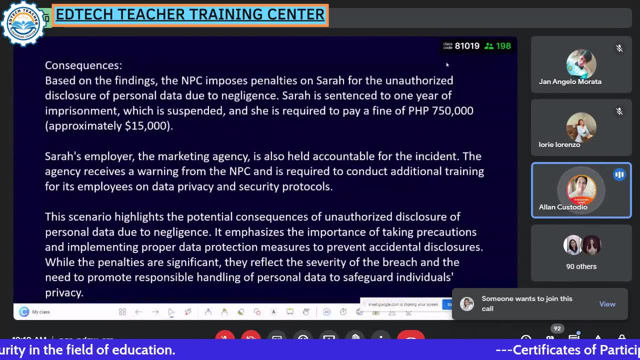 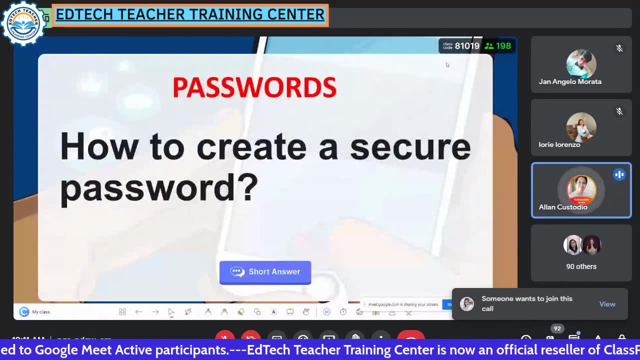 Or even if she doesn't have malicious content Not intended to harm any other, There was harm because she was sent to another person. She was killed. It became $750,000 and $15,000.. Now how can we create a secured password? 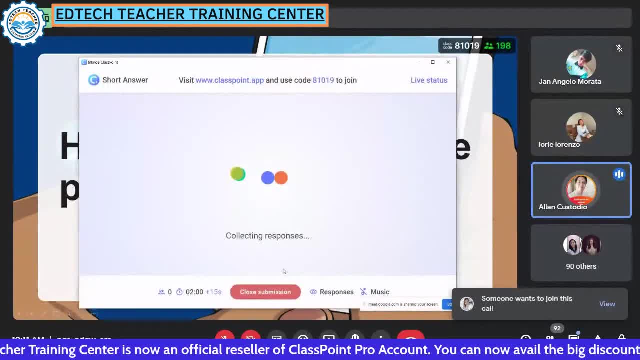 Let's go to education first. Our samples are also education Practical example. Okay, How can we create a secured password? Let's go to this first, So that we don't see that my laptop and my desktop are always being opened. What is the correct password? 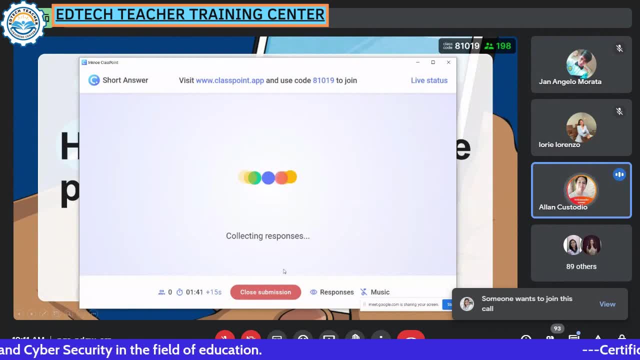 What is the correct password? Okay, Let's look at the answers. We are full in our class, point right There. It looks like we are having a hard time listening. Okay, So it says: use some number and character. 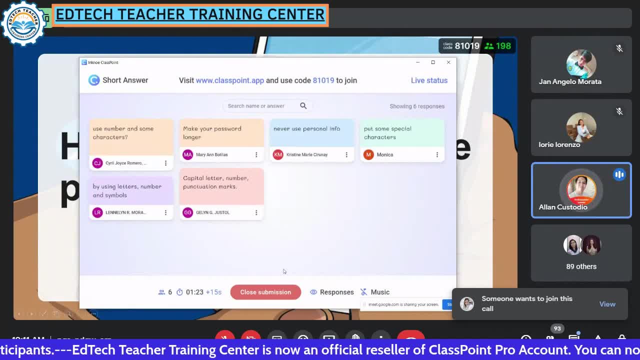 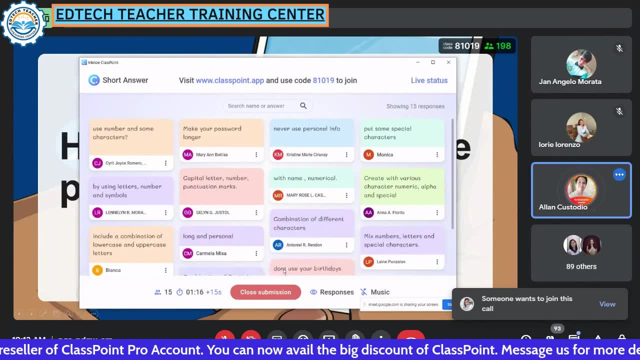 Correct? I want to hear the answer of Ms Cyril. If you use number and text, it is weak. It is weak. If you use the so-called character, it will be strong. Now, it will be strong if there are uppercase and lowercase. 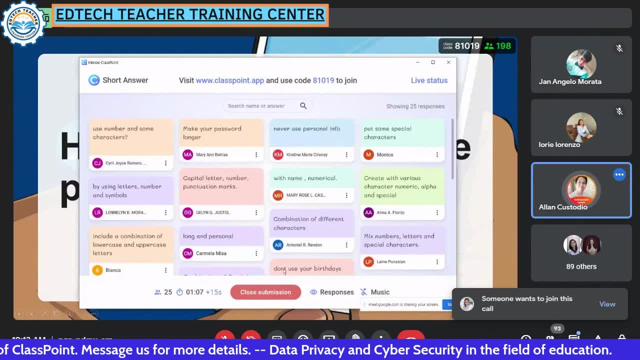 That's it. There are so-called characters that she can't think of. that you can put, Because the meaning of characters is at hashtag, but if there is a different character- But take note- you may not be able to type that character on the keyboard. 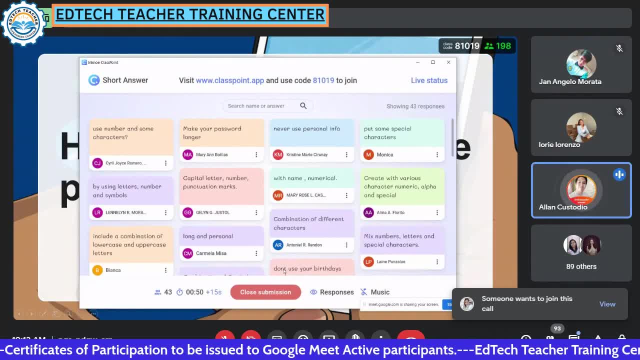 It is also difficult. So always remember that you can type and you can put the password. Okay, Capital letter, number, punctuation mark. That is correct. Combination of different character: Correct. Let's lower the answers in the class point. We are full. 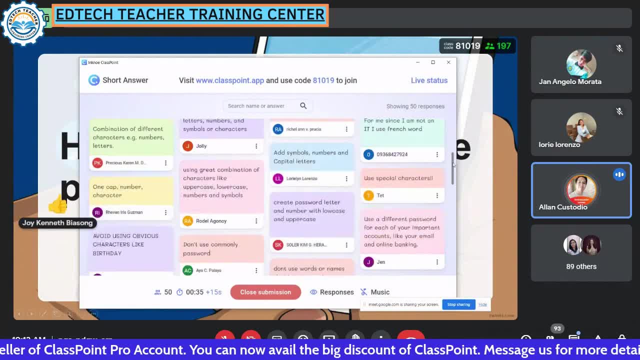 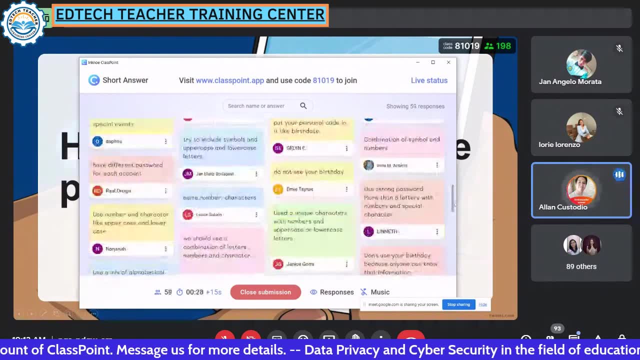 There are so many here, So we can see that it is really a combination. When we say combination, when you combine all the passwords, that is the strongest. So I have a friend who has worked in a company before- In what? 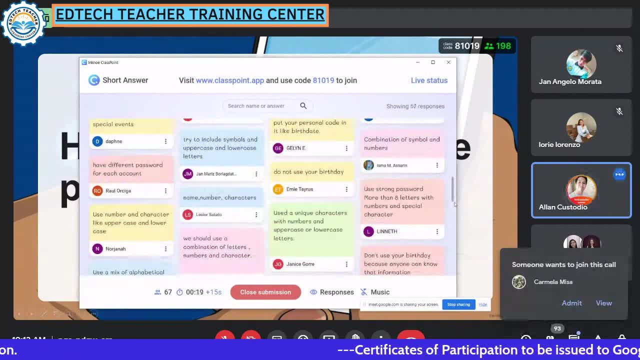 In other companies In other countries And she is a classmate. She graduated from IT And all of these are correct. I will just lower it And let me share what she said to me. She is a cyber security team. That is correct. 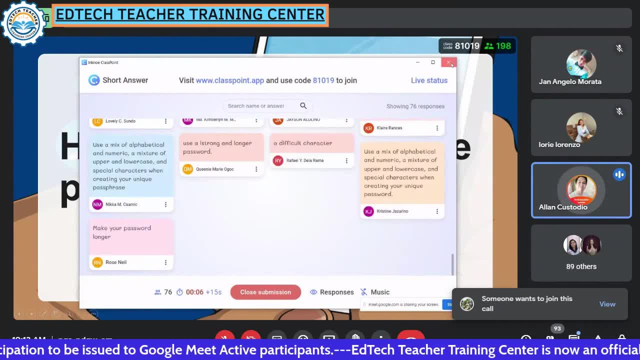 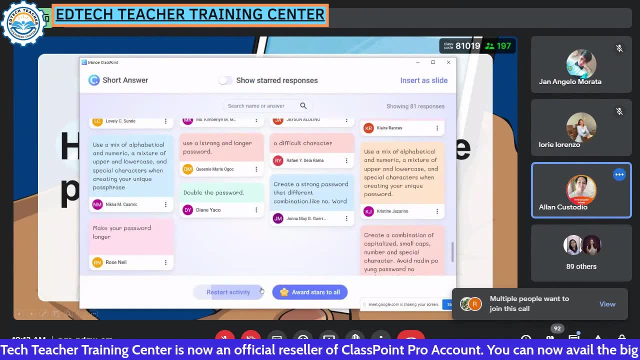 All of what you said here And this is what she shared to me. Now award all star because you are very active, Thank you. Thank you, Who will we share later? Okay, Okay, Okay, Okay, Okay, Okay. 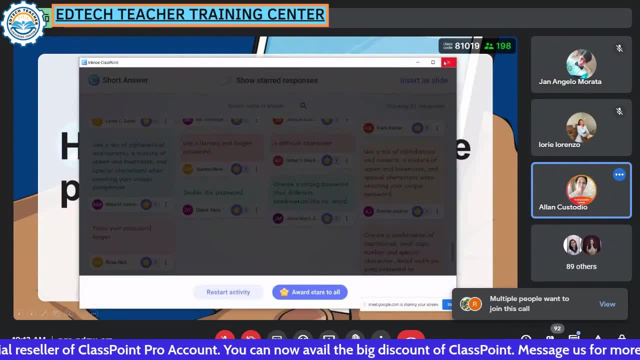 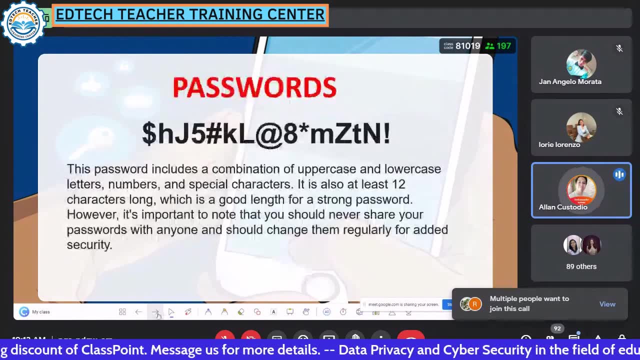 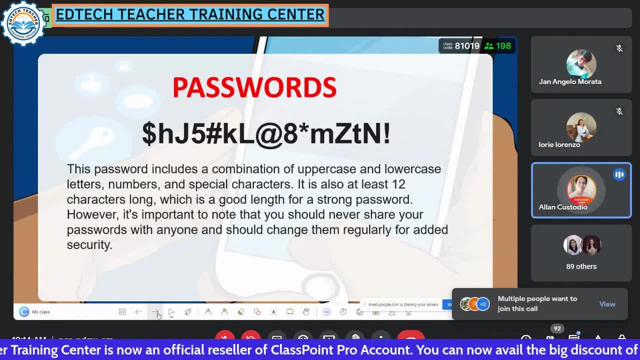 ay tatlong taon daw nung team nila bago ma-hack, Depende pa din kung sa pattern or like that. Kasi ang iniisip nung hacker ay: iisip ka nang hindi mo maiisip na magiging password. 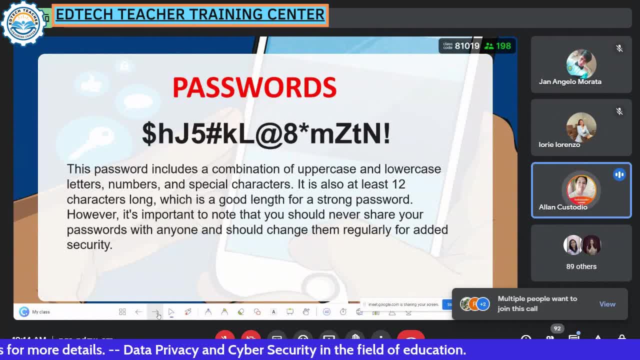 Ngayon, pag pinasok nila sa system yan, meron daw silang nakukuhang clue na mga ilang number at letter. Gina-jumble nila yun at may application silang auto-generated. Pag nilagay nila yung password mo daw, 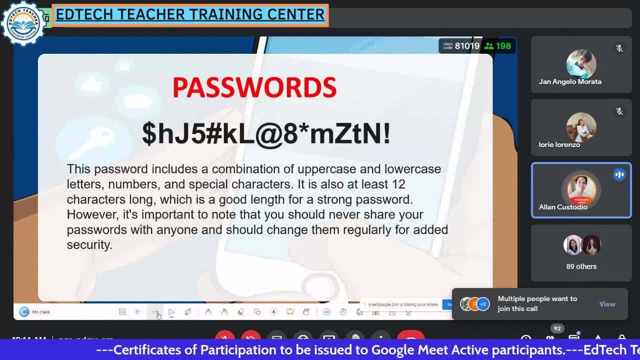 ito sinare sa akin na ng cyber security ko nung nahuli nila in interview ay automatic inilalagin nung application doon yung password. Ang ibig sabihin may application silang naglalagay doon. 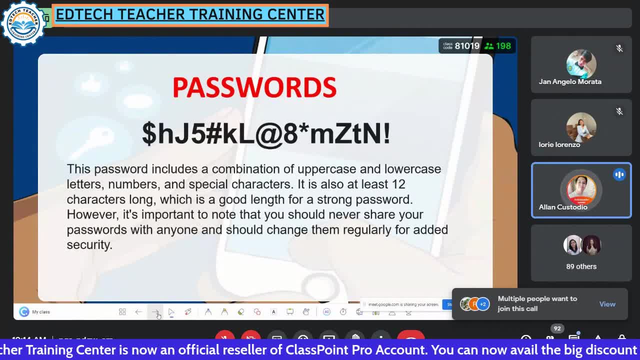 wrong password. wrong password laging. may naglalagay na gano'n Imaginin kung sa loto yun, kung ilang beses kang tatama sa probability, sino po bang math major dito may application silang gano'n lang gano'n. 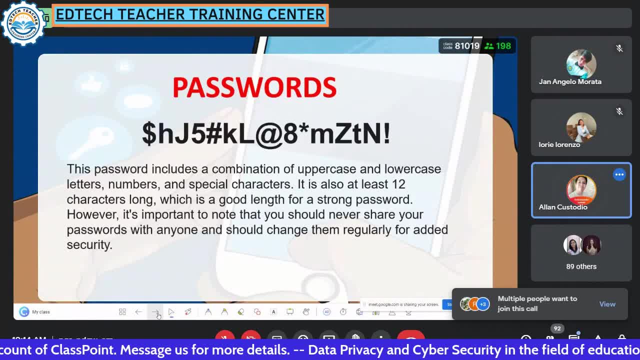 So kapag ganyan daw katindi ang password mo, tatlong taon nilang ma-figure out. Pero dahil may clay password mo, pangalan at saka favorite, ano mo daw, pag gano'n lang, eh, minuto lang daw ma-hack na yung Facebook mo. 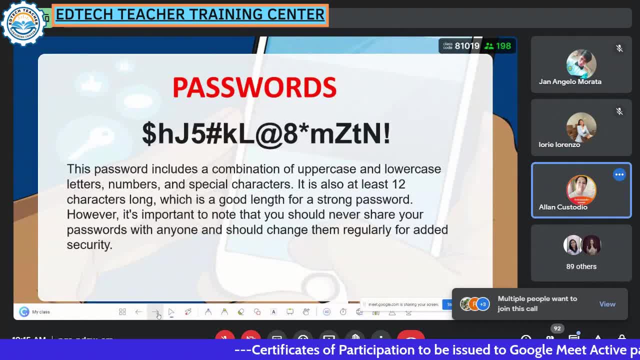 Gano'n sila kabibilis. Ngayon, matatali na po yung mga hacker. tama po ba Kasi? pinag-aaralan tayo Ang tanong, pinag-aaralan ba natin sila? 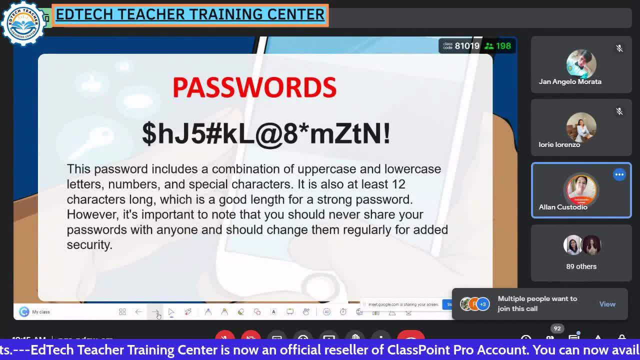 Madalang natin silang pag-aralan. May gano'n na palang application na ginagamit sila sa brute force. Yan ang matindi at sana malaman natin Sa ibang bansa po kada 6 months, 2 months, nagpapalit po ng password. 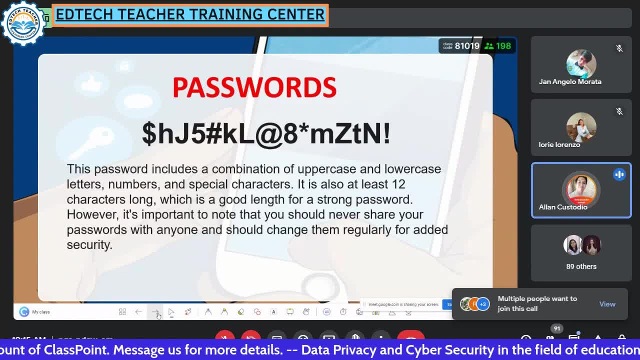 Pati po empalayado, Nasa discretion na natin. kung magpapalit Sa ibang bansa, pinapatupad po yun. Nagpapalit sila ng password sa isang taon at least 1.. 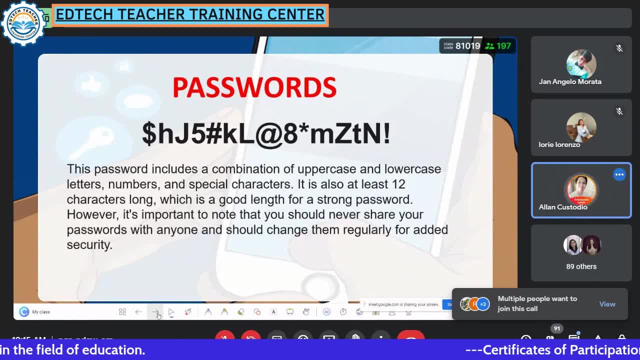 Marami po ba kayong natututunan Chat. nga po kayong number 10 sa chat box Yan number 10.. 10, 15. Wag po kayong maglila Matataas po tayo 11.. 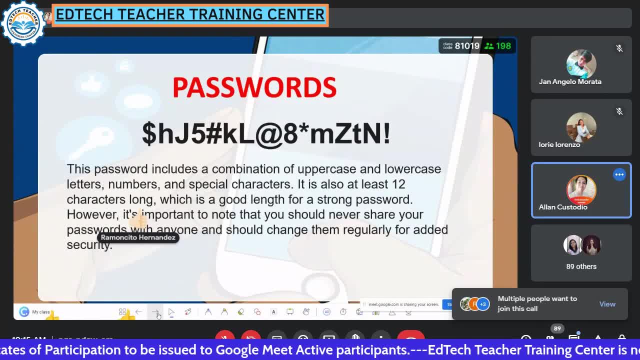 Marami po ba kayong natututunan Chat nga po kayong number 10.. Yan number 10.. Ayan number 10.. Ayan marami pa rin po nagkocomment. no Ayan naglalike sila number 10.. 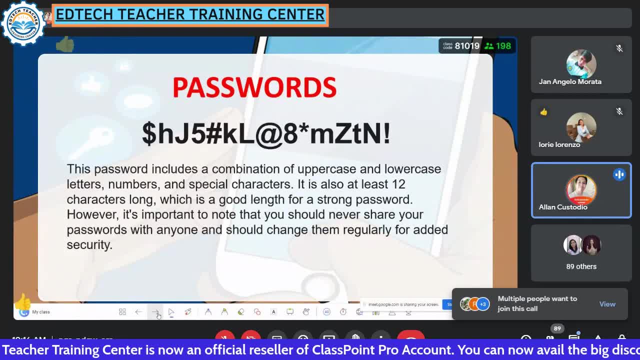 Ayan, So ganun pala, sir. sa ibang bansa Nagbabago pala sila ng password Correct, May regular po sila Maski government employee Nagbe-bell pa nga po. eh Kasama yun sa kanilang cyber security measure. 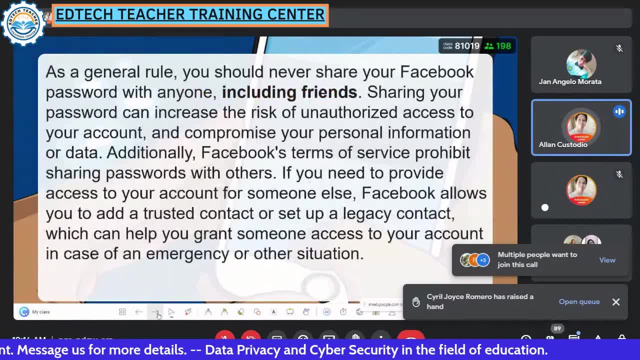 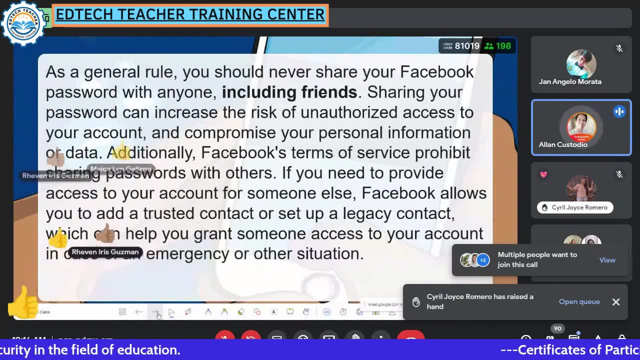 Ganun po ang ibang bansa na Pinapatupad Maski education Ngayon yung pagshare ng password, nakalagay din sa Facebook. Ito yung kanilang rule General rule: Maski sa friend mo wag mo bigay. 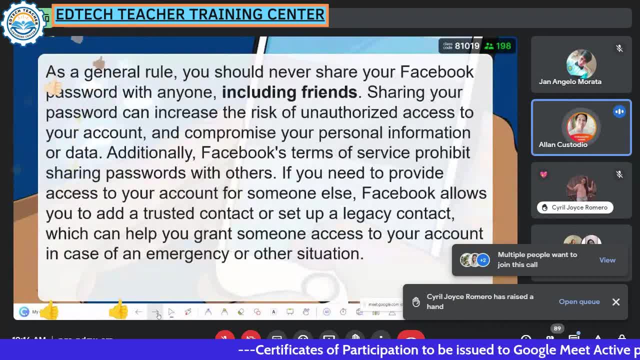 Wag mong bebihin. Dabihan nyo sa mga estudyante Ang mga best friend nyo, alam nyo yung password nyo At gagawa ka na naman. Tapos sasabihin nila: 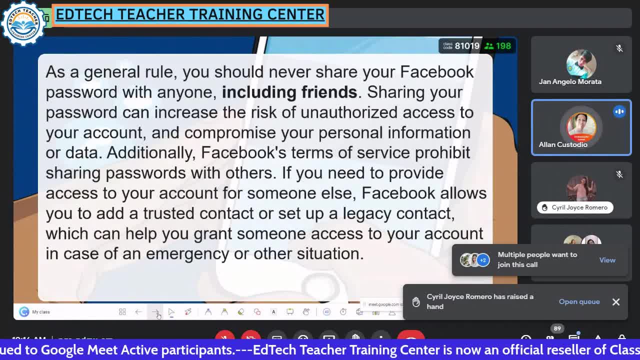 May nahak ka. Uy, hindi naman ako yan Nahak. eh, Ang mali pa nga po ganito. Hindi naman sa mali Kulang ang information ng kabataan. Pag nahak yung Facebook nila, post na nila na nahak na yun. 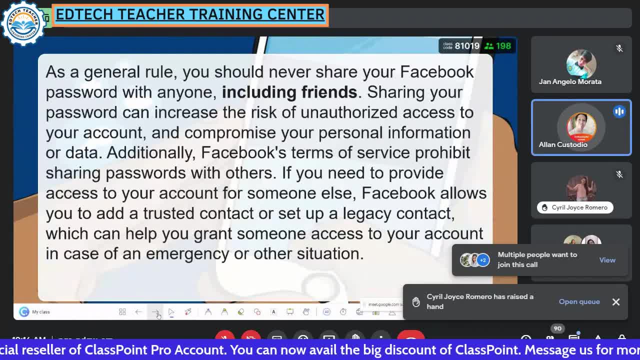 Tapos, eh, wag ipaalam agad or ireport na yung account, Ang iba naman kasi pinapabayaan nila Na. ano pa kala nito Pag nahak sila? hmm, bayaan mo na. 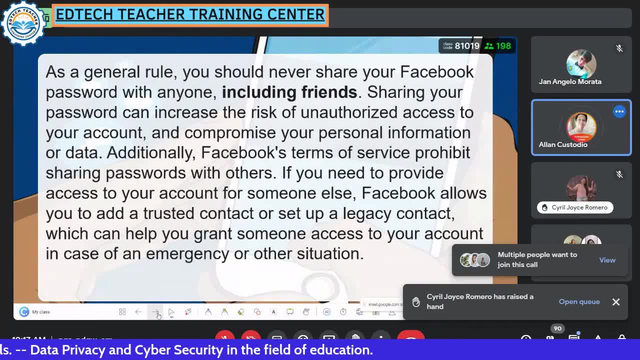 Ngayon naka-perwisyo, Pero kung imaginein mo, kung na-post mo yun, na nahak may Facebook ko, baka ma-aware yung mga kaibigan mo, eh, Kasi hanggat hindi nalalaman yung isang bagay at hindi mo na inilalantad. 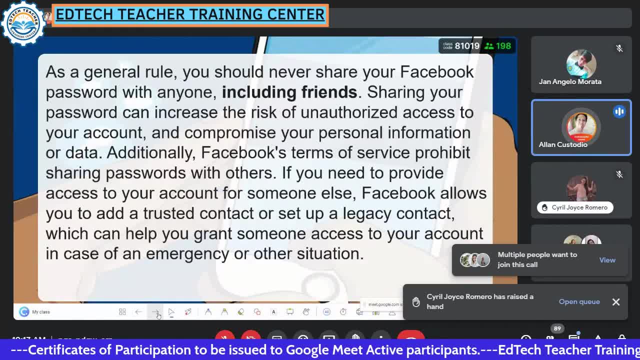 ay maraming maloloko. So lagi nating tatandaan na ang measure ng pinaka-safety ay pagiging sensitive, Especially hindi lang safety, Especially hindi lang sa sarili mo, Sa mga matatamaan. 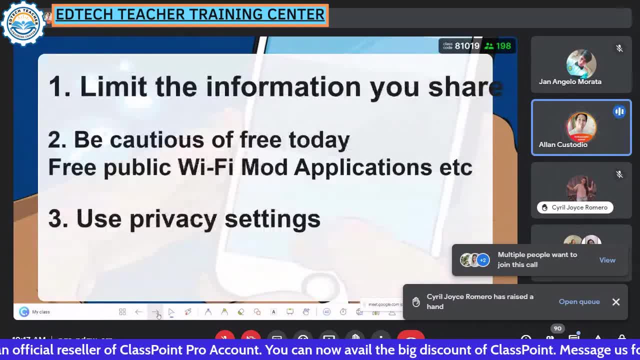 Yan, Okay, Next natin Eto wag nyong gagawin Sinong kumakonect ng pre-Wi-Fi sa mall. wag nyo na pong gawin, Kasi may nahuli channel 2.. 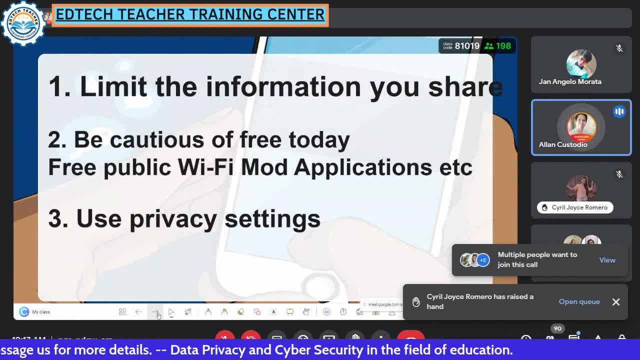 May device. Panawarin nyo po channel 2 na public Wi-Fi Search nyo public Wi-Fi hacking channel 2.. EBS-CBN Na nahuli sa mall Ang tina-target nila matatanda. 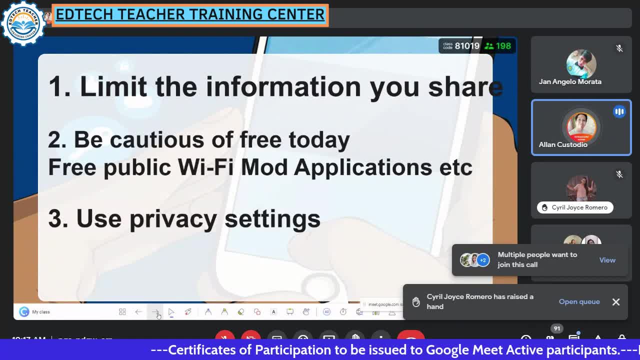 At ahakin doon nila yung GCash OTP. Yan ang sinabi: Grabe, no, Okay, Wag kayong kukonect sa mall Sukat na mag-data ka na lang, Kasi meron silang device na kukolekta ng IP address mo. 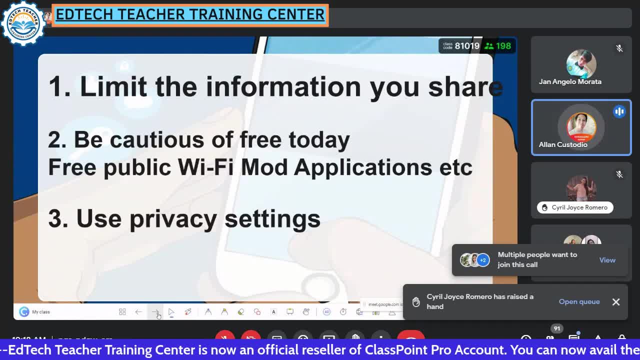 E naka-on yung GPS mo Habang naglalakad ka, nag-withdraw ka at nakitang antagal mo, andun yung sindikato Binaril ka na Ganon Napakatalino nila. 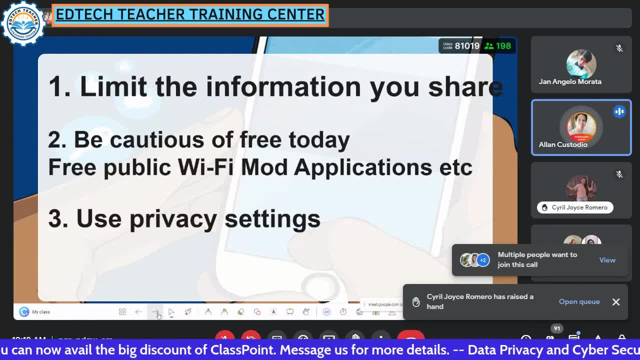 Ngayon hindi mo alam yun. eh Ba't biglang may ano dito kriminal Hindi nila alam. Kasi hindi natin alam na may application, at may device na palang ganon Nahuli po yan channel 2.. 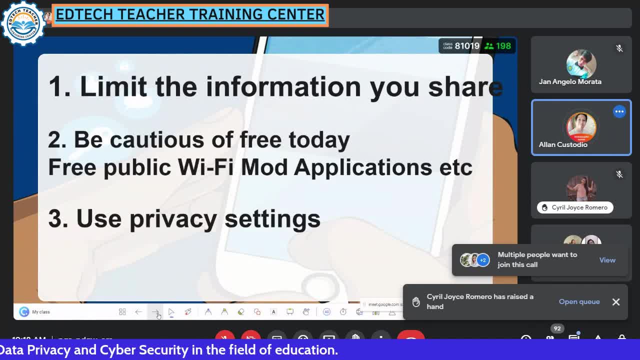 Panoodin nyo mamaya sa YouTube. Yan ang sinasabi natin, Na advance na silang masyado, at hindi alam yun Maski kabataan. Basta free wifi, sunggap agad, Eh mayaman pala yung bata. 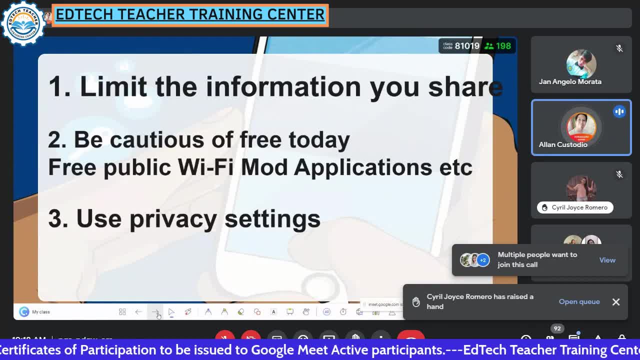 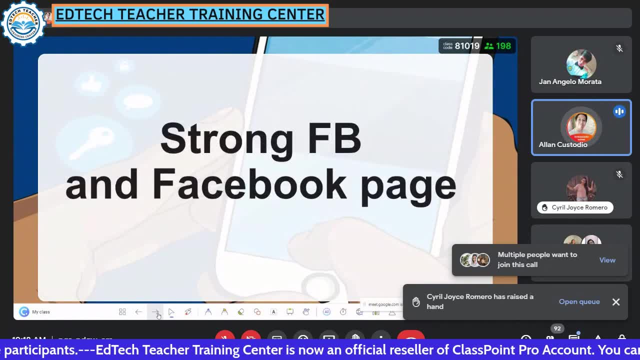 Kidid na Patay na Yan ang sinasabi nating hindi sila na-inform agad. Ang ganda nito, irigyan sa mga ano eh Kabataan, eh Strong FB. Tingin kayo mabuti dito. 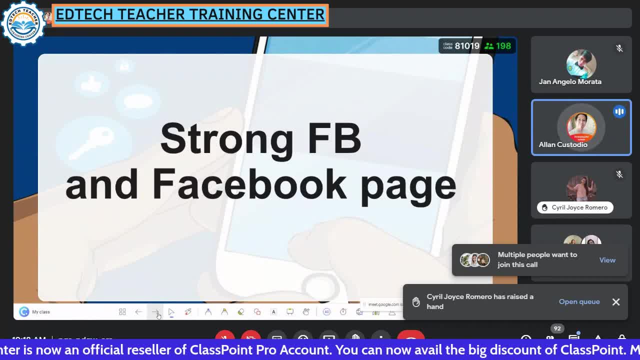 Mag-memeta na po tayo. Masaya po ba kayo sa session. Okay, Masaya po ba kayo. Ayan marami nag number 10.. Ngayon itong Strong FB at saka Facebook page. 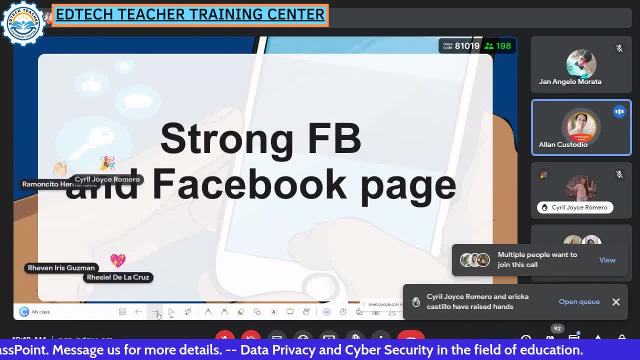 Sino ang mga may Facebook page dito Di ba lahat ng school, Lahat ng organization, Maski nga po NPC may Facebook page. eh Paano magiging secure yan Yung profile locking ay hindi pa binabalik ni Facebook. 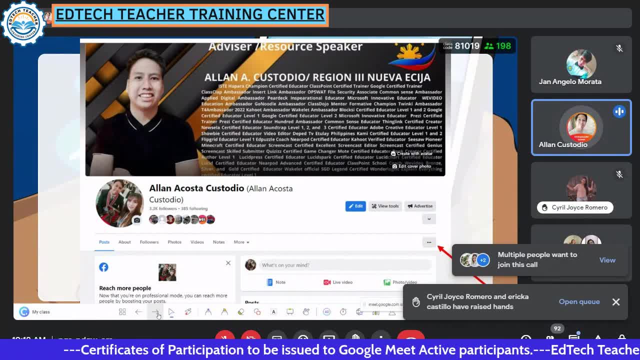 Kasi masyadong mataas yung security nga niya Ang naging problema po ba. Alam nyo, nun Meron kasing mga hacker na nagpo-profile locking Ngayon hindi mapasok halos Ngayon. itinanggal muna yun. 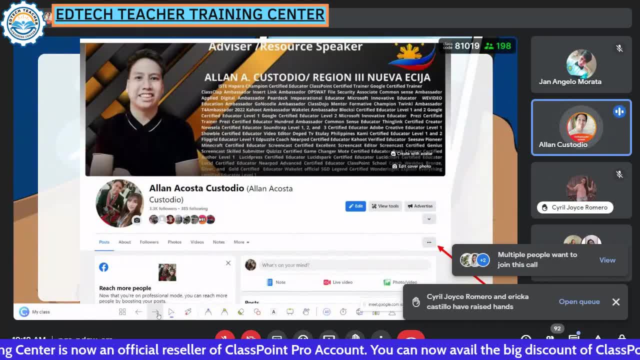 Pero meron pa tayong mga measure. Okay, Tingin Ito na po Facebook ko. Yung Facebook ko na to ay hini-share ko na sa inyo, Para nang sa ganun malaman ninyo ang setting. 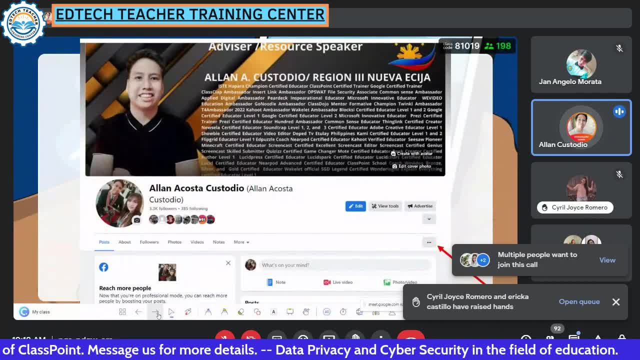 Pwede itong ulitin. Pwede itong ulitin: mga mam Ngayon tingin ng mabuti. Ito na yung puso ng cyber security sa education. Bakit ko pinili ang Facebook? 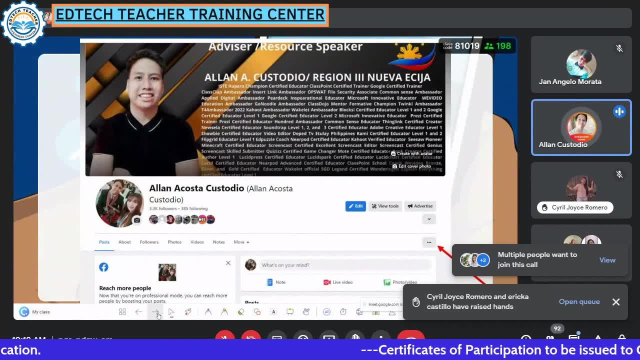 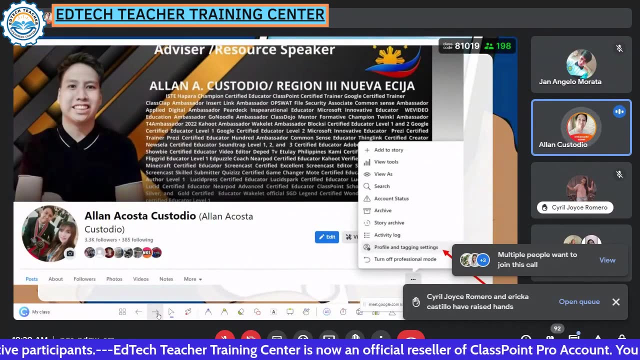 Kasi 99% of the time Filipino, especially students, are using Facebook right now. Ngayon, may three dots dyan Tingin ng mabuti. Lahat po Next natin profile tagging setting. Ngayon, pagkatapos ang profile tagging setting. 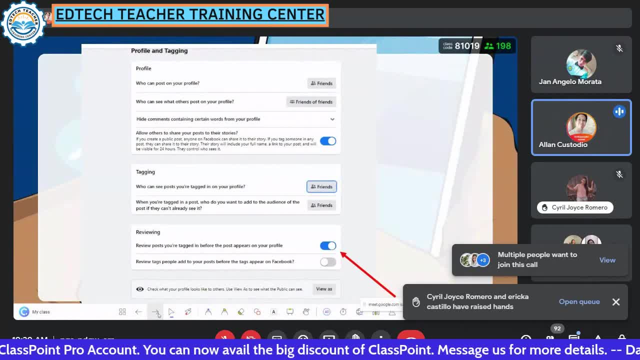 ay i-on nyo yan Sinong natatag dito na biglang may laylitaw na kabastusan na experience na may malaswang tinag ka ala ka namang kinalaman doon. Chat nga tayo, number 11.. 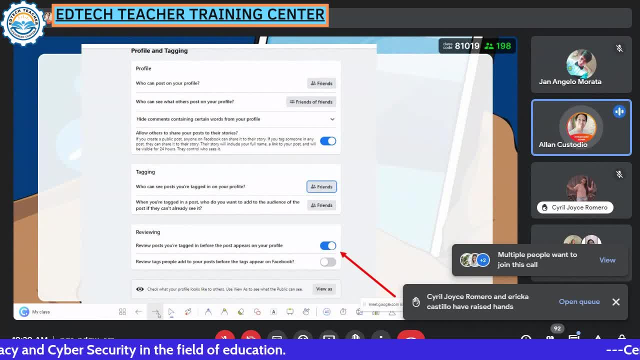 Number 11. Chat nga po tayo. kung may biglang may nagchat sa atin ng ano eh Kalaswaan Ay nagchat, Natag ka bigla ganun, Hindi mo alam. Ito na po ang solusyon. 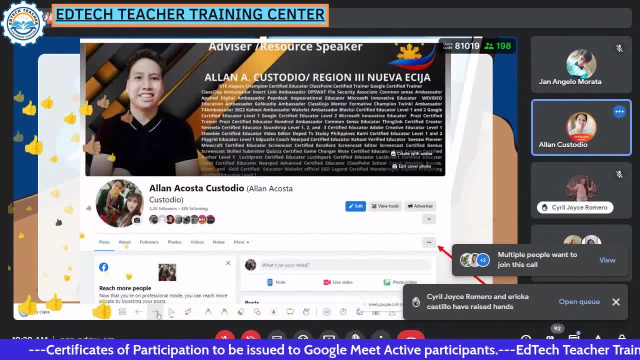 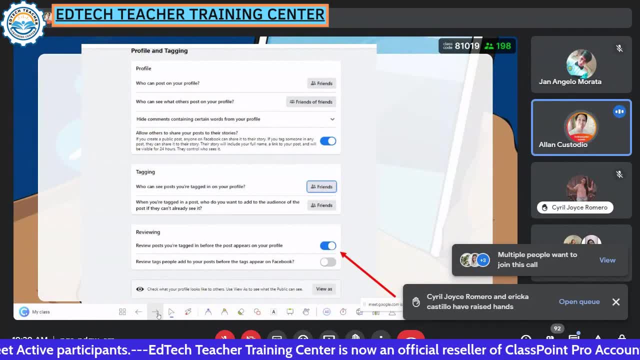 Ulitin natin Three dots Profile tagging setting I-on nyo. Nakaka po kay Facebook yan Pag na-i-on nyo. yan ay magnonotice sa inyo. kung gusto kayong matag Pag pwede mo yung i-reject. 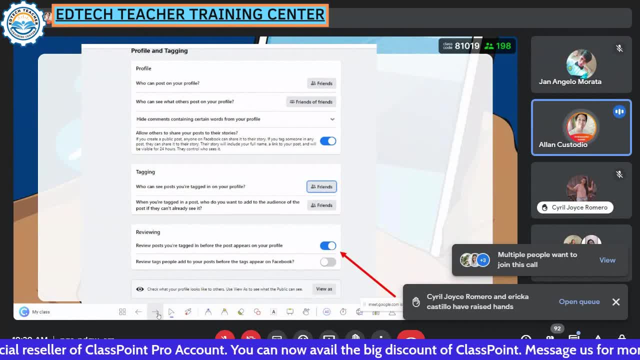 Okay, Naka-on po sa akin yan Facebook account, ko po ginamit, ko po dyan para sa inyo, Kasi syempre matututo kayo by experience at ano ba talaga Kaya ipinapakita natin dito. 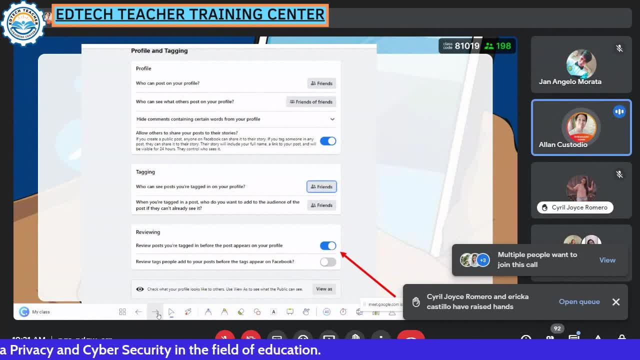 Hindi lang basta sinasabi dito sa EdTech Training Center: ay tinuturuan talaga kayong mabuti para maligtas kayo sa mga bagay na makakaharm sa inyo, I-share nyo to sa pamilya nyo. 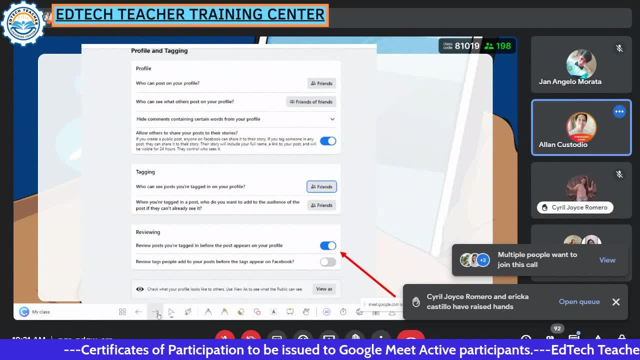 I-share nyo to sa mga studyante nyo Lahat. Ulitin natin Three dots Profile tagging Profile. Ayan, nga pala Tapos. review post On: Okay, Now Eto Para sa mga kabataang natitrigger. 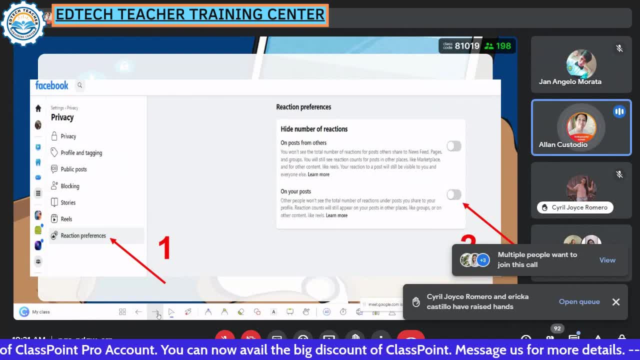 na dahil yung reaction nila ko konti lang sa Facebook. Puso to Punta kayo dun sa privacy Reaction preference Saan na po to Sa cellphone. meron lahat, eh, And on your post, Okay. 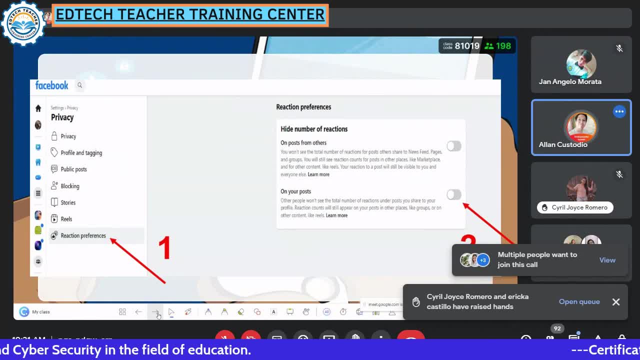 Okay On your post or on post from other, Lahat mo kasi yan naka-off. Pwede nyong i-on Ako kagabi ko po inan eh. Pero dito po kasi sa screenshot ko na off pa yan. eh. 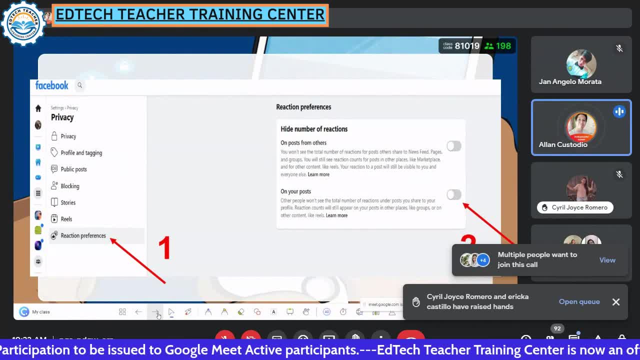 Pwede nyong i-on Lahat ng post mo ay makikita mo na may puso at like, Pero hindi mo makikita yung number Marami po kasing mga sensitive. eh Uy, bakit hindi ako nilike? 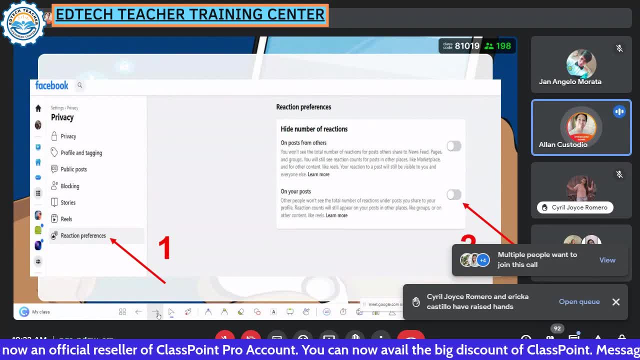 Hindi ako nilike ng kapitbahay ko, Hindi ako nilike ng kwant. Pero may tanong ako sa inyo: Ah, Mindset lang po yan. Hindi po nyong mapiplace lahat ng tao. Hindi nyong mapiplace lahat ng tao. 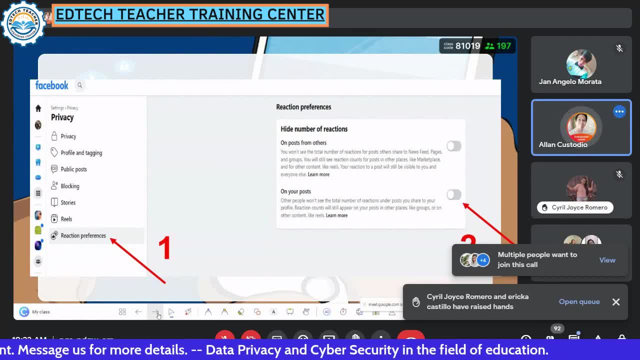 Pero ang happiness makokontrol mo sa sarili mo. Kung ngayon, kung diyan ka magre-react diyan sa mga emo-emotion na yan, emo-emoji, eh, huwag po sana tayo maging mababaw. 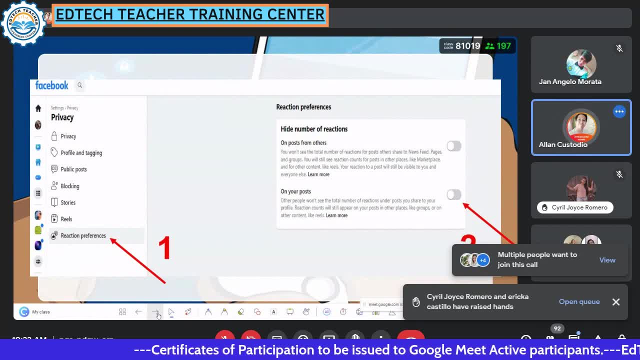 Ang buhay ay hindi iikot sa emo-emoji. Ang buhay ay iikot kung pa, paano ka nagpapatuloy sa aksyon na ginagawa mo sa buhay, Kung wala man naman. 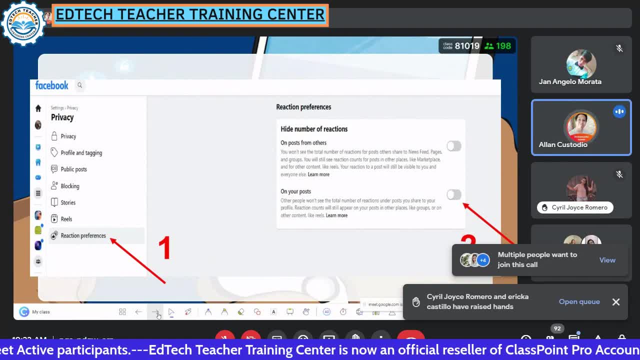 kung wala man naman nagtitiwala sa iyo, dahil ikaw ay student, may mga pinost ka dahil maganda ito. hindi nilike, it's okay. At least na gampang namang dapat mong gawin. 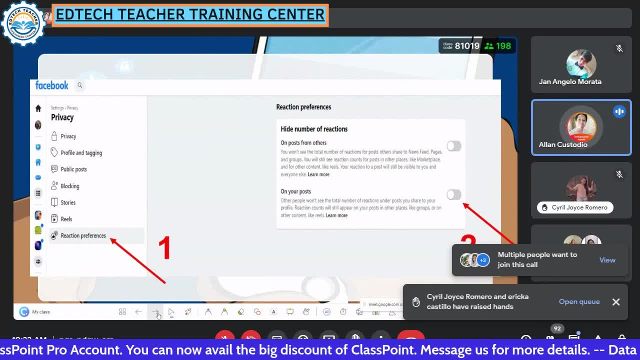 Kung ikaw ay teacher, hindi ka nilalike ng mga estudyante mo, it's okay. Alam mo namang tama yung mga pinopost mo At kung ano ka pa, mindset lang din yan. Pero kung talagang ayaw makita reaction preference on your post, on nyo yan. 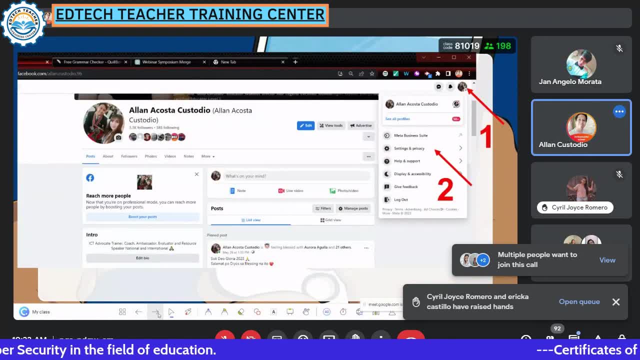 Okay, Next natin Eto Tingin ng mabuti. mga mamat, sir, Eto need nyo ng kailangan. Meta na po tayo dito. May picture na maliit sa taas. Ngayon ikiklik mo yung setup privacy. 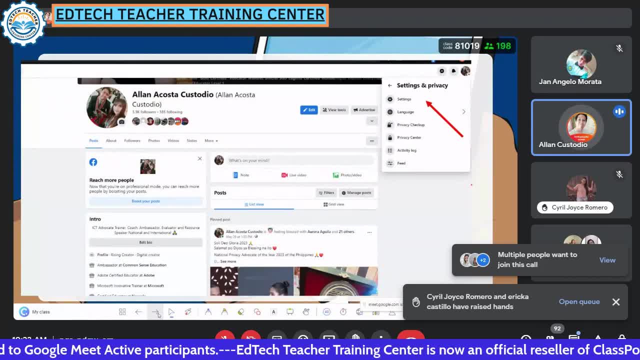 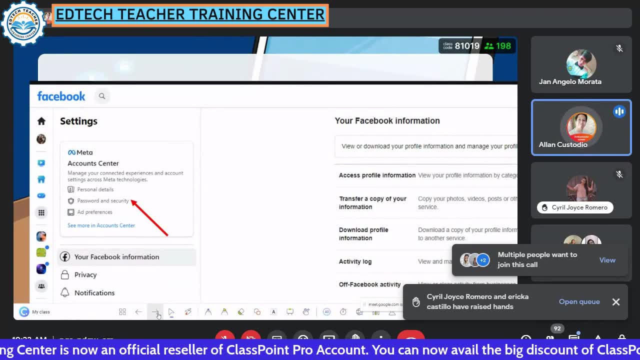 Setting and privacy. Tapos, pagkatapos nun ikiklik mo yung setting, Ngayon pupunta tayo sa meta Ayan na Yung meta, ikiklik mo yung password security Ayan na. 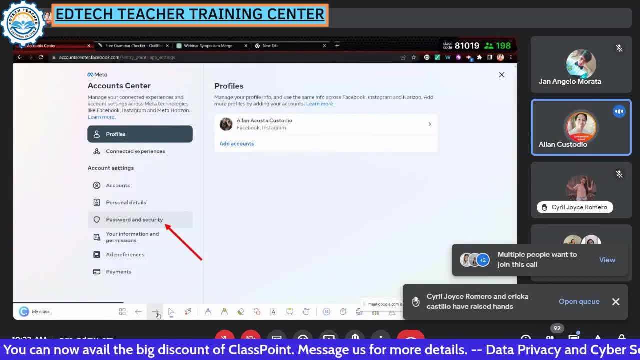 Pagkatapos nun ay pupunta ka ng password, security, Meta account center. Bakit po dyan nilagay ni Facebook sa meta? Ang meta po kasi lahat ng may meta at saka web3, ang unang inaayos nila at requirement sa kanila ng ibang bansa ay security. 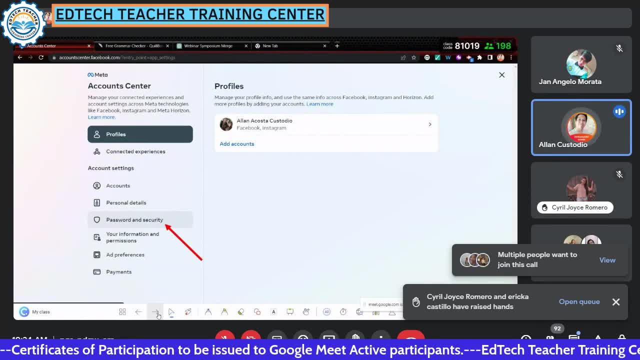 Saka na lang po, kung anong picture dang ilalagay, nila Mas pinapalagahan ang security ng bawat isa kaysa yung ma-offer mong picture. Bakit, Eh, syempre makakasuwan sila ng data breach. 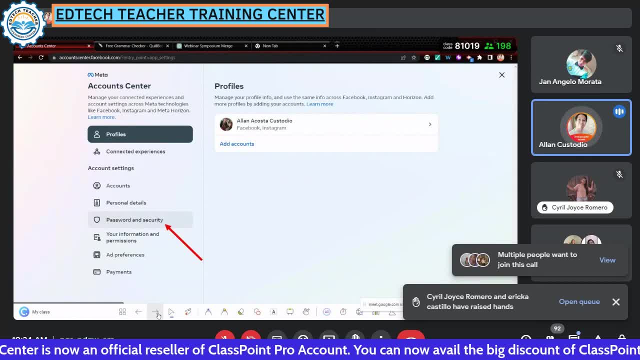 It depends upon the nation kung ano ang batas nila doon at jurisdiction Sa atin kasi NPC. Ayan Sige nga po kung marami kayong natututunan. chat nga po number 12.. 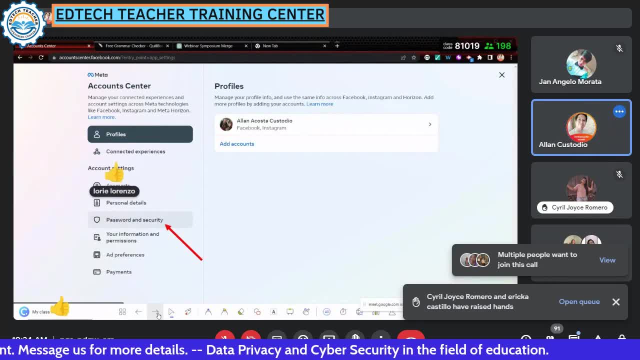 Chat nga po kayo number 12.. Okay, Kung meron po talaga ding mga active ay number 12.. So marami po mapalakpak din sa Google Meet. Thank you. thank you, Tuloy tayo. 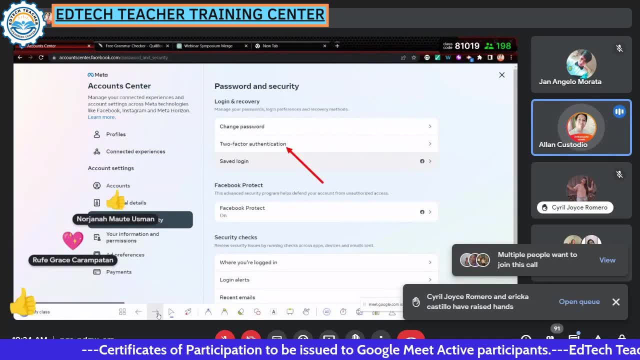 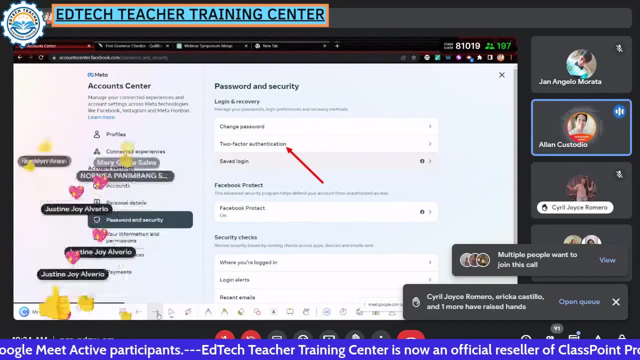 Dito pagkiklik may password papasok kayo Dito two-factor Sa two-factor na ito. hindi po ito option Obligado Ayan, ah, Obligado na sana ito. 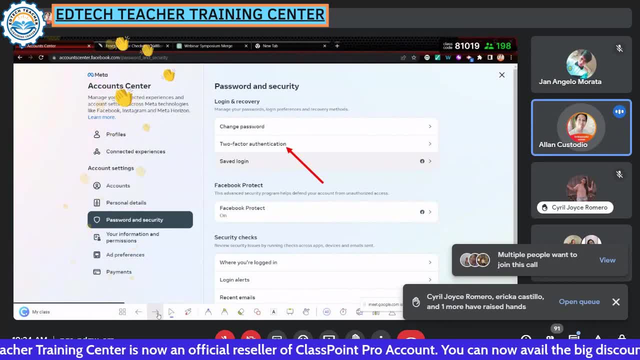 Ngayon sinasabi nila: oh, option ko lang mag-two-factor, Tandaan mo pag namali yung password mo, hindi mo na yun ma-re-recover, Kasi walang two-authentication factor. eh Paano mong ma-re-recover yun? 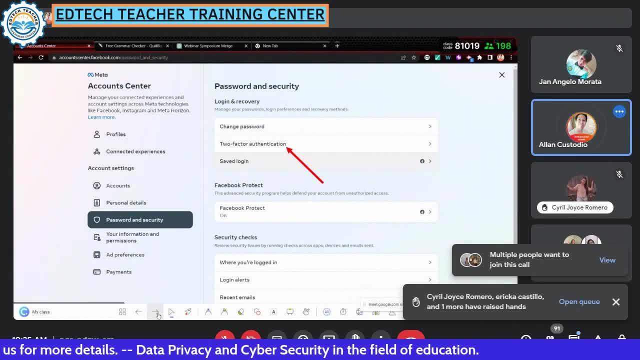 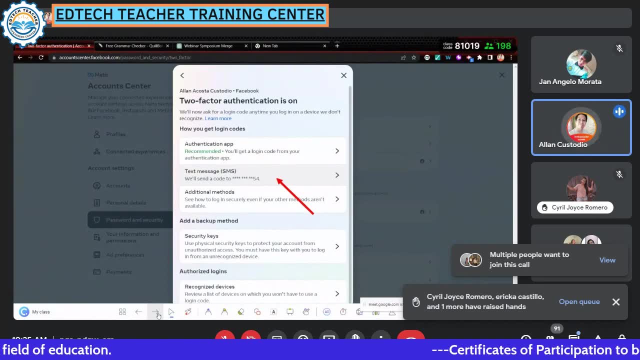 Diba, Kailangan ka maglagay nito at dagdag protection. Ngayon, iklik mo yan, Pagkilik mo yan may number dyan. Ako naglagay na po kasi. So therefore meron dyan. 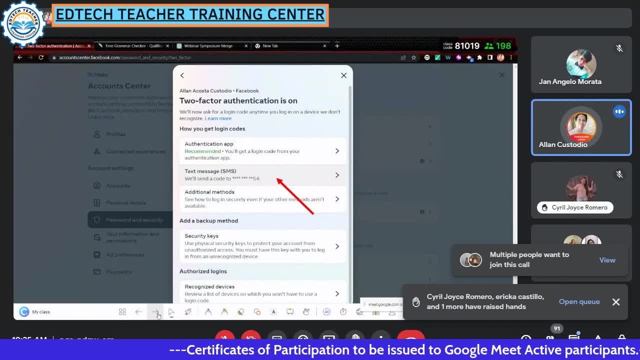 Pero pwede kang magdagdag. Ano, pwede mo magdagdag dyan kung Facebook page nyo para matinde Number mo, Number ni principal mo, Number ni ICT core, Kung sino pa yung dapat maging admin ng page. 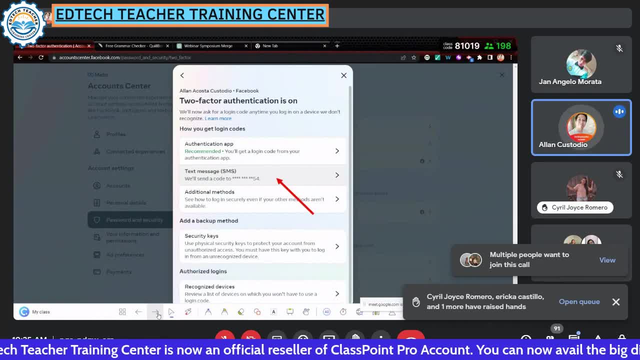 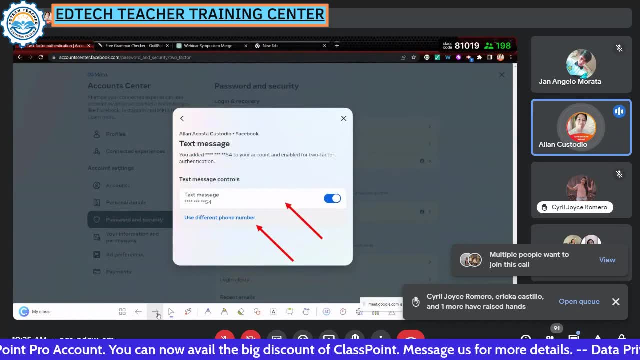 Para lahat doon mag-notice kung may nag-hack. Kasi, alam natin tayo-tao lang nagpapahinga, Iba-iba yung time ng pahinga natin, Pero kung may mga nilagay tayong ibang number ay mabe-verify din nila. 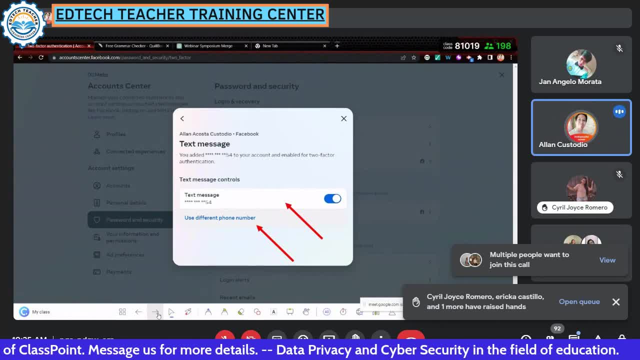 So diba, Kahit tatlo, Pero huwag masyadong madami. Huwag masyadong madami, Kasi hindi naman kaalaman ng iba. Naku lalo lang madisgrasya. 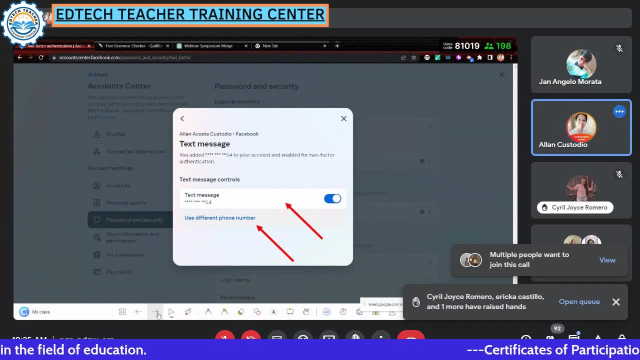 Yung bibigyan nyo ng two-authentication factor. yun nakakaalam. Okay, Maging totoo lang, Kasi minsan ang nilalagay hindi alam. Tapos pagtatanong ngayon hindi rin alam ang sagot. 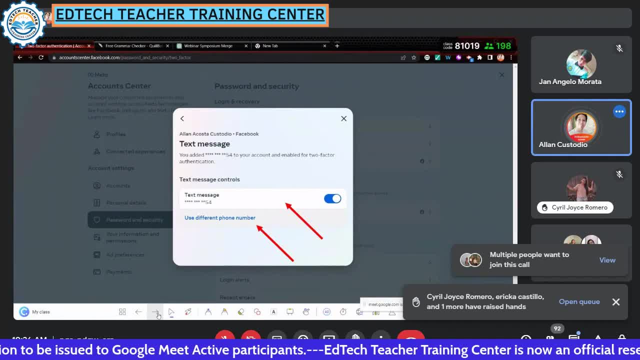 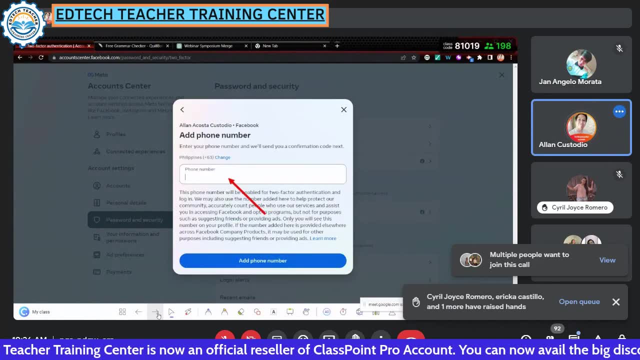 Anong gagawin natin dun sa security ng Facebook page natin sa school? Eh, wala, Okay, Ngayon, pag nagdagdag ka ng bagong number, kiklik mo to, And kapag nagdagdag ka ng number, lalagay mo yung number mo dyan. 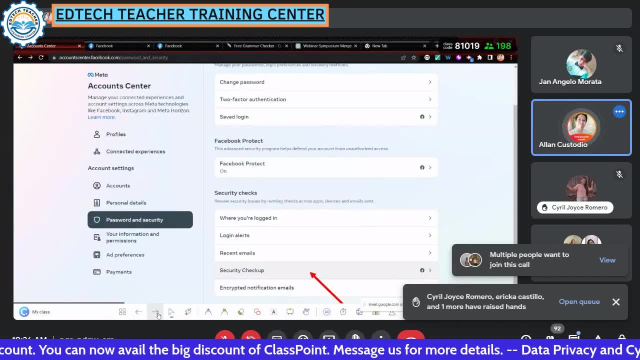 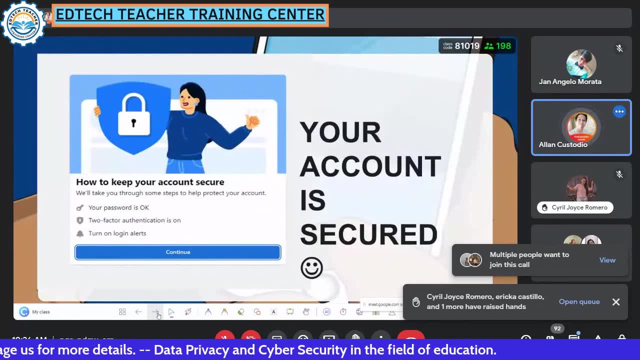 Lalagay mo yung code, Magte-text sa'yo. Ay, okay na yun. Ngayon pupunta ka sa baba Security Checkup. At eto Paki-screenshot to Eto ang dapat muka ng ating Facebook profile. 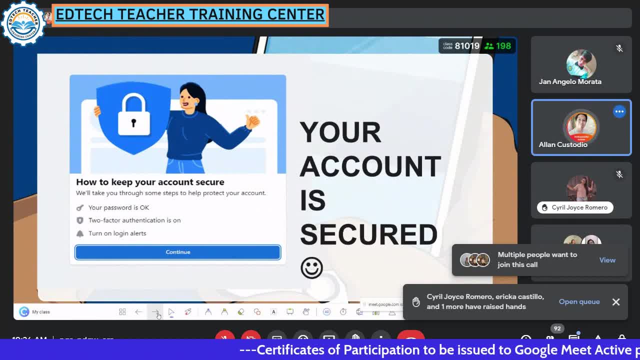 Pag kinlik mo yung security checkup At dapat ganito din yung page. Pag hindi ka pa nakaganito ay hindi secured. Your password is okay. Your two-authenticator factor is okay. Turn in on login alert okay. 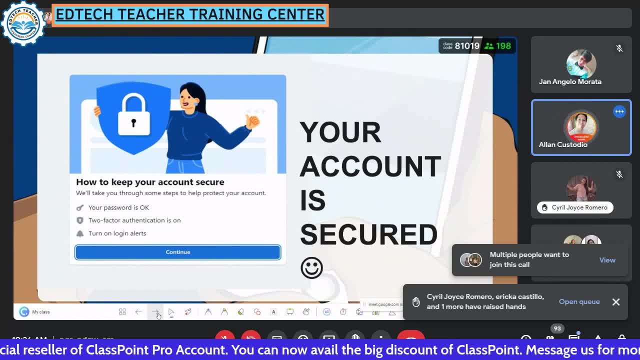 Naka-off po yan kay Facebook Ngayon. i-on natin yan San ba tayo pupunta O malapit na. Ibigay nyo tong screenshot na to sa kayo. Kung ICT coordinator po kayo or kahit ano kayo may Facebook account kayo. 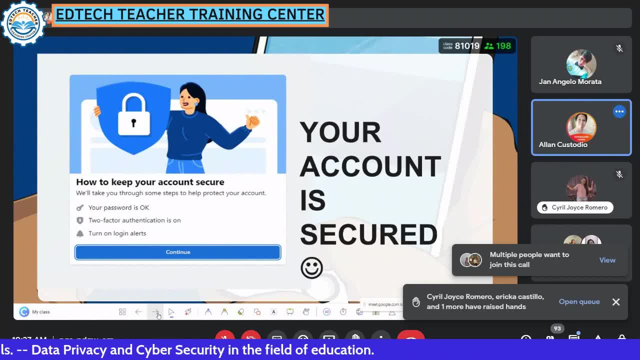 Ganyan dapat. Yan po yung nakalagay sa account ko. Totoo nyong nakikita yan, kasi yan ang nakalagay din sa Facebook ko. Okay, Ngayon Dito, i-click nyo po natin ito. 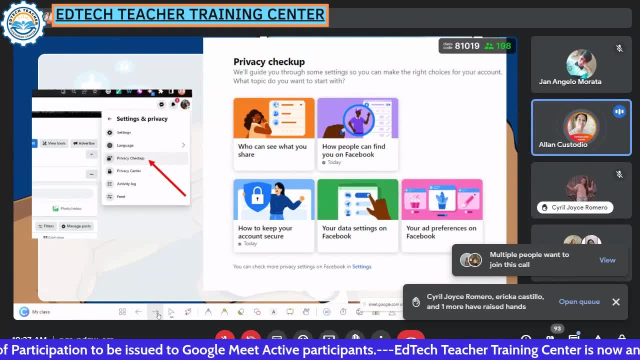 Eto yun yung picture din sa taas, And then Privacy Checkup. May lima kayong pagdadaanan sa meta. Eto yun I-click nyo po lahat yan Tapusin nyo. 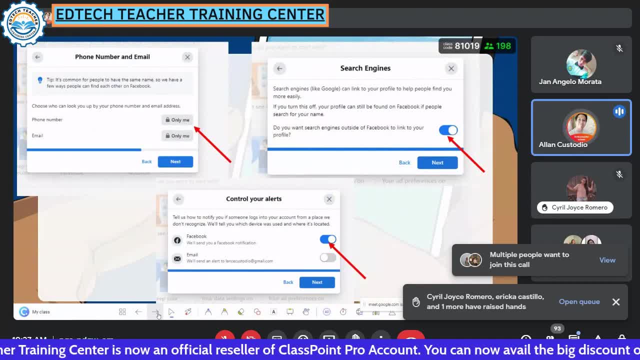 Para magkaroon kayo ng secured At una naka-Friends po ito Phone number at saka email Naka-Friends po yan. Kung may Facebook ka, I suggest only me, Ina-only me ko yan, Pero pag Facebook page po kasi okay lang naman may email at saka number. 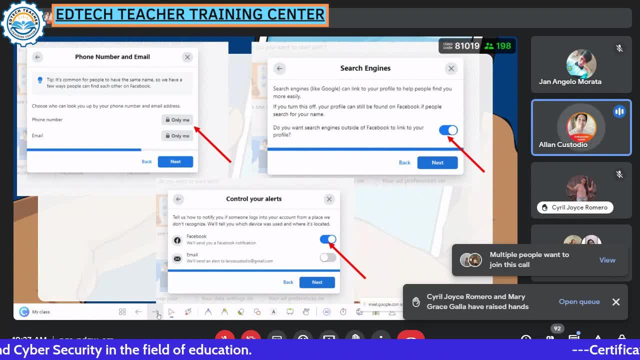 Diba, Kasi nga pinopromote yung page, Pero para sa akin, kung personal mo, huwag mong pamigay yung number mo, Only me, At saka huwag friends-friends E papano. kung hindi na pala friends, yun na-hack. 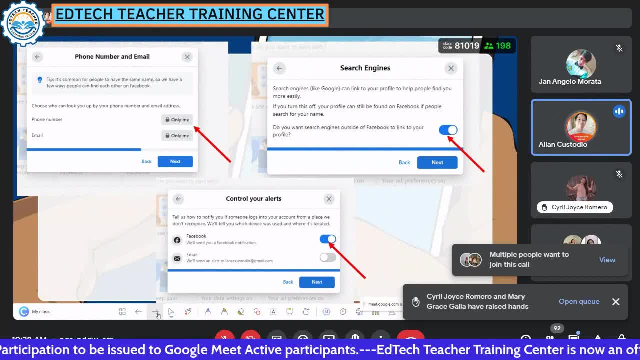 Tapos kinakita yung number mo Nasa about Doon sa may setting mo sa about ando yung number mo Naka sa bulat doon O tawag-tawagan ka Diba. 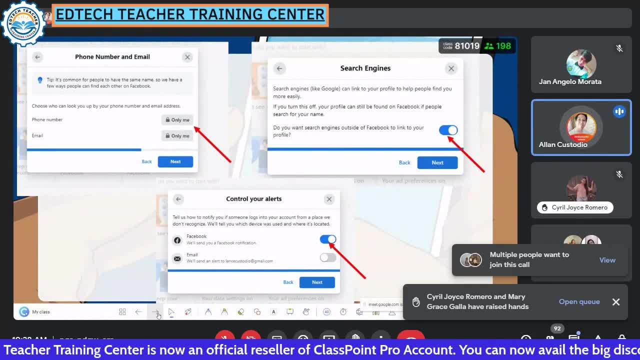 Ngayon I used to authenticate or pa-ano to For my Facebook. Okay, It's si, Ma'am Maria Kimberlyn. Very good, Ma'am Watching Maria Cristina, Okay, Thank you. thank you, po, Good morning, good morning. 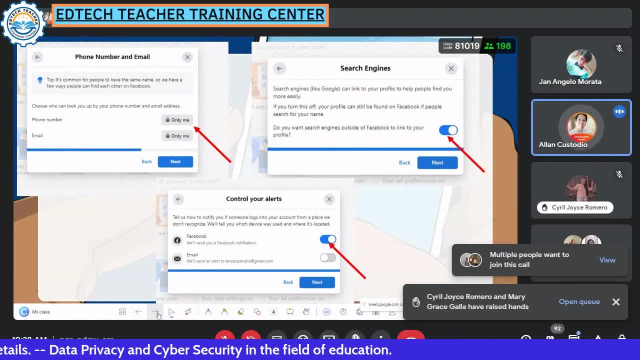 Ngayon yung control alerts po ay naka-off, kay tinatawag natin Facebook. I-on nyo yan. Tapos yung search engine automatic naka-on naman, Pag in-off mo yan. hindi ka masasearch O kita nyo to May nag-hack sa inyo, Pero naka-off yan. 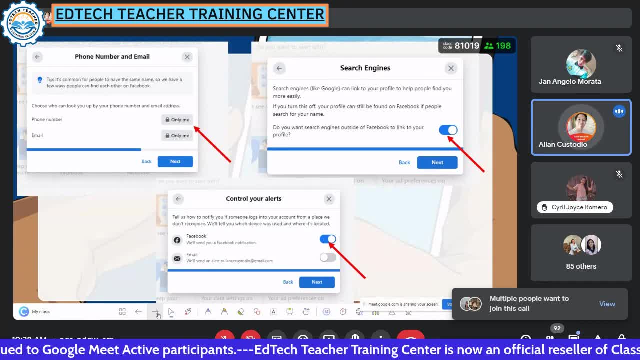 Papano mong malalaman siya Lalo't, hindi mo pala alam yung setting na yan, Kasi gusto lang niyang patamaan ka eh, Gantihan ka niya Diba O Dito Papasok na ngayon. 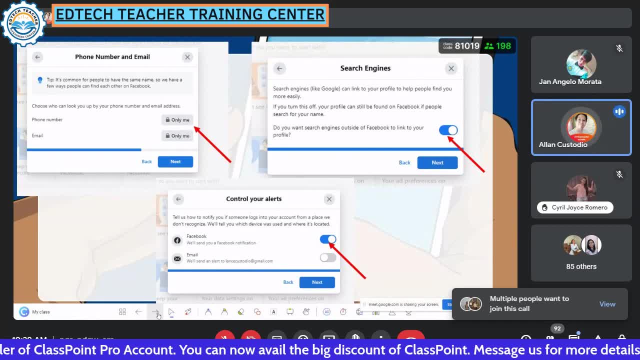 I-locate ka ng IP address Pwede ka nang patulong kapag ikay argabiado I-send mo yung mga screenshot Kaya yung file of evidence. mahalaga po yan Mag-screenshot tayo. 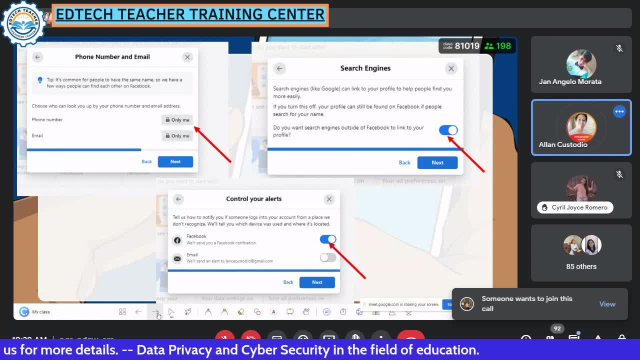 Bigyan ko kayo yung sitwasyon: May nang bully sa'yo, May nang bubuisit sa'yo Katrabaho mo o ibang tao, Kada bully niya sa'yo ina-unsend niya. Alam niya po yung unsend diba. 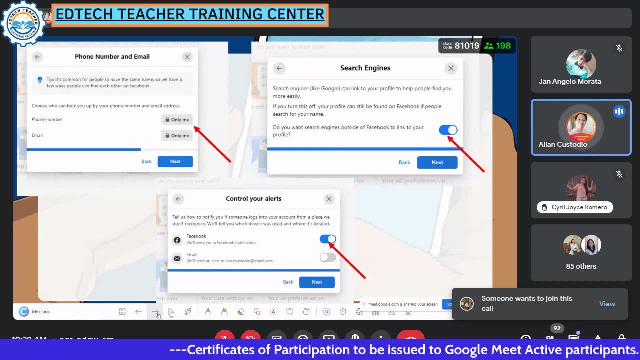 Kaya dapat mabilis kang mag-screenshot. Alam mo yung mga boton na yun sa cellphone mo, Kasi pag nag-unsend sila papaniwalaan ka ba kung na-unsend tapos ipinapakita mo. Yan po sabi kasi dati. 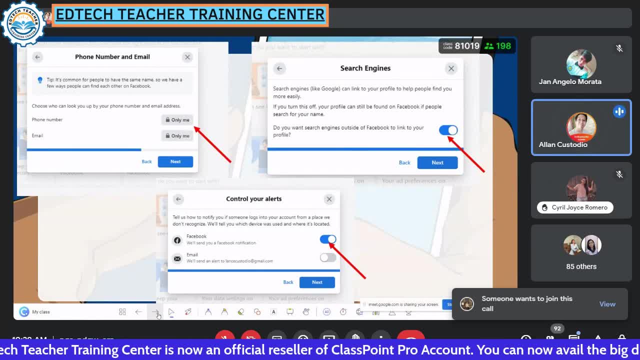 Ang daling pabulaanan eh Ang daling palusutan. Kaya alamin niyo kung saan niyong i-screenshot mabilis, kayo dapat Yung mga ebedensya na yan hindi pinapalagpas. Matatalino po hacker. 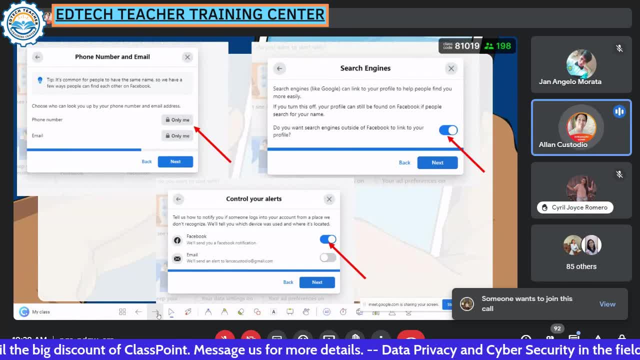 Naniniwala po ba kayong matalino sila? Eh, halos matalino talaga sila, kasi marami silang naloloko At yung naloko nila ay na-outsmart, Na-outsmart, nila Dapat mas smart, Mas maano tayo Discarte syempre. 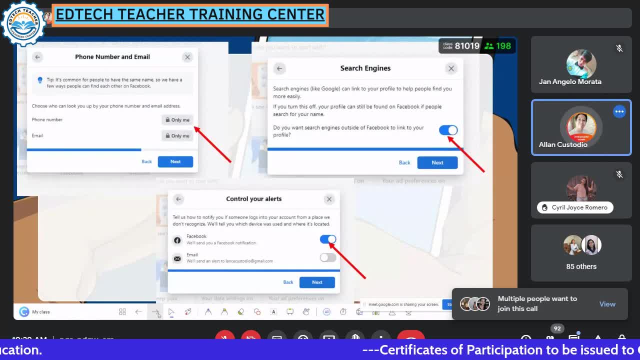 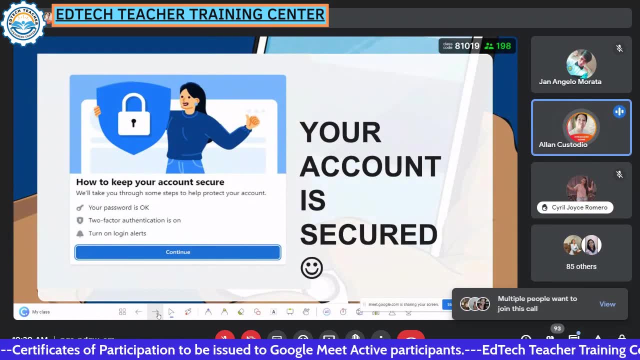 Ngayon, siguro po natutunan niyo na po ito, Punta po kayo mamaya sa privacy check-up at ayusin po natin yan Dapat ganito yung account niyo, Kasi yan ang magbibigay ng cyber security sa inyo. 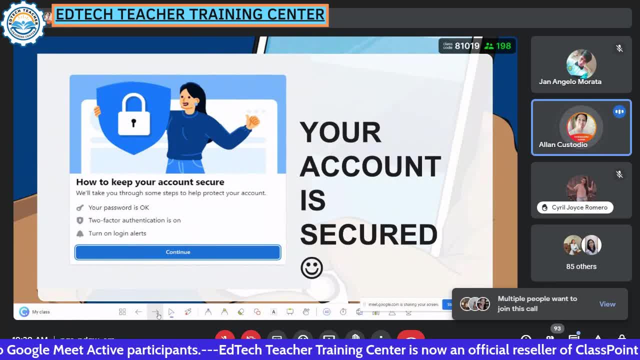 Lalo na sa mga kabataan natin. Last time mag-talk din po ako sa isang high school, na big school na almost mayroon po sila na population na almost magpo 4,000 estudyante po, At tinuruan ko po sila nito At secured na po silang lahat. Yan po yung magandang maging tulong natin. 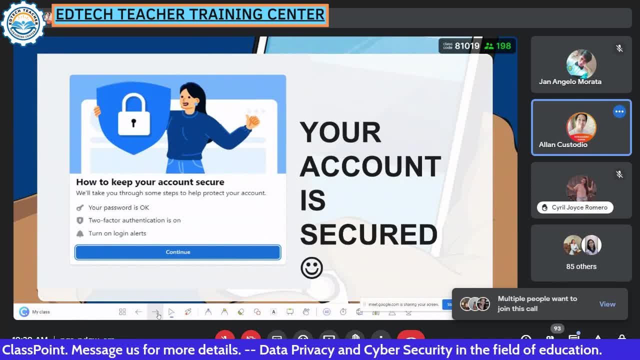 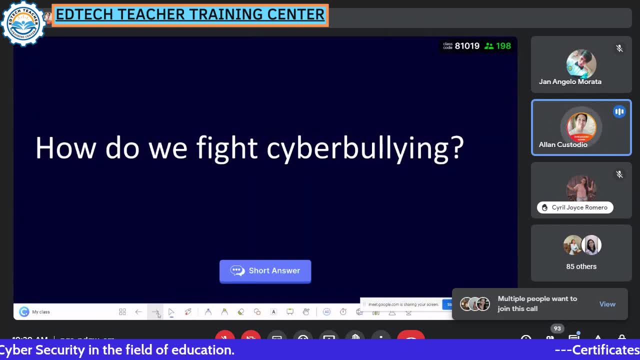 Sabihin niyo po sa anak niyo na yan pwede, yan Ok Sa cyberbullying. magpakalalim po tayo ng konti. Paano nating lalabanan yung cyberbullying? Ang dahing pa rin pong nasa chat, ha Sige. 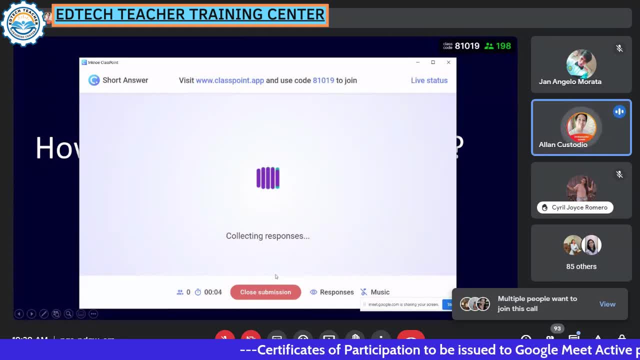 Time check natin 10.30.. Sakto po 11.30, matatapos tayo. Huwag po kayong mag-alala: No, Makapagluluto kayo ng mga bulalo dyan, Mga palalambutan Kasi Sunday ganda gumawa ng forms. 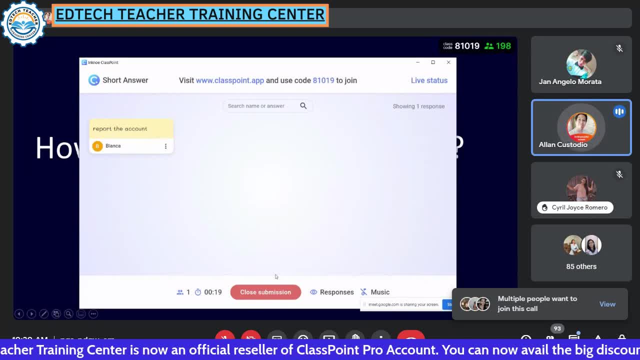 Ngayon ko lang nalaman ang ganito. Thank you, sir, Ma'am Roseanne, thank you din sa iyo, ma'am. No Recorded to Pwede niyong ulit-ulitin Pakishare po ito sa ating mga estudyante, mga iba't-ibang school, Kasi ito pong talk ko na ito, natalk ko po ito sa guidance counselor ng isang division. 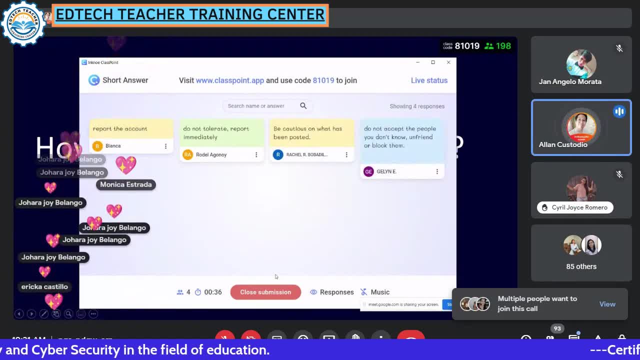 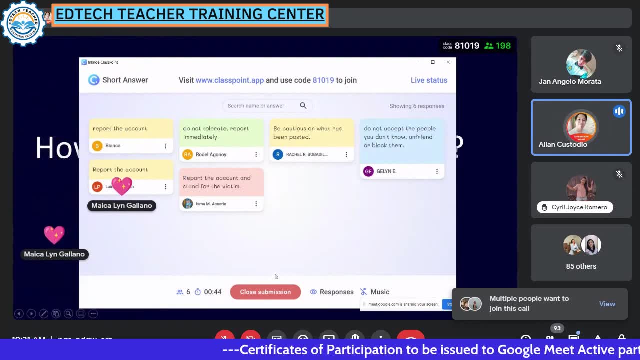 Natalk ko po ito sa Philippine National Police, Natalk ko po ito sa mga big school. Talagang nagbago sila yun sa mga setting-setting nila. Kailangan kasi eh Hindi po option Obligado na Ang daming pong matatalinong hacker eh. Very informative session. Thank you, sir. 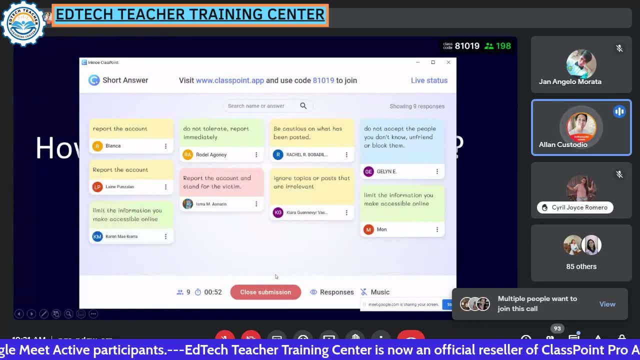 Thank you, sir J. Thank you, thank you, sir J. Shoutout sa iyo, sir Ma'am Ivy. thank you. thank you, Sir Job. thank you, thank you. Okay, So yan ang nakalagay dito. Report the account. Do not tolerate, Be cautious, Do not accept people. Limit information. 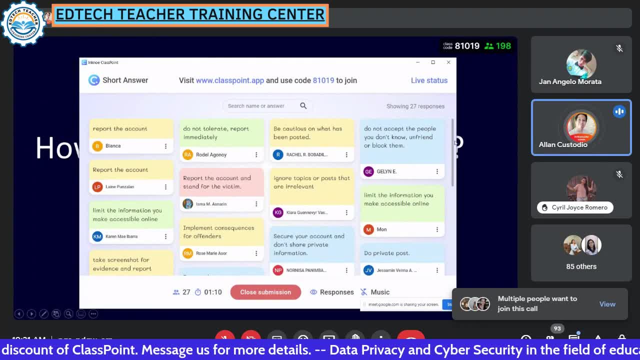 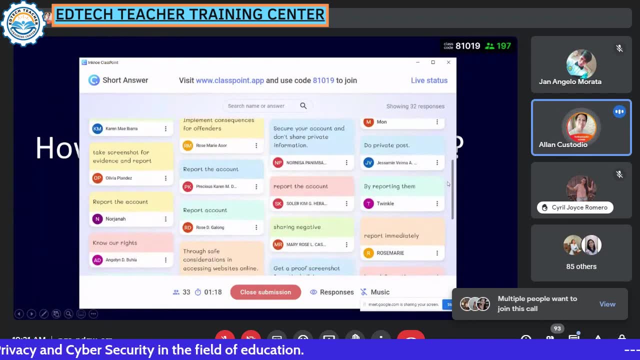 Babaan natin para makita lahat ng sagot niyo Live yan Live Facebook. Pwede niyong balikan Ayan Yung mga nagpa-participate Shoutout sa inyong lahat. Hindi ko man kayo masabi, pero lahat po yan tama. 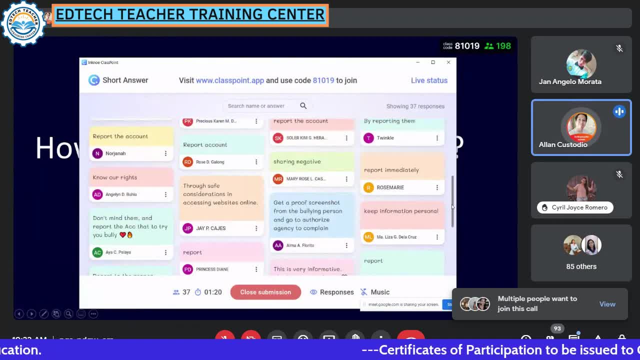 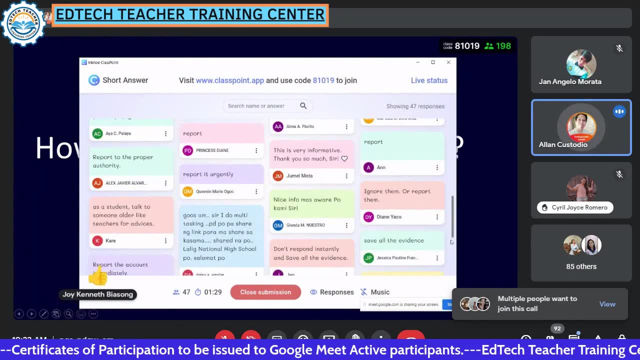 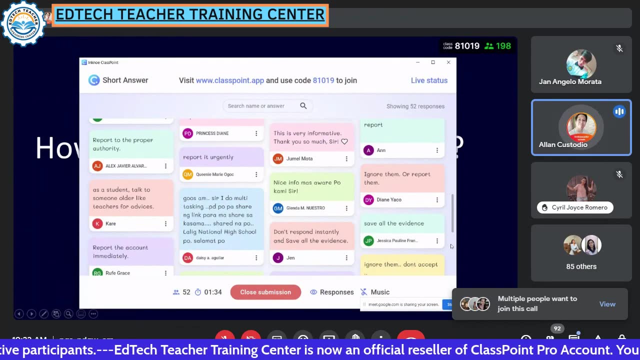 At talagang alam ko yan ay galing sa talagang pinag-isipan. Kasi think, before you click nga po. eh, Diba po Ang rules natin Ngayon. Nice info, Aware na po kami, sir Ayan o Shoutout, ma'am Glenda, Report it urgently Correct. Pwedeng i-report agad yun. Ignore them or report Correct. 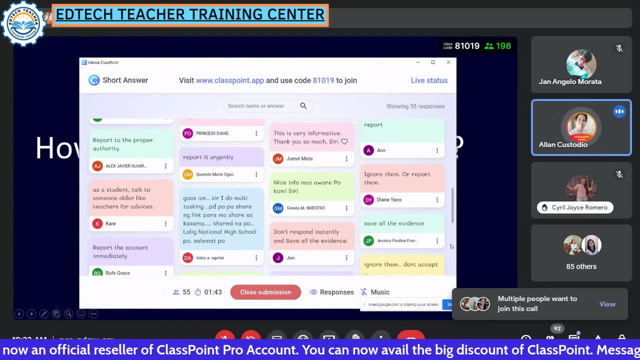 As a student talk to someone, Teacher po Advice. Ma'am Carrie, Balik po ako sa ignore and report Yung sa ignore. kung talagang gusto natin, talagang mabigyan ng leksyon, may mga bagay na hindi tayo makokontrol. Yun yung environment sa social media. 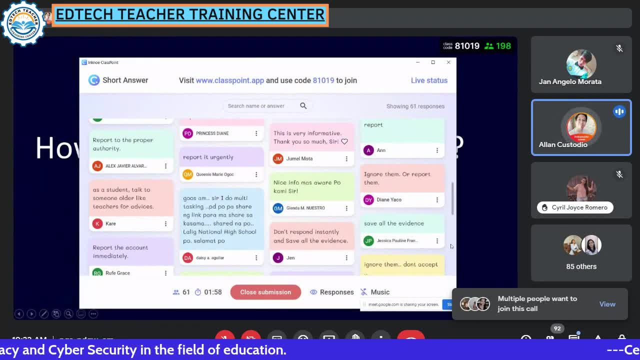 Sige, nga po, Kapag nag-scroll po ba kayo lahat po ba maganda makikita niyo sa social media? Diba hindi, And sometimes talaga nagre-report yun talaga iba eh. So kung talagang ano po Ako marami na rin ako na-report na kung ano-anong ano, Tapos parang hindi maganda eh Na-report ko, Bakit po. 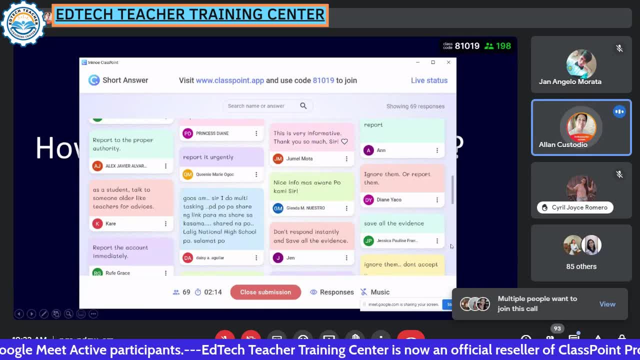 Kasi rights mo, kasi yun Ngayon. yung iba naman, kapag na-ignore ko na lang din. pero sometimes talaga kinakaya kong i-report Kasi para makabawas-bawas ng mga alam nyo na na hindi magandang pumupunta ng online, kasi kailangan natin yun. 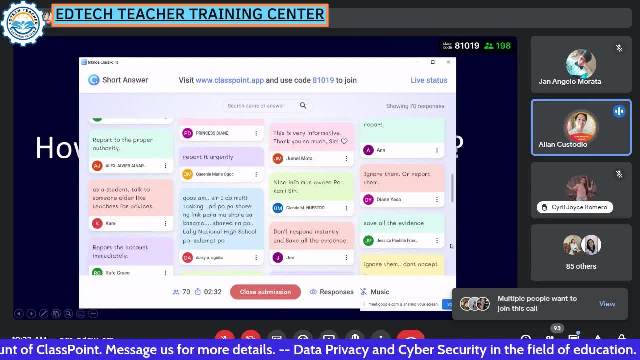 Thank you po sa ganitong wave kami. Thank you po no Di pa din nakapasok. Okay, Very useful po sa amin. Ma'am Maria Lea Angela. Okay, Mamaya, pupunta tayo magpakalalim Anong ika ka. 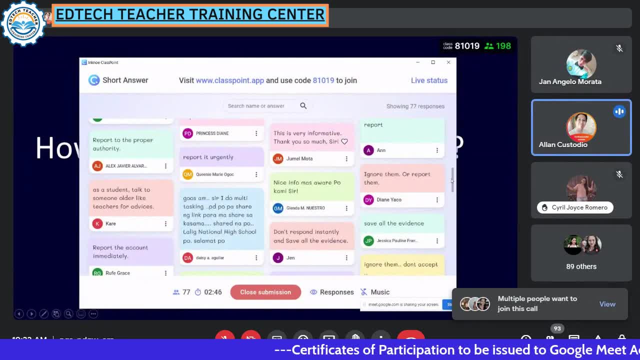 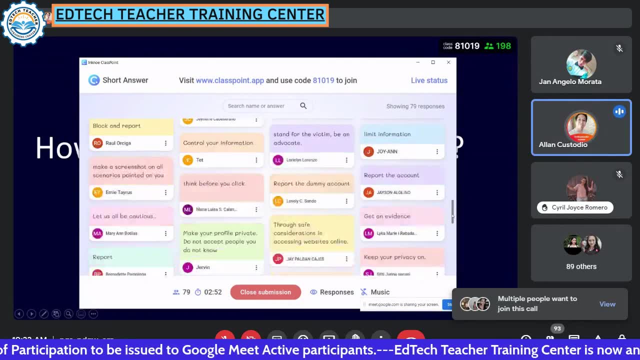 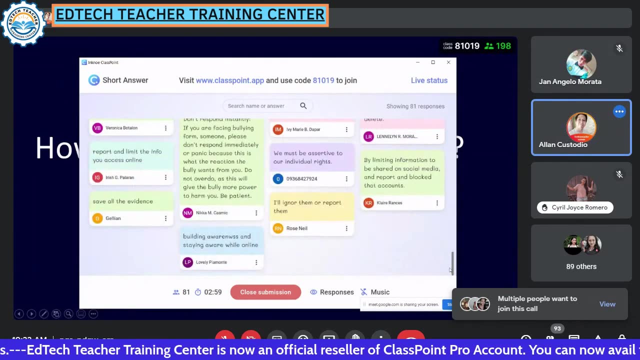 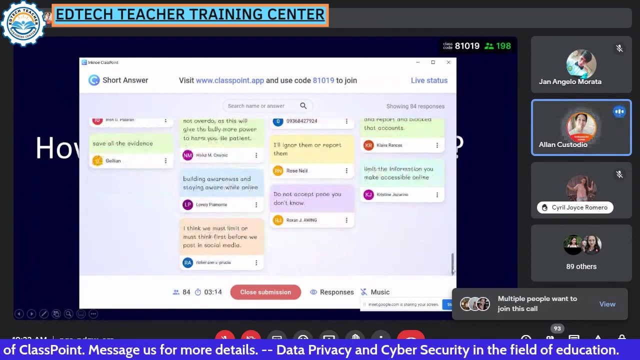 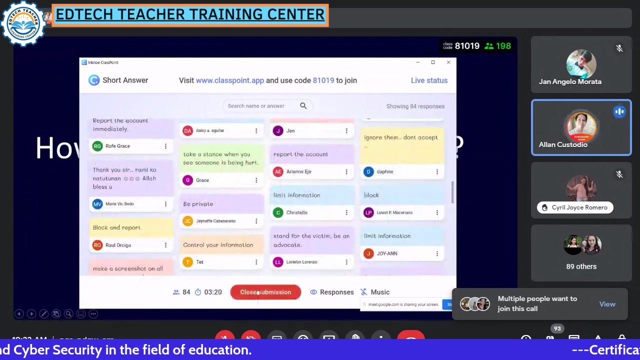 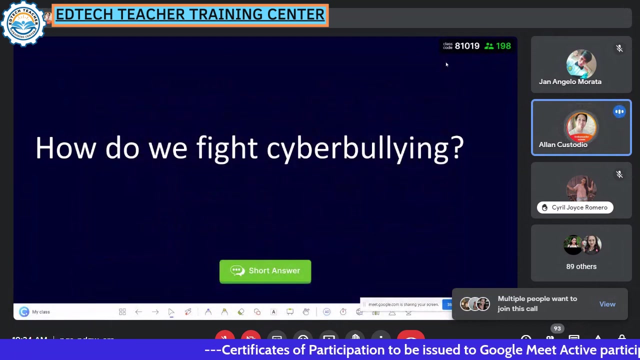 Okay, Okay. So lahat po yan ay tama, Kasi po yung number hindi po masyado talaga yung binabandera. Okay, Close po natin And award ko po kayo all-stars, So maganda po ang ating session. Puno ang class point natin, Puno po tayo no, And tuloy po tayo. Paano bang labanan. 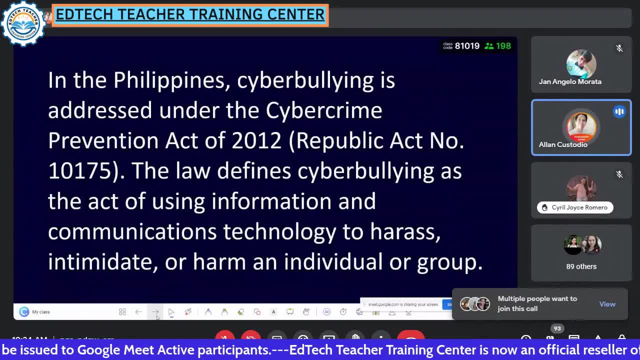 Sa Philippine cyberbullying. yung kanina po 173., This time 2012,, 175.. Hindi po sila nagkakalayo, no, And indicate to harm individual or group, Kahit group. yan individual ang hinaharm nyo. cyberbullying effective. Hanggang dito na lang, sa livestream, ang beauty natin. 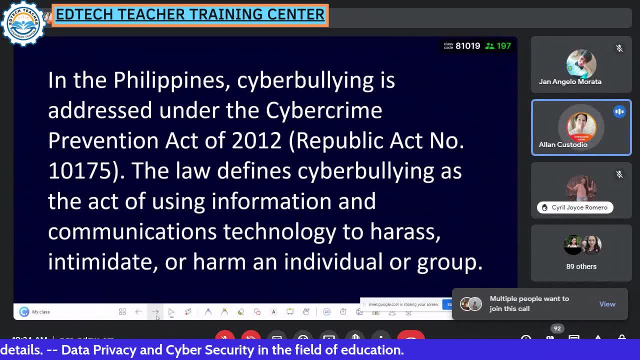 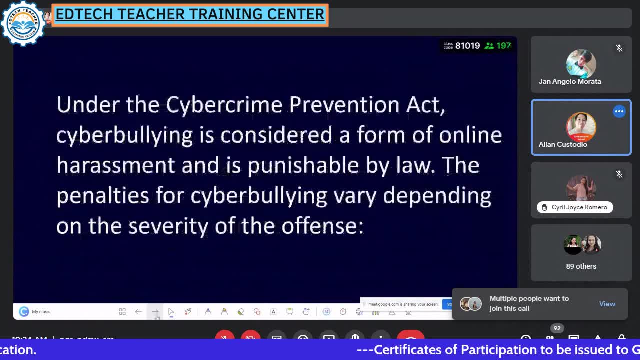 Ma'am Parthria, pasensya na po, ah, Nakalimit po kasi kami dun sa ano. pero kahit andito po kayo eh sulit ang inyong pakikinig Ayan Ngayon sa Under Security Prevention Act ang cyberbullying ay dalawang form. Marami po pala doon pag-ingat kayo Sa under security prevention act ang cyberbully ay dalawang form. Marami po pala doon kayo Sa under security prevention act ang cyberbully ay dalawang form. Marami po pala doon dalawang form. Marami po pala doon ay dalawang form. 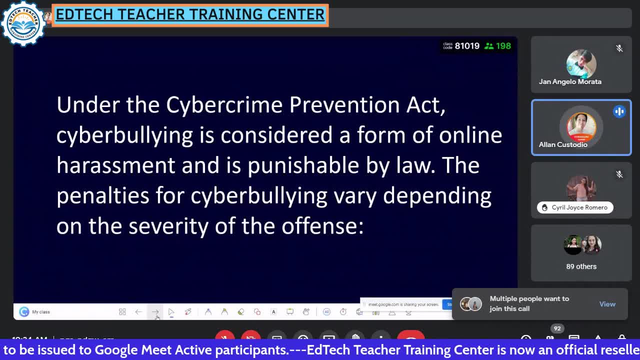 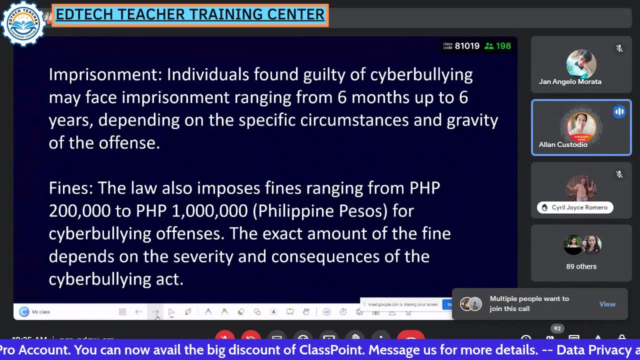 ding it on form nano. we have the online and physical. may verbal din tayo at marami pang iba den. and barring the, depend being on the severity of the offense, now imprisonment of six years kapag dinamin or the a dad at the pencil began, the pine is raging: 200,000 to 1 million Philippine pesos, the exact. 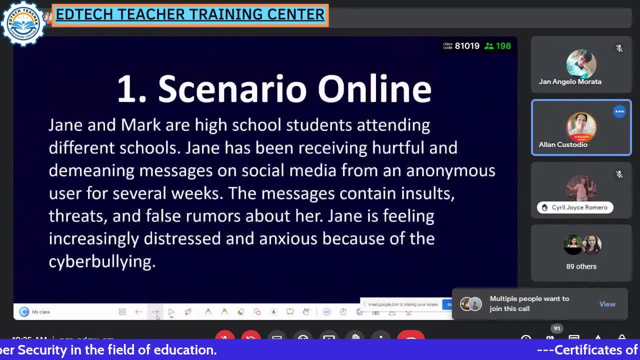 amount is depends on the severity. okay, scenario number one: cyberbullying seduction. CJ now at the mark. a high school student, the bank school. ngayon CJ nakareceive Shannon hurtful the meaning message. social media, the Hindi nakikilalang tao na nangangalang mark now nag message. 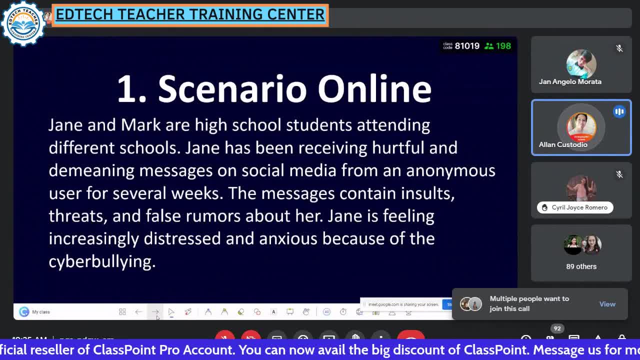 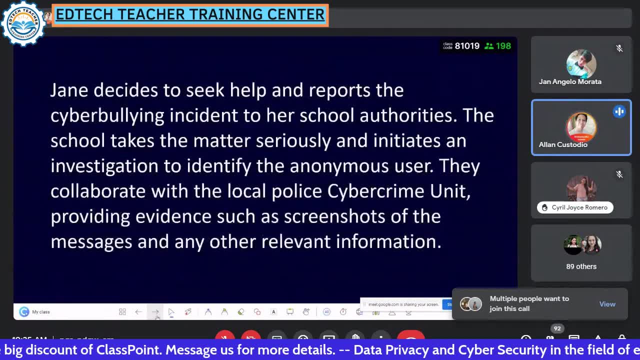 ng insult o kasi nungalingan at saka: talagang na is, talagang na is press, at the anxious na siya sa mga pangyayari na iyon. so, CJ, nagdesign siya na pumunta at tumulong sa dumulog, or nag ano siya, open siya sa teacher na. 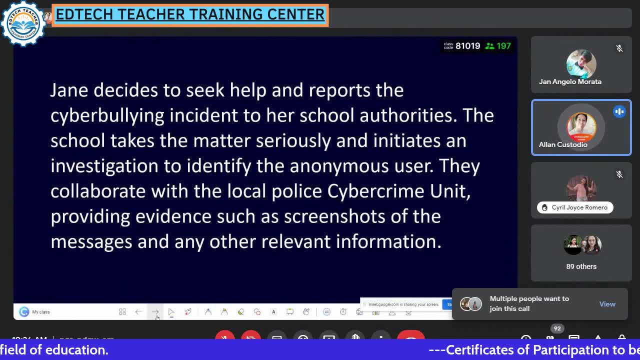 sinulungan siya at hindi mahinto talaga. kahit anong gamitin niyang number or kahit ano bang gamitin niya ay sinusundan siya. so nakipag-ugnayan na rin yung school sa cyber security unit or nireport na rin nila, pwede rin sa NPC. 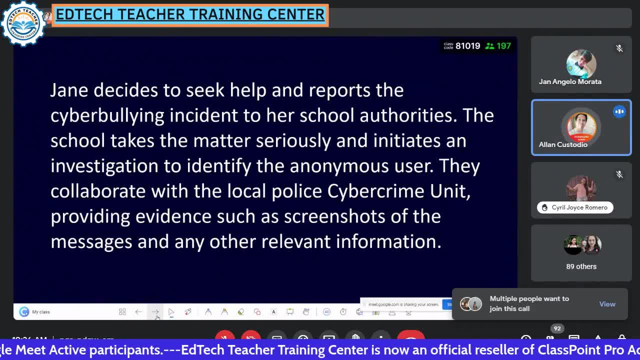 at may screenshot. si Jane, yan yung mahalaga may screenshot kah mabilis ka dapat diyan, kasi mag a-un-send diyang magagaling ng mga cyber bully act na yan. eh papabasa lang sayo na scene mo tapos. 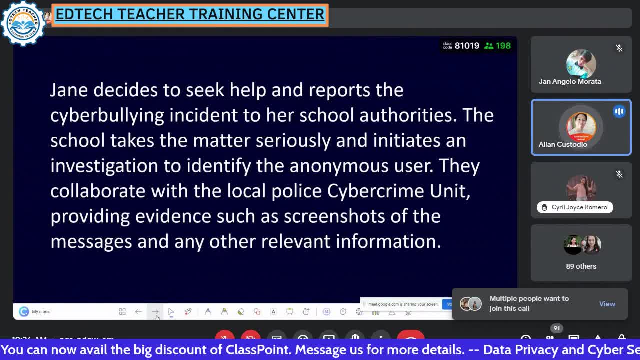 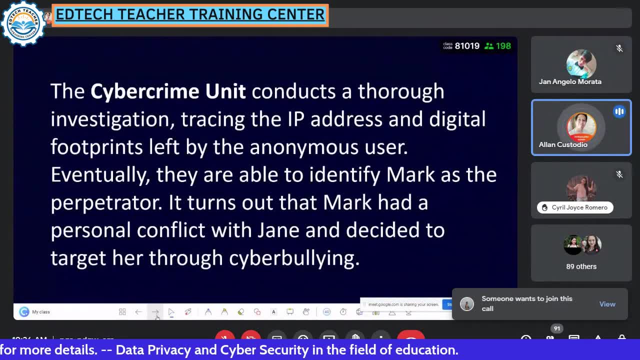 engines hinihintay nilang na machine mo sa baba, tapos UNCends katutulin. no, kaya ang gagawin mo mabilis ka ring mag-iscreenshot, pang- Grind out ng cybersecurity unit na nagconduct. 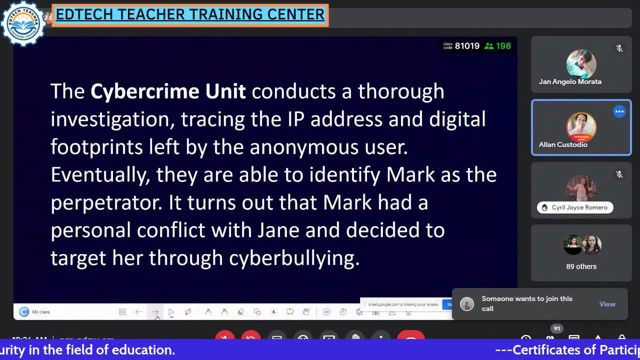 ng investigation, IP address nung tao na yon at eventualli si Mark, ngayon ang הזak Nung tao na yon At eventually ay si Martha, ngayon ay si Marq, ay si Mark. 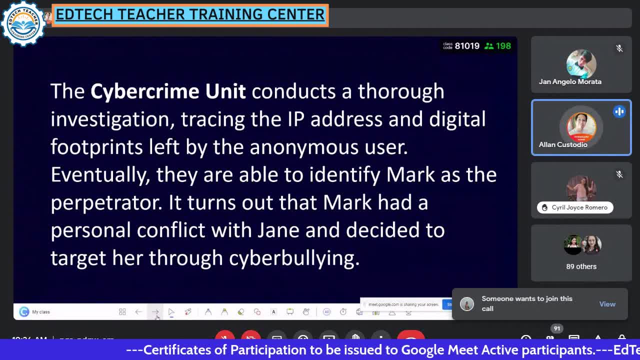 ang perpetrator, ayaw siya, yung utak talaga at sabi natin: siya lang mag-isa at dahil doon sa ginawa niya na hindi mahinto ang bullying, isang taon, siguro, ilang taong, tiniis ni. 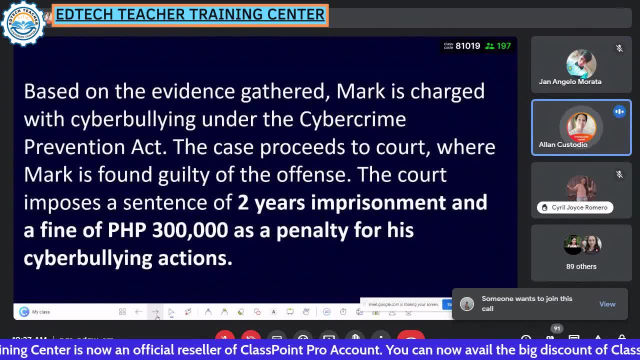 Jay na puro ganun na lang at hindi niya malaman ng mga account. ngayon na-detect siya ay dalawang taon na pagkakulong. Bakit po nakulong? Kasi may senior high eh 18 years old pa taas. 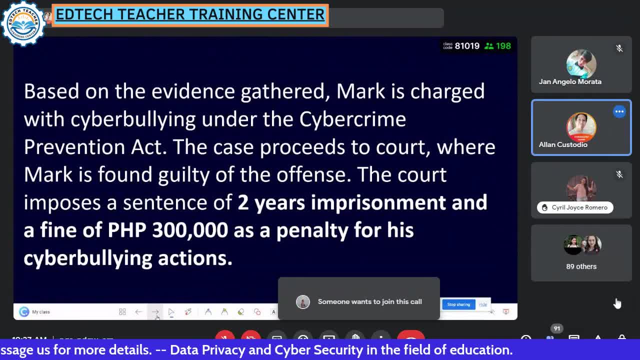 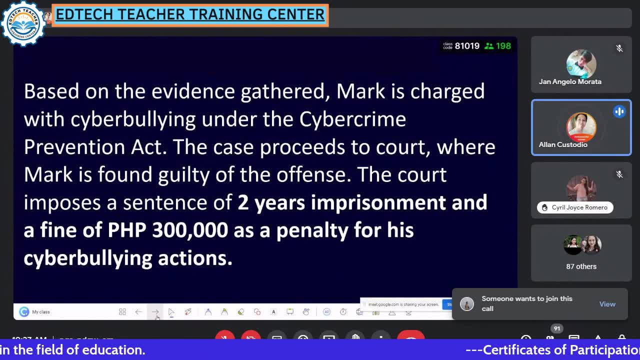 19 years old pa taas at marami ng hindi minor de edad sa high school. ang ibig sabihin ay pwede silang makulong, at pag nakulong sila ay pwede pa silang magmulta, at ang masakit ay 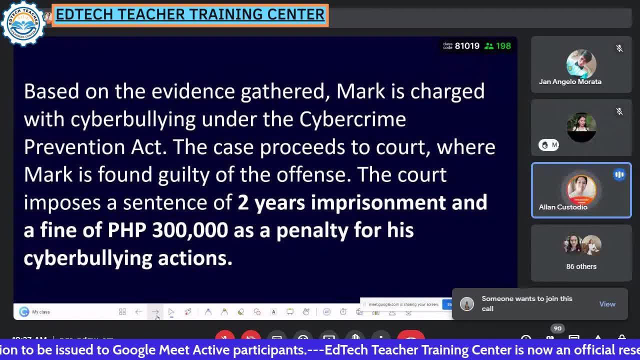 ang jurisdiction ng school ay hindi pinapayagan ng unethical at pwede silang i-kick out or pwede silang mababa na yung kick, mababa nga po yung suspension and detention. kick out po yan, kasi napatunayan din eh. 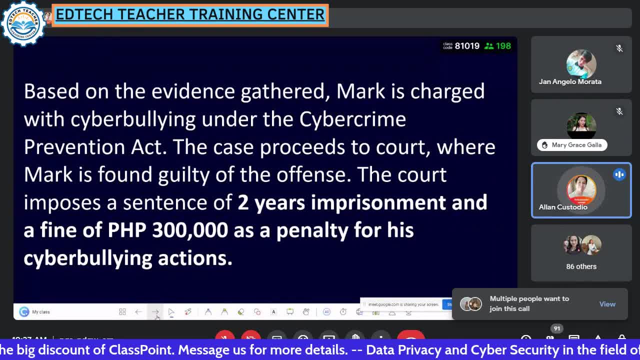 and sometimes talaga kapag hindi yan, at talagang kapag yan ay na-tolerate, I mean pag na-tolerate po yan ulit-ulitin lang ng kahit sino. Eh, ako hindi naman. ako nahuhuli, dyan, wala naman saking. 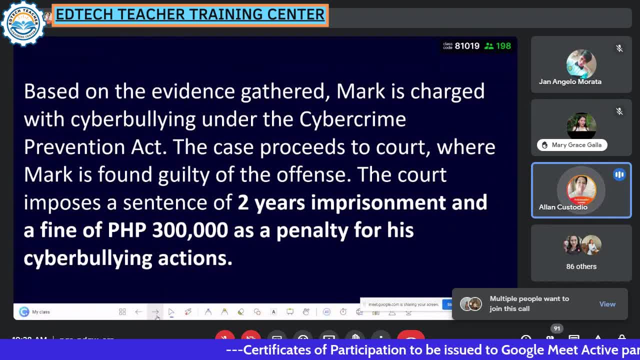 bumabangga dyan. eh padar ako. eh sige nga, tubo ka nilang hanapin. marami kong dami account Ngayon nagcha-change ako ng IP address. sige nga Imaginin kung may onting alam yung bata. 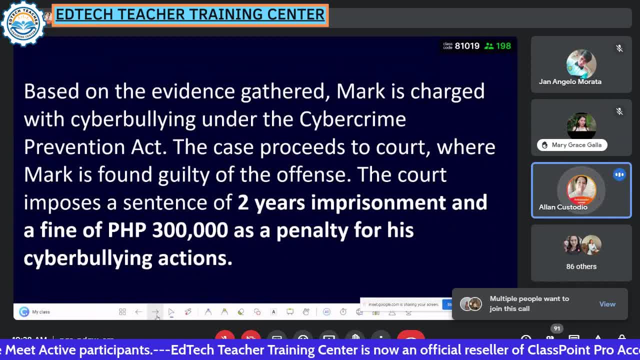 sa ICT. kung gano'n siya kalakas, Kung gano'n siya kalakas, mambuli ng kasama niya, eh binubuli ko. wala naman siyang alam, eh kilala ba niya ako. 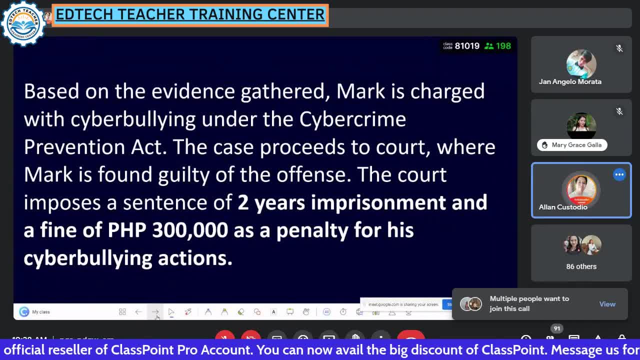 Ganito, Eh trip lang natin. eh nakita ko lang kasi pangit kasi siya. eh Eh nakita ko sa intramurals, gusto ko lang pagtripan. eh Nakita ko pa yung pangalan niya sa ID. 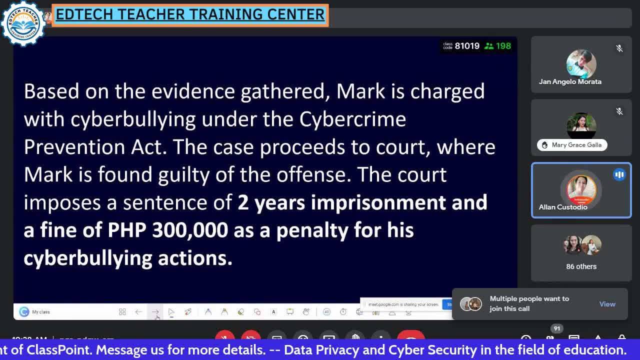 Okay, Andaming pwedeng mangyari. eh kaya, pag hindi nilabanan niyang mga salbahe na yan, wala Hindi sila masasampulan. So eto, sabihin nyo po, eto yung batas na yan. 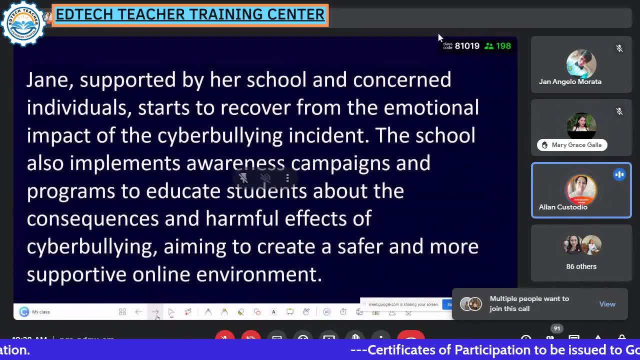 at yan ay effective. Now si Jane ay sinoportahan ng school at nakarecover siya. Siyempre, alam naman natin na may child protection policy ang school, kasama yung cyberbully diyan, Hindi yan tinotolerate. 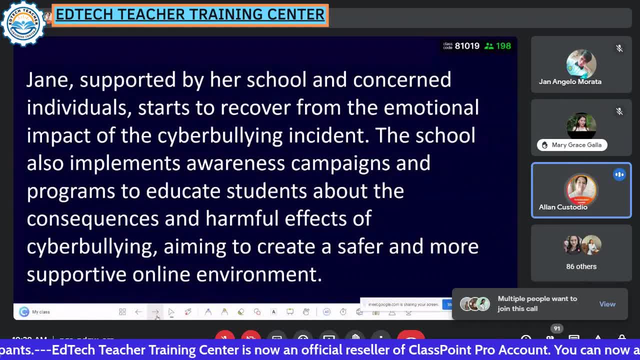 At dapat ay nilalabanan yan. Ngayon yung school nagkondak na mga refreshment. wag gagawin, Kasi kahihin din naman ng kabilang school na may estudyante. silang ganon Kaya sa. 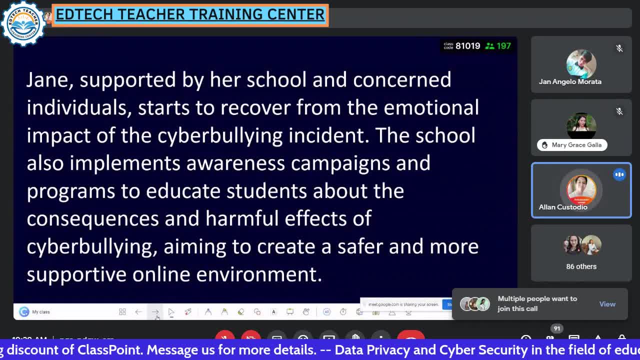 jurisdiction ng school policy. i-kick out yun Paalisin, Kasi pag pinanatili nila yun ay malalaman na na mababa ang anilang tolerance sa ganong klaseng bullying na. 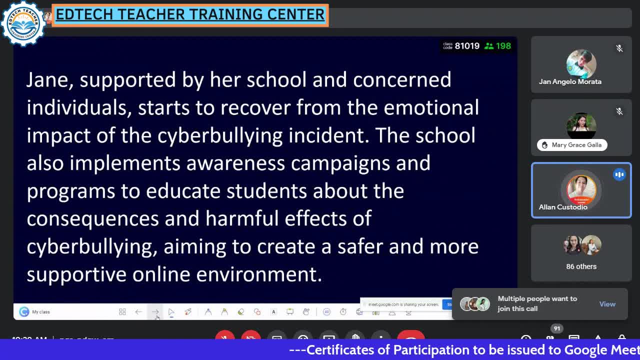 continuous pala at talagang ayotigilan ni Mark. Sometimes kasi po minsan may warning, Pero it depends upon kasi sa bata May nagpapakamatay nga po ng bullying, di ba. 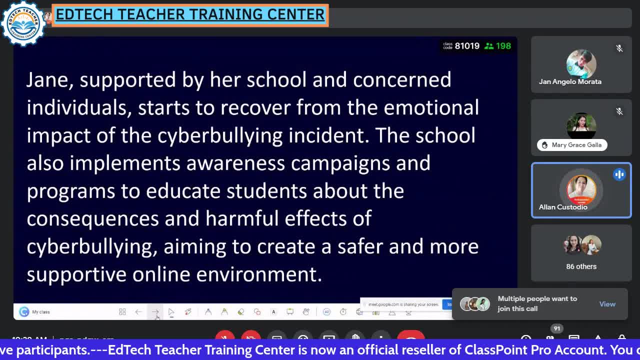 Tagot nga po kayo ng number number one. kung may nagpapakamatay sa bullying, cyberbullying, Meron po ba kayong nabalitaan. nagpapakamatay sa bullying sa mga balita, Di ba po meron. 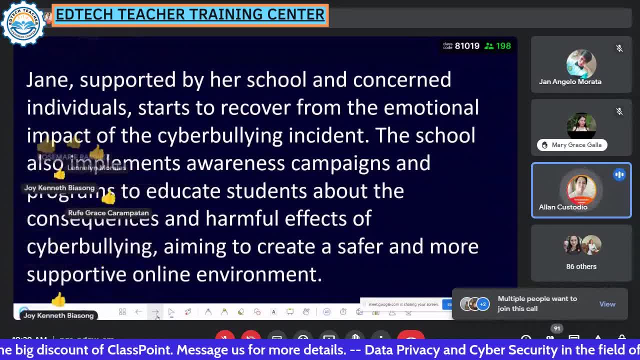 Kasi hindi nila makaya. eh, Ngayon hindi nila makaya. Walang mapag-openan yung bata, Wala silang matakbuhan, Hindi makapag-open sa hiya na hindi nila masolusyonan. 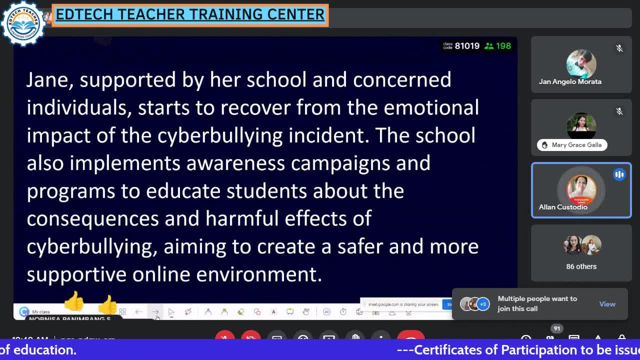 Nagpakamatay na yung mga nabully ka Ang nakakalungkot. eh ano ang daming pangarap na sasayang dahil sa mga perwisyong, mga bully na dapat ay hindi, yun hindi. 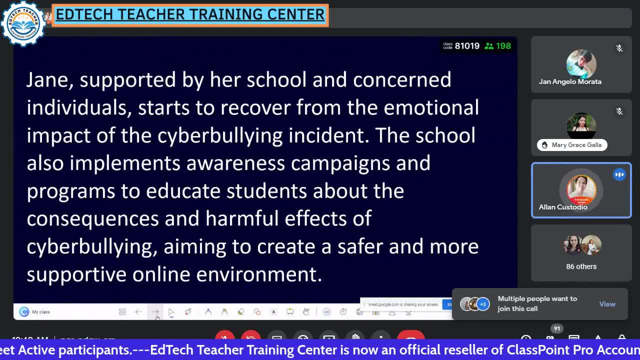 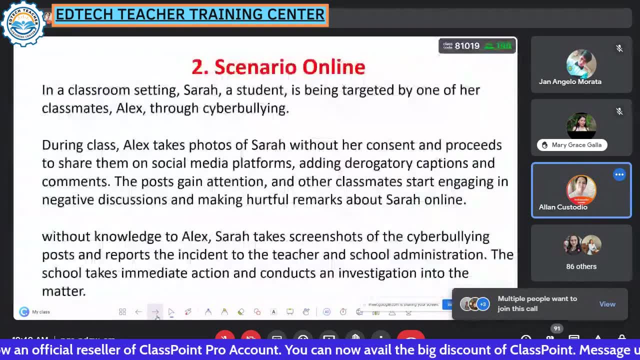 tinotolerate yung mga yan. Okay, tuloy po tayo. Nakakagigil yung mga perwisyong na ganyang tao. Okay, Senaryo sa online Tuloy lang na lang po tayo. 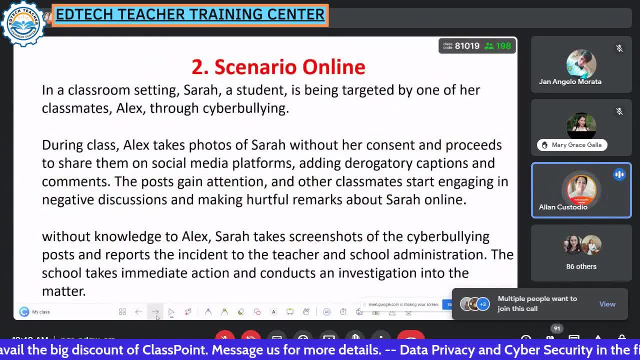 Ito naman po yung under 18.. Ngayon pwede pong maging DSWD. Si Alex daw ay nag-take ng foto ni Sarah ng Without the Consent. May platform sila na ginamit na social media, Facebook or what? 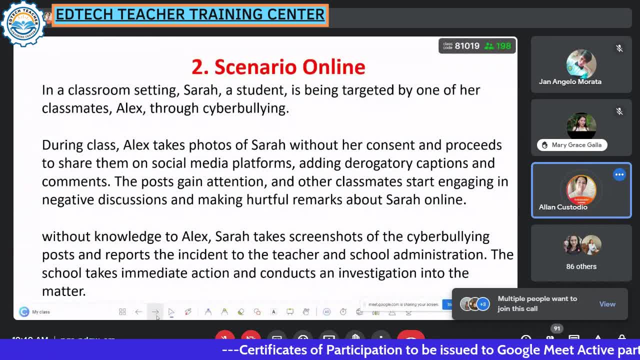 at nag-adding ng derogatory caption. Thank you po sa lahat ng number one: Sobrang dispresyon din po yan Correct, Ma'am Lorendo, ba to Shout out sa'yo, Ma'am Ngayon, tignan niyo tong. 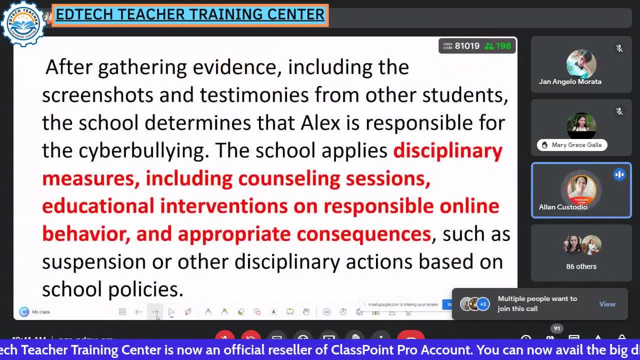 pangalawang senaryo natin. Ito hindi ko maintindihan sa kabataan Dito ibain ko ng konti example, pero siya rin Ito. to Sino po ba dito taking for granted kapag nag-birthday yung isang kasama niya? 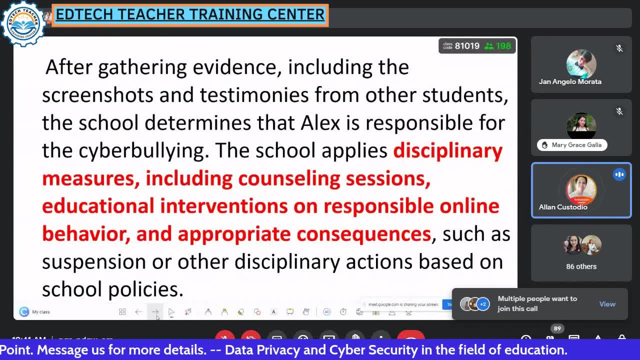 pinipicturan talaga niya naglaway. tapos eto, kilala ka na, sikat ka na, ngayon naglaway, pangit yung mukha mo, or something like that, tapos ipopost nila. 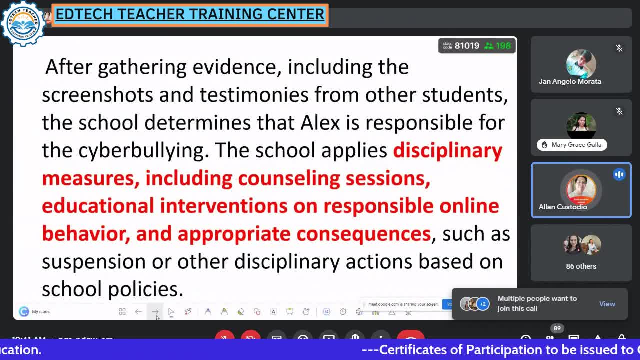 sa Facebook. Ano po ang dating nun sa taong pinag-postan Sir, okay lang, Bestfriend naman kami, eh. Tapos may caption na derogatory ganito: huling pamumuhay na niya sa mundo. 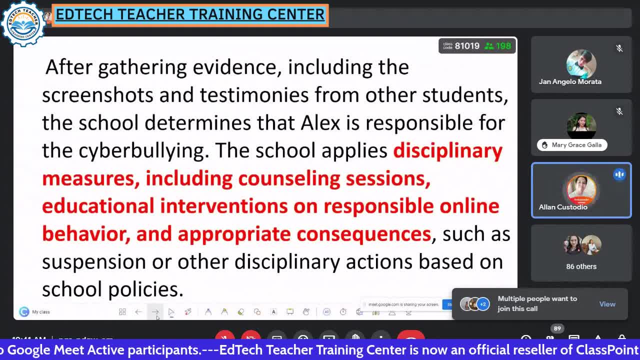 20th birthday. 21st birthday: BFF ko, Bestfriend ng bata sa high school, Yung sinasabi ko po ba na to ay may point sa privacy ng bata Napakalaki. nun Tignan niyo po ah. 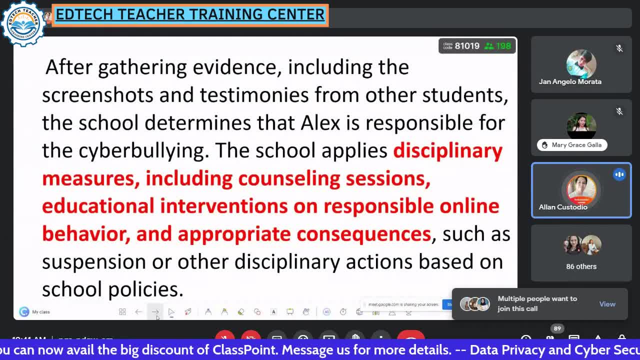 yung mga bata Ako inuorient ko, mga estudyante ko, Huwag niyong gagawin sa kapwa niyo yun na lalo. wala siyang permission Nakatulog sa pagod Yung mga empleyado. 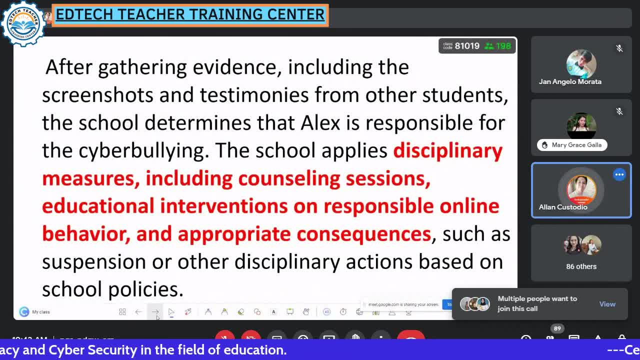 sa government. diba nakatulog tayo Minsan. totoo eh, nakatulog ko sa pagod. eh ngayon nilikturan ka tapos birthday mo daw, so ineditan ka pa nung pagmamukha mo. 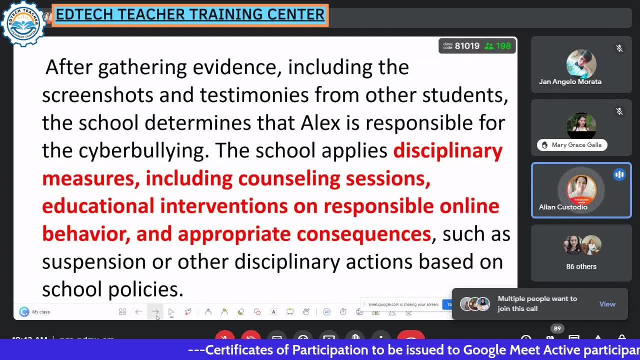 tas, eto na ang pinakamasipag naming empleyado. Parang andating eh, tamad ka eh, Pero sa pagod mo lang nakaigblip ka, Tapos binati ka ng happy birthday. Pwede ba yun? 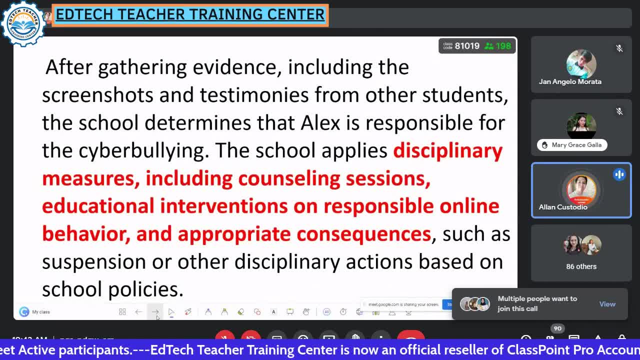 Pwede ba yung ganong bagay? Ay, hindi po pwede yung ganyang bagay. Pwede mo siyang anuhan dyan, Kumabigat dyan at naperwisyo ka. pwede yung ireklamo sa? 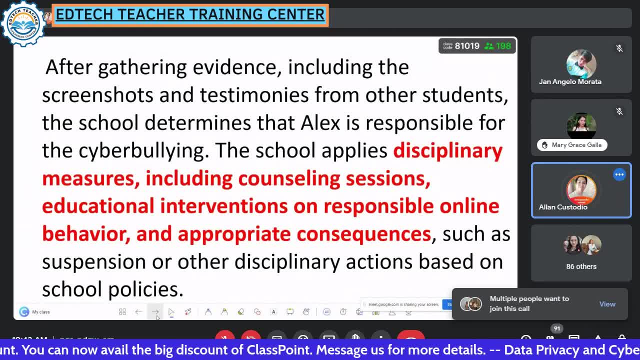 NPC At tignan ko lang, kapag nakita talaga ng NPC, lagi nyo tong tandaan po or talaga naireklamo sa school guidance po yan. Disciplinary action, yan Ayun o disciplinary action, hindi yan. 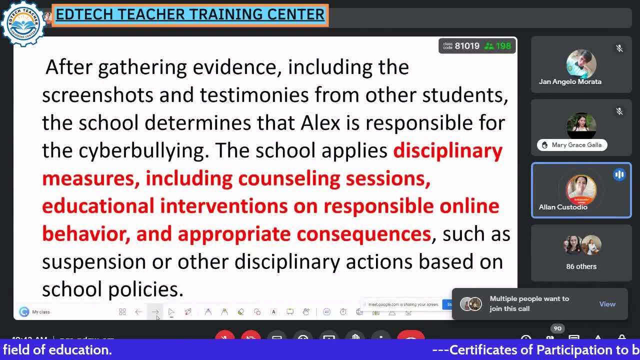 pinagbibig yan. Imaginin may tao na lang sayo bibiglang gaganon porkit birthday mo. O wag niyang bibihin Ang sinasabi ko, lagi yun, eh, Wag niyang bibihin. 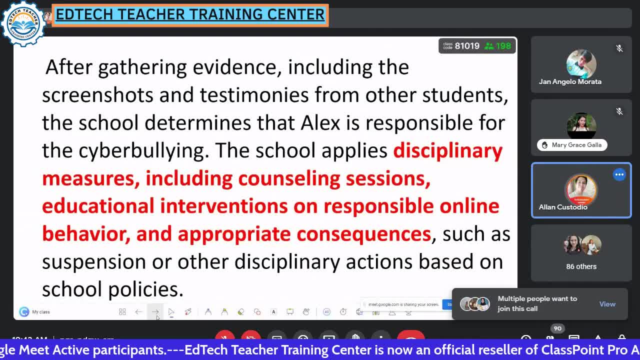 yung mga close nyo, Alam nila ang limitation mo. Kung totoo kang kaibigan sa kanya at totoo siyang kaibigan sa'yo, ire-respeto ka niya, birthday mo, man o hindi mo. 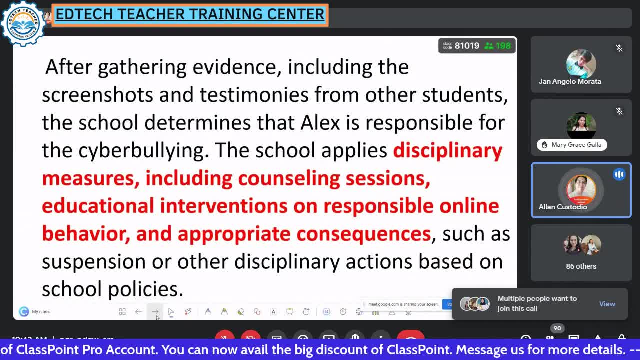 birthday hindi ka niya pagsasamantalahan. Naniniwala po ba kayo Hindi mahalagang maraming kaibigan. Ang mahalaga ay meron kang totoong mga kaibigan, Ang totoong mga kaibigan. 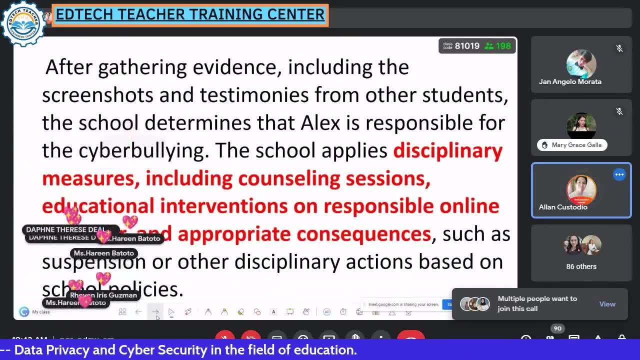 yan ang magtatanggol sa'yo at ire-respeto ka, Andami mong mga kaibigan, dinirespect ka, dinirespect kung ano-anong sinabi at kung ano-ano na lang, Eh, tasasabing sa'yo. 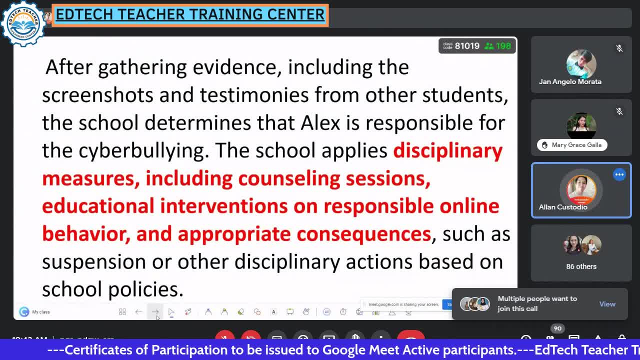 friend naman tayo. eh Diba, okay lang sa'yo yun Anong, okay lang yun. Hindi totoong okay yun, Dahil hindi ka nalang nagsalita. eh, Eh, diba, Ang sabi nga nila. 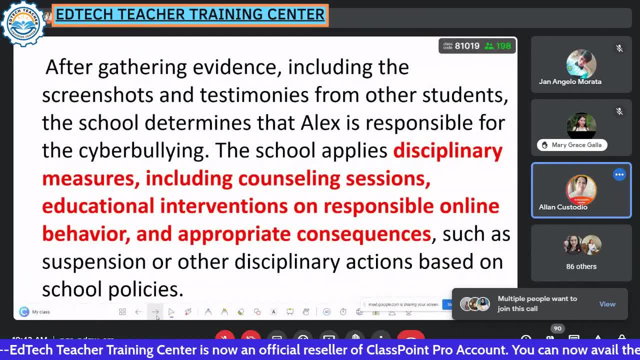 yan nga eh, Quality friend is better than quantity friend. Lalo na, kapag hindi yun nakakaintindi sa'yo O kita niya maraming nagtutro eh, Quality over quantity correct. Kahit lima lang yan. 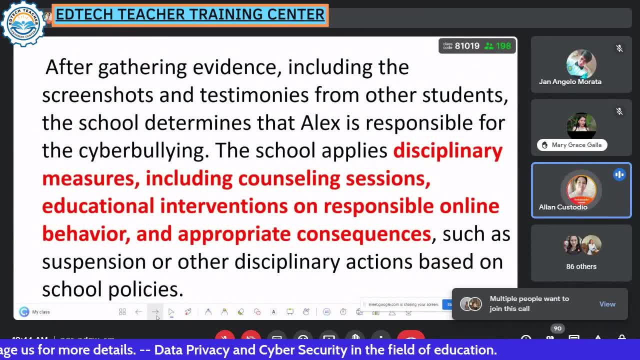 Eh yung lima naman na yun talagang hindi ka talaga susukuan at alam nila yung hindi dapat gawin sa'yo. Yun na ang kayamanan mo sa mga kaibigan, Huwag nyo silang. 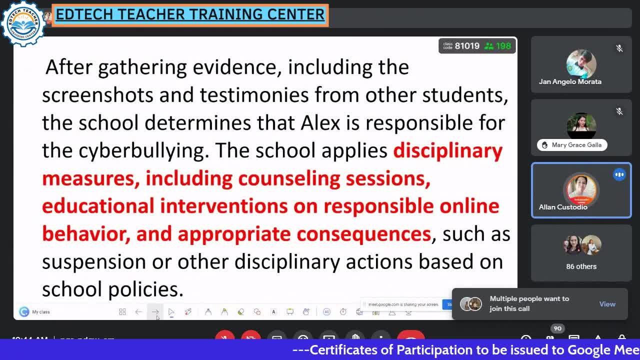 ah, idadawn yung mga kaibigan ganyan. Piliin nyo silang mabuti sa buhay. Ang pagpili ng friend sa social media ay option, Hindi yan sinasabi nila: oh konti ng friends mo, Hindi po. 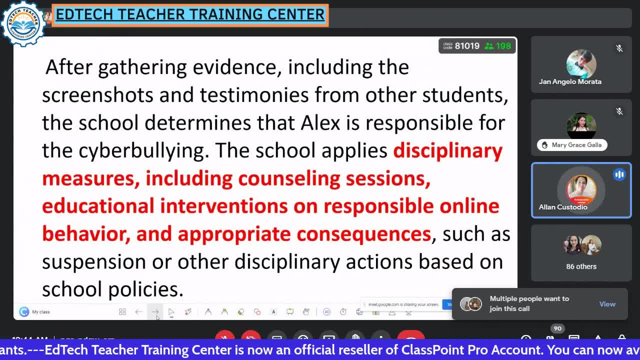 dun yun. Ang point dito is: kung may healthy environment ka sa social media, Gusto mo ba lagi nakikita mo sa social media yung mga kaibigan mo? Iba puro toxic yung post Karapatan mo rin. 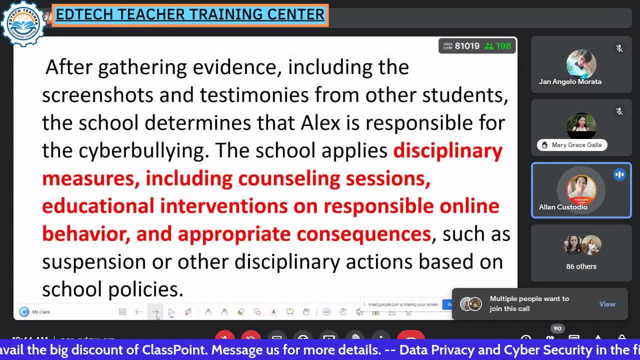 mag-unfriend or friend Mag-black Tatlo yung karapatan na yun. Pero may mga ano dun Ibat-ibang klaseng ah, ah, pangalan nito. Dahilan na lang. Pwede ka mag-unfriend, Pwede ka. 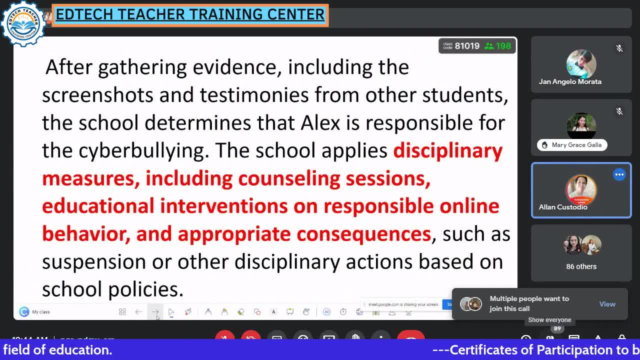 mag-friend. Pwede ka mag-request, Pwede ka mag-cancel ng request. Lahat ng yan ay kapangyarihan mo At hindi ka dyan makokontrol ng ibang tao At pag nagpakontrol. 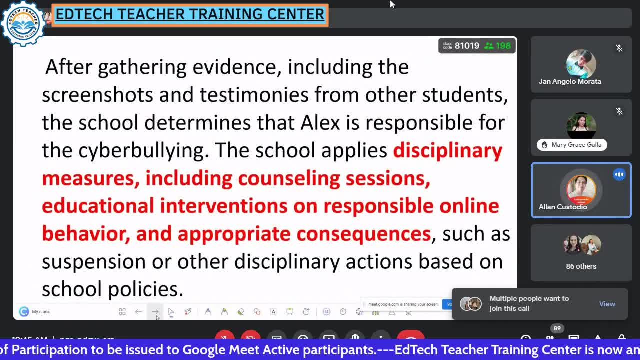 ka dyan uy kaibigan, pwede kang tumanggap ng suggestion, But the last of all option para maging kaibigan mo, yung mga taong gusto mong i-friend ay nasa sayo O yan, Madami? 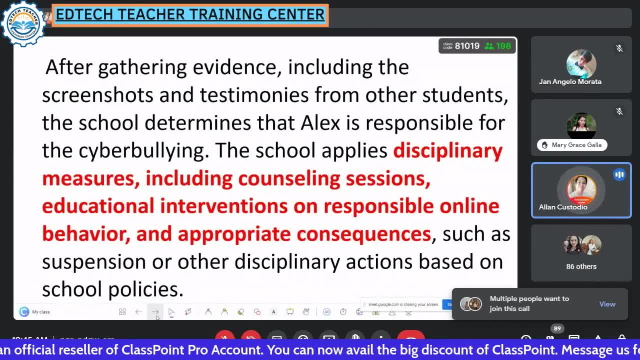 po ako na black na unfriend, Ganun talaga Ma'am Shane correct O yan- na magiging peace of mind. Naniniwala po ba kayo ang peace of mind ay kailangan? pangalagaan Number two. 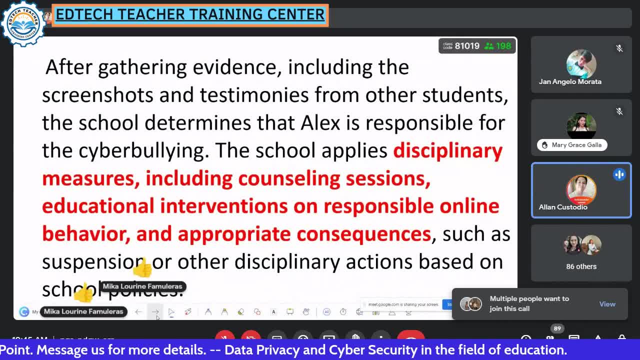 Set nga tayo ng number two. Yes, tumpak, Unfriend ko talaga yung mga friends na toxic, na Correct, Nasa sa inyo. yun Set nga kayo number two. Kailangan pangalagaan. 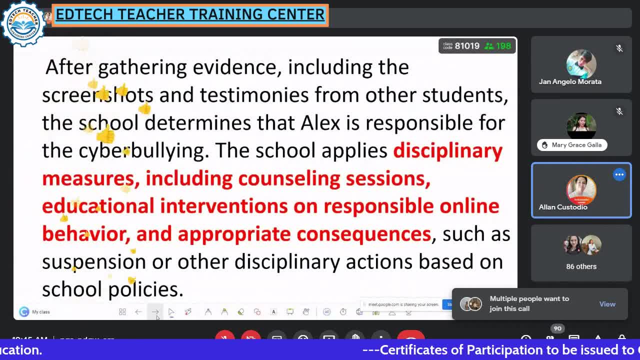 yung peace of mind. Hmm, Okay, So sa pagpapatuloy natin, o ayan, Ma'am Juby, pinapangalagaan ng peace of mind, Napakahalaga niyang peace of mind na yan. 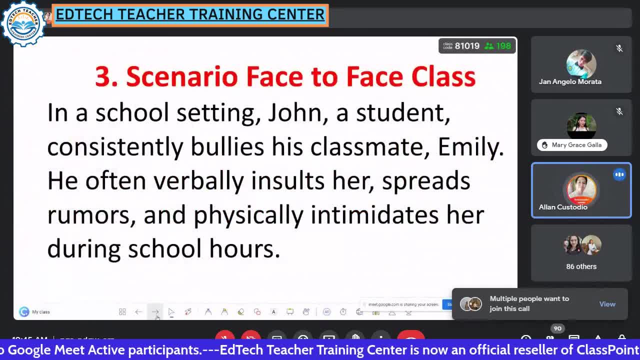 Okay, So dito balik tayo sa topic. So time check natin 10.45.. Dito sa senaryo na yun ang nangyari. pwedeng si Alex ay makounseling intervention. 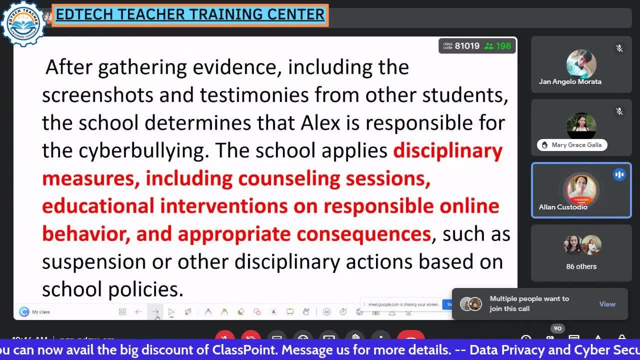 at kung ano-ano pa Kasi nag-post siya ng picture na hindi maganda. Nagreklamo si Sarah na kung ano-anong pinasta kanya at hindi niya nagustuhan, So pwede siyang. 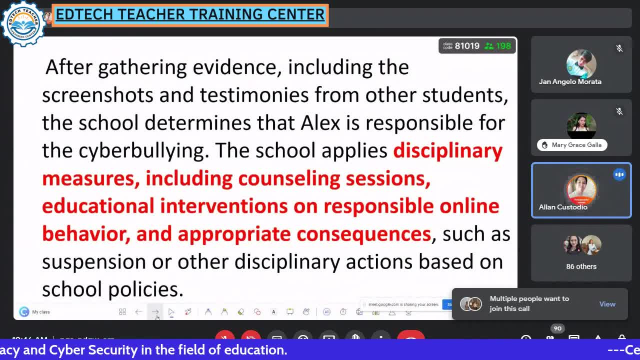 i-guidance talaga dyan, or sa teacher muna, para hindi ma-bypass. Eh ayaw talagang paawat ni Sarah, Gusto siyang bigyan ng warning in-guidance, So pwede rin naman makausap yung parehong both. 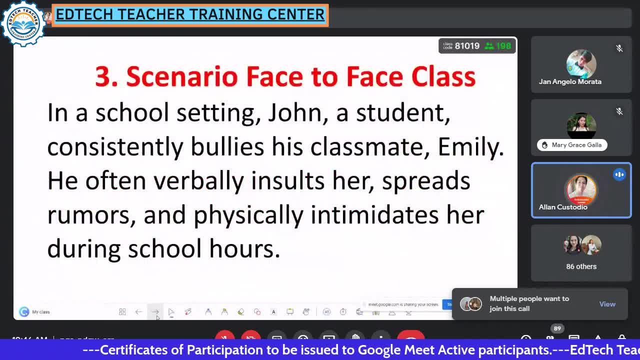 parties, yung magulang Diba. Tama po ba Ngayon ang senaryo naman dito face-to-face, So sa face-to-face may physical na nangyari, intimidate rumors Ngayon. 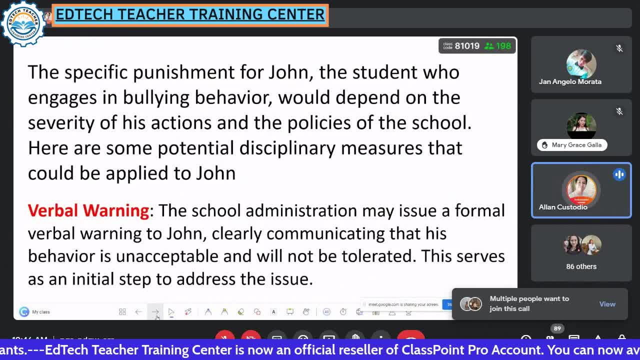 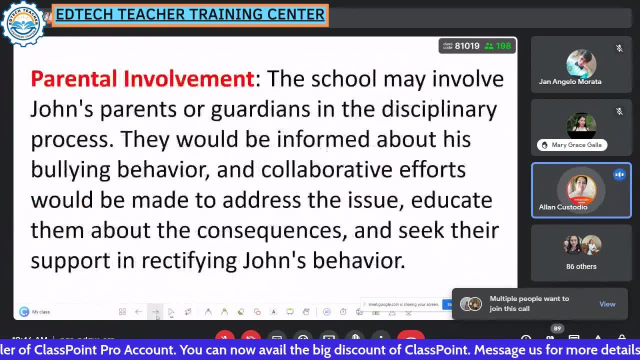 hindi sila ano. eh, minor de edad sila. eh 11 years old, sabi natin na to grade 7-8.. 14 years old, 13. Ay, verbal warning ginawa dito sa bata, Si dyan naman pinatawag. 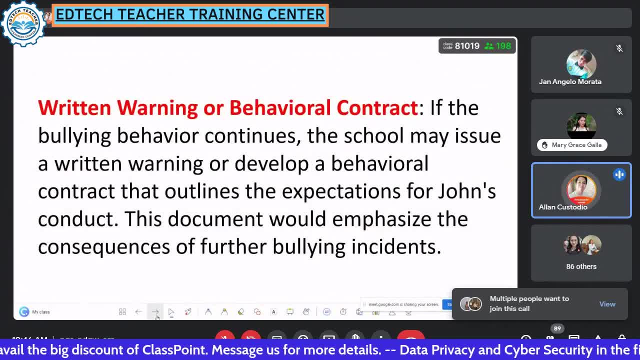 yung kanyang parent Tapos gumawa ng written warning or behavioral contract. Nangangako po ako na hindi ko nauulitin Lagi nang ganun po yun sa guidance. Diba po So kailangan. 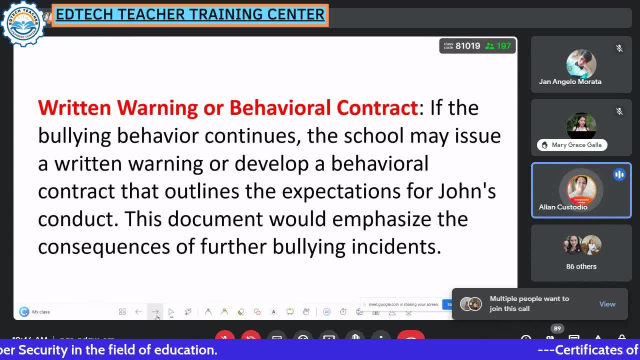 nilang tumupad doon. kasi pag hindi based on the school policy or the jurisdiction of the school, depending upon how many act na ginawa nung bata at pag umabot siya ng ikatlo, ang alam ko is kick out. 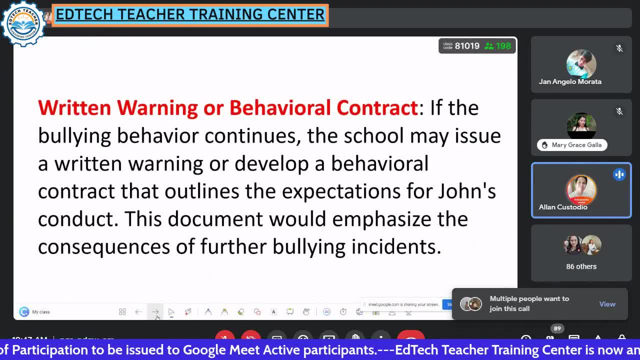 Warning, pwede rin na community service. Ang community service usually ng school: maglilinis ka sa loob ng school. Yun po yung sinasabi doon. para maano mo, matandaan mo yung ginawa mo: maglinis ka. 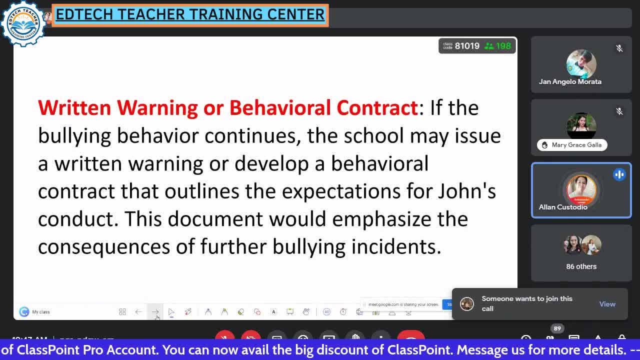 ng school, para rin siguro makatulong ka na rin. Tapos, yung iba naman na ginagawa kapag huli na talag kick out, Depende sa bigat ng ginawa mo. Okay, next natin. 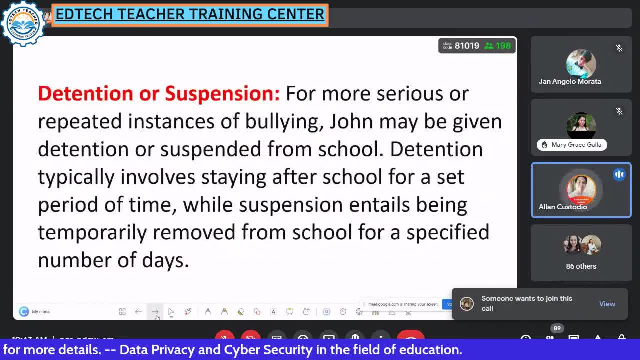 Detention, suspension, Pwede ka suspindihin ng ilang araw, 30 days, ka Magmodule ka muna Mag-reflect ka kung ano ginawa mo Talagang gano'n hindi ka mapigil. 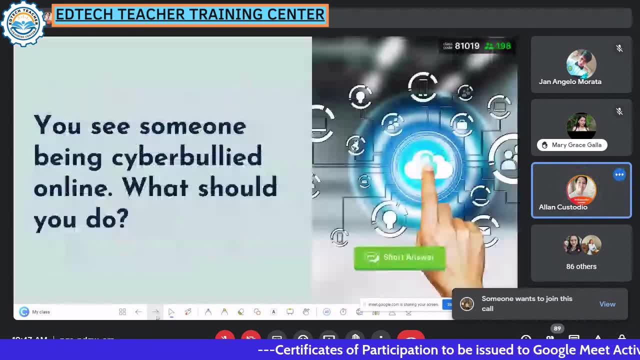 Okay, may mga ganyan Ngayon may cyberbully, tuloy na lang po tayo. time check natin: 10.47.. May nakita kang cyberbully na bullied online Ang dapat gawin. puno pa rin po tayo. 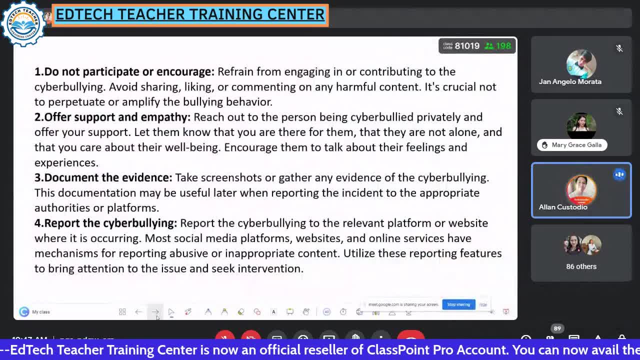 sa group chat Number one. huwag ka makikipag-participate doon Kapag tinarget ka ng masyadong buwisit itong isang to di ka namang kasali sabi ng bully to. 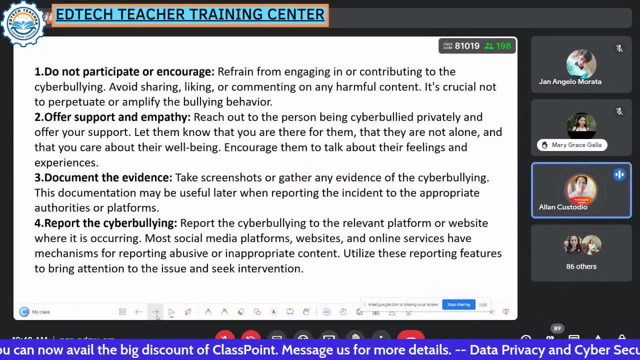 isasama na kita Lagi nyong tandaan. pag nakisama ka sa isang gulo, nakisausaw ka, kasali ka na Kaya yung mga nakikipag- parentess dyan hindi naman kasali doon. 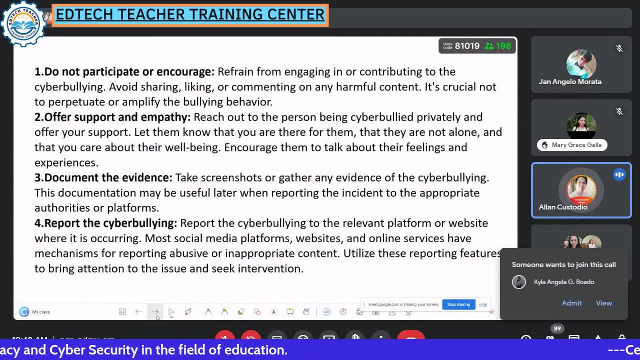 at hindi nyo alam yung tunay na kwento. ay: huwag ka nang mag-comment, Pero may kapangyarihan ka rin namang mag-comment kung gusto mo. Tandaan mo lang na handa ka. 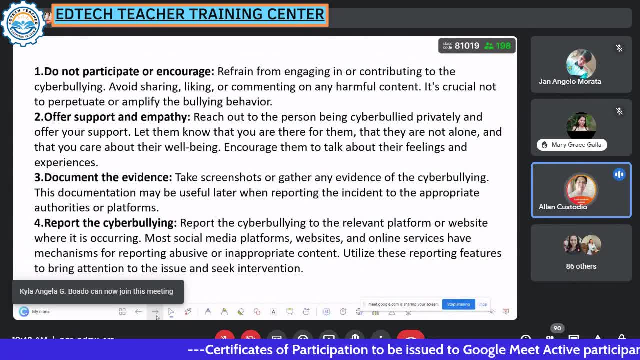 sa consequence na magbabato sa'yo doon At baka kinabukasan ipinost ka na Etong nagko- comment na to masyadong pabina, ikaw na isusunod nila. 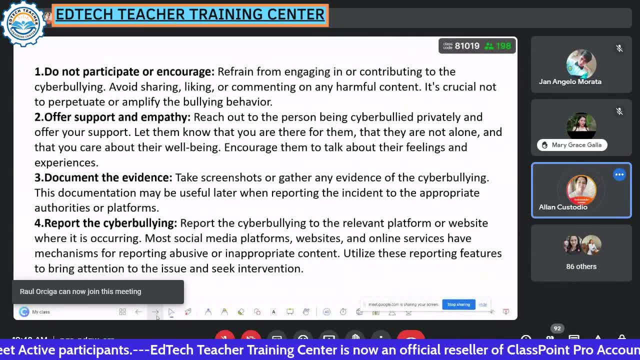 Lagi mong tatandaan yun, Pwede ka naman kasi mag-report. Lagi nyong tandaan na kung ano ang papasok ninyo ay handa kayo, accountable kayo at responsible Lalo sa. 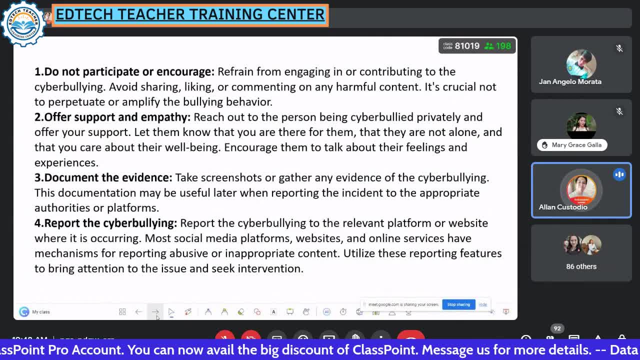 may bullying na sitwasyon O diba alam nyo na may issue May ora At saka yung issue doon sa bar. Wala akong sasabihin. ha, Ang dami doon nung nag-check ako. 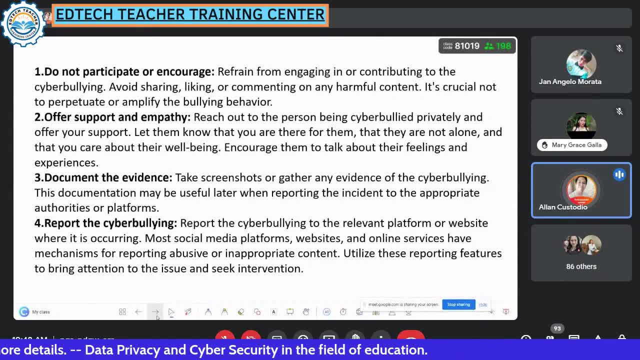 ng comment na kung di naman talaga kasali, dapat doon. andun Nag-uubos ng oras doon at ang nakakalungkot ay karamihan nga talaga. yes, may pakailam tayo sa issue. 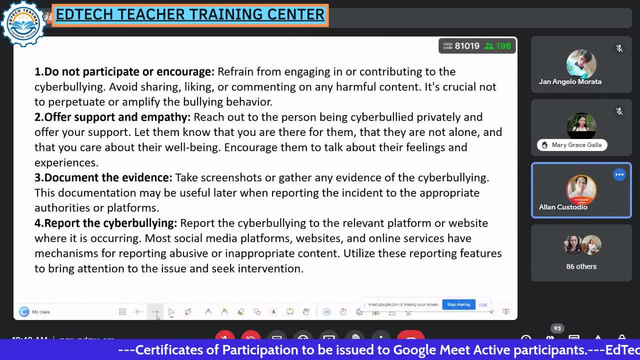 Pero yung iba doon talagang unrelevante. Eh gawang ko ba Yung iba pa bully type pa Nakakalungkot lang yung comment section. minsan talaga Okay, Okay. 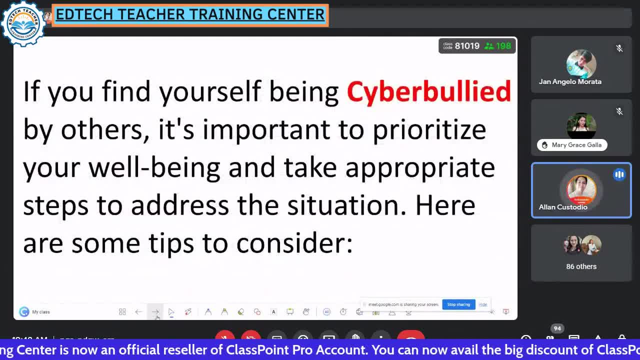 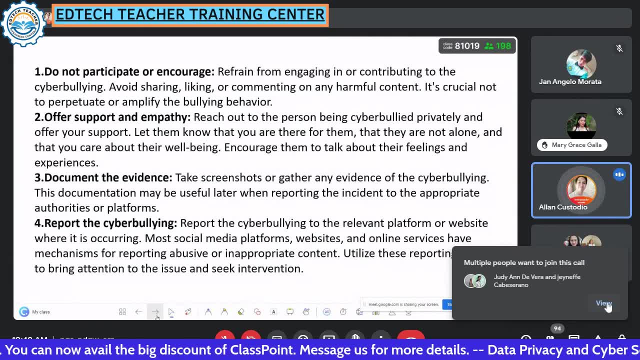 Alam ko narami kayong, sana narami kayong natututunan Tuloy tayo Hindi Punta tayo dito sa offer support empathy document evidence. Ayan Bago kayo mag-report kay Facebook. 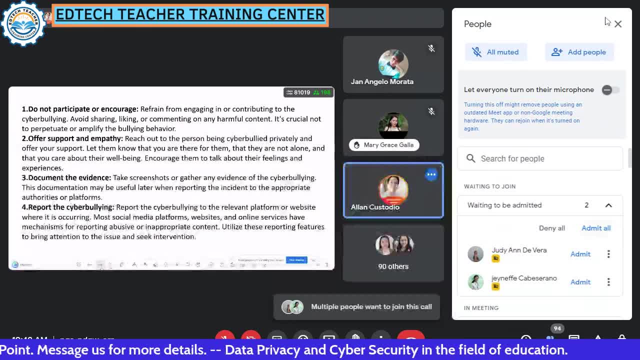 i-screenshot nyo, saka kayo magsasend ng screenshot. Ganun na po si Facebook, Hindi na po basta yung dahi-dahilan lang. Kailangan mo mag-screenshot, magsend sa kanila. 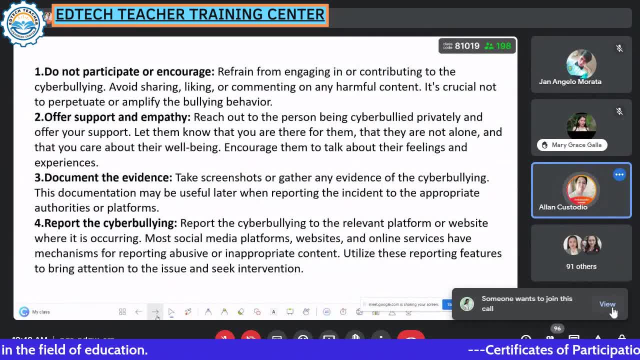 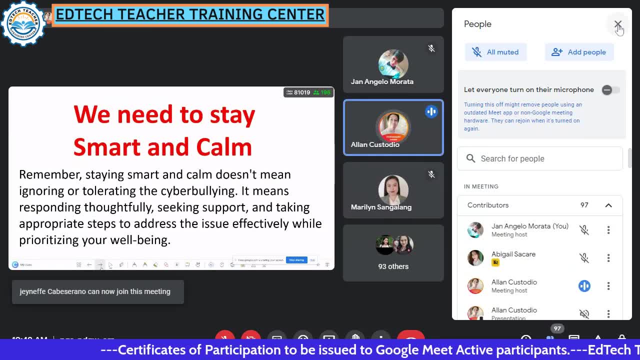 Okay, Thank you. thank you sa mga umaaten Report, cyberbullying Report nyo. Okay, Yung mga na cyberbullying. eto mahirap tong gawin, Pero eto dapat gawin, Kasi sino ba naman hindi gagante. 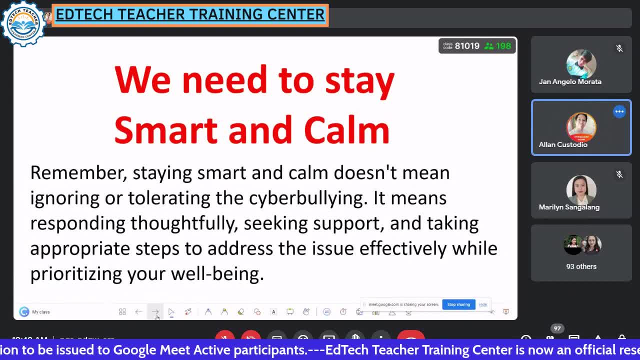 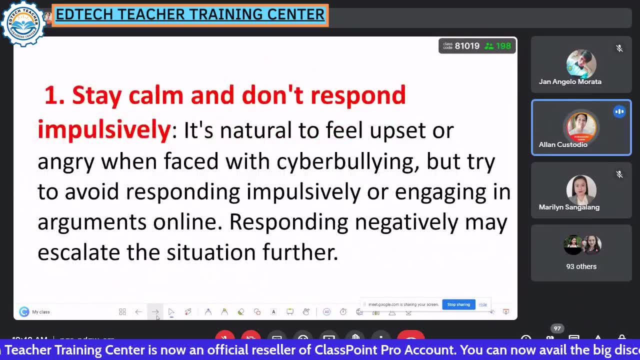 pag ikaw ay inap, eh Tama po ba Siyempre gagante ka. eh, Usually ganun, Pero hindi dapat yun. We need to stay smart and alert. Calm Tapos hindi naman na. calm ka, eh, hindi ka. 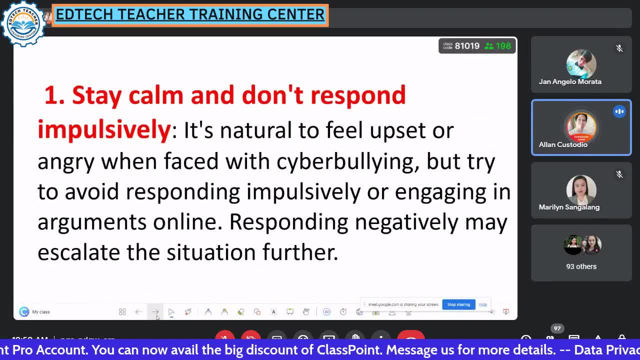 nalalaban. Ang gagawin mo doon: nag-screenshot ka, nagpe-prepare ka, Nagpe-prepare ka para ipagtanggol yung sarili mo. Ipe-preserve mo, yung evidence mo, screenshot ka. 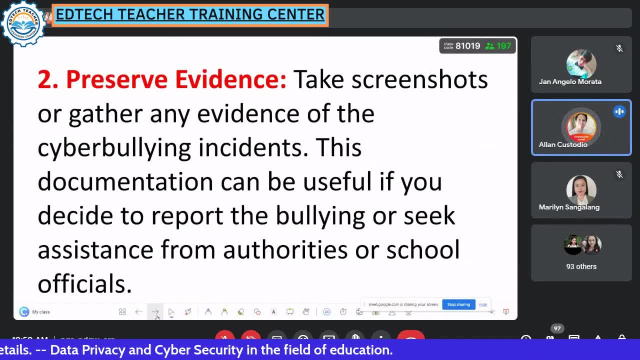 dyan, tapos lahat ng authorities na pwede mong bigyan nun na pa-possible na matulungan ka ay ibigay mo Meron, ako sa inyong payo, mga kabataan, Pag nabuli ka at hindi sure. 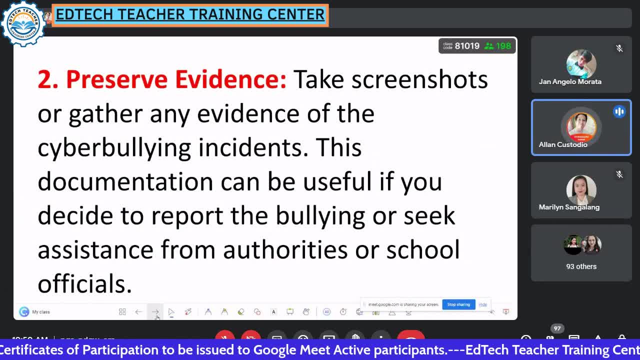 na kaibigan mo, pagsasharean mo ng evidence. wag mo nang ibigay, Kasi pag nakaabot yan sa nagbubuli ay meron kang ebidensya. o binubuli, Ms Kwan, kaibigan din naman pala niya. 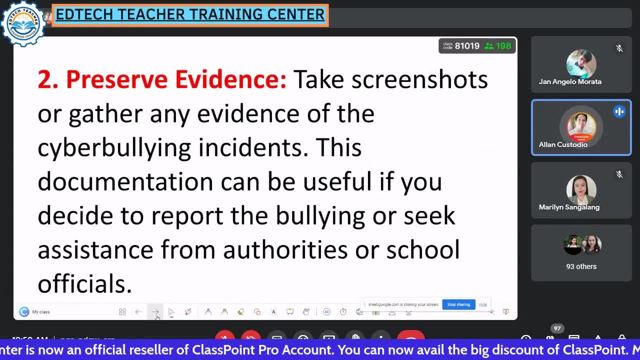 Ay, biglang babae, biglang gagawa ng solusyon at hindi mo na makakantam ang ustisya mo. kung sakaling umikot-ikot na mahihirapan na naman Laging. tandaan ang pagsasharean ng. 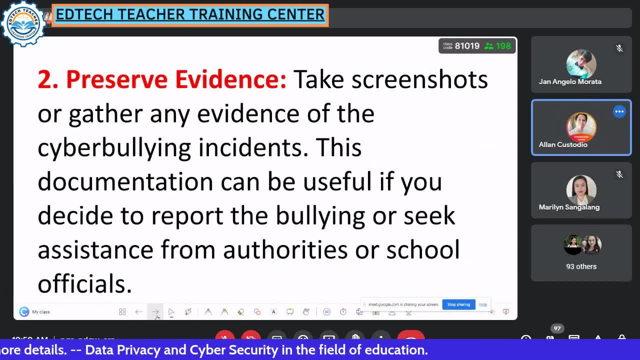 evidence ay authority, yung nababagay, Kung okay kay ma'am, sa guidance sa principal, kung sa school level, wag agad-agad sa kaibigan: basta-basta, Ay naku, kakalat lang. 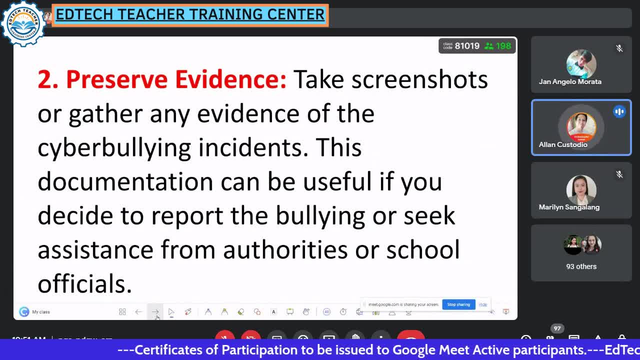 yan, tapos mai-issue ka pa. Uy may kumakalat na chat mo kumakalat. Uy meron ba, Sige, gumawa ka na ng ibang account mo. Sabihin mo dami account. 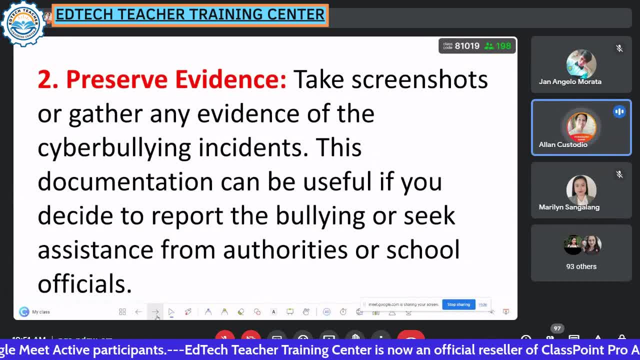 yun tapos sabihin mo: hindi ikaw yun O diba ang talino ng mga nag-ano. Alam ko yan. eh Kasi ICT din po ako. Alam ko yun. Ngayon ang hirap. 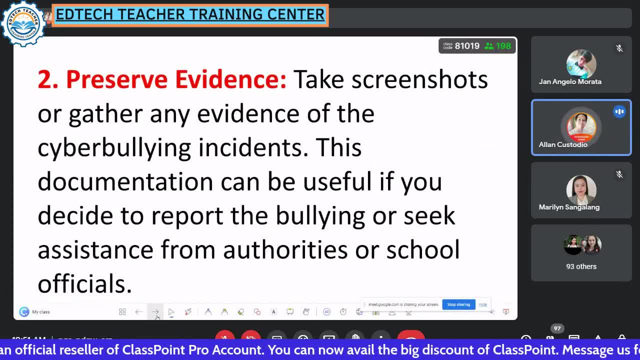 kasing kapag natapatawag din kami sa guidance or something, ang hirap kasing i-trace, Tapos ang dami nilang mga palusot, eh, Hindi daw sila yung kuno, hindi daw sila. 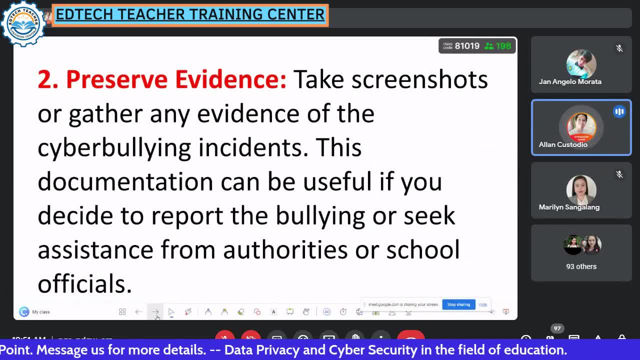 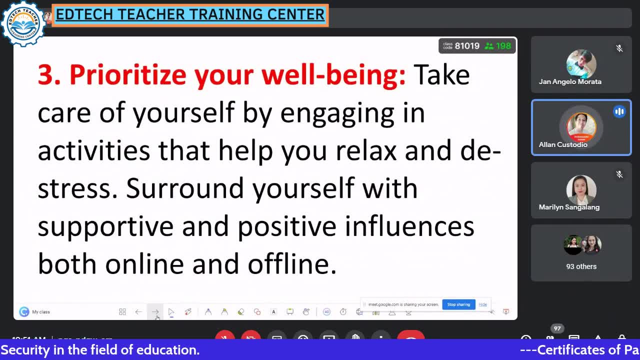 Tapos dami account wala daw picture, yun hindi daw sila Diba. Kaya pag nag-share ka ng evidence, wag basta-basta sa ibang kaibigan, Sa proper authority. Prioritize your well-being. 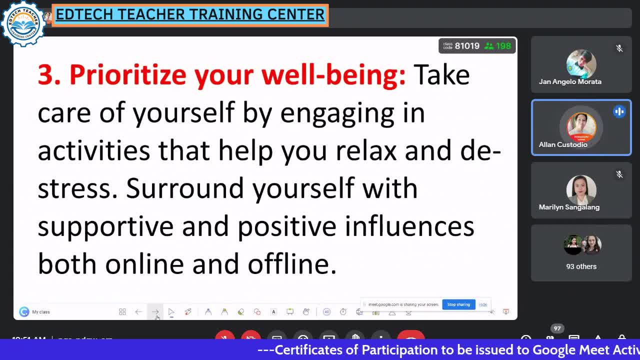 So mag-relax ka, Huwag mong patulan. Alam mo hindi mo ka-level, Mabuti ka. Alam mo, ginagawa mo Sa tamang panahon, reklamo mo At doon mo ilabas ang. 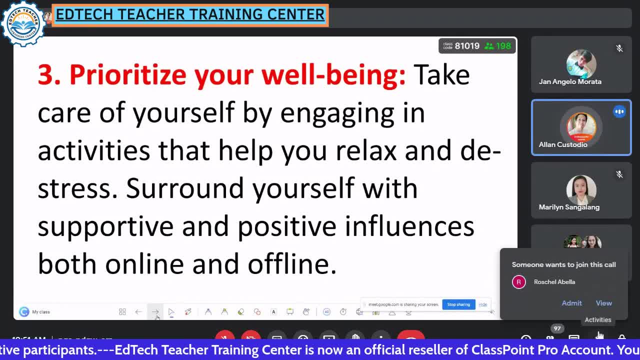 mga natutunan mo sa buhay, Especially sa webinar na to At doon siya tatamaan at wala kang sabit, Usually nababaligtad pa, Kasi sumagot ka, Eh ma'am tingnan niyo, Sinabi niya. 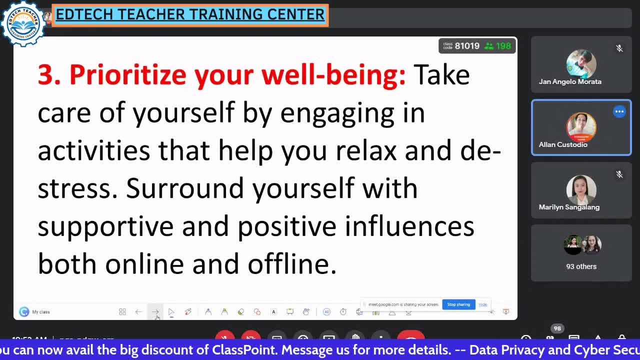 sa akin: eh Buong lahi ko nga daw Ganun-ganun, eh Kesok ganun daw, eh Kami daw ay hampas lupa. Eh, ito lang naman po sinabi sa kanya. Nabaligtad pa tuloy. 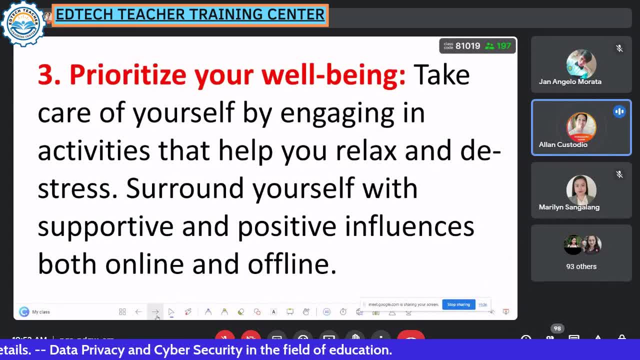 So dalawa kayong may consequence. Ang iniisip natin dito is: wag mo nang gayahin. Ang isang mali hindi matatama ng isang mali, Eh ginantihan, Alam ko natitrigger kayo mga. 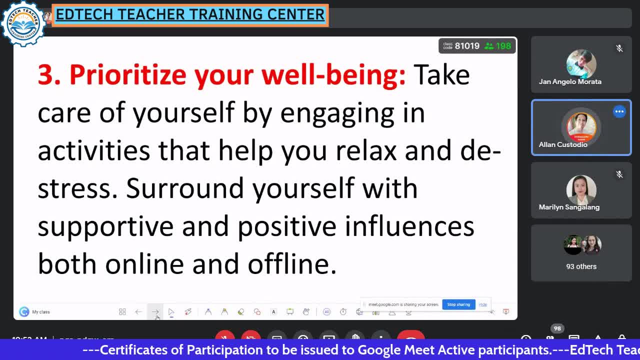 kabataan, Pero hindi dapat gaganti. Ang kailangan is smart ka lang at alert Pag nalagpasan mo yan. matured ka, Nagmamatured ka na bilang mabuting individual. Ha Lalo na po nasa government employee. 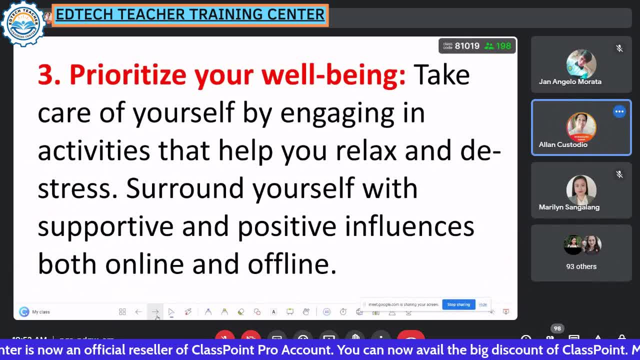 Rat-ratan talaga, eh. Eh may sinumpaan tayo sa ethic of code diba Na mataas ang tolerance natin. Ano po bang ginagawa sa polis? kapag ang polis ay mababaang tolerance, Sinisibak agad. 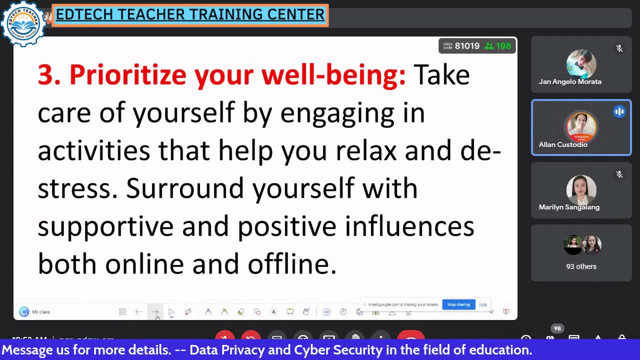 Sinisibak May pinatay, May itinutukan ng baril Example: Ganun Sibak agad. yun Kasi tolerance po, eh Kaya believe din po ako sa mga talagang nakakayanan magpigilan. 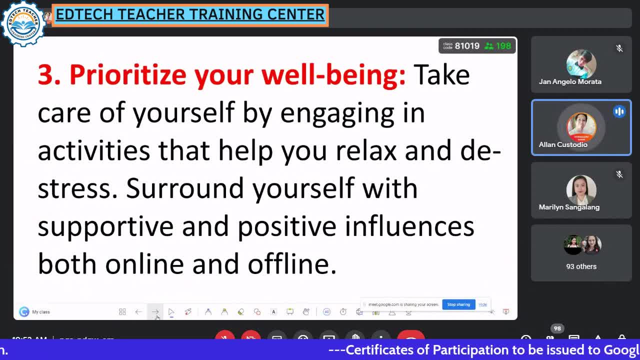 Ang hirap po nyan. eh Siyempre minamaliit ka na, eh Inaalisposta ka, Pero sa huli ang ustisya sa'yo, Pag wala ka talagang sabit talaga at nakuha mo. 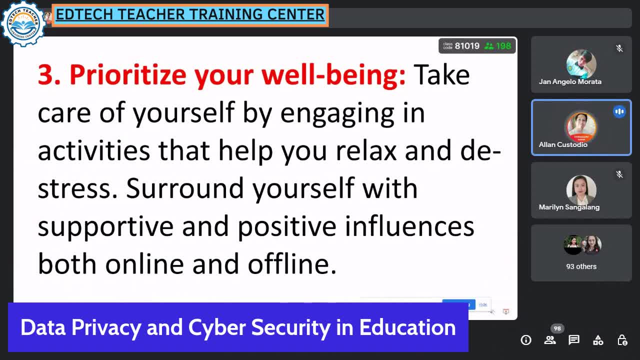 ebedensya makukuha mo yan. Kung di mo makakuha ngayon yan o sa ibang bagay, Alam na eh Nakikita ng Diyos yan Ngayon, ayan At marami pa po dito May katuloy. 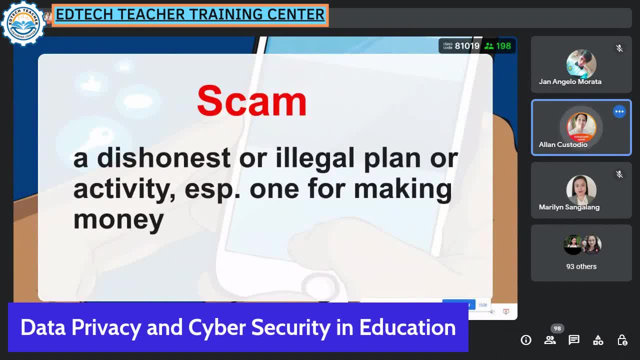 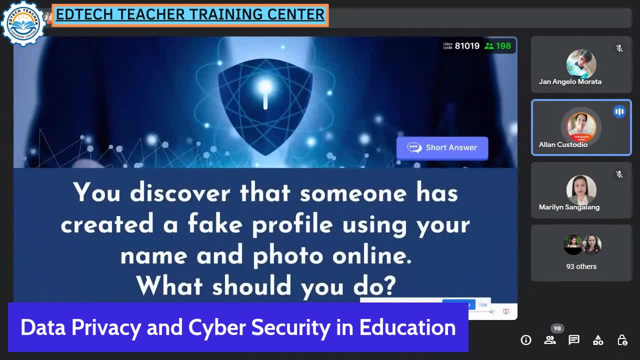 pa po pala to no Pahapyawan natin kasi sabi ko talaga ay eleven, tayo kakain. eh no, Ingatan ng mental smell. Work smart, not hard. Correct, Sure dyan. Okay, Mga scam natin Marami. 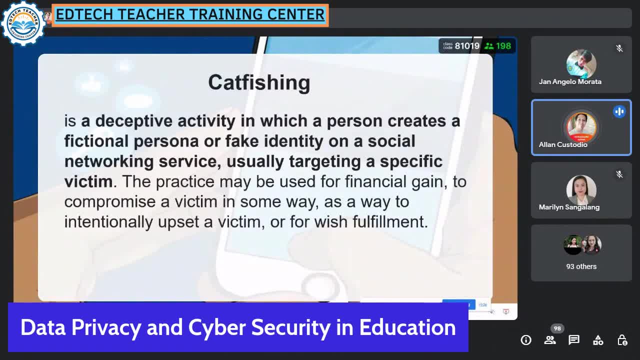 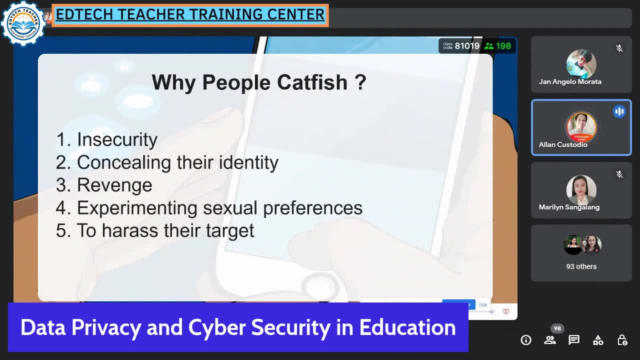 ditong mga tanong: Cut phishing, Pahapyawan na lang natin Itong cut phishing mga poser Ayan Kaya mga poser na yan gusto nilang may insecurity, concealing identity, Kasi hindi pala talaga lalaki Gusto. 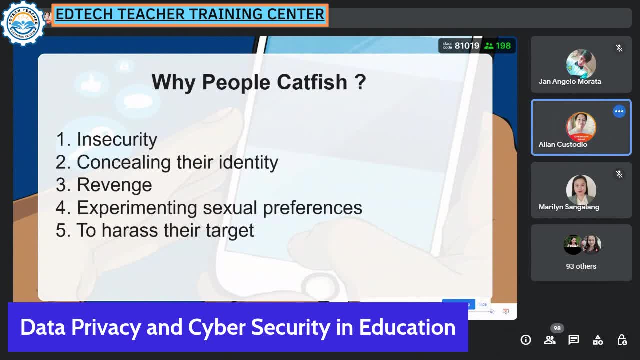 nilang maging babae Revenge At may mga hinaharas na target Yang mga yan dapat kapag inorient yan. huwag nang gayahin yung mga ganyan Tapos kapag may mahuli sabihin. 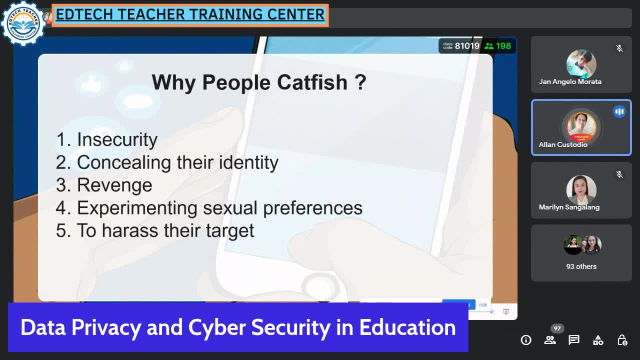 sa school policy kung anong magiging sanction sa mga yan at pag naghaharas yung mga yan. Yan ang dapat inculcate sa umpisa ng klase. Not only yung personal, Kailangan inculcate pati yung online. 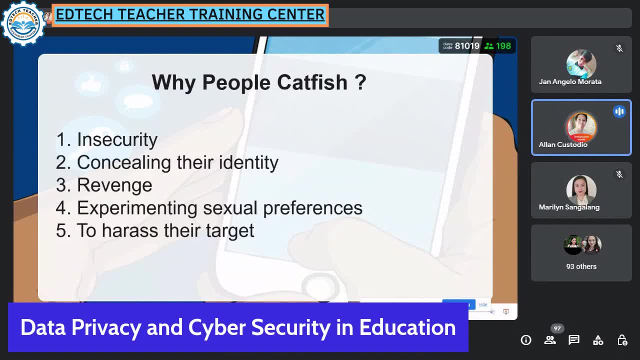 Sa online. saan ba mas marami nag-aaway Online personal? Sa online muna nagsisimula yan Gatong-gatongan. Lalakas na yung apoy Ayan na Buong school na Kada. 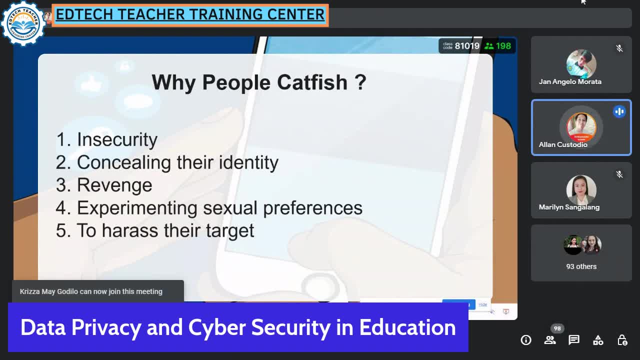 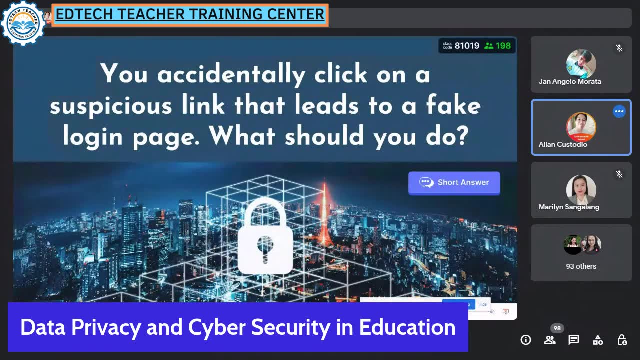 section nag-aaway na sa isang chat, Sa isang post, Mga kalungkot. No, Dahil doon sisikat yung school. Siyempre, sa solusyon ng school ang laking paruhisyo Lalo sa. 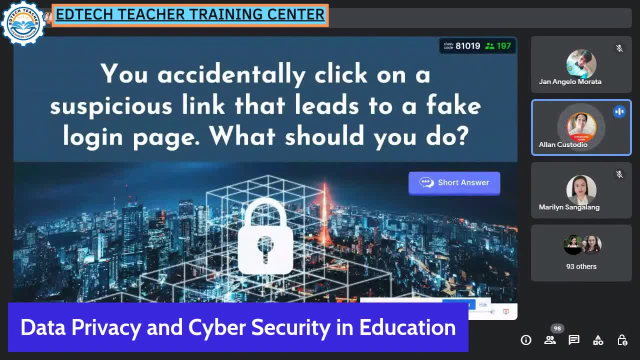 guidance office. Ang dami na nga doon minsan Meron pang ganun na kumakalat na video, kumakalat na suntukan na video, kumakalat na kwan. Lahat ng yun, lahat ng. 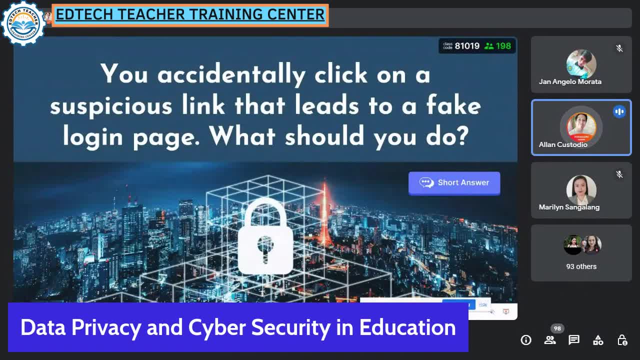 magpo-post na yun. bigyan ng sanction. Bigyan sa school policy Kailangan ma-orient bagong mag-start yung klase nasusunod na taon. Okay, Kaliwa-kanan ngayon mga. 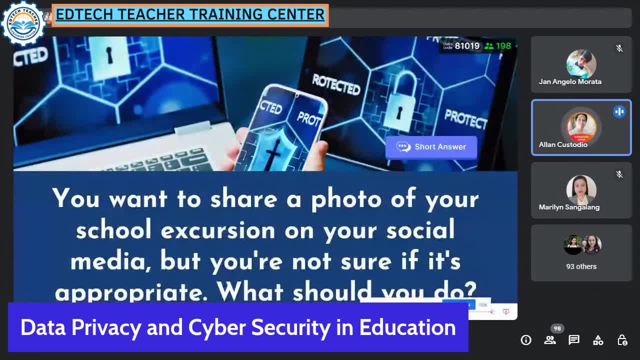 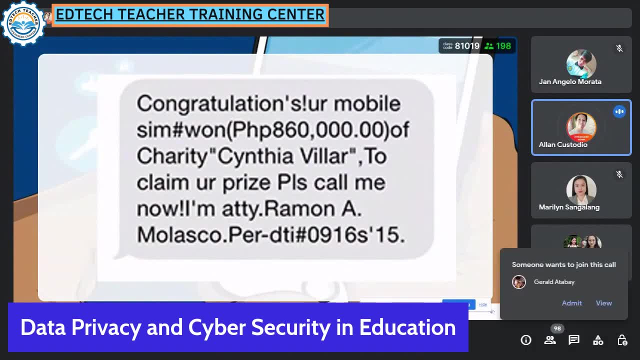 scammer. Correct po Ngayon. ano ang dapat gawin sa mga scam? Ismishing sa text yan, Phishing sa email: Ayan yung ismishing Yung ganyan, walang ganyan. 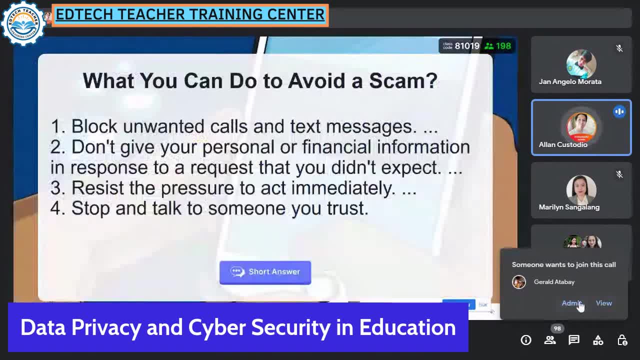 At nung gagawin yan email naman yun Eto gagawin natin Auto-block agad po yan Tapos hindi bibigay personal, Tapos ire-recess natin. Oo, nanalo ko Hindi po Dapat. 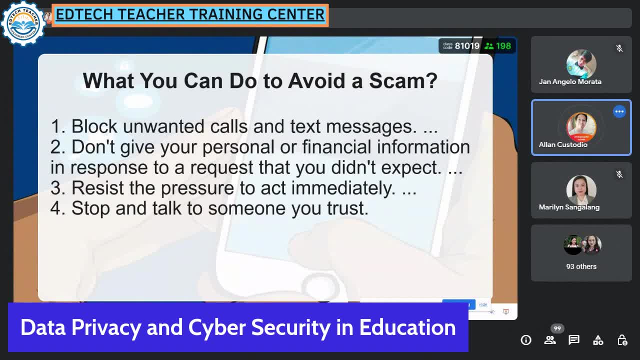 mag-isip pa rin So good to be true. Baka yun ay scam. Kapag hindi alam gagawin, magtanong sa dapat na nakakaalam. Meron nagsend sa akin ng padala Ikiklik ko to Ay wag. 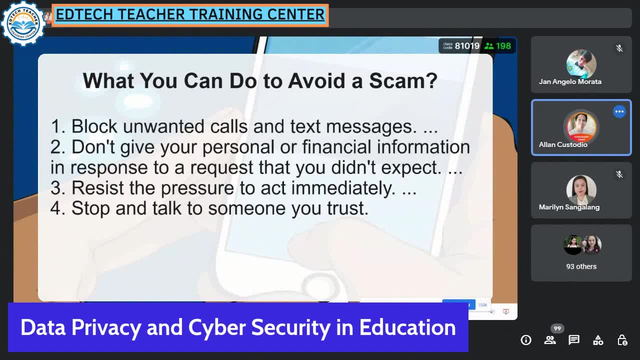 friend Wag Scam yan Ganun Alam nyo naloloko Mga lola pamilya. Kaya eto gusto ko pa share to eh Sa mga pamilya. Bakit po ba Tayo kasi mga techie? 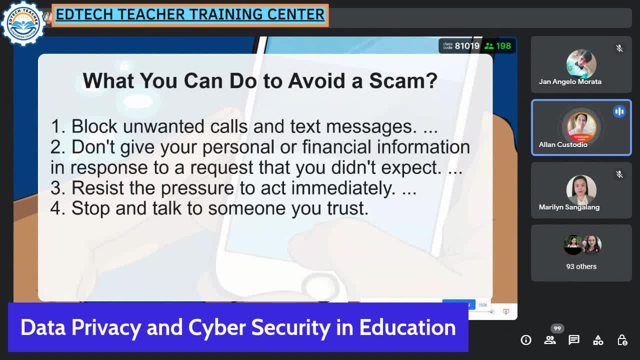 Yung mga lolo at lolo natin nanay tatay, hindi sila techie Oo, may nagtitiktok pang ilan-ilan, May nagtitiktok pang nanay tatay, Pero karamihan wala silang ganun. 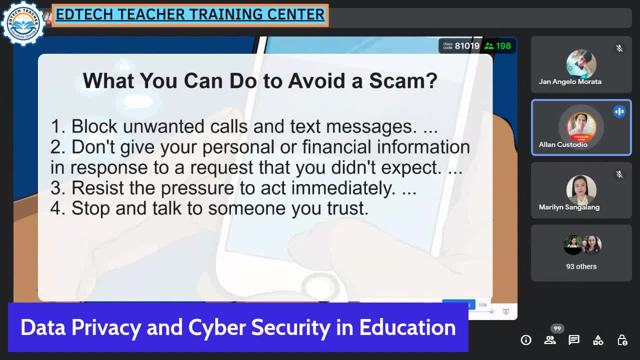 Diba, Mga kabataan, tanoyin ko kayo, Ano yung cellphone nyo ngayon Touchscreen? Ano yung cellphone ng nanay nyo? Halos hindi touchscreen, Or may touchscreen sila Hindi. 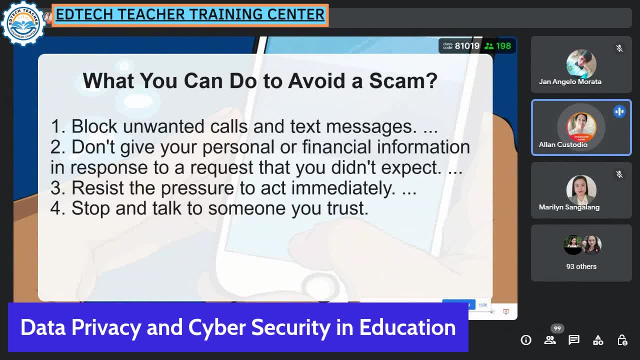 mabigat, kasi ipinundar pa ng nanay nyo yung magandang cellphone nyo para mag-aral kayo, mag-online class. kayo, Diba, Ngayon ibalik nyo yung ano natutunan nyo. 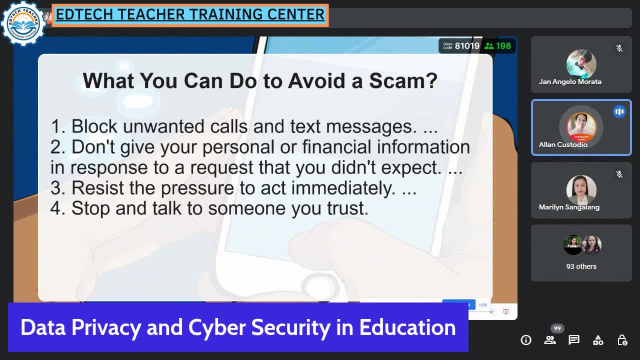 Turuan nyo sila, Activate nyo yung factor, ayusin nyo Lahat ng scam, ituro nyo. Huwag i-click Yung mga cellphone ng mga kabataan ngayon. mas maganda pa minsan sa nanay. 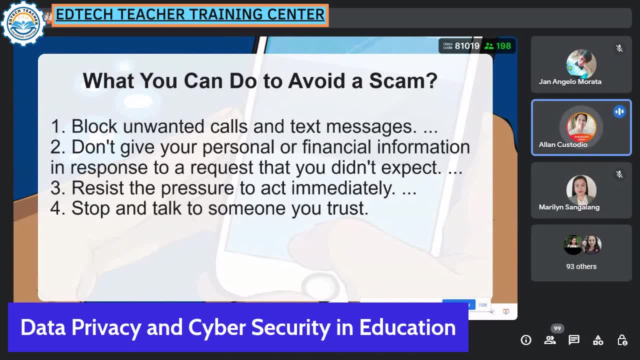 nila Sa pinagpawisan at pinagpaguran ng nanay nyo. napakaganda ng cellphone nyo, Diba Totoo O ngayon, ibalik nyo yung mga natutunan nyo sa school na magaganda. 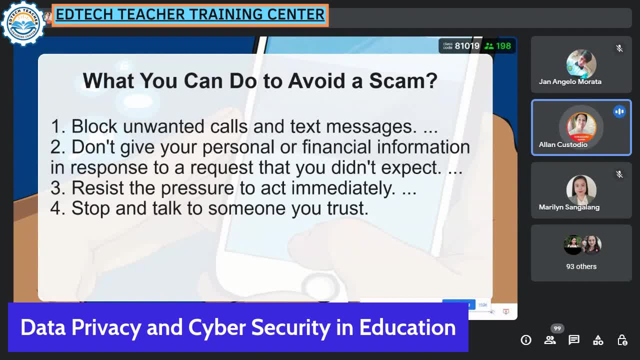 para sila itulungan Diba Kagaganda ng cellphone ng kabataan ngayon. Mas maganda pa nga sa cellphone ko. Totoo lang po yan ha Sudyante ko din na iba O. 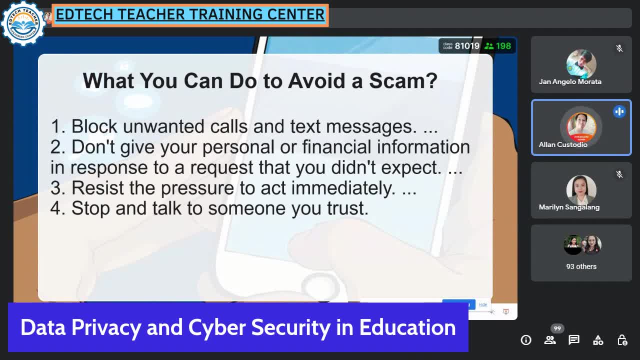 yung mga magulang nila. nakikita ko mag-meeting yung iba Hindi ganun kagandahan eh Kasi nagsakripisyo eh O turuan nyo ngayon mga nanay tatay nyo ha. 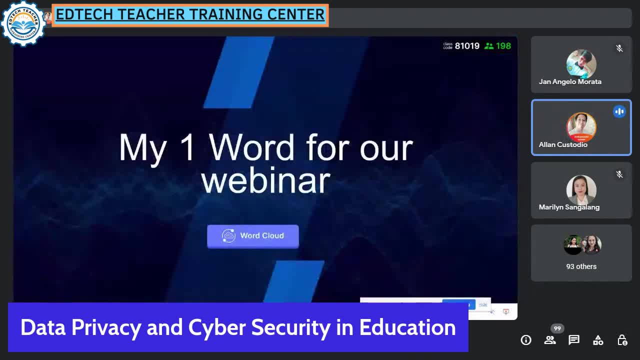 Yung iba O Totoo yun Ngayon. ano po ba isang word nyo sa webinar. Matatapos na po tayo. Nagpapasalamat po ako sa inyong lahat, Katulad ng promise ko. 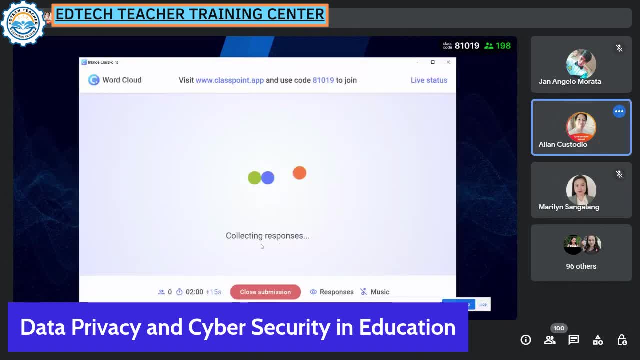 eleven po tayo magtatatapos. Ano po ba isang word nyo sa webinar. Thank you, thank you po No Umaten. ngayon, Sana maraming kayong natutunan. Ano yung isang. 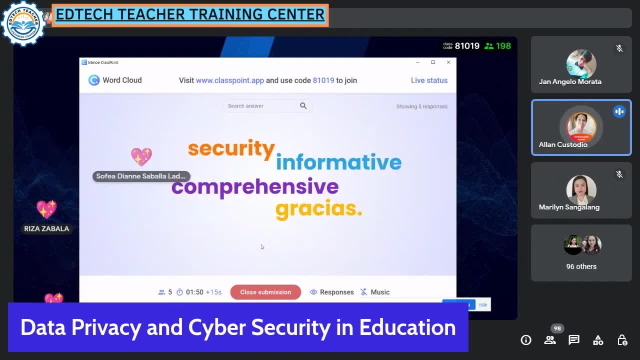 word nyo sa webinar, Pwede po din dito sa ating comment section: Ayan, Informative, amazing security, gracias, Gracias, muchas Dabi yata yun sa ano, Ano ba yung gracias Spanish. 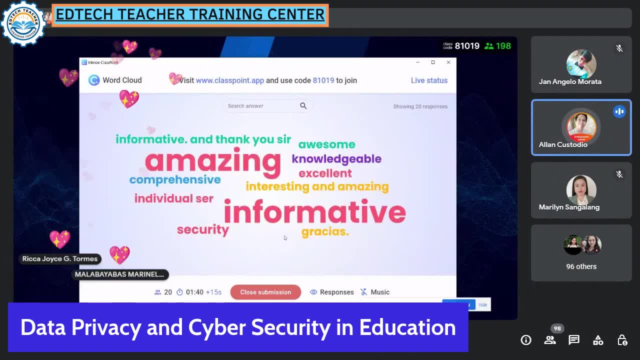 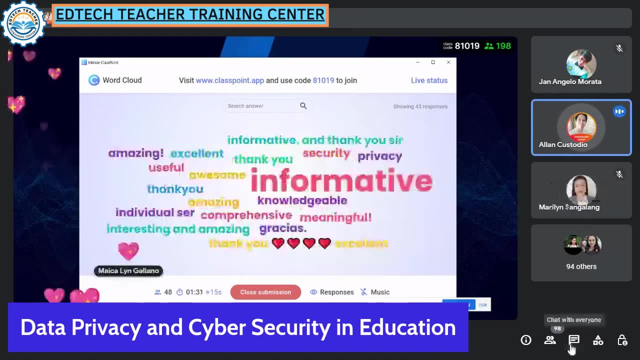 Ayan, Excellent, Okay, Individual, Okay, Ano po yung isang ano nyo sa webinar natin. Thank you, Thank you, thank you. No Informative relevant. Thank you, thank you, At naka-attend po kayo. 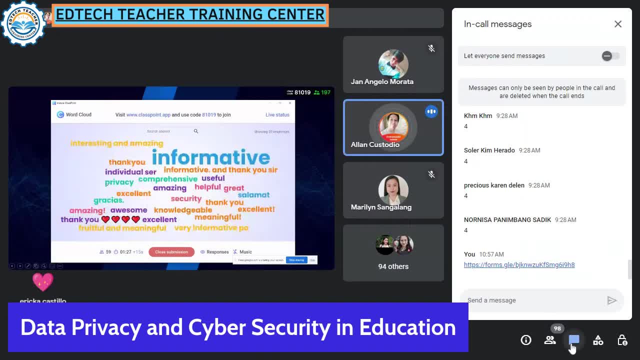 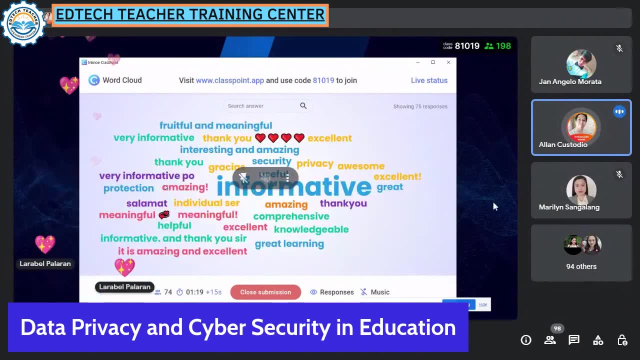 sa ganitong webinar At maraming salamat sa ating Google Meet. no, Ang daming sumasagot Um. thank you At hatid po ito ng EdTech Training Center with Sir Director John Morata. no. 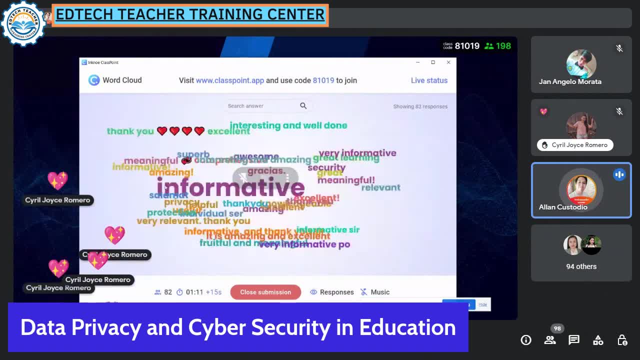 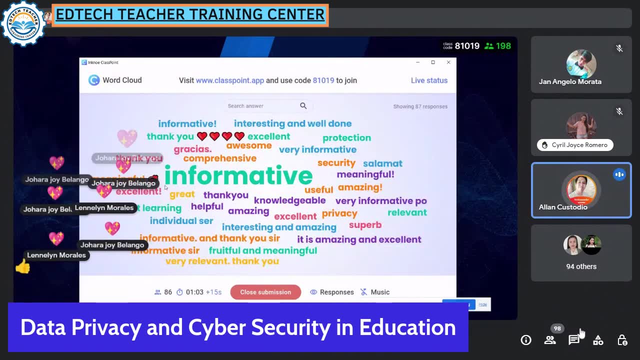 At Sunday, pero andito kayo upang makinig. Pwede itong ulit-uliten At very much welcome po kayong. ishare like follow page: EdTech Training Center. At ang mula po sa puso. 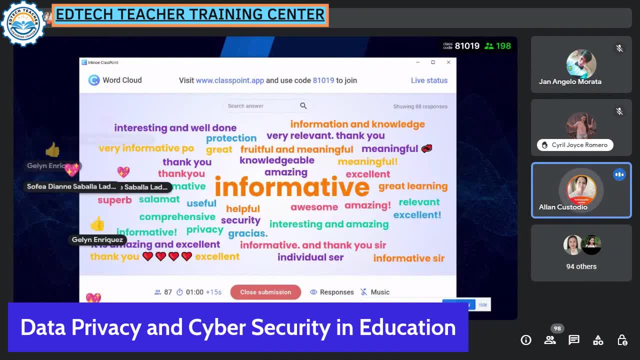 namin, mula din sa puso ko, thank you, At huwag po kayong magsawa. Maraming ba pong mga darating na training. Maraming, maraming salamat po. Ingatan po natin data. 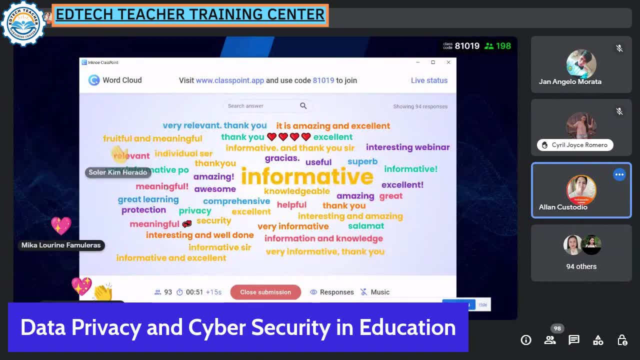 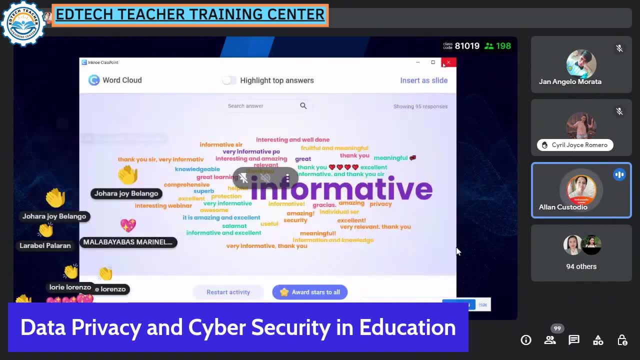 privacy At ikaklose ko na rin po dito sa submission And ayan Thank you po. no Very much Ayan Sa pagtatapos po natin Ayan Shout out po sa inyong lahat. Thank you po. And. 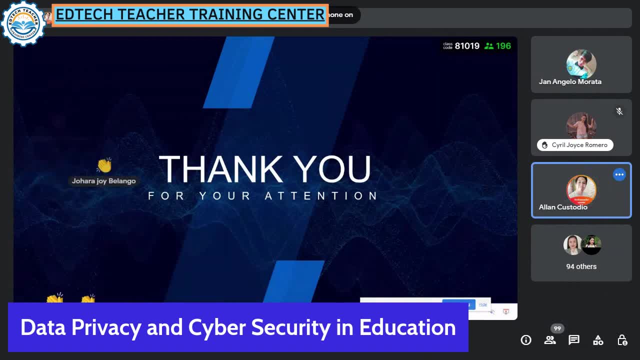 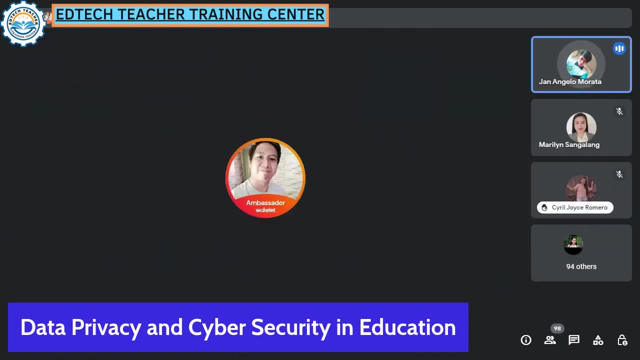 maraming, maraming salamat So ayun. Thank you, Sir Alan, for sharing your expertise with us. That is all about the data privacy and cybersecurity and how to protect and secure our precious private data, details and information in different. 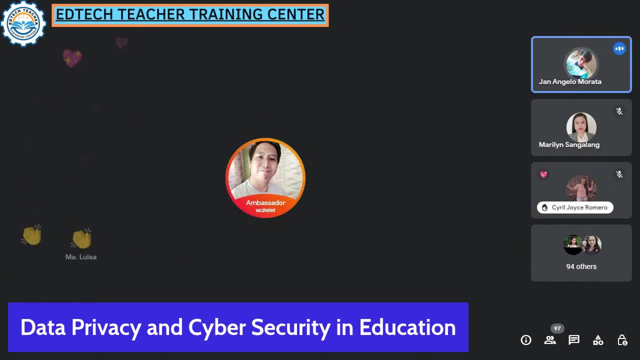 situations. So with that po, that ends our webinar for this day. Thank you po sa ating mga participants And also sa ating mga Google Meet participants. the link is already Okay po So ayun, So the. 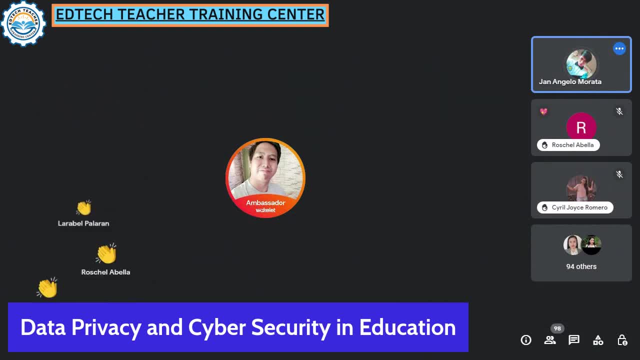 certificate link is already on the chat box. So ayun po, The certificate link is already on the chat box po. So this is only for the Google Meet participants. So nahin po muna natin yung mga Google Meet. 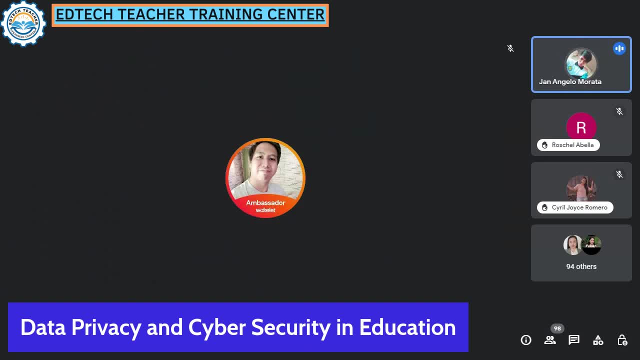 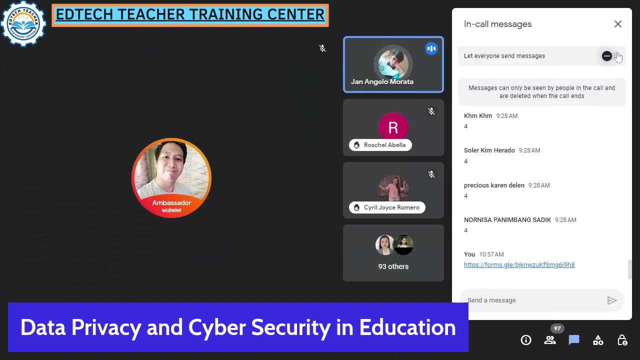 participants, because they are the one that is really registered in this webinar. So yung mga nauna. So this is first from first services po. So with if you have questions with our source speaker, on ko na po yung ating chat box for our. 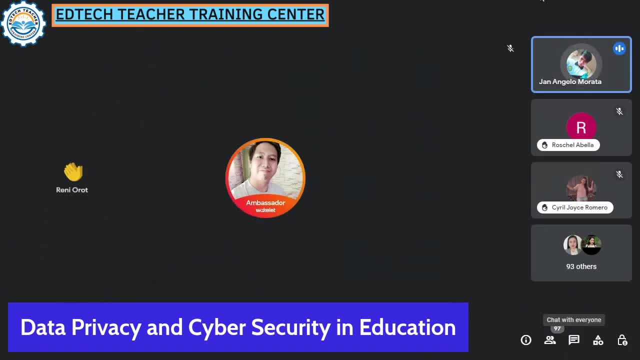 questions, So chat box po natin dito sa ating Google Meet. So yung mga nasa Facebook Live participants po actually na-instruct, ko na po dito noong nag-post kami for this webinar, noong nag-announce kami. 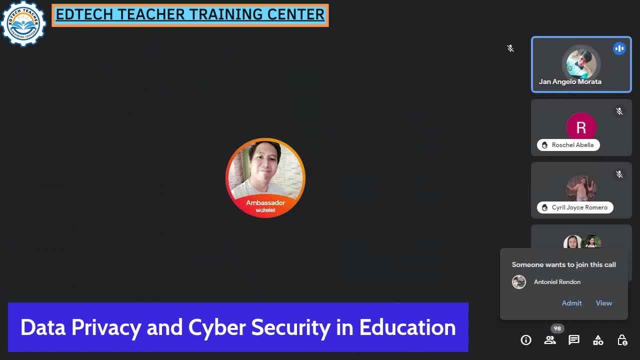 is that only Google Meet participants will be the one to have or to be issued a certificate of participation. But sige po, we will share also the link sa comment section sa Facebook Live. But priority lang po muna natin yung Google Meet. 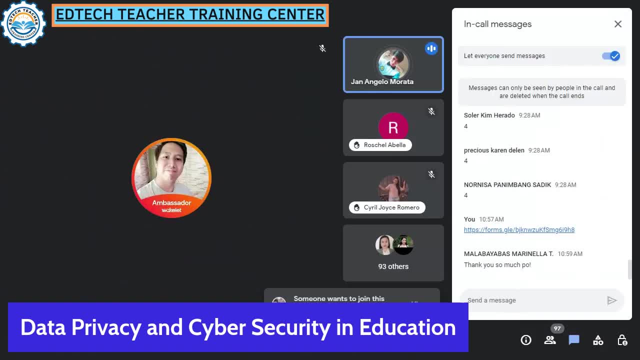 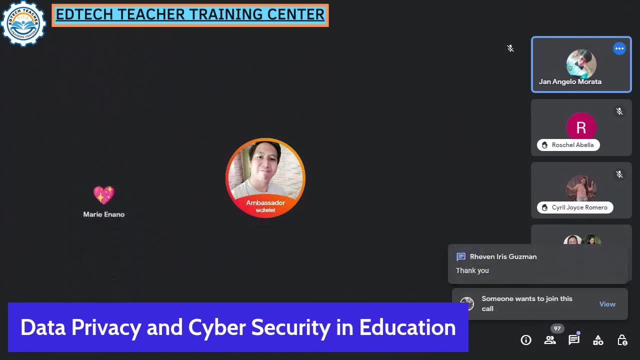 participants. Okay po questions po. May questions po ba tayo to our source speaker. So again na-instruct ko na po kasi ito from the very beginning na only the Google Meet participants are the registered ones. So sila lang po. 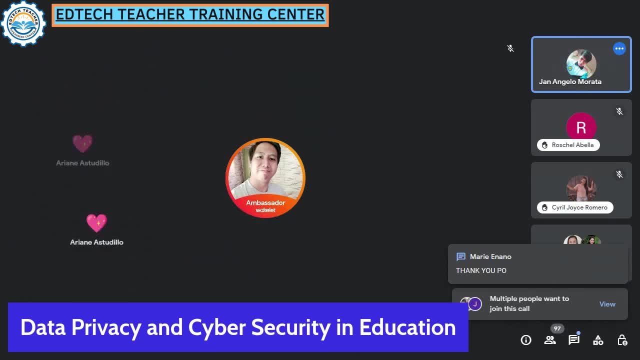 dapat yung may certificate participation. Okay po, thank you for being with us. po Siguro wala naman po tayo siguro mga questions from our Google Meet, So ayun wala naman po siguro. So thank you very much po, Sir Alan, for a very 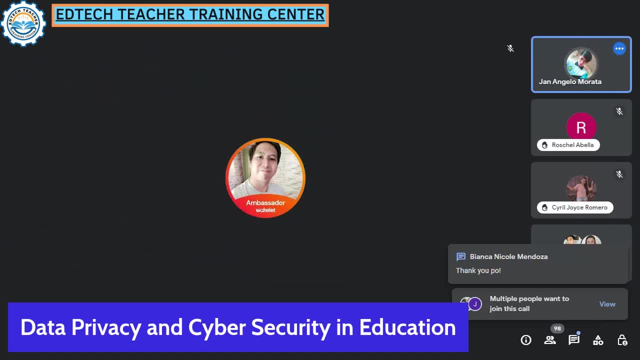 detailed, comprehensive discussion about the Data Privacy Act and Cyber Security. Thank you po, And with that po, that ends our webinar po. Thank you po. Thank you po. thank you po. Ingat po tayo lahat. Thank you po. 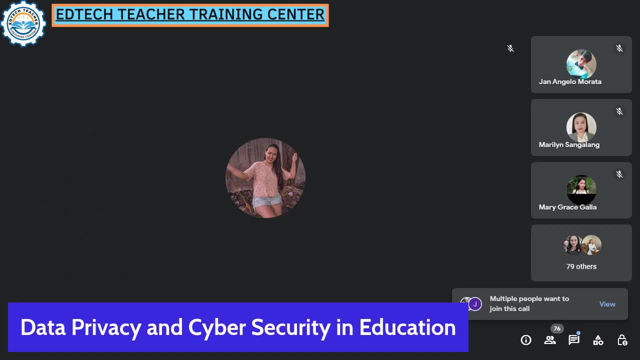 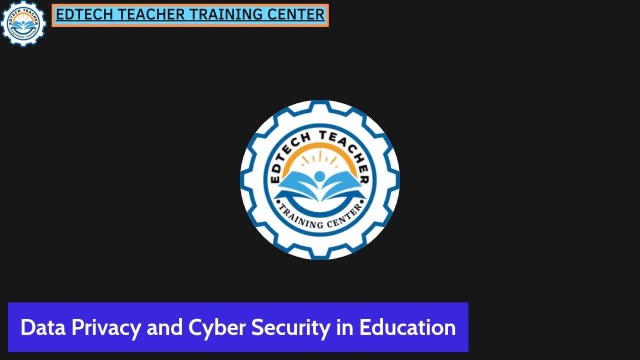 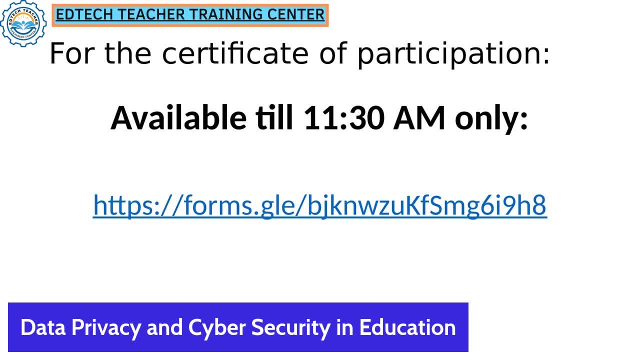